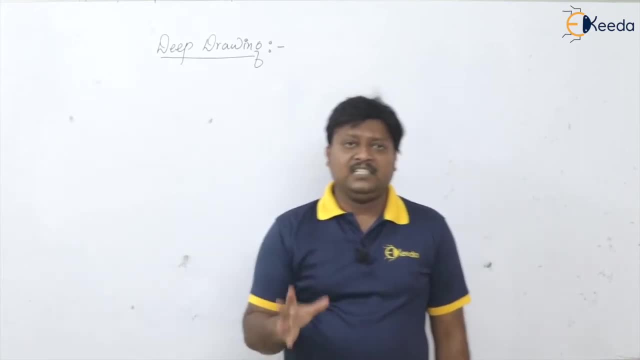 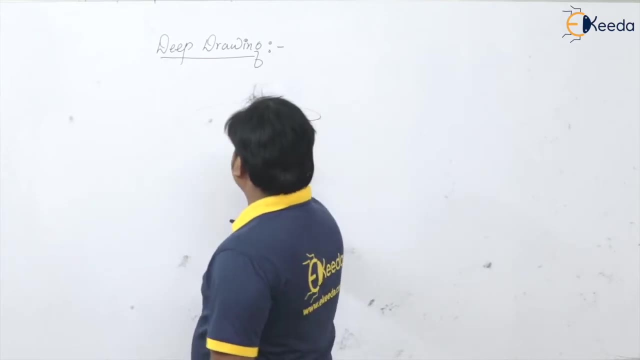 die combination to produce these cup shapes or the shells, or the shell like article. so this is: say the given blank is available with us. okay, with the thickness, T and diameter of the blank, say D. okay. so this is again, it is going to use the sheet that is blank and punch and die. 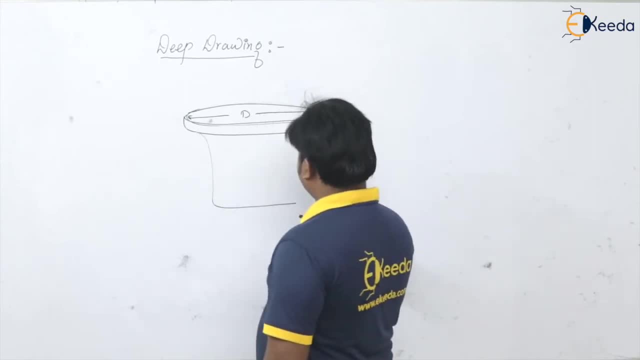 so this blank we are going to deform into the die, so to get the cup or shell like article. okay, so like this: suppose we have deformed, like up to this. so you got here. of course you are going to use the punch and die combination. so this is punch. 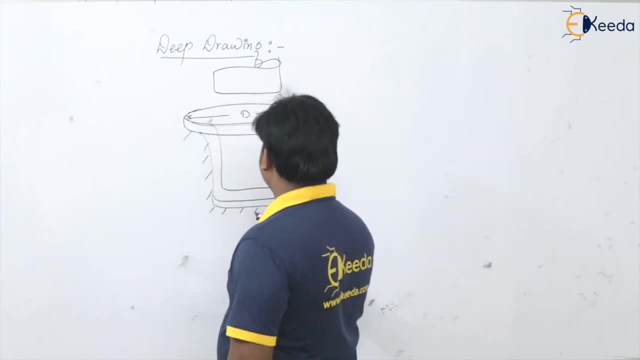 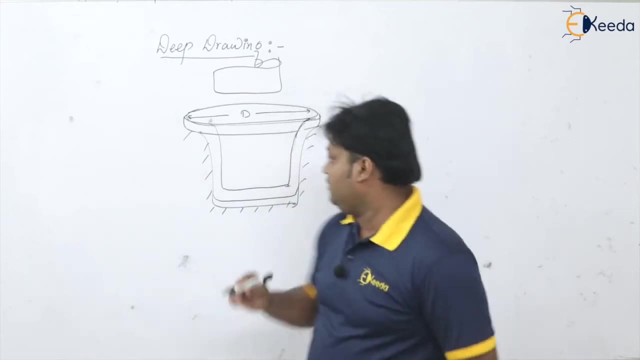 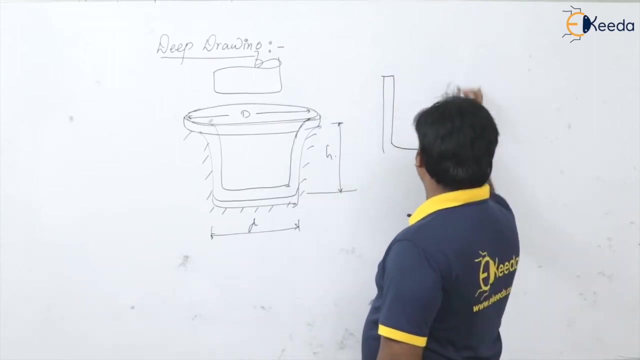 and say: this is the die. okay, so here we are going to produce a cup or a shell of diameter d and height h and height h. so simply, you can see, observe, here you are going to cup like this, you are going to get cup or shell like article. 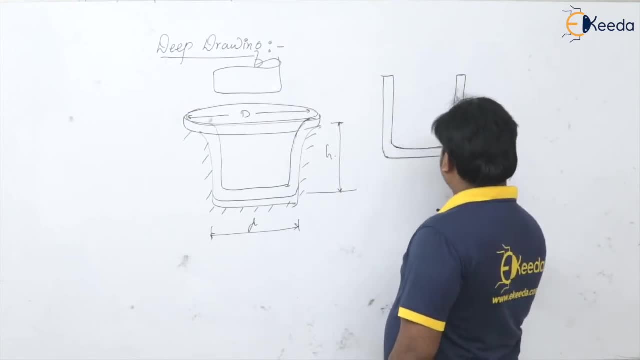 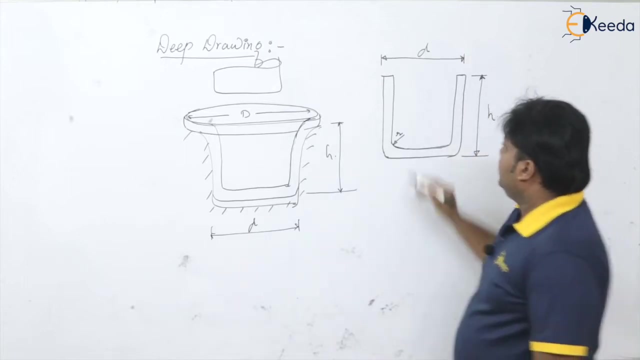 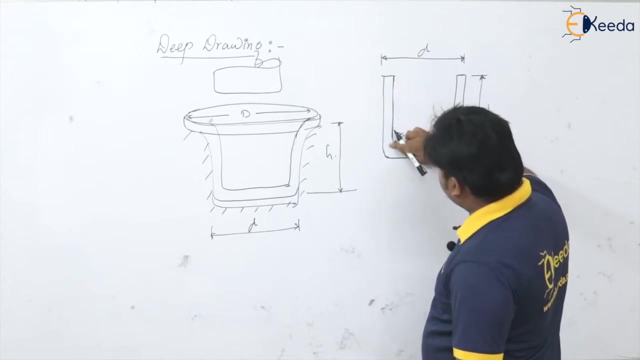 okay, of course this is the corner radius, small r. this is the diameter that you are going to produce and this is the height of the cup. okay, so corner radius is of course you have to put there to avoid the cracks or failure at the corners because of stress concentration. okay, 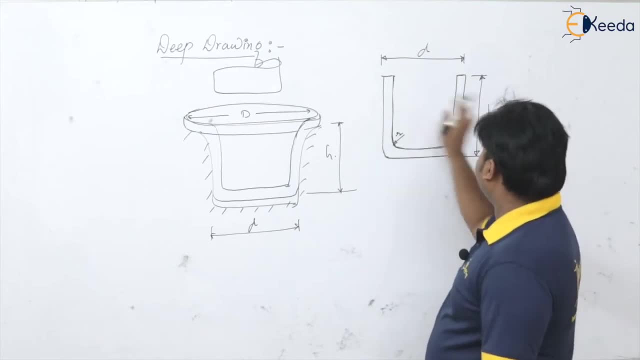 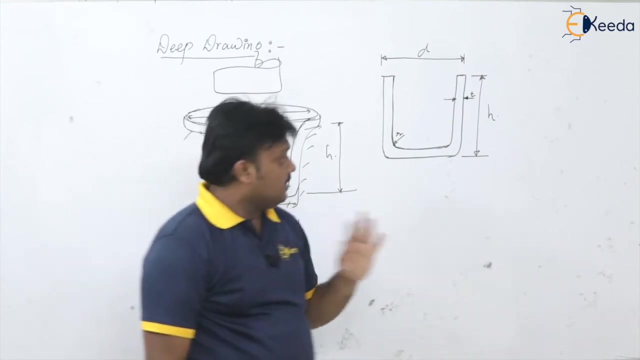 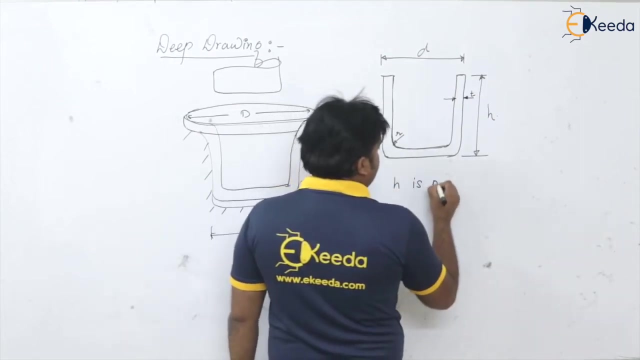 so this is the cup. of diameter d as a sheet. thickness is t in millimeter. okay, so this is the deep drawing operation. we are going to produce a cup now, whenever. see here in the deep drawing operation. the height of the cup is more than more than the half. 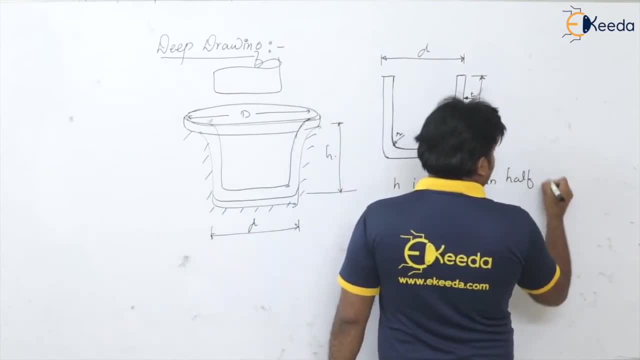 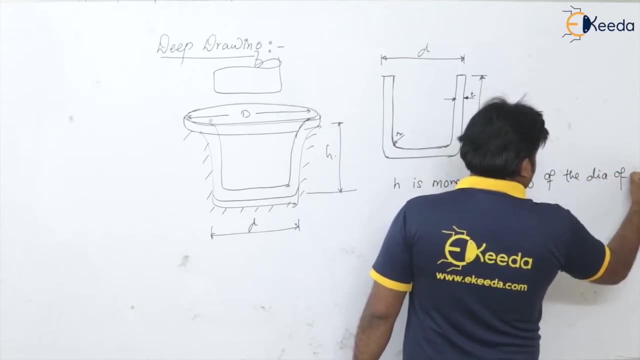 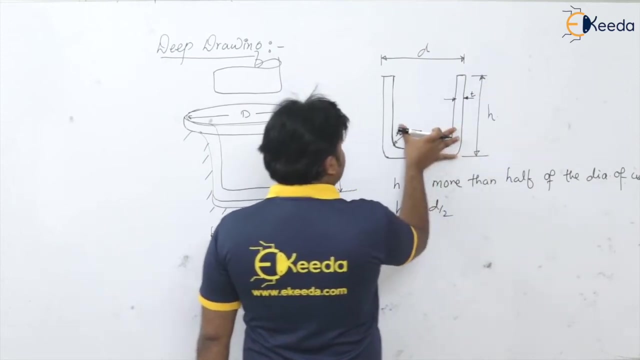 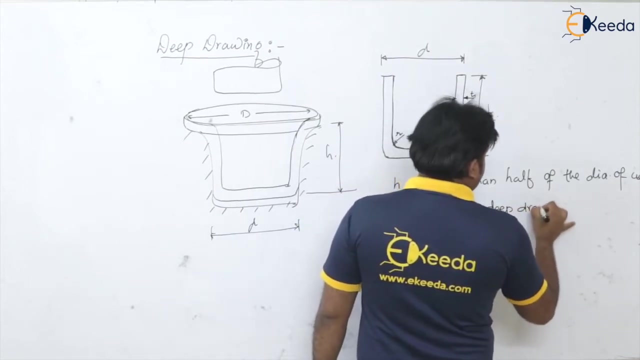 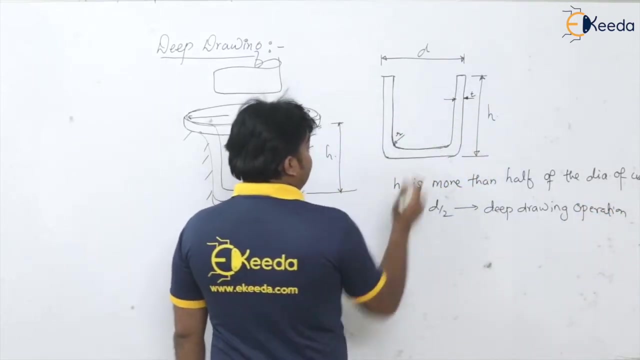 of half of the diameter of cup. okay, that is, this h will be greater than this d by 2. when this h is greater than this d by 2, it is known as the deep drawing operation. it is known as the deep drawing operation and when the obtained height of the curve is actually less than or equal to say, 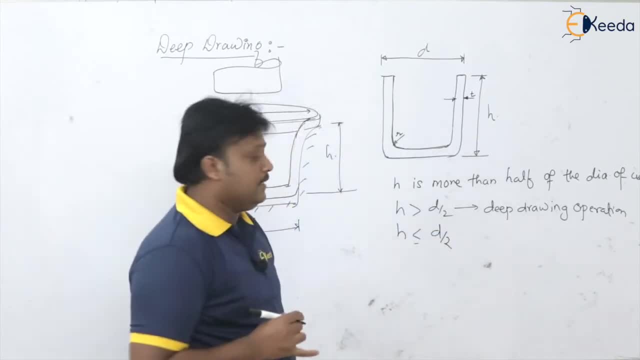 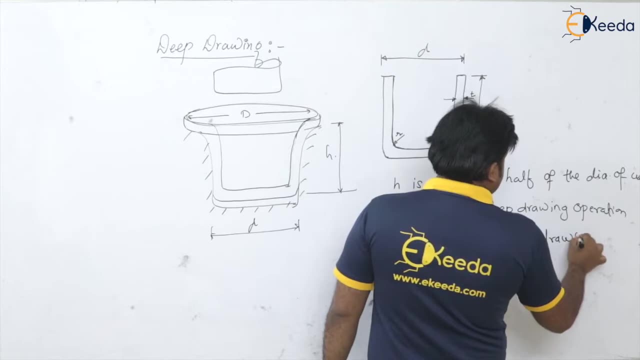 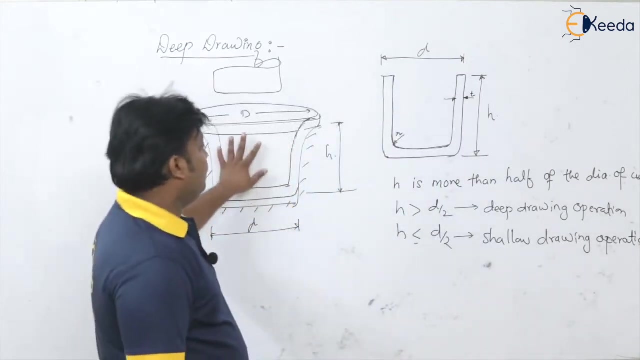 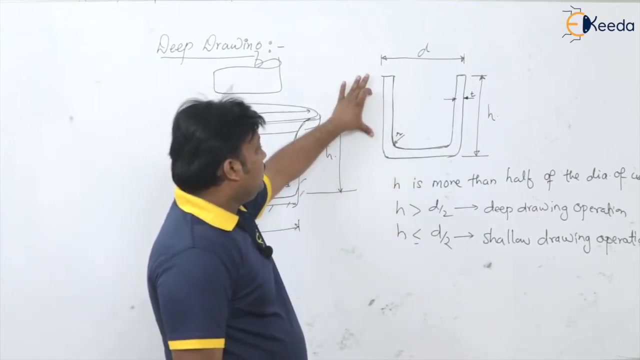 the half of the diameter. it is called it as the shallow drawing operation. okay, it is shallow drawing operation, so we are talking about the deep drawing. so definitely there will be what this h by d ratio will be more than half, that is, height of the curve will be more than the half of. 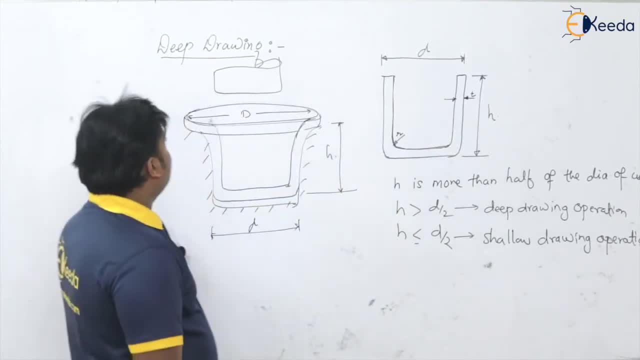 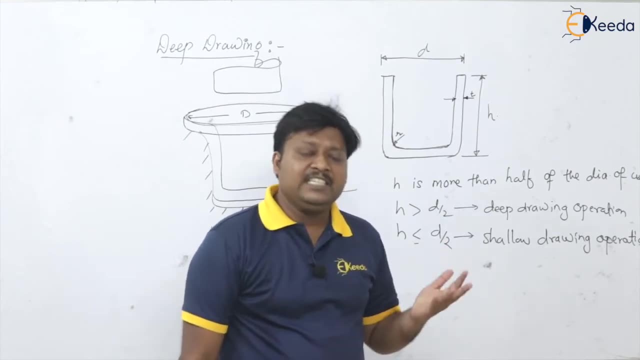 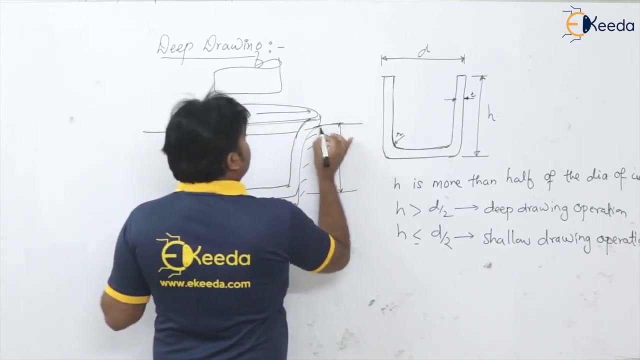 the diameter of the curve. okay, so this is the deep drawing operation. now, this is not the cutting operation. please remember. even we talk about the sheet metal. the shearing is going to happen there, but here in deep drawing operation we are not going to cut the material. so shearing is definitely. 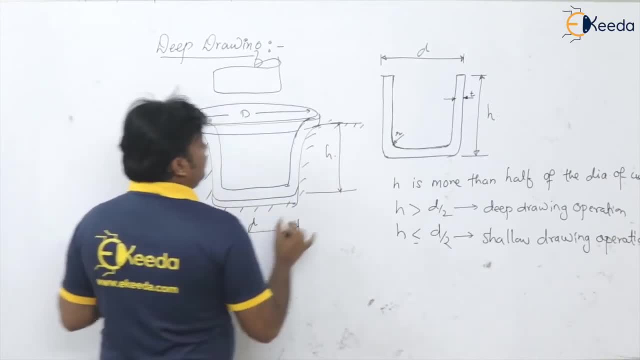 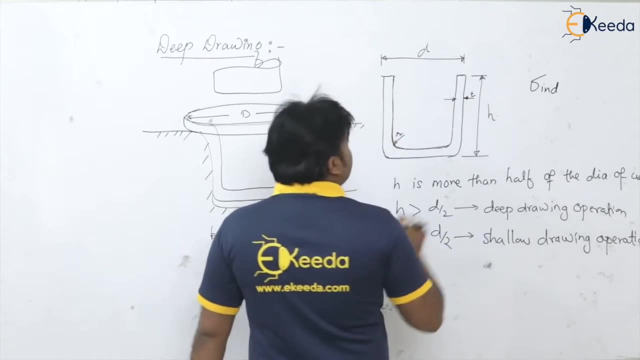 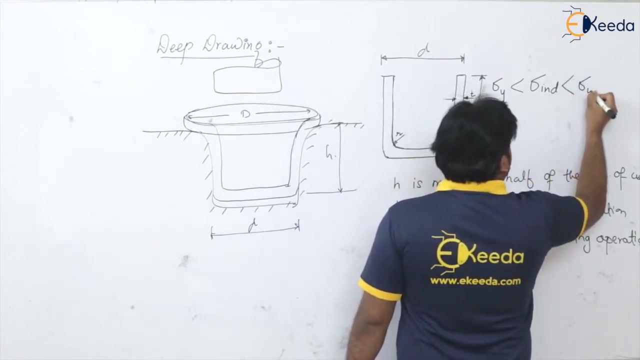 not there. so what is there? so there will be what? the deformation, isn't it? so the stress induced in this material in the deep drawing operation is greater than the yield strength of the material, but less than the ultimate strength of the material, please remember. so here we are getting the deformation, not the 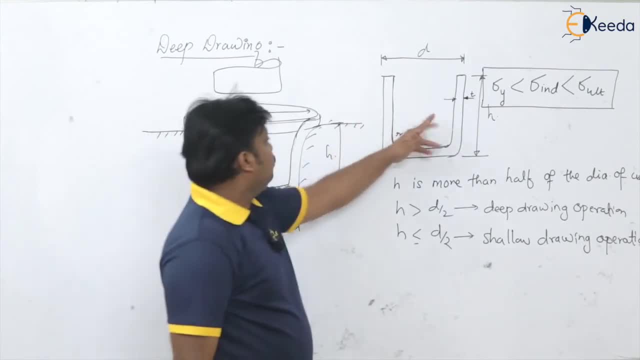 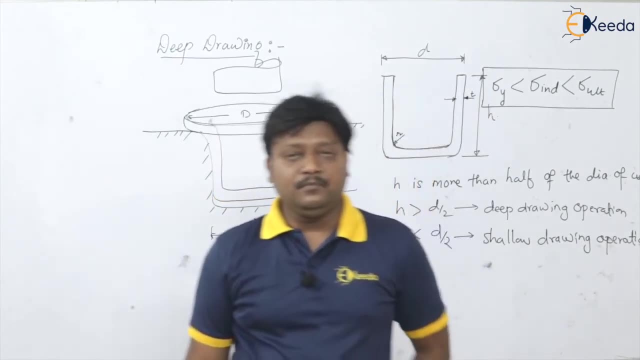 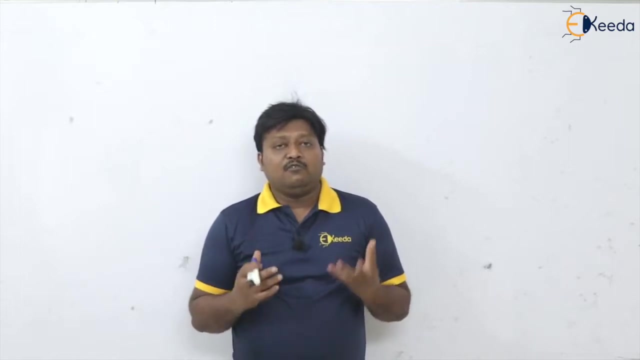 cutting action, isn't it? so whatever the stress has induced are greater than the yield strength and the ultimate strength of the material. now, the very important, the very important thing in this deep drawing operation for the designers is that to determine the size of the blank that is going. 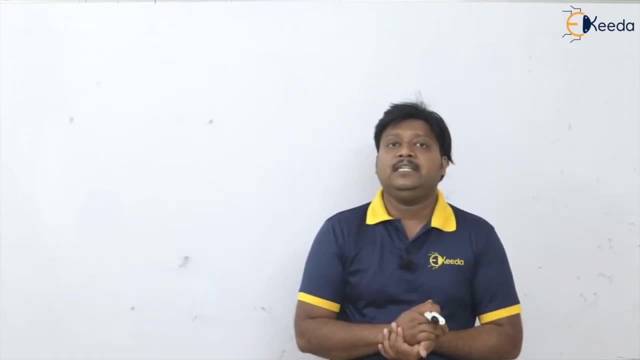 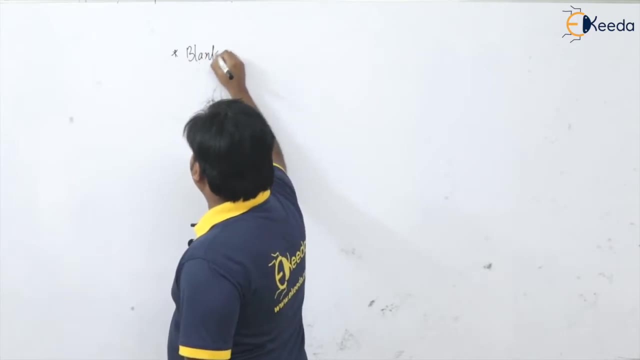 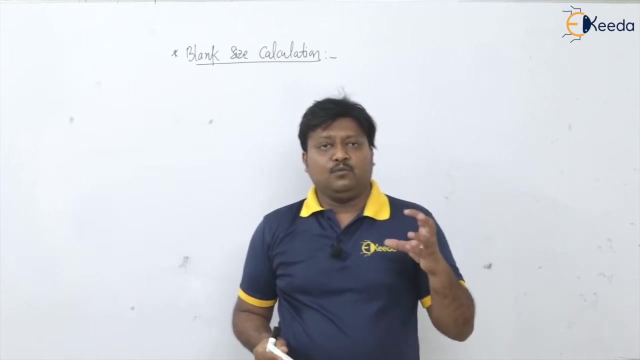 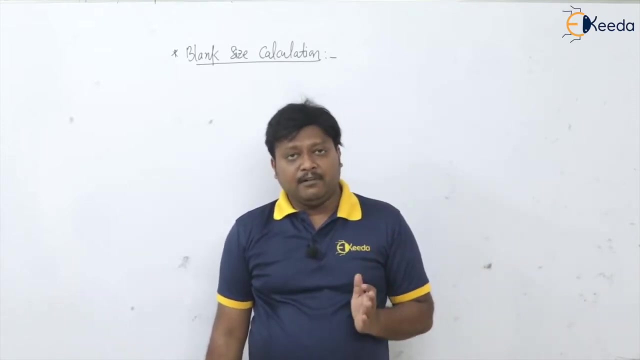 to require to produce the required height and diameter of the cup. so here the blank size calculation. blank size calculation is very, very important thing that can be done by mathematically, graphically, okay, by using the volume, by using the surface area, we can able to find out the blank size required to make the cup of diameter. 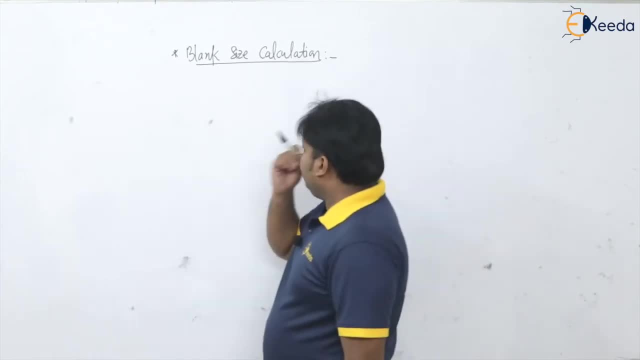 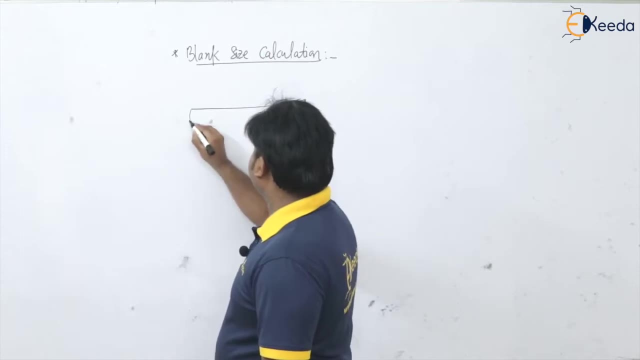 say small d and height h. so if i say that the blank which have i, which i have taken for the operation, is of thickness t and i have taken for the operation of thickness t and i have taken for the operation of thickness d and the diameter of say d, okay, so d is the blank diameter and t, t is. 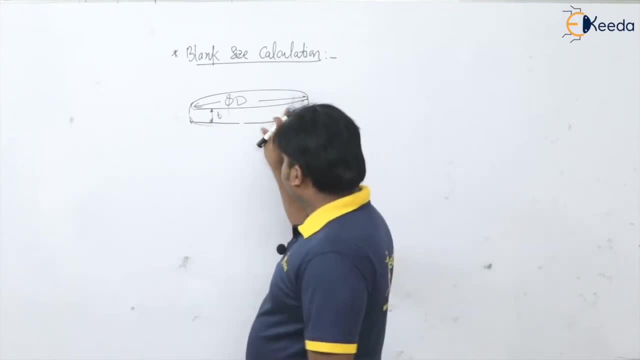 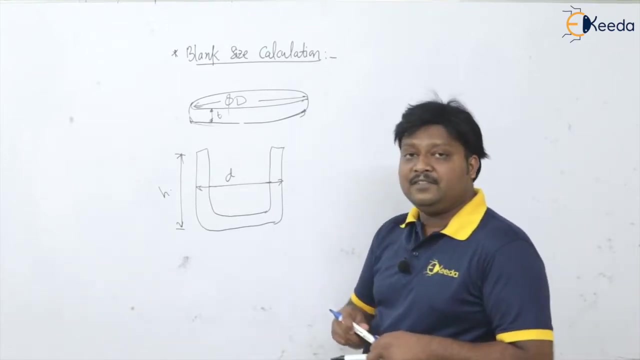 what the thickness of this blank. so from this blank what we are going to produce? we are going to produce this cup of, say, diameter d and height h. so if i say that the diameter of this cup is of thickness h, okay, now for that what we can do that. so we can do one thing. if you consider the surface, 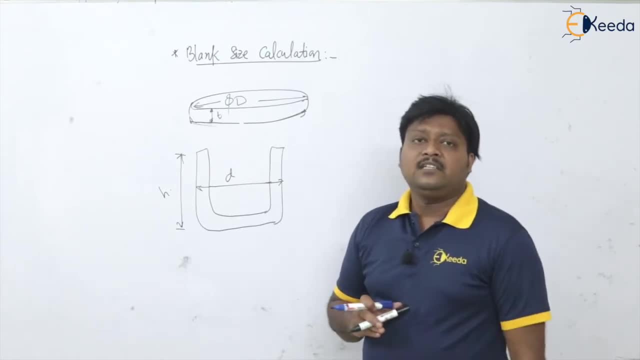 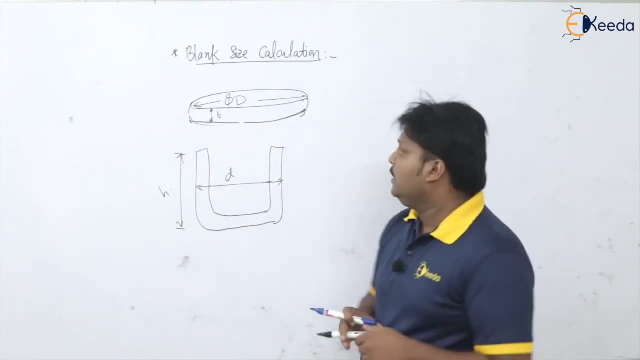 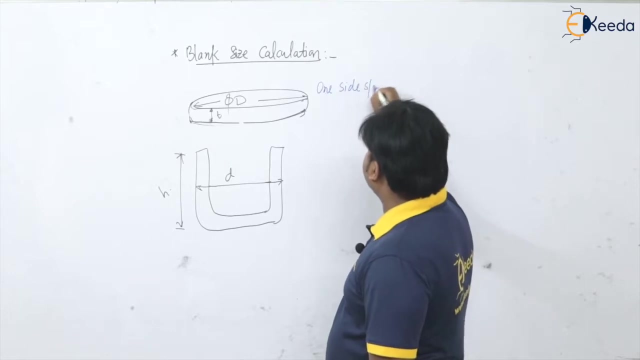 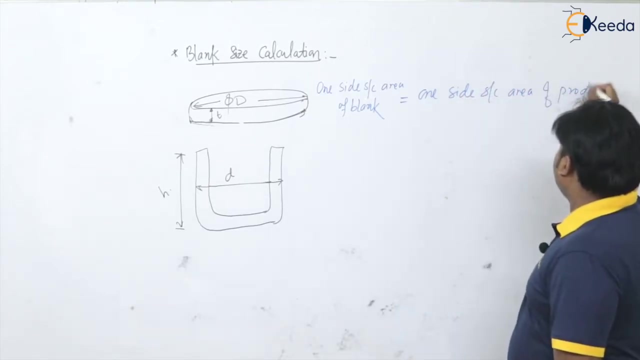 area there are. there are various techniques to get this blank size by volume, by graphical method- okay, so minute methods. but here we are, using this surface area method so that i can have the one side surface area. blank is equal to one side surface area of product and our product is what we are going to get. cup of. 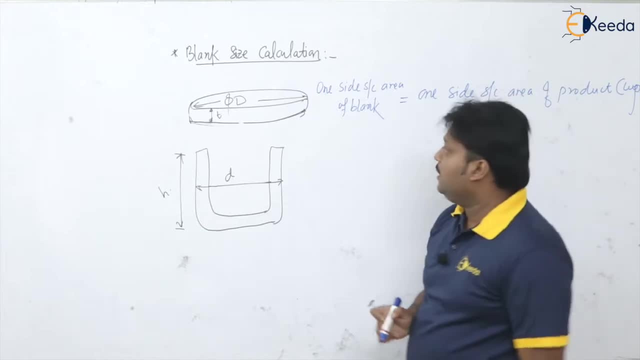 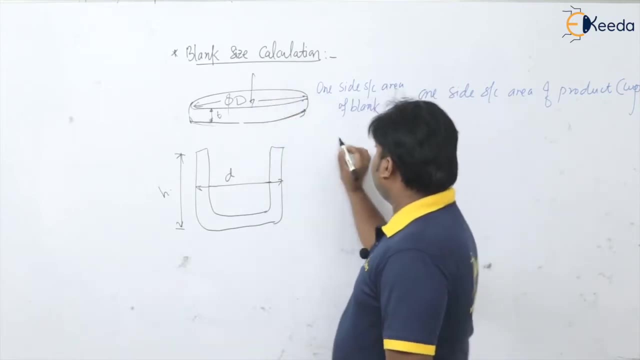 course, the surface area of the cup one side. so if you look at from the one side, of course it is nothing but the cross section of the blank. it will look like a circle only isn't it so? pi by four, capital d square. so d is our diameter of the blank and- this is very important thing, that the 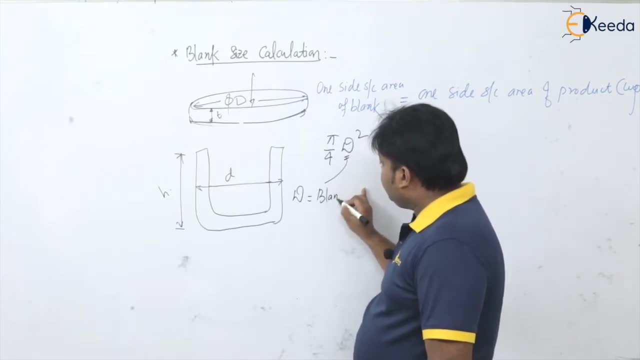 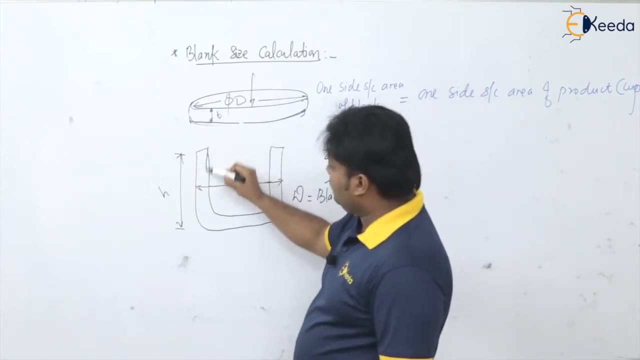 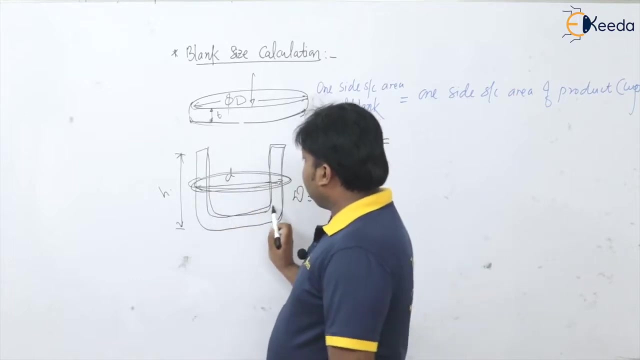 thing we are going to find out: the blank diameter. blank diameter, okay. so pi by four d square is equal to one side surface area of the cup. see one side surface area of the cup. what you are getting here? you are getting this surface of the, say, cylinder, and here, at the base, you are getting 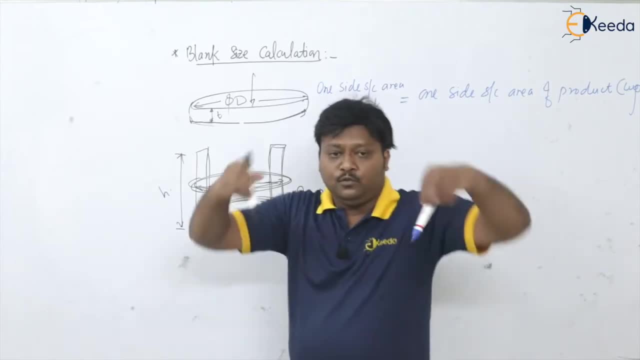 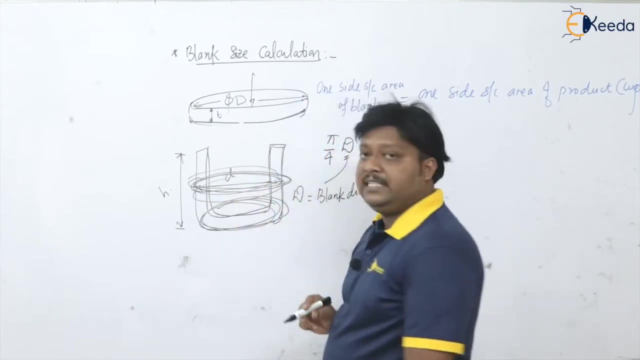 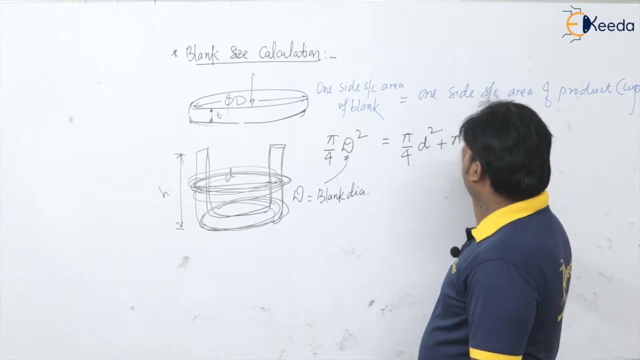 the circular cross section, isn't it so? if you, if you look from the top, what you will get here? this is at the base, this is the circle and this is the face. pi d h, isn't it so? if i write here pi by four, small d square plus pi d h is the one side surface area. 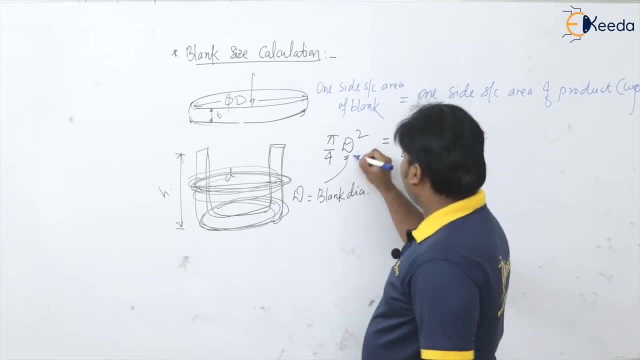 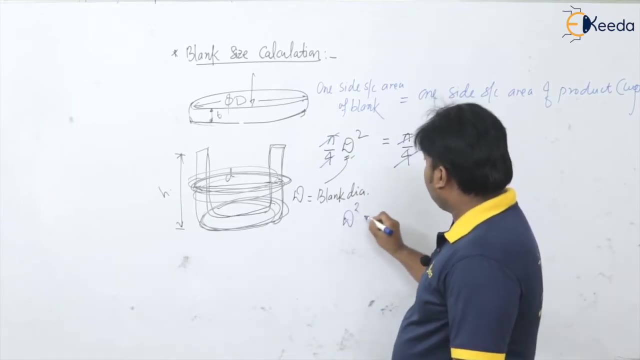 isn't it so? very nicely, we can get the value for d pi pi. get cancelled four, get cancels here. get multiplied this side, so d square what you will get here, this small d square plus four times small d into small h. so what is the d? it is nothing but. 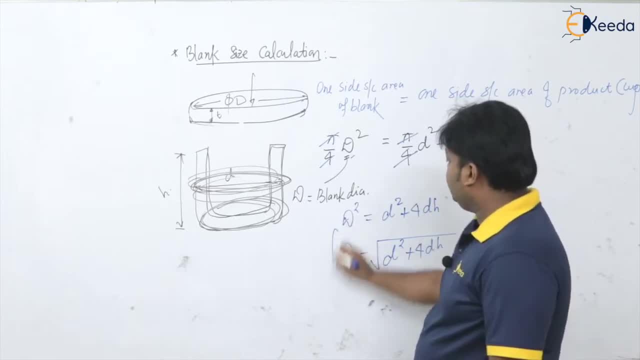 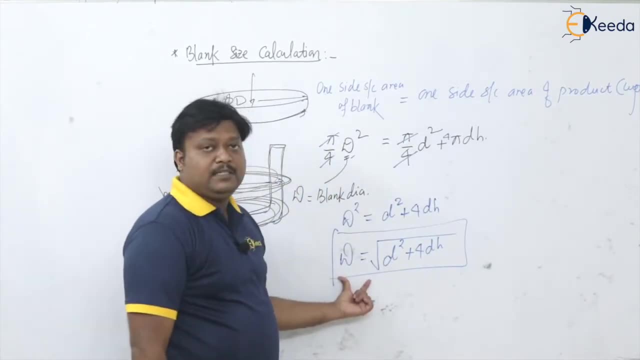 root of d square plus 4 times dh, isn't it? so this is the formula for the blank diameter, isn't it? this is the blank size. this is the black side that we are interested, very, very important. many times, question us many times. so please remember the formula for blank size: diameter is equal to. 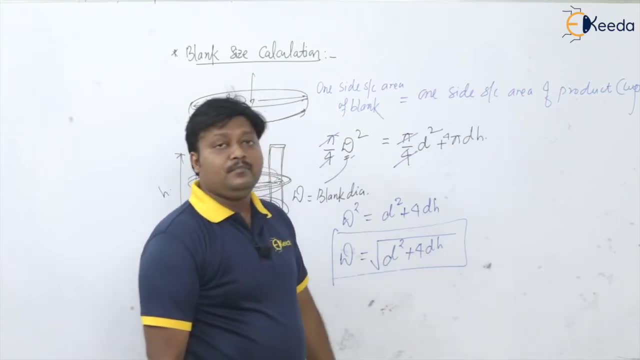 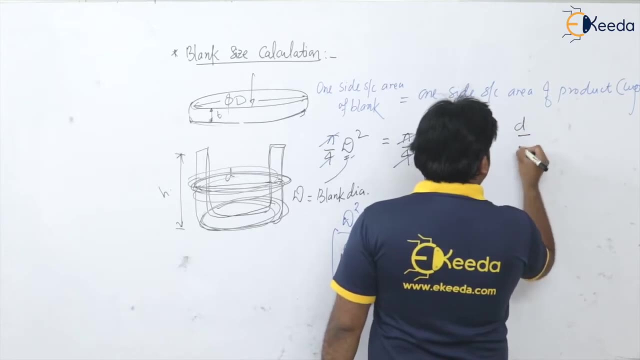 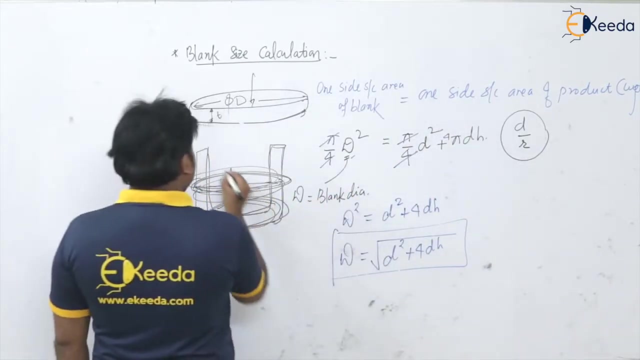 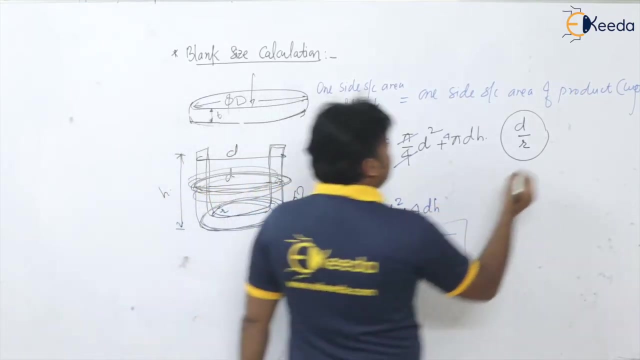 root of d square plus 4 dh. now see here when we have to see the d, d by r ratio. okay. so here we have to see first of all d by r ratio, so d by ratio, what this is our diameter d and this is the corner radius, r. okay, when this d by r is greater than 20. so this is the formula, okay. 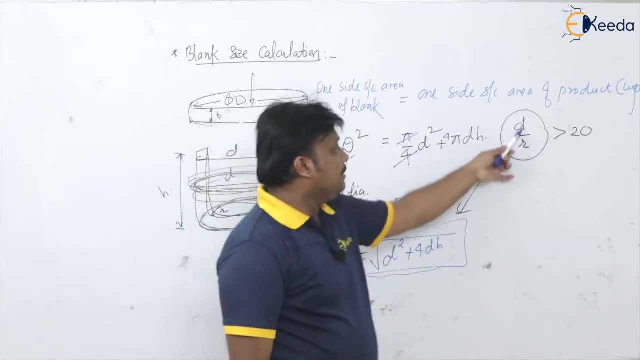 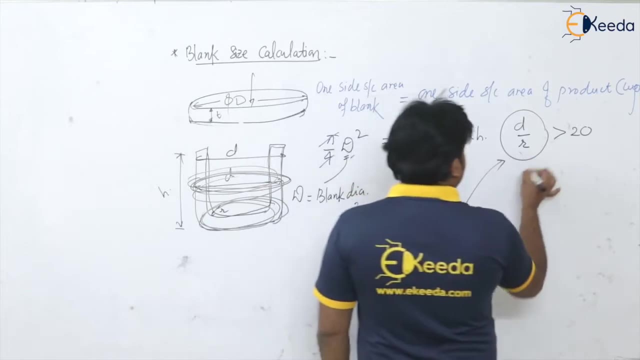 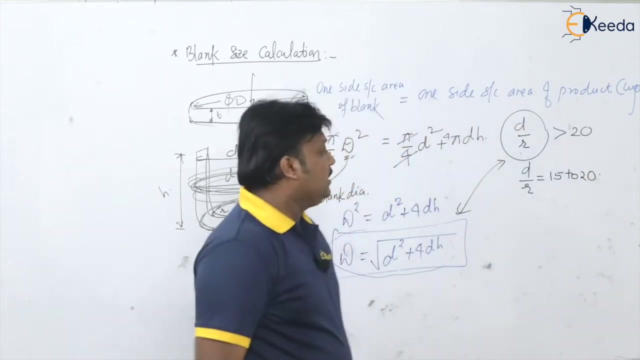 when? when to use this formula? when the d by r ratio for the given cup is greater than 20.. now, when this d by r is ranging from 15 to 20- 15 to 20- then what we have to do, we have to minus. 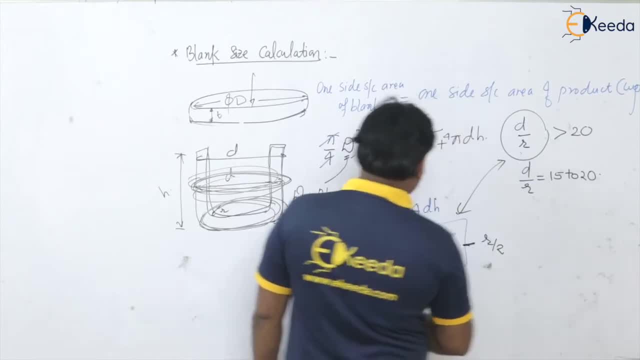 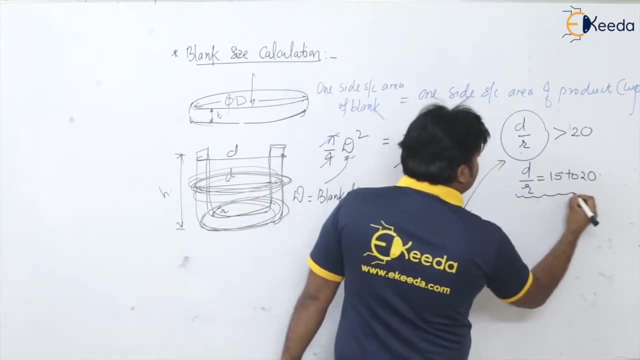 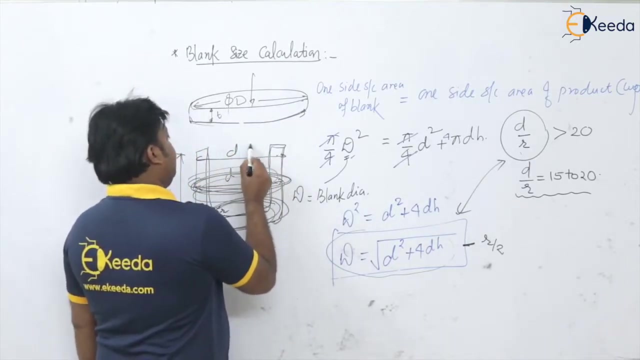 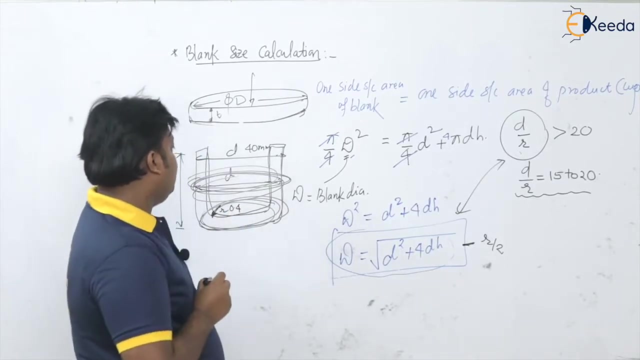 the half of the radius, corner radius from the obtained blank size. this is your, the correct answer, when the d by r ratio ranging from 15 to 20.. so let's say the diameter is 40 millimeter and this r is, say, 0.4 millimeter. so of course, here you will check first d by r ratio. 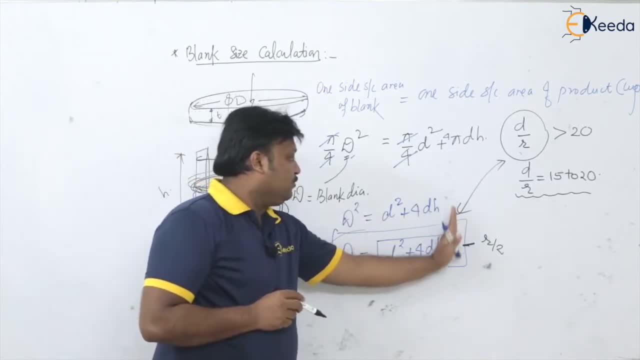 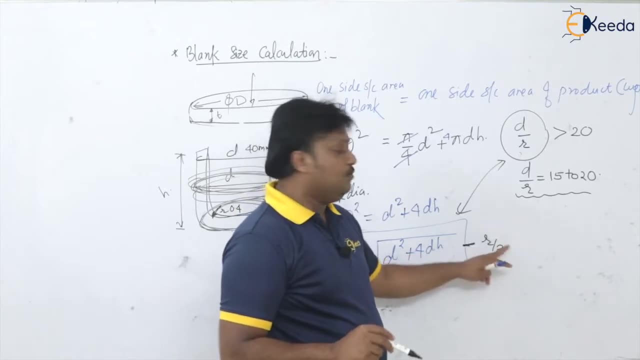 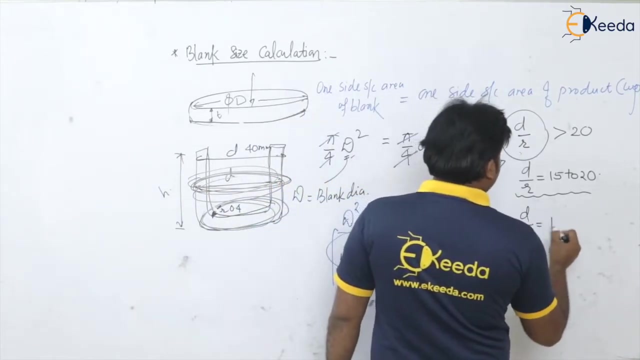 if it is more than 20, you will simply use this much formula: if d by r ratio ranging from 15 to 20, you will minus the half of the corner radius from this. you will get the correct value. now, when this d by r is from 10 to 15, then what we will do? we will minus the corner radius from this. 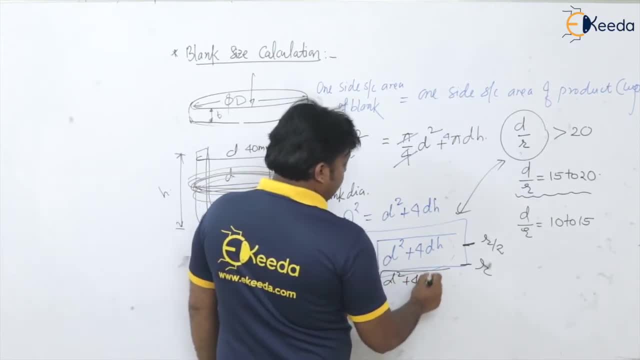 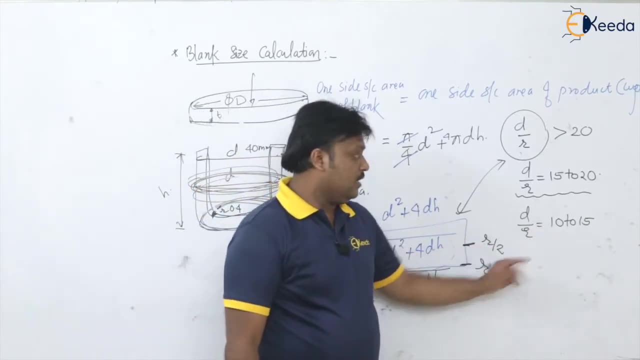 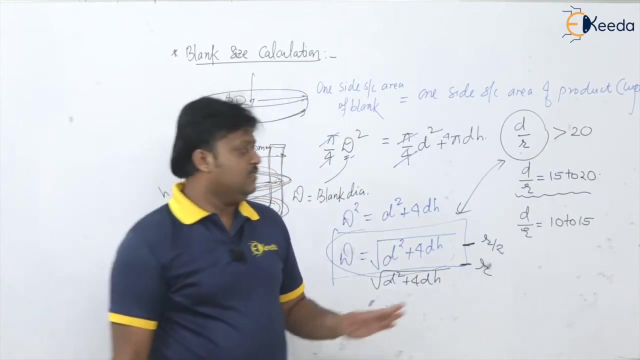 d square plus 4 dh. please remember what you will do directly. we will minus the corner radius. you will get the correct answer. now, what will happen if the d by r ratio is less than 10? so in that case you can simply go for total surface area of the product and total. 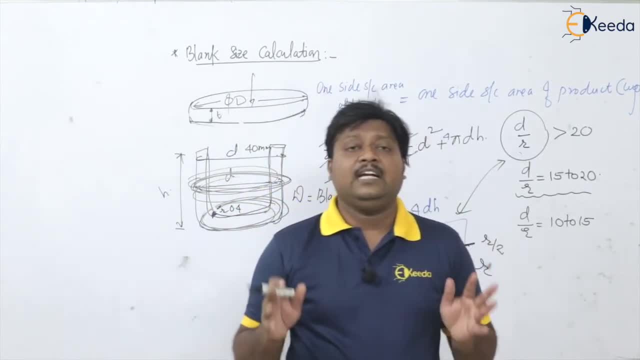 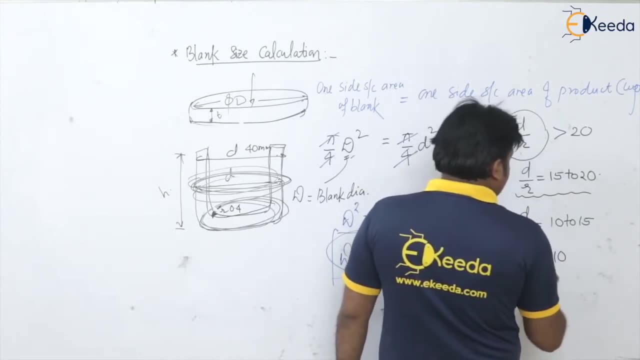 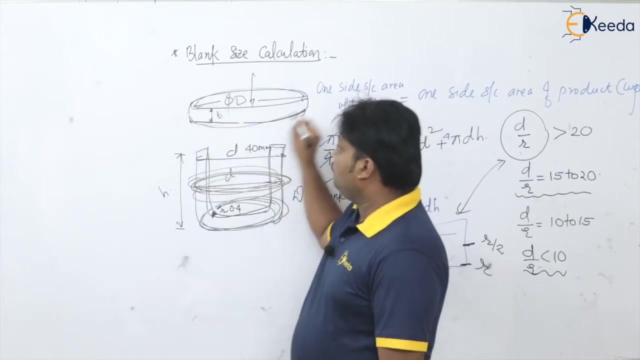 surface of area of the blank. you equate that and go for calculation of the size. so if d by r less than 10, what you will do? you will go for total surface area here. we have taken only one side surface here, isn't it? then you will get. the total surface area of the blank is equal to the. 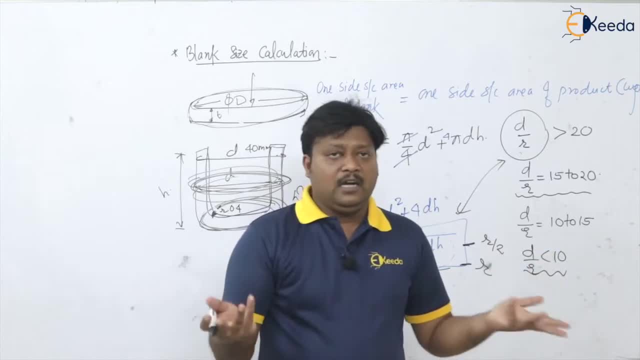 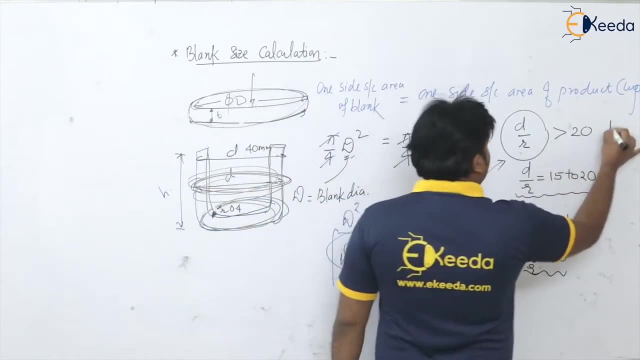 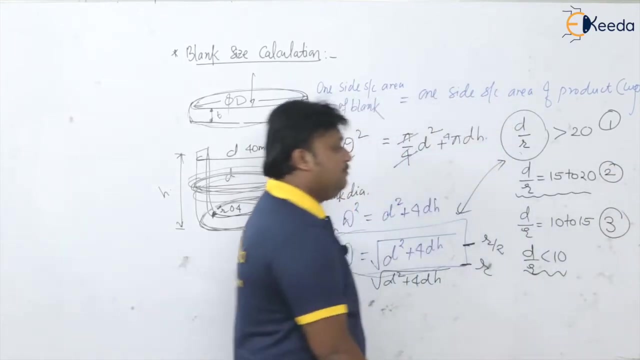 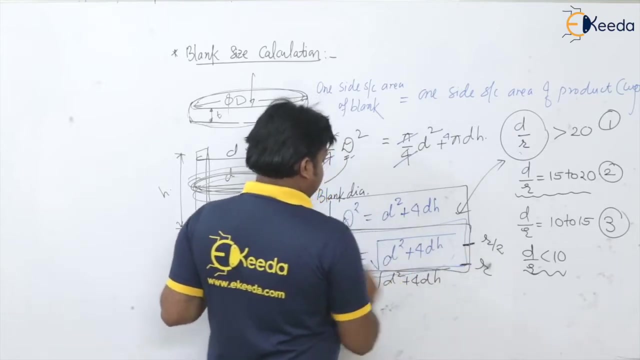 total surface area of the product or the cup, you will able to find out the value for d. please remember these three conditions: d by r greater than 20, d by r in the range of 15 to 20 and d by r in the range of 10 to 15. okay, so this formula is very, very important. this formula blank sides. 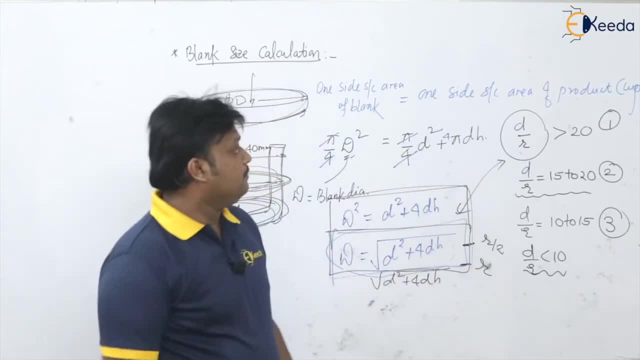 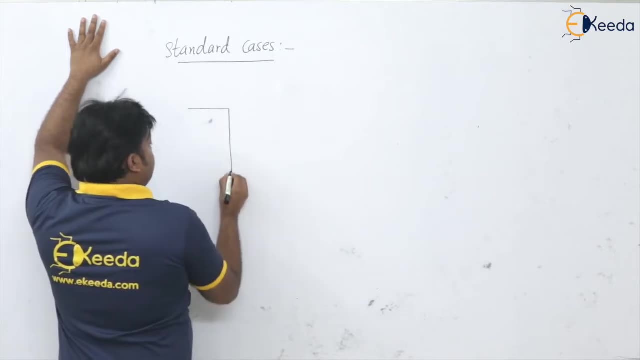 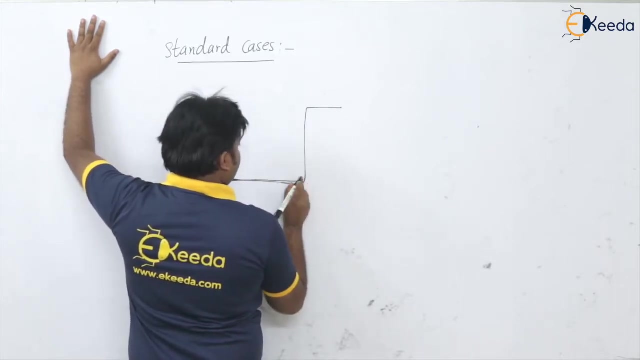 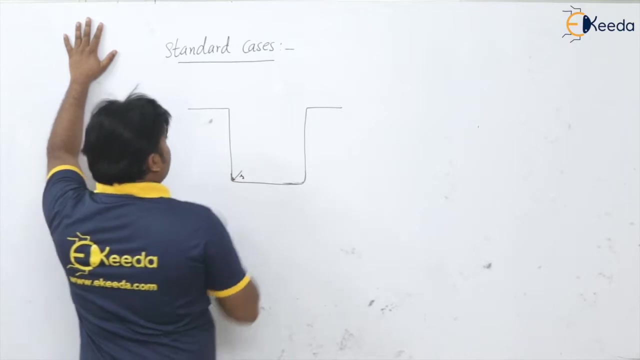 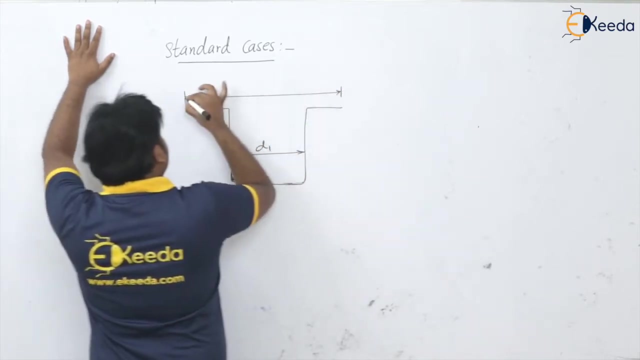 okay, blank sides. okay, let us take some standard cases for that. let us say: my cup is having the flange, my cup is having the flange. okay, of course, a corner radius is given here. this is t1 and this is say d2, and this is the cup height. 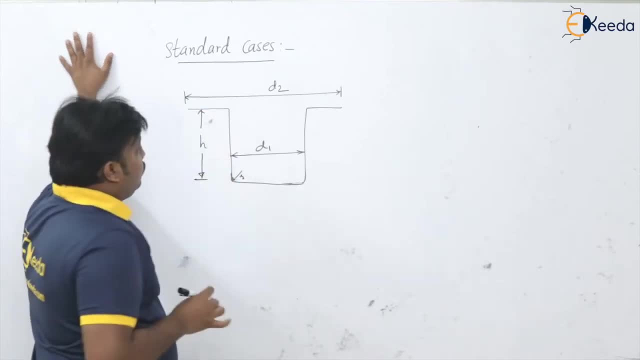 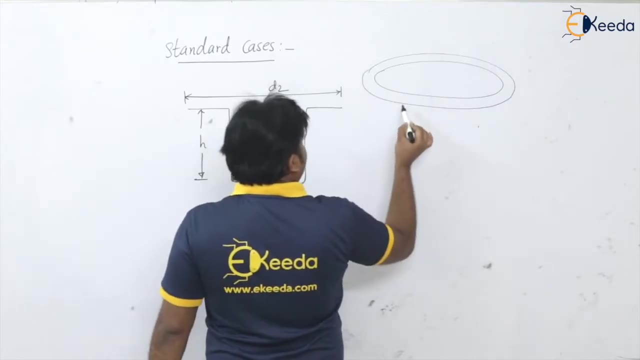 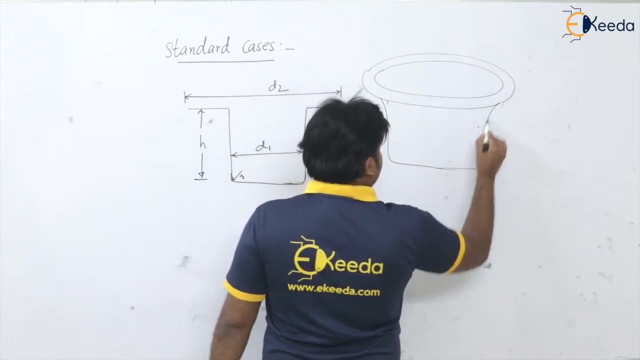 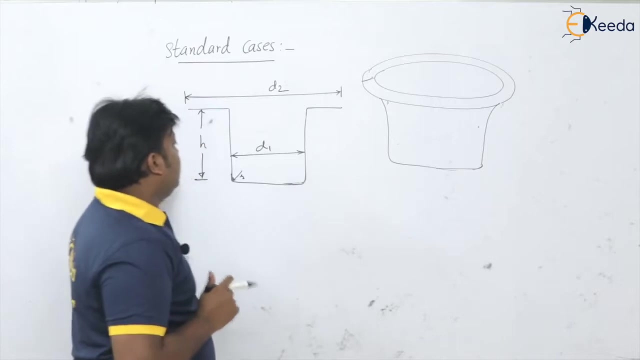 okay, so there is a flange for the cup, right like this. so this is the flange. now, okay, so this is the flange you are having to the cup. so for this cup, calculate the blank size. so we know that one side surface area of the blank is equal to one. 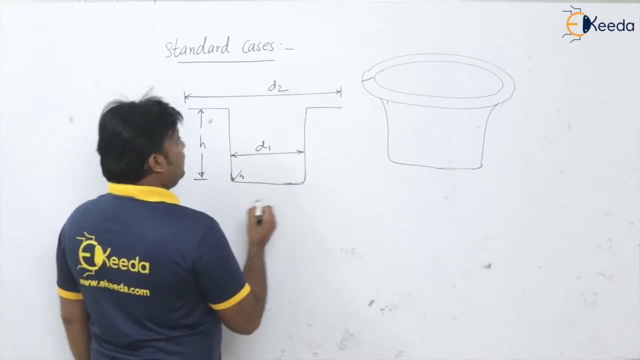 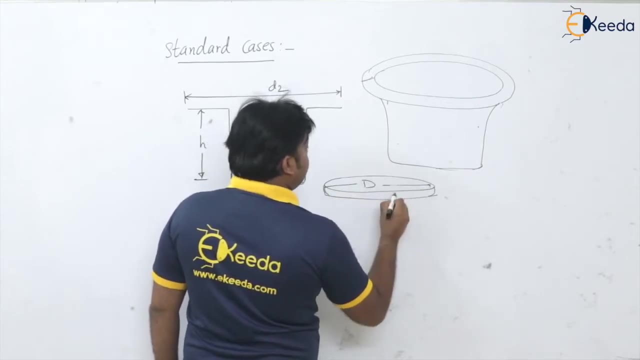 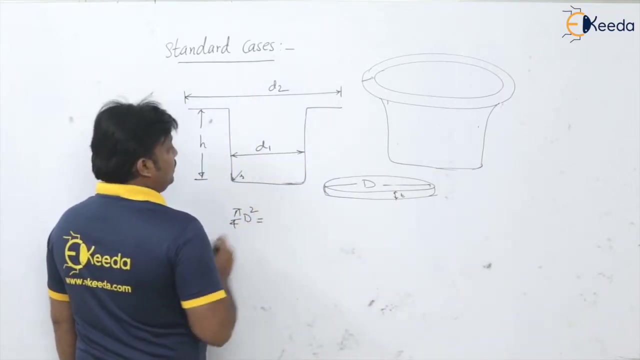 side surface area of the cup. so one side surface area of blank blank, always the available like this. okay, with this diameter d and thickness t, now tell me one side surface area of the blank. pi by 4 d square is equal to one side surface area of the cup, that is, pi d 1 h. 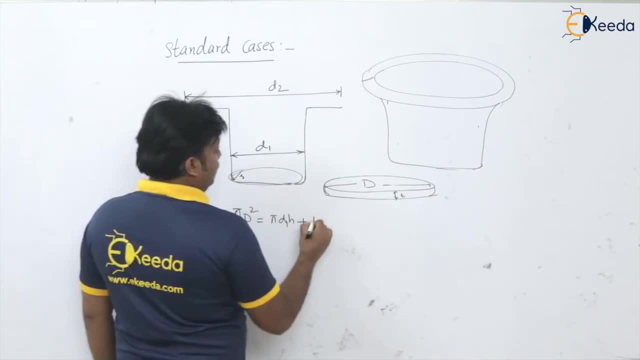 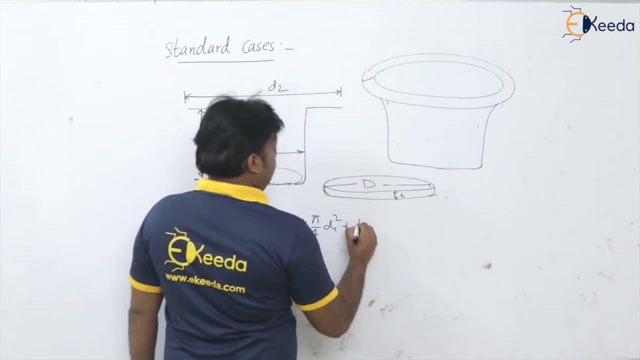 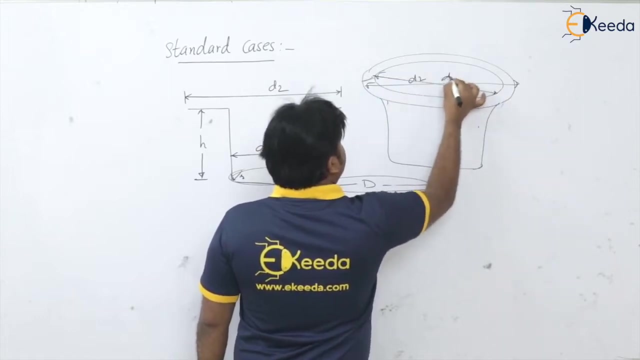 plus. what will happen at a lower level? this is circular: pi by 4, d, one square plus. how will it appear from above? it will look like this: that is pi by 4, this is d 2 and this is d 1. so pi by 4: d2 square minus d 1 square. so simplify this. 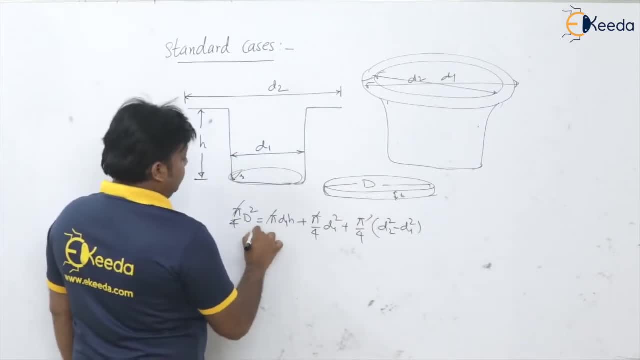 pi pi pi gate cancels four will come here. that is d square is equal to four d one, h, f and same here. let's see. so d two square is equal to 4d1, h 2 square plus i, 4y2r, v will look like this clamping point. and if we simply this pi pi pi gate cancels, four will become here, that is d2 square is equal to four 8d2ドlares. and we can tell: in the future we will cooperate between the four d1 square. so simplifying this pi pi pi 4d2 skincare, let us pass, let's create our square and we are going to order that badd4. so let's start with alphabet. that is quarter1. recognize value. 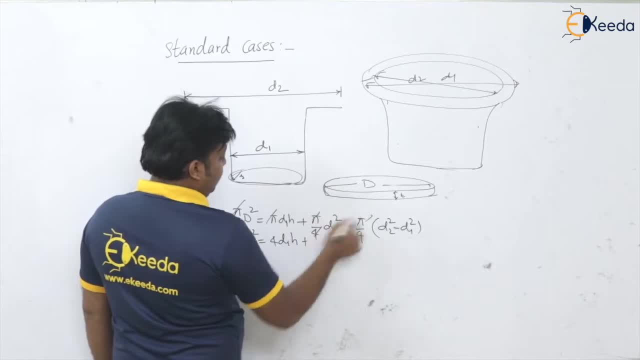 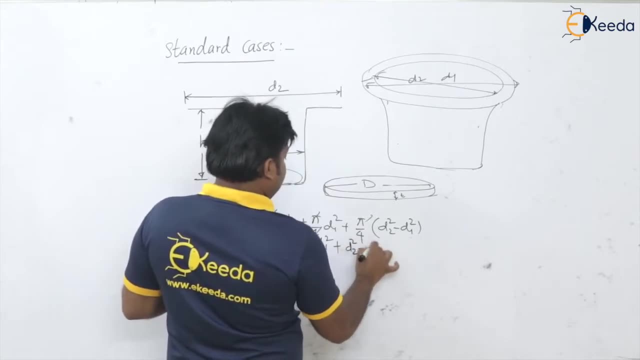 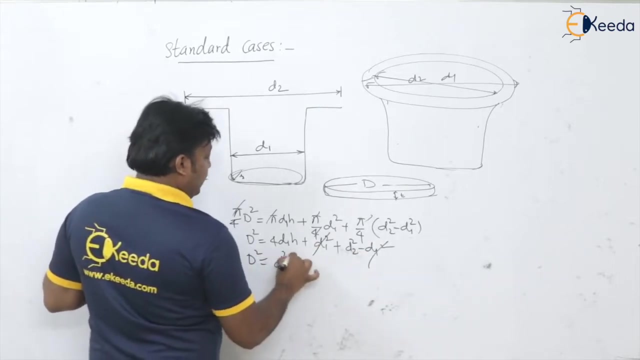 d square is equal to 4. d1 h 4- forget cancel d1 square plus 4. forget cancel here. so d2 square minus d1 square. so d square is equal to d1 square. d1 square- get cancels here. so d2 square plus 4. 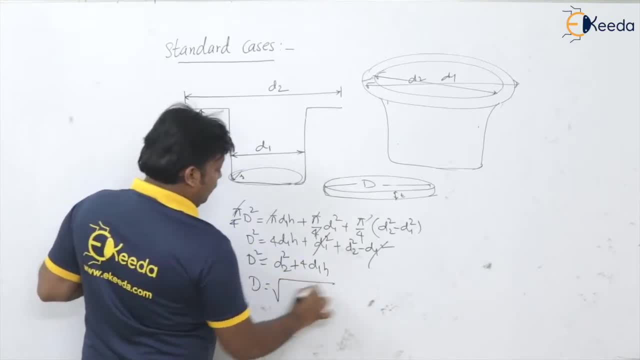 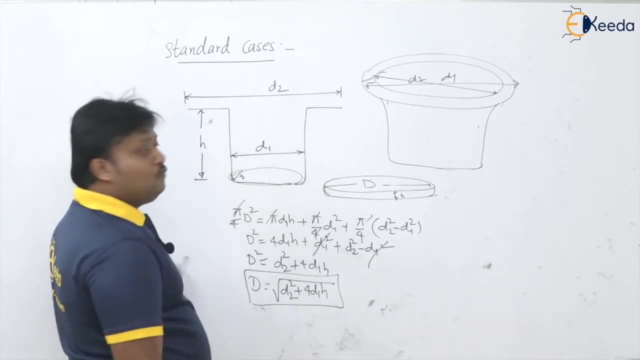 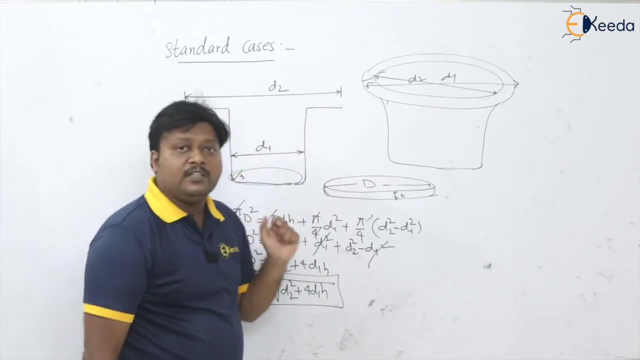 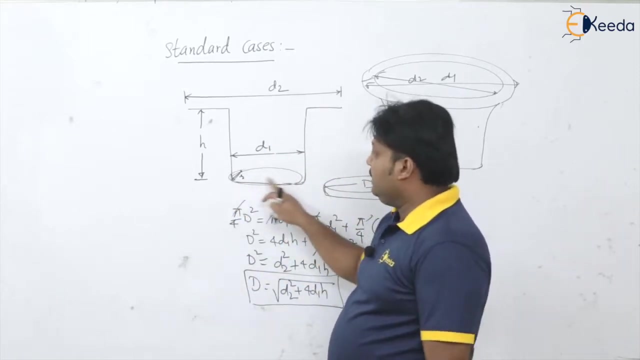 d1 h. so d will be equal to under root of d2 square plus 4 d1 h. so you get the value for the blank sides when the flange is provided or the flange is on the cup. okay, so of course you can. you can use the same thing. this is the d1 by r. you check the d1 by r less than sorry, greater. 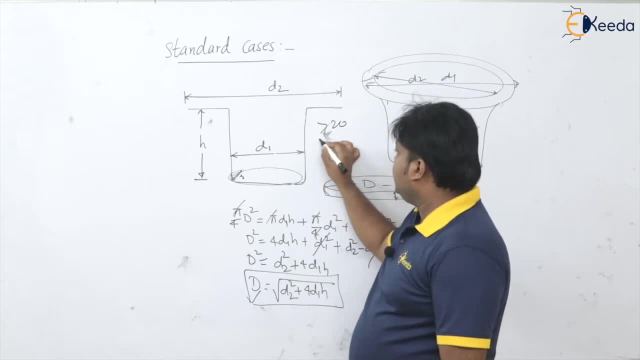 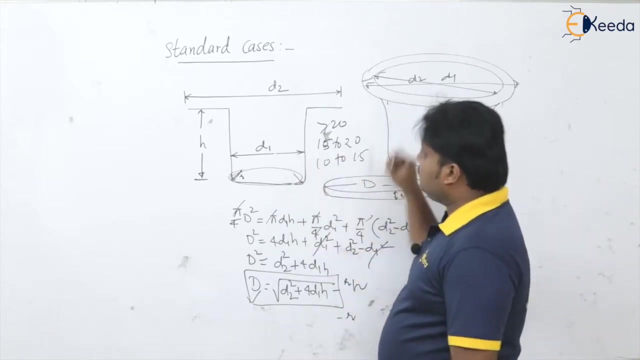 than 20, then use the formula as it is. it is in the range of 10 to 15 to 20, minus r by 2. if it is 10 to 15, then minus r. you can have like that, okay? so this is for this standard case number one, that is, cup with flange. 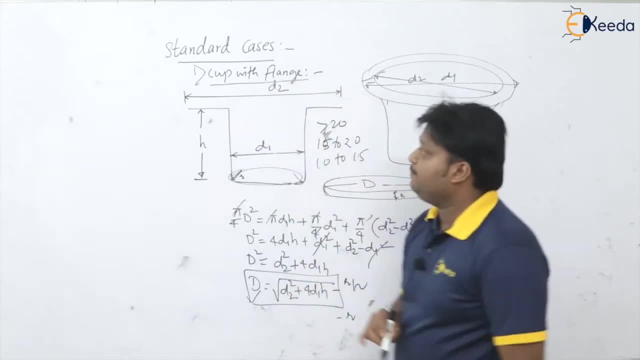 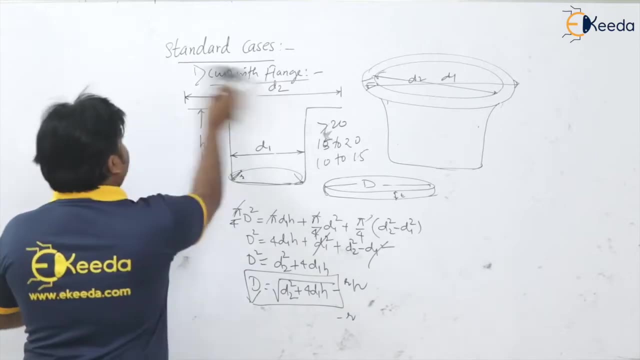 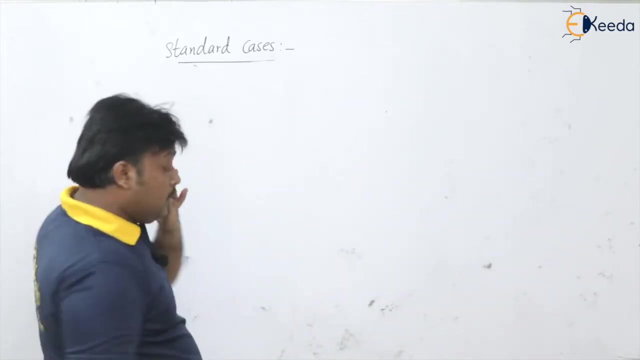 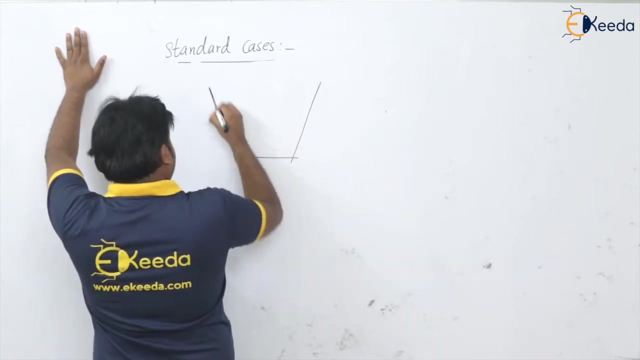 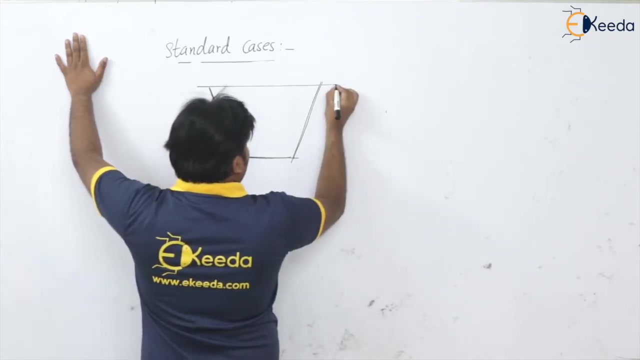 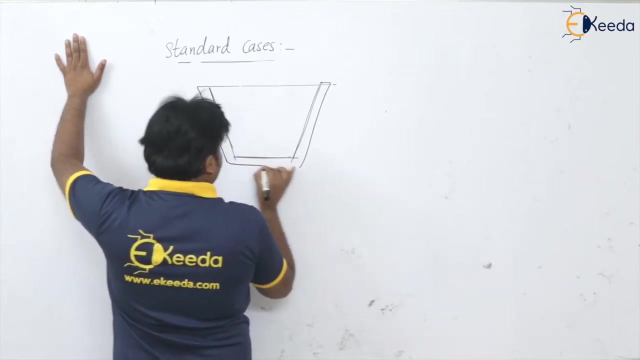 okay, so this was the flange. now let us take the second case, say: this is the cup like this shape. okay, so, whether there is a slant height or there is simply height is given, okay. okay. so, whether there is a slant height or there is simply height is given. 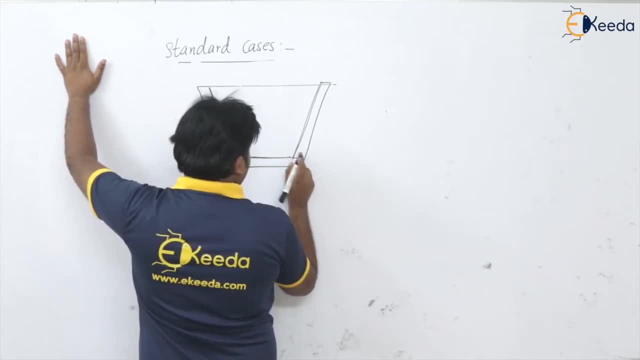 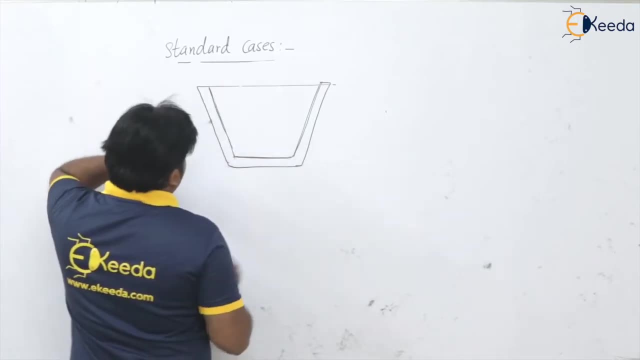 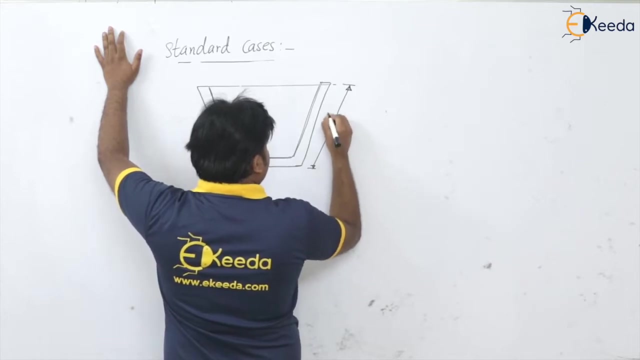 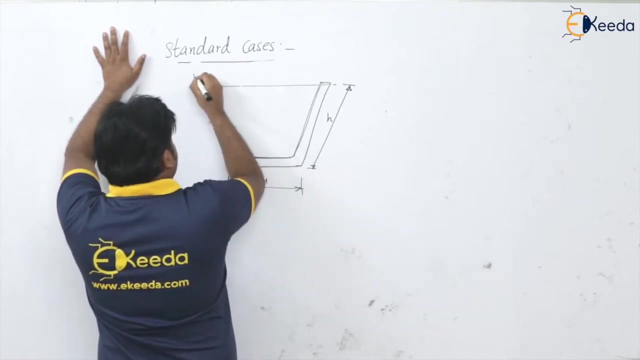 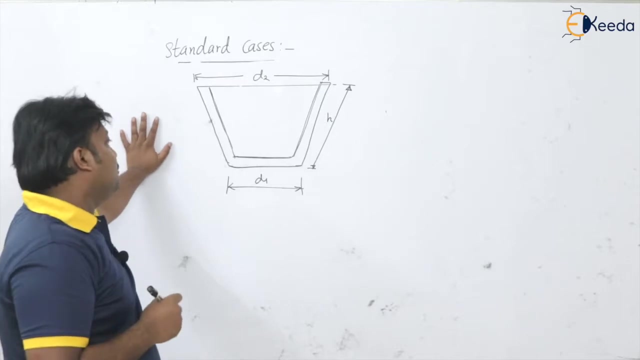 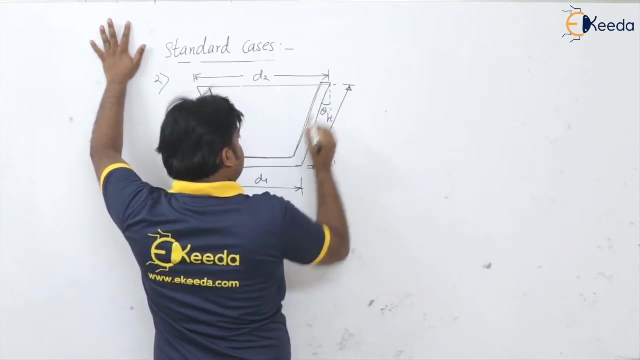 say: this is H, okay, this is d1 and this is d2 v-shape cup- okay, v-shape cup is going to analyze here for the blank size calculation. okay, so sometimes see this: either H or sometime this angle is given to you, this angle, theta or this angle, theta, okay. 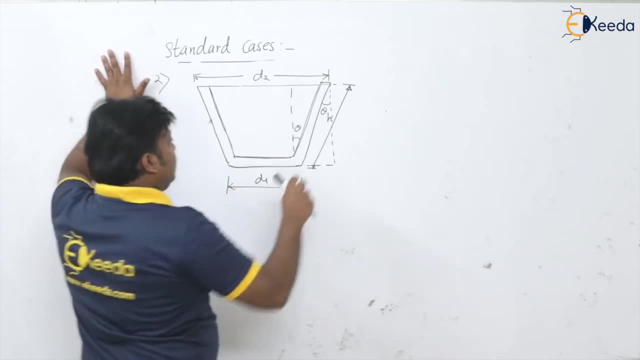 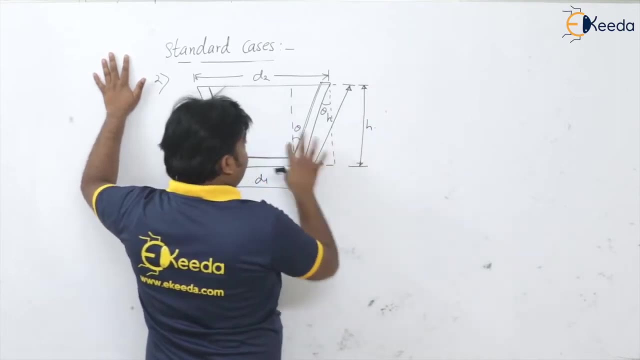 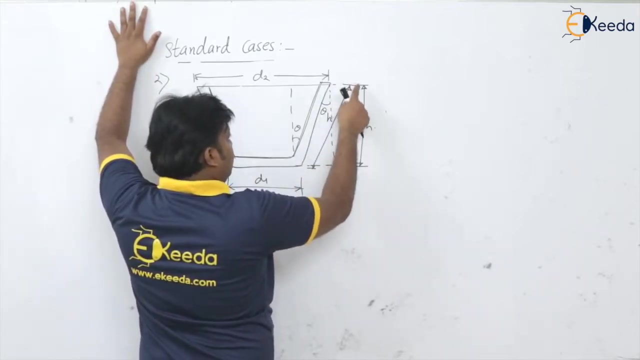 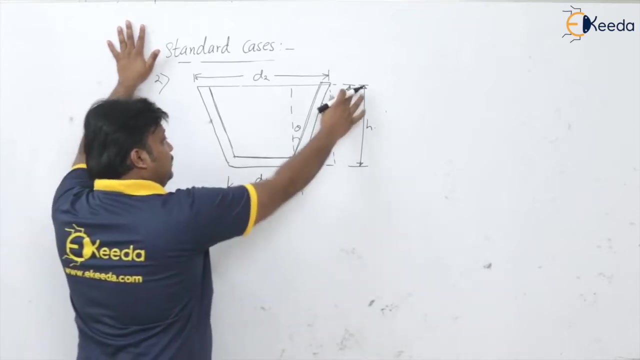 so you can get the value for the H here, okay. so it is not like that that there should be the necessity of the H this or this H. so whatever the height is given to you, okay, you can take the height there. okay, no, any issues. if slant height is given, take it as slant as if the angle is given. 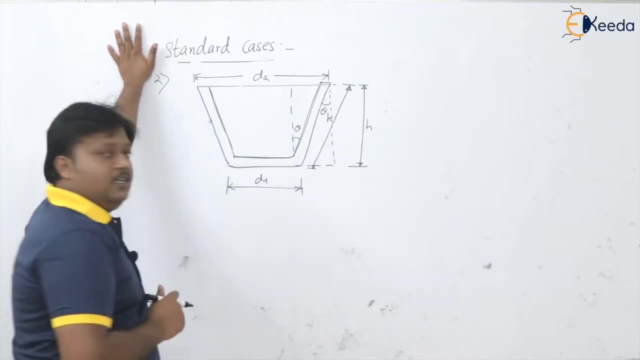 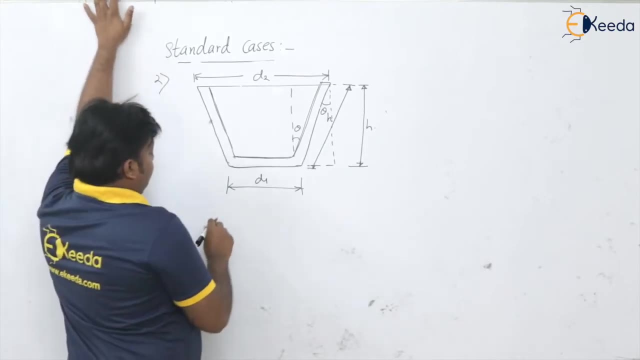 calculate the height. okay, you will have no any issue for that. actually you can take any. so here, what is the blank size? one side surface of the blank is pi by 4 dc. so the blank is pi by 4 d square. for this at the bottom it is circular, okay. 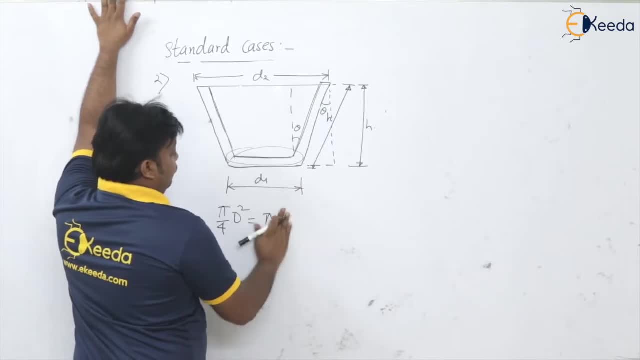 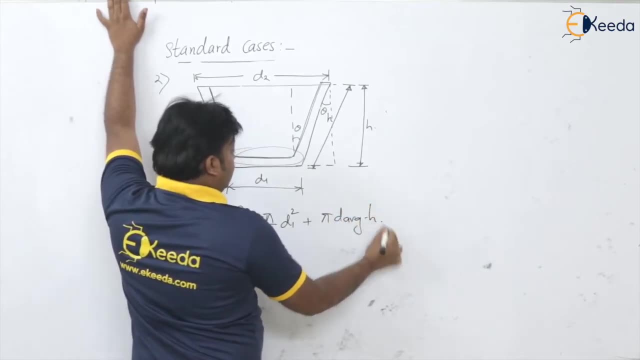 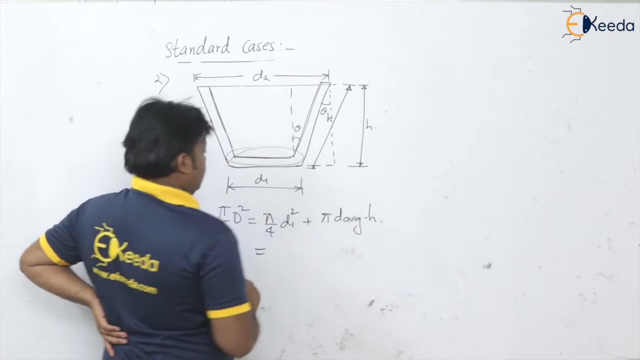 so pi pi by 4 d, 1 square plus here, pi D average into H, pi D average into H: pleasure, remember this. so here this pi by 4 d, 1 square plus pi time D average is what this is. it is 2 in H, So remember this. so now, if you have done this, 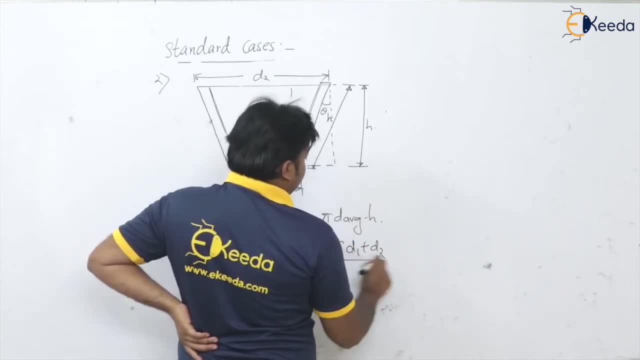 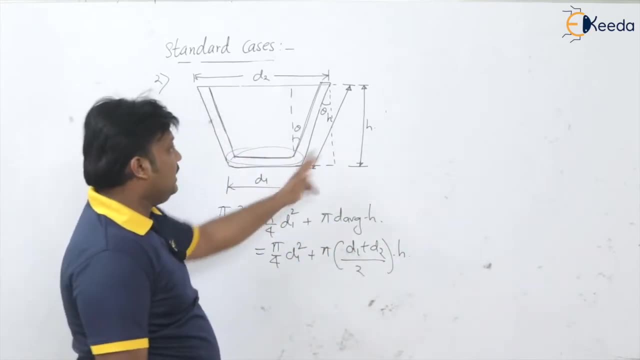 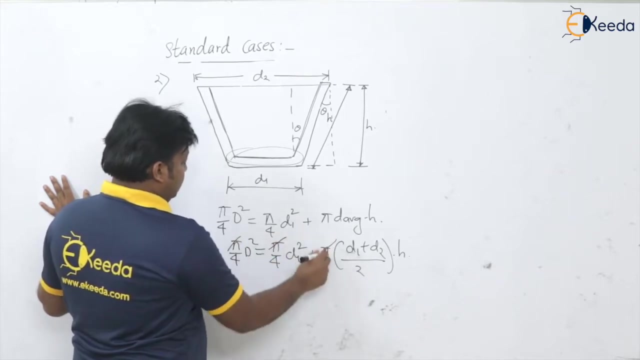 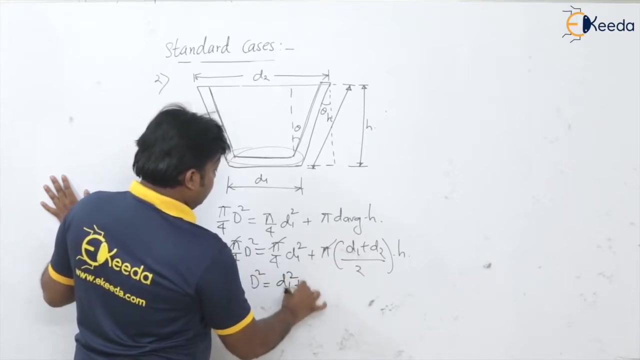 d average is what this? d1 plus d2, divided by 2 into h, into h? this is a slant height, or this height, any height you can directly take. okay, no initial. so this is pi by 4 d square. pi, pi get cancelled. 4 comes here, so it will be: d square is equal to d1 square plus 2 times 4 comes here, this 4 by 2. 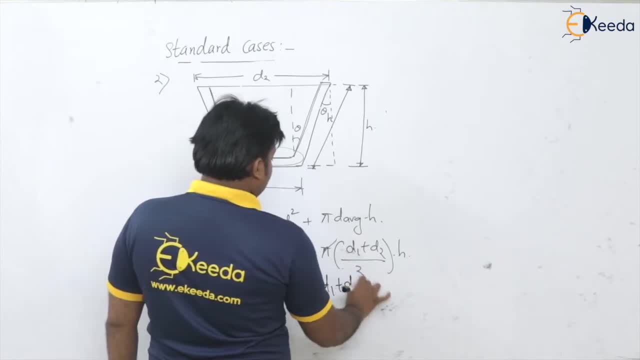 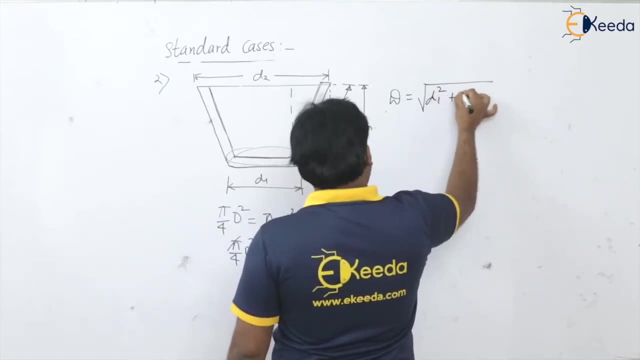 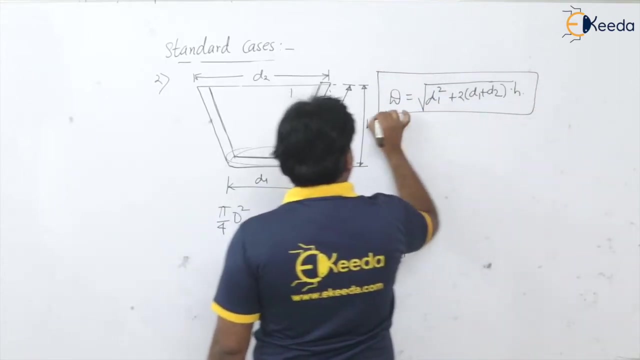 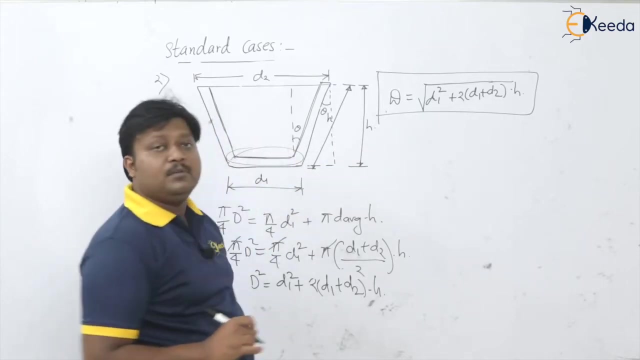 is 2 times d1 plus d2 into h. so what is d is equal to root of, say, d1 square plus 2 times d1 plus d2 into h. so this is the diameter of the blank for producing this v-shape cup. okay. 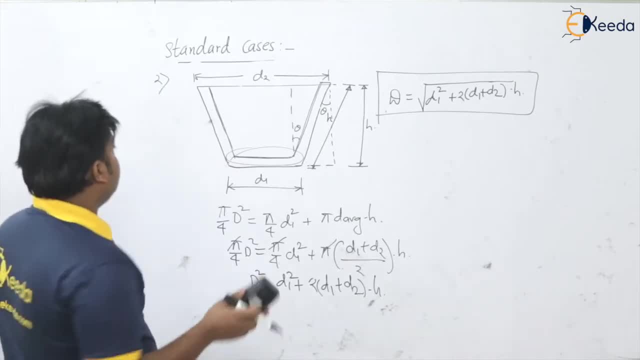 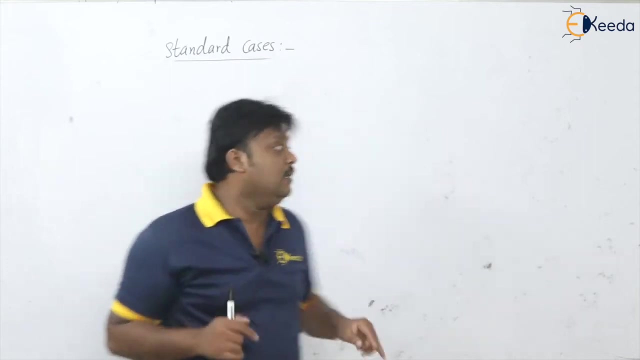 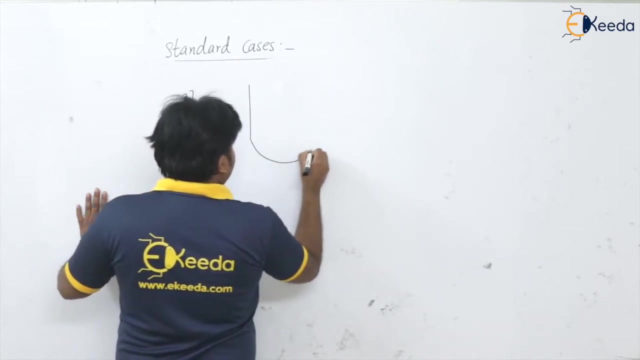 okay again, if corner radius given, then only you can go for the consideration that i already told you. okay, if not, no. initial now say: take the third case, after this v-shaped cup, that is, we are having the cup having the hemisphere at the bottom or the spherical shape at the bottom. okay, 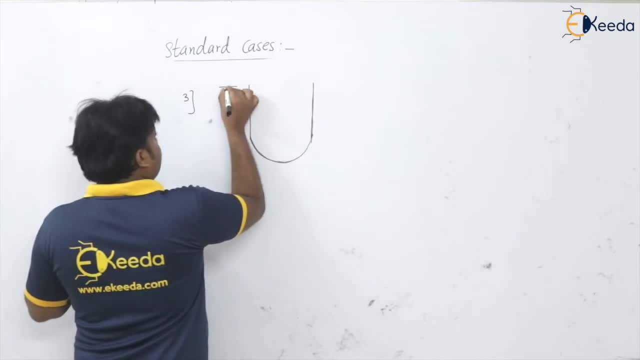 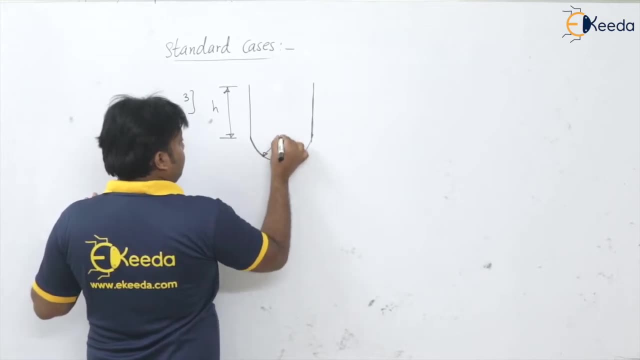 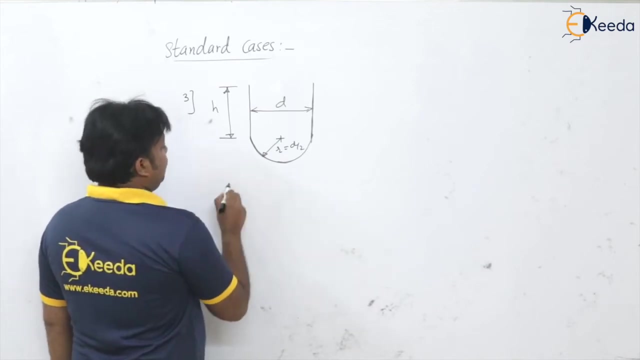 so say this is the height h. this is nothing but say r, which is equal to d by 2. okay for this shaped cup. if you want to find out the blank size, how will you find out? the one side surface area of the blank? pi by 4 d square is equal to 1. is pi d. this is 4 pi d 2.. 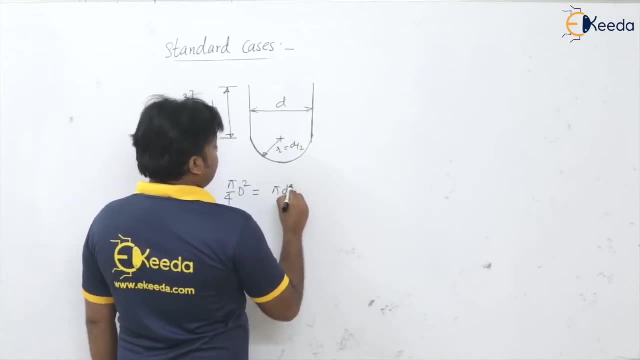 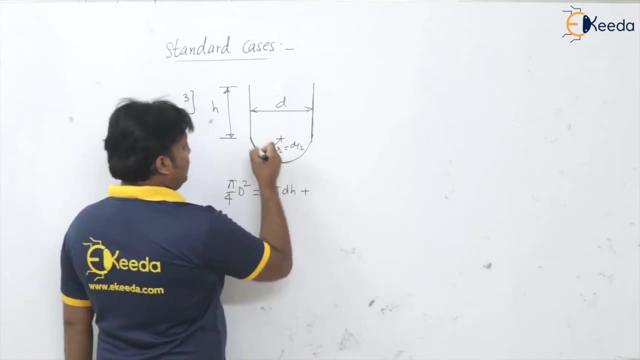 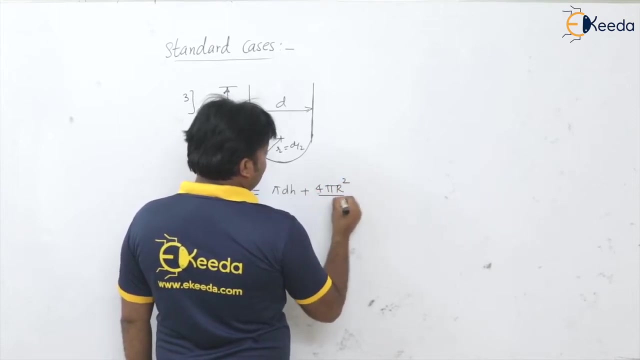 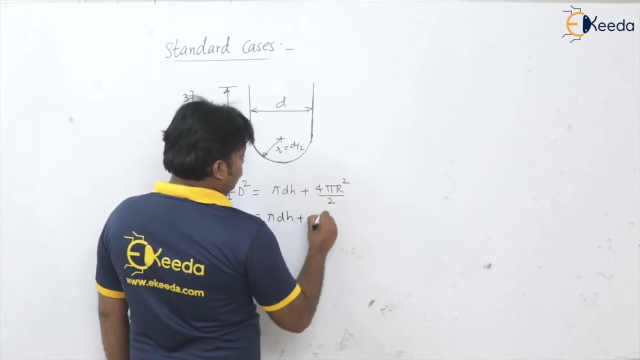 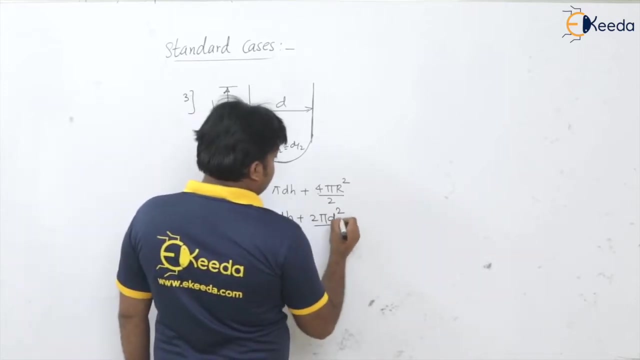 H, pi D H plus at the sphere that is half spherical. so what is half spherical surface area? and the two times or 4 pi R square divided by 2. okay, so this is nothing but pi D H plus 2 pi. this r can be written as d square by R is divided. 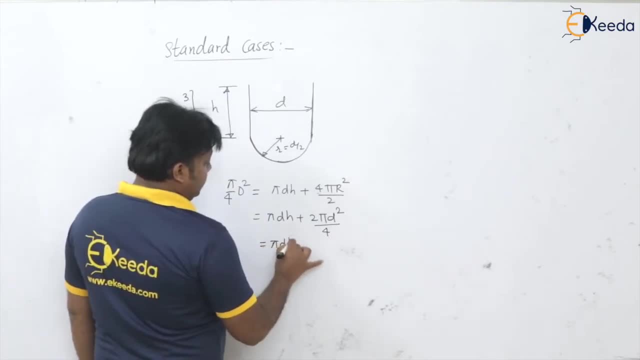 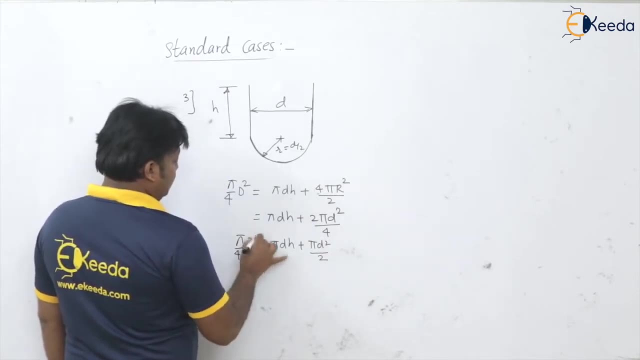 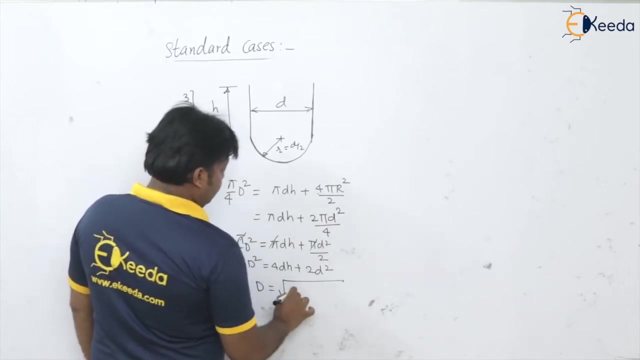 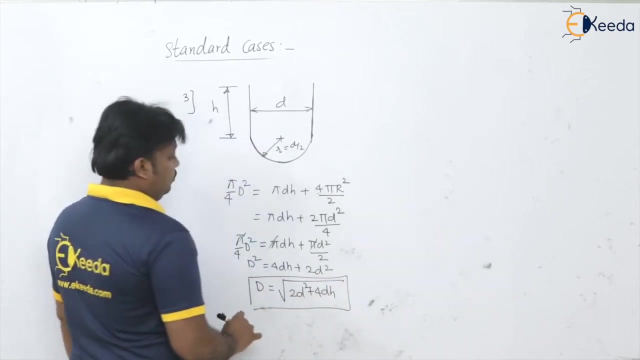 to that is 4, so you'll get pi D H plus pi D square by 2. that is equal to pi by 4 D square. so C pi pi pi get cancelled. so d square is equal to 4 d H plus dangles 2 d square. so d is equal to under root of 2 d square plus 4 dh. okay, for here no need of having 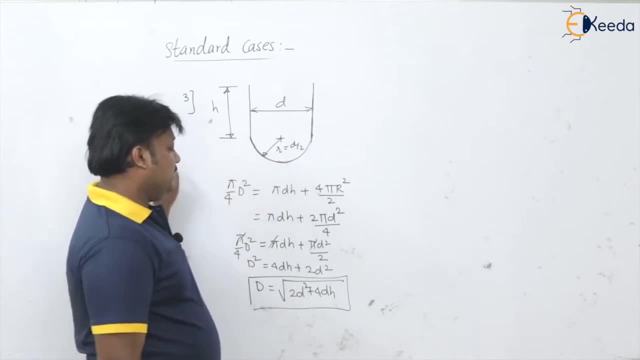 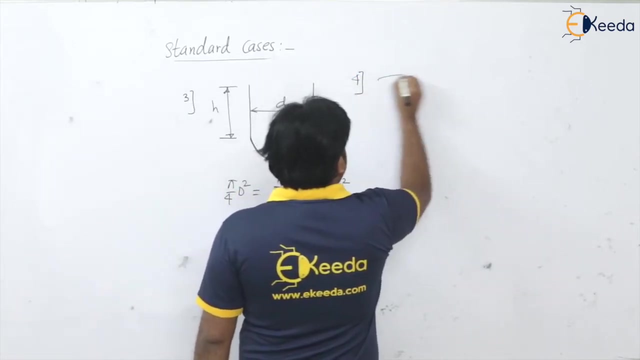 this d by r. so as this is a radius, there, spherical shape is there, so no need of any corner radius. so what is the blanks as you are getting in case of the spherical bottom of the cup, as d is equal to under root of 2 d square plus 4 d into h. okay, now if i take the fourth case as the hemispherical, 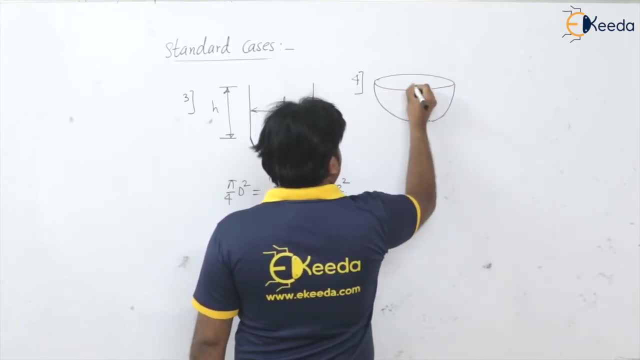 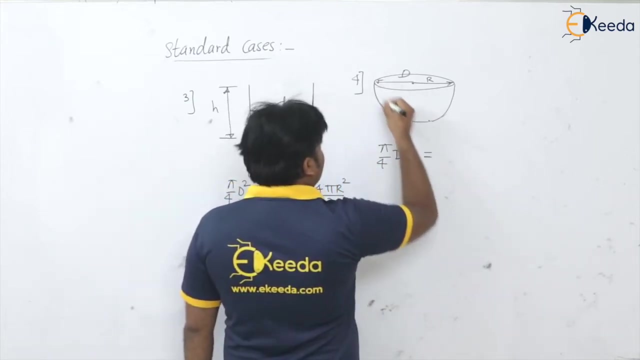 cup is there, okay, say of radius r, or you can have the diameter d, okay. so how can you calculate the blank size for the given cup? so please try one side surface area of the blank from where is going to produce pi by 4 d square? that is common. it is nothing but one side surface area. 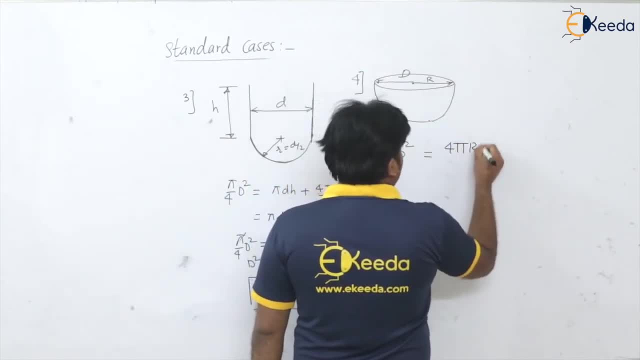 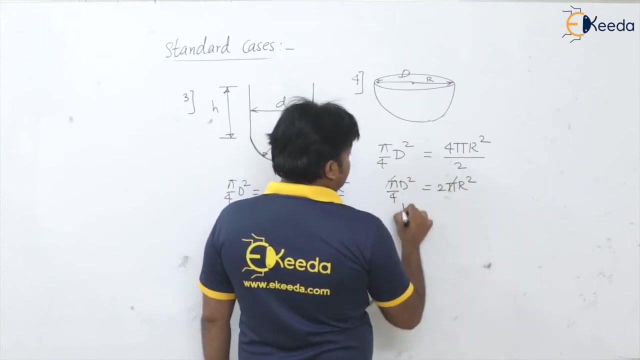 of the sphere is what that is. 4 pi r square divided by 2. that is, 2 pi r square divided by 2 pi r square isn't. it is equal to pi by 4 d square. pi pi get cancelled, so d square is equal to 8. 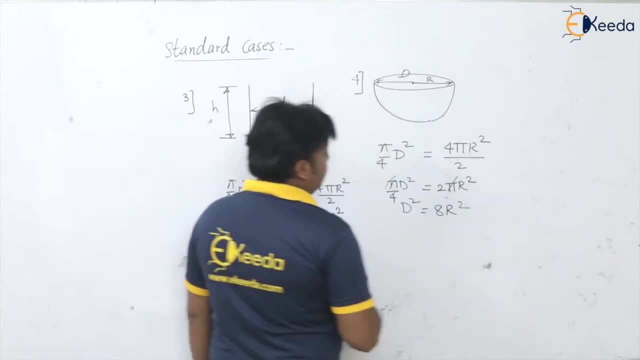 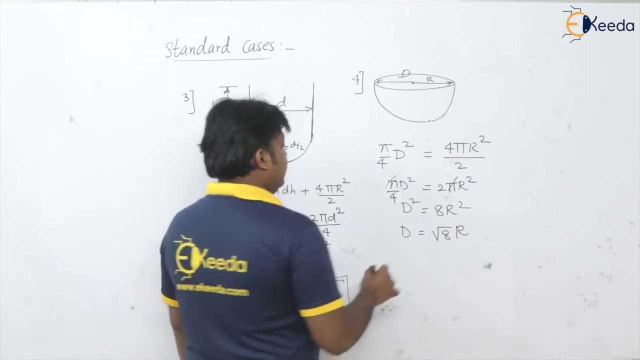 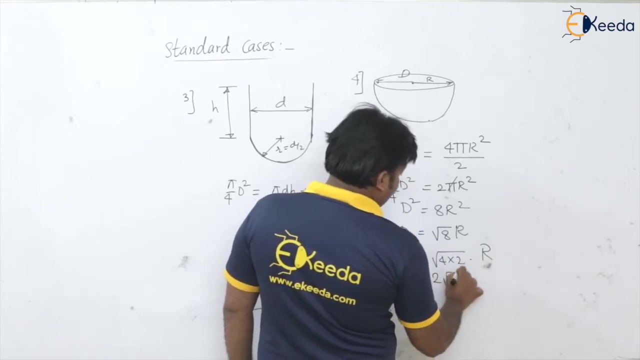 into 2s are 8 r square, isn't it? so d is equal to under root of 8 r. d is equal to under root of 8 r, so root root 8. how can you write this: 4 multiply by 2 into r, which is equal to 2 root 2 times r. 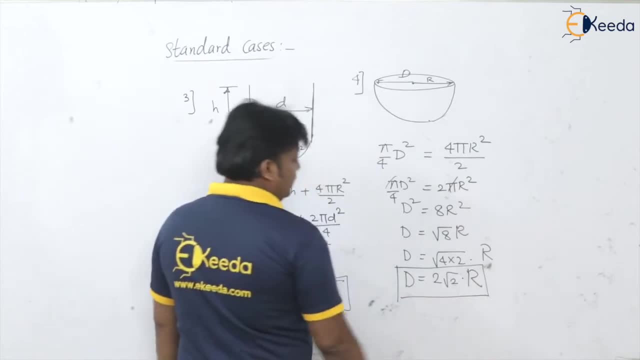 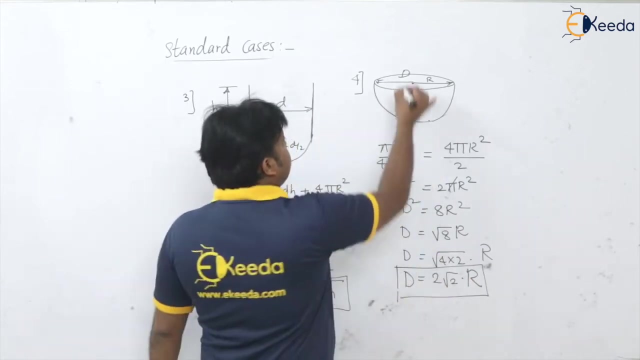 that is the size of the blank, for this size of the black for producing this hemispherical cup. is it equal to 2 root r, or in terms of diameter, 2 r is equal to nothing. but what the d say, d d is what the diameter of this hemisphere. so it is nothing but. 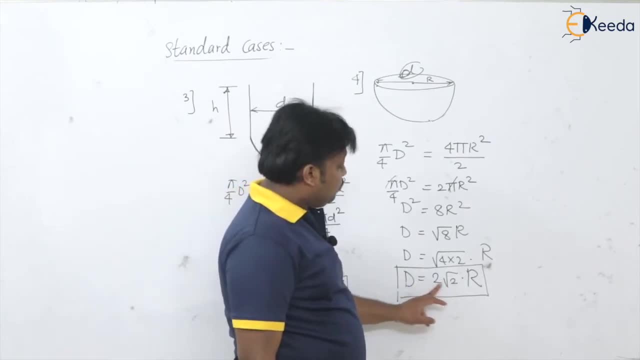 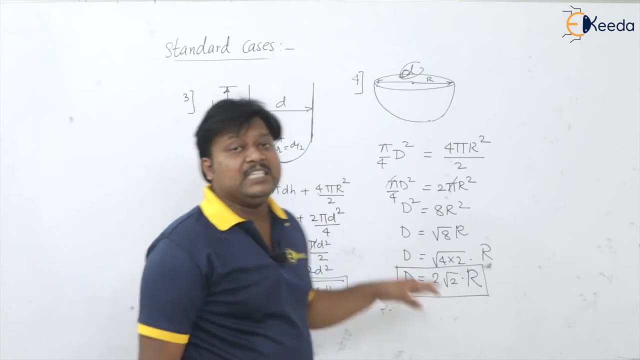 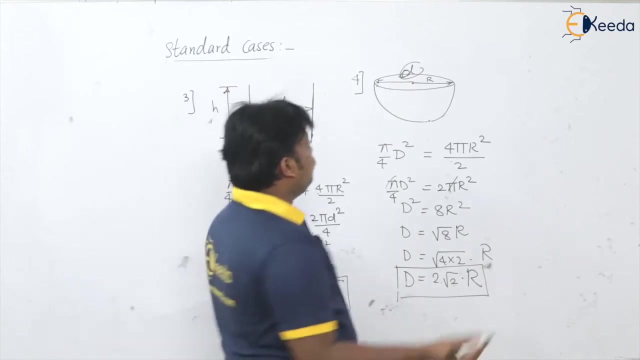 capital d is equal to root 2 time. root 2 times 2 r is nothing, but simply you can write the d. so these are the special cases for that we can able to calculate the blank sizes. okay, you can try it at home. let us take this fifth number as. 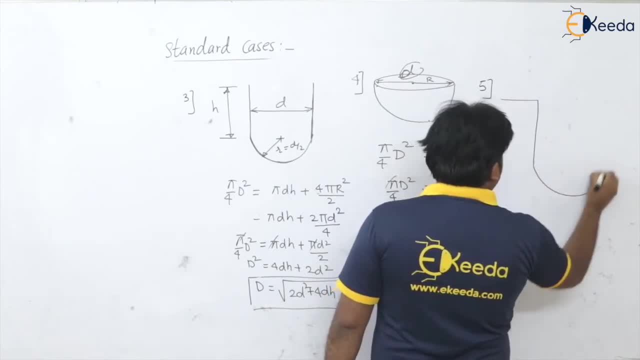 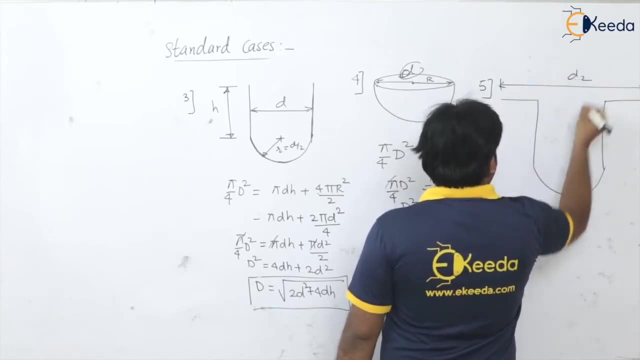 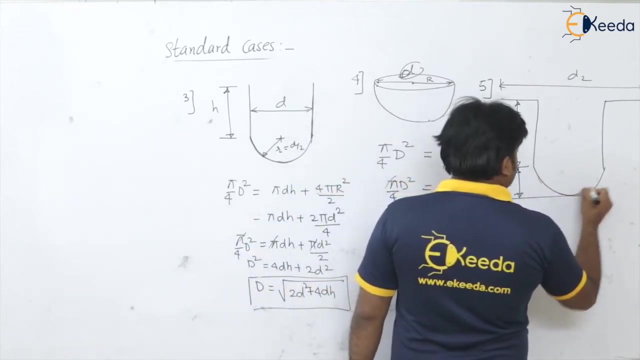 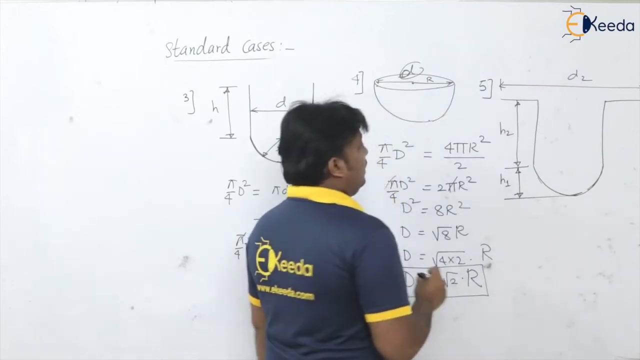 this is flange d2, this is h2 and this is as h1. okay, so let us assume that this is the semicircle circle part here, not hemispherical, it's a circular and you want to find out, and this is also provided with the flange at the top. 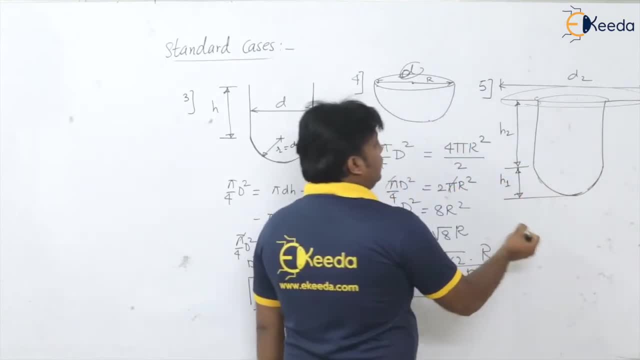 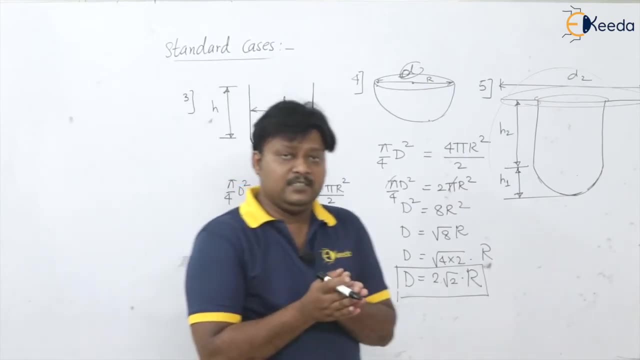 portion. okay, so calculate the blank size for this shape so you can take the shape. just what we have to do: you have to equate the one side surface area of the blank with the one side surface area of the product or cup. okay, so this is very 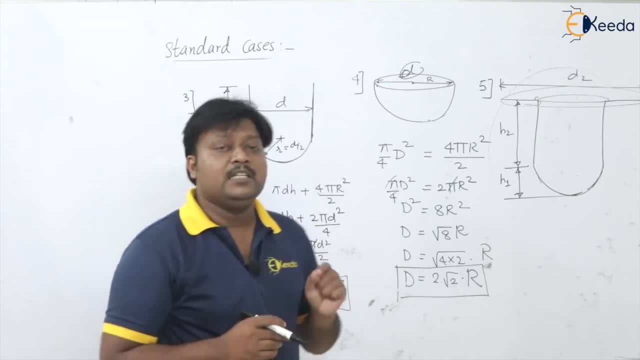 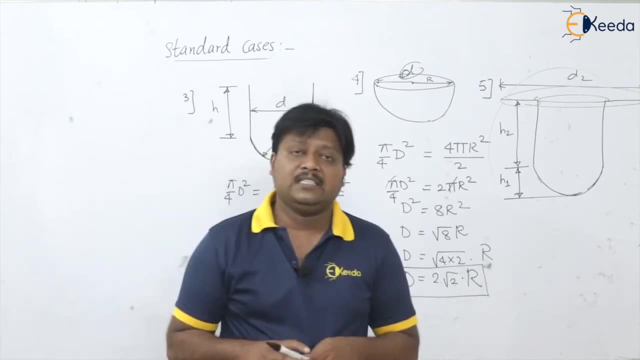 very important thing to know. okay, so this is very, very important thing to know. there is a reason why we are saying that again. okay, so let us find out. and then, how about further the idea here so that we will get the total energy right just by using this form- housenorm in the roughness population and left? 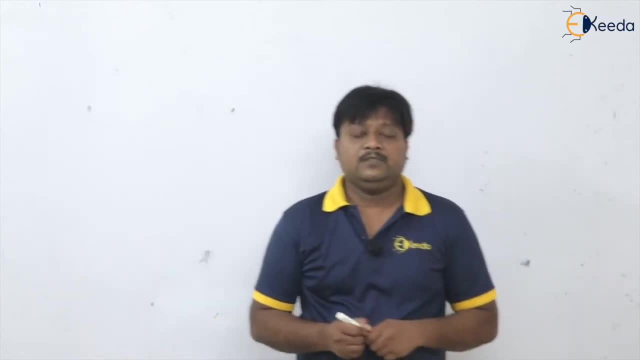 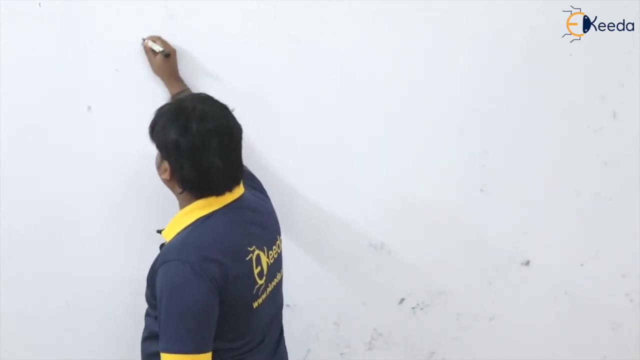 we can use that for the simply so, whether we have z that isgerÞOÌÌÌÌÌÌŋËÈÊ� cuiqrÝààÛUÕ ÈTÄÏ se LanaÏÌÈtÔ Û 95 Finnish˛ºçÔçÔÉ ãæ narÏÎšææḳõ correantº æÜè éŒ ę†. 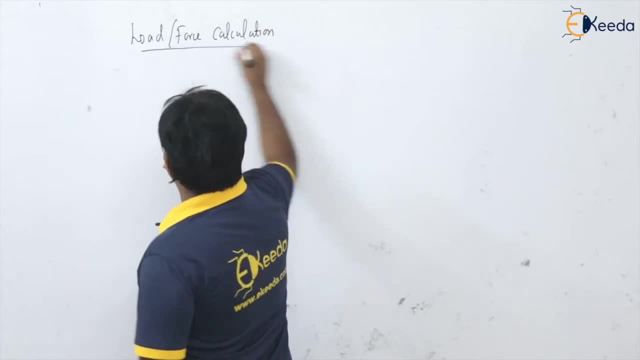 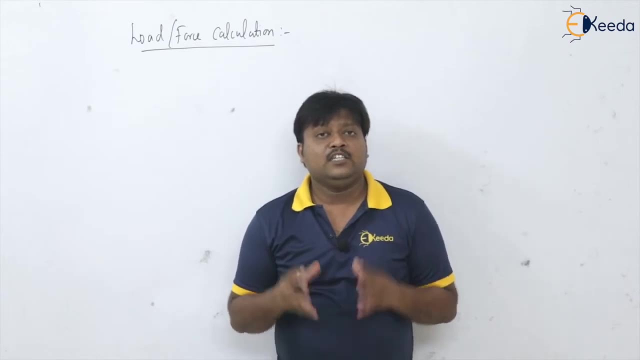 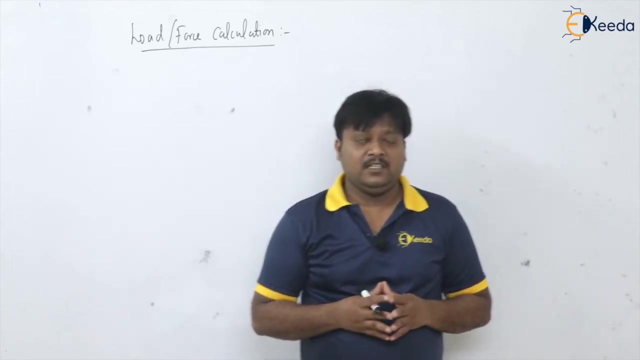 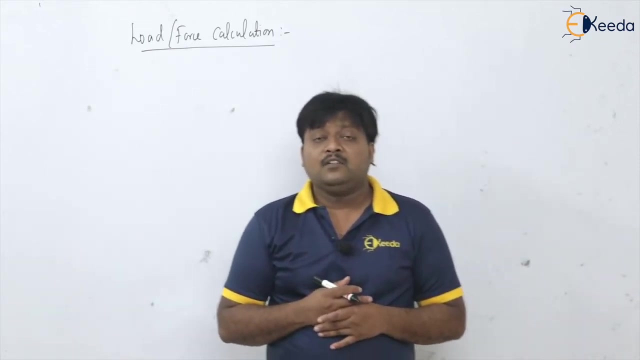 þόs deep drawing operation. so, students, basically in deep drawing operation, we are using the punch and die combination for doing this operation at the same time, if you talk about the clearance between this punch and die. so of course, here no cutting, no shearing is going to happen. so we are providing the clearance. 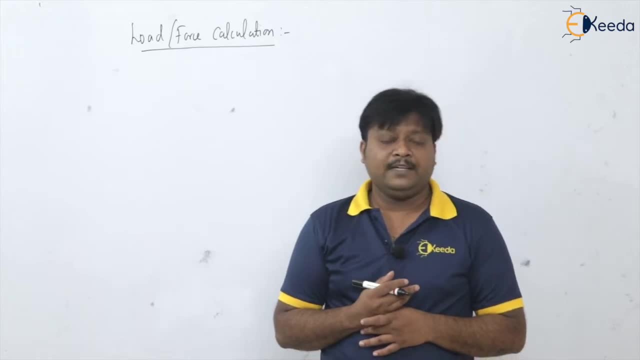 as equal to the thickness of the sheet. okay, so this is the clear about the clearance. now, if you talk about the loads in the deep drawing operation, see, it is always better to do this deep drawing operation in the number of stages- it is number of stages are preferred for doing the entire operation. 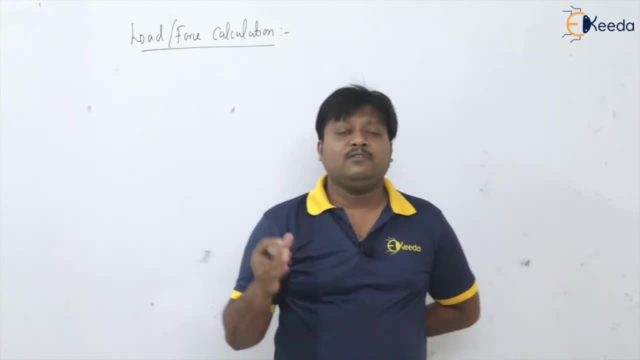 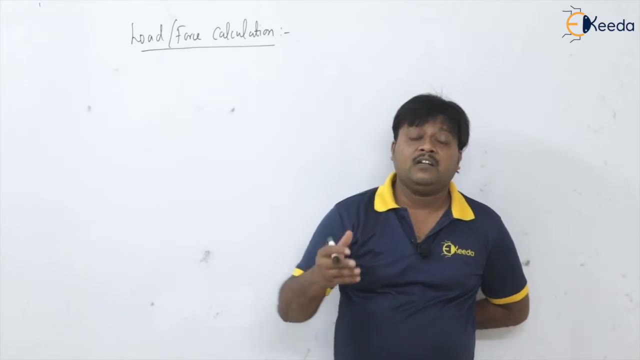 why it is so. so suppose if you are going for is only a single pass deep drawing operation. so the stresses in this operation are, if you talk about the average, stresses induced are just equal to the ultimate strength of the material and there are very damn chances that, definitely at certain critical sections. 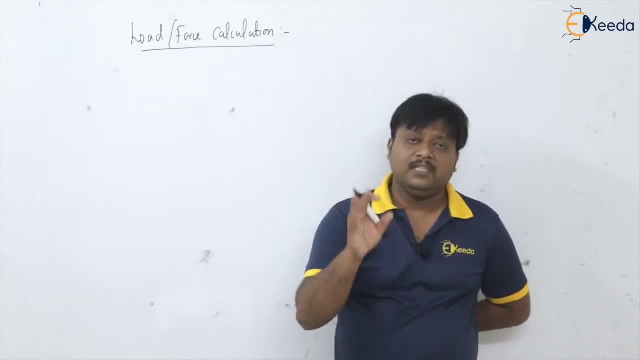 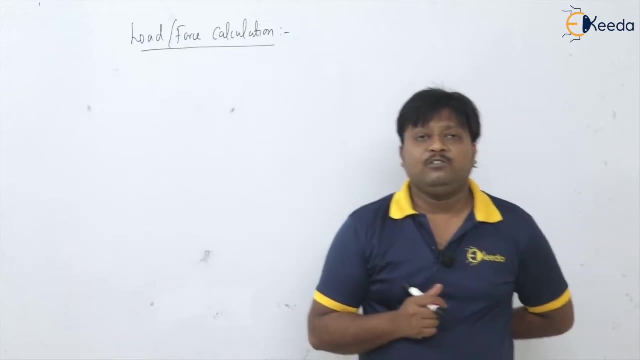 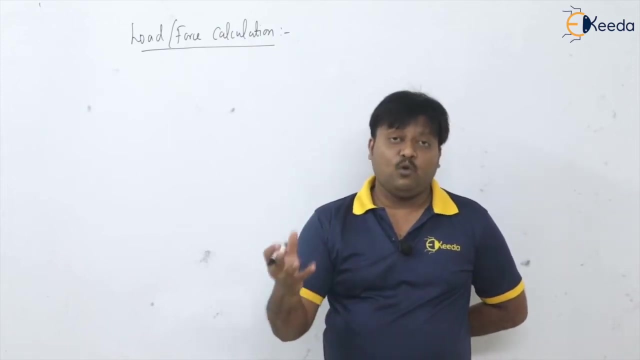 the cracking or failure will occur. so that is the reason why we are always trying to have the deep drawing operation into the number of stages, or that. stages are also called it as the drawers or the strokes or the blows. you can use any word: stroke, blow, draw, step, pass- any word you can use. 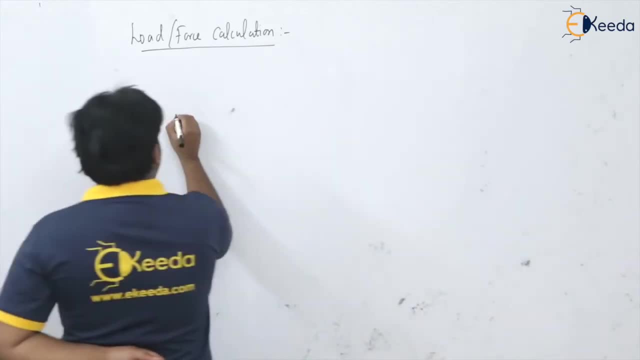 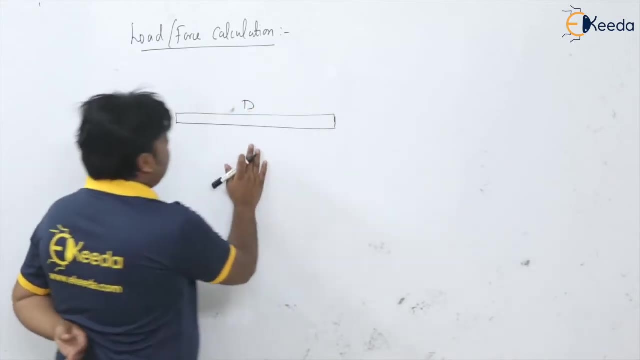 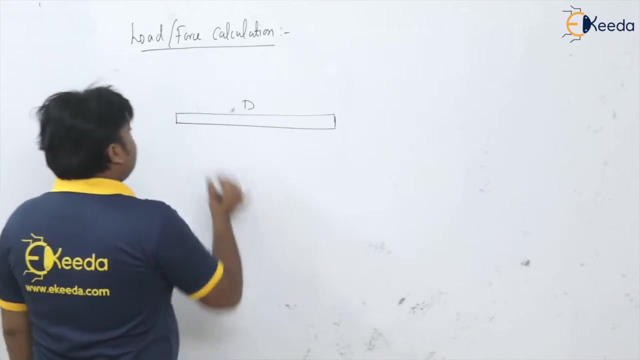 so see, suppose this is the original but blank that we are having with the diameter D and this blank is undergoing the deformation to form the deep drawing operation for a cup we know very well. so suppose, if this blank diameter say 120 millimeter, okay, and from. 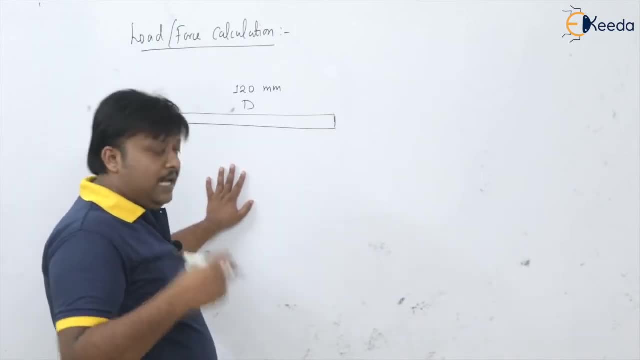 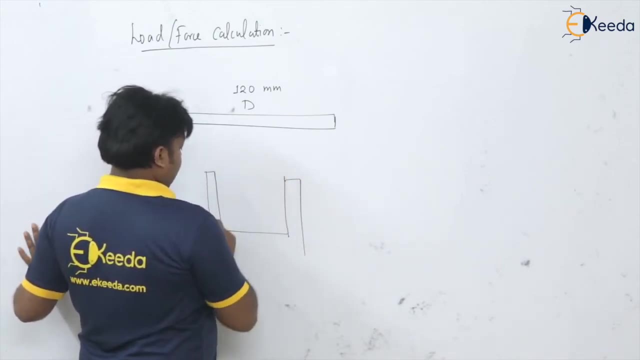 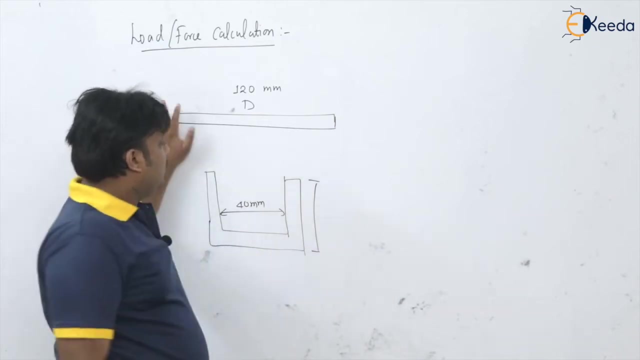 that suppose I need to produce. suppose I am going to produce the cup of, say diameter, say 40 mm, okay, whatever the height, okay, but directly, see, I am not going to have that directly, this 120 millimeter size of blank getting converted into the 40 mm cup diameter. 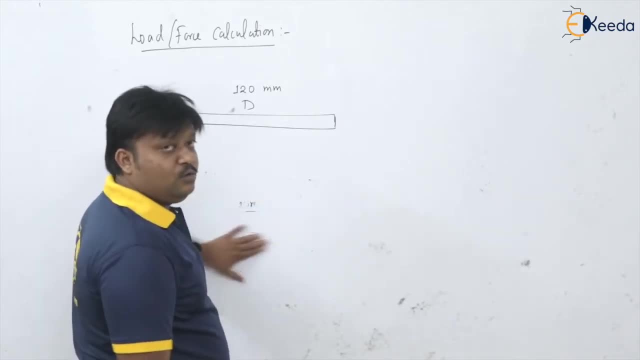 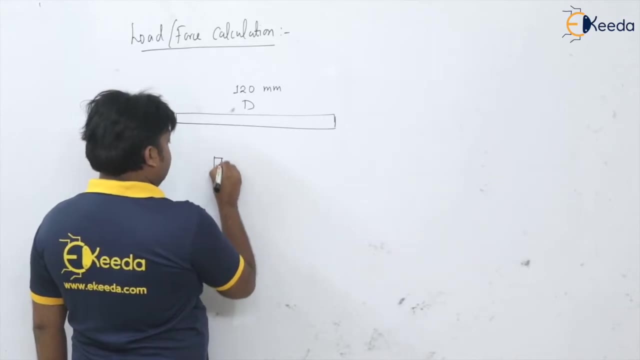 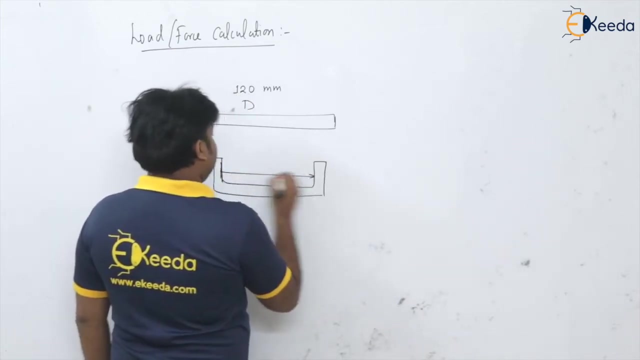 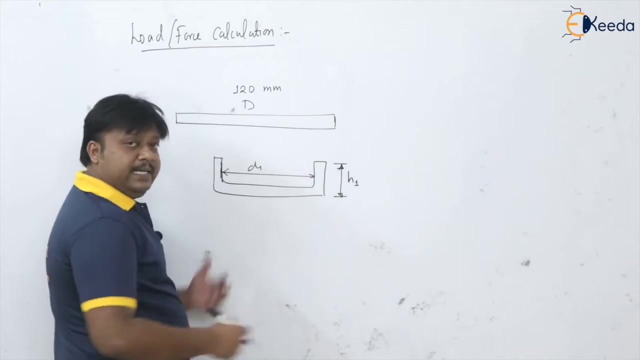 okay, so how I can go for that. so I will have the number of passes for that. so say, first pass, I will go for this much reduction in the diameter. and at the first draw my diameter say say D1 and the height which achieved is H1. now again, I will have the subsequent reductions, like now again. 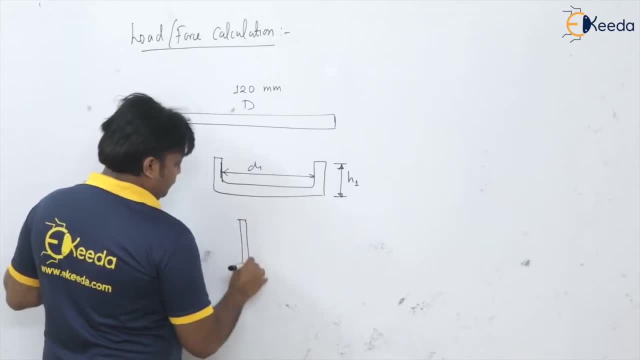 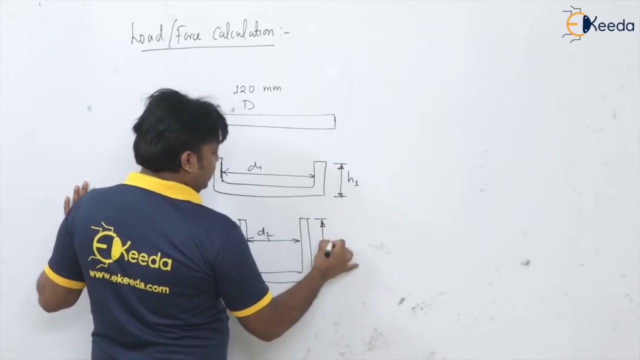 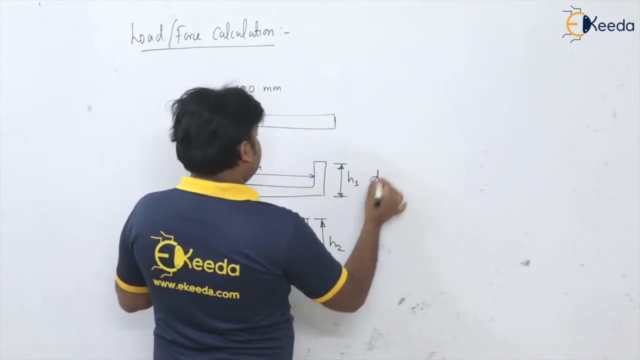 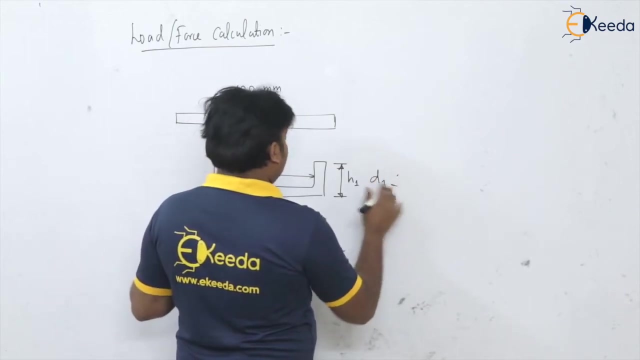 I am going to have the reduction in diameter and increase in. so this is, say, diameter D2 and the height in this draw or pass is H2. so every time what I am checking, so obtained diameter should be what less than equal to required one. once it is gate this equal to the required diameter, so I will stop the reduction. 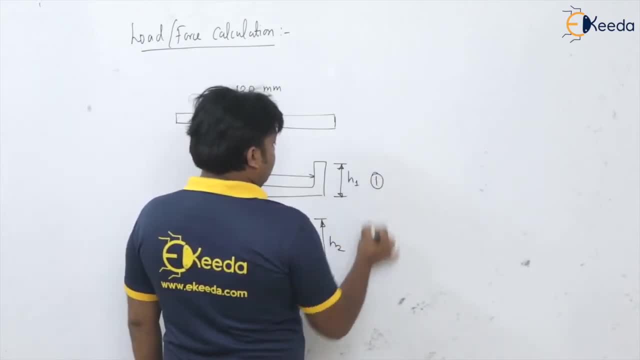 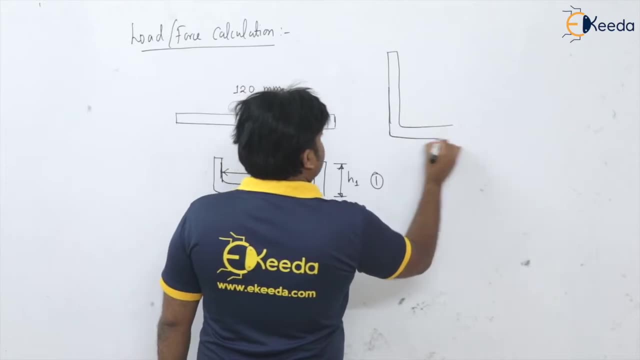 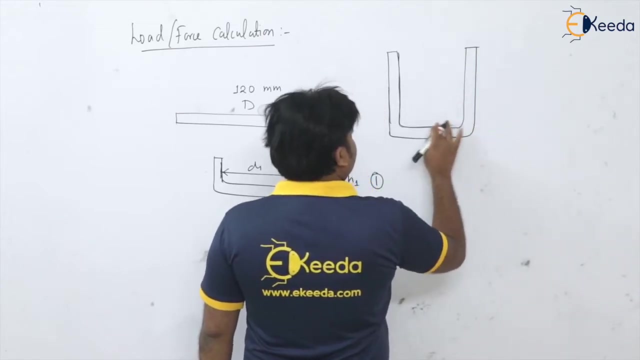 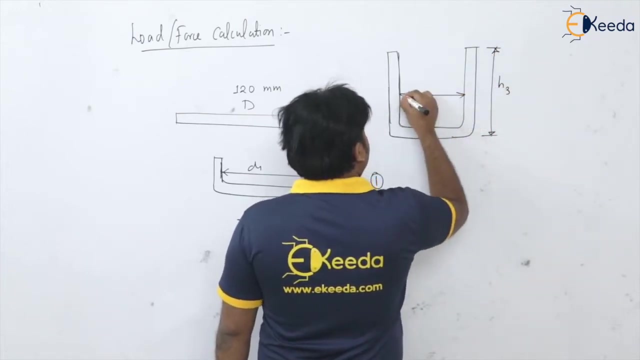 isn't it so like that in number of states say: this is pass 1, this is pass 2? again, in pass 3 I got the required height or the diameter less than or to the required one. say, at the third stage, i got the required height, h and the required diameter. 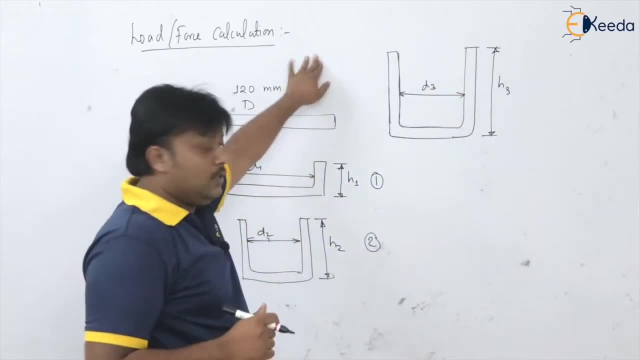 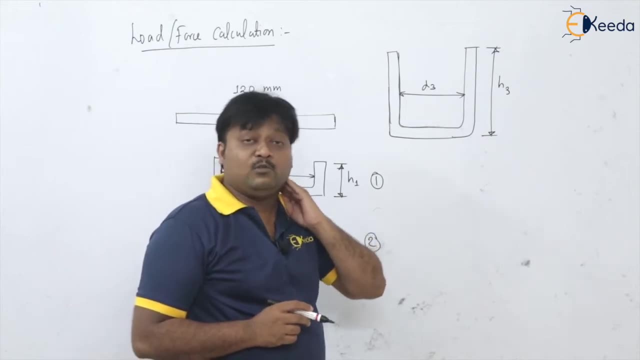 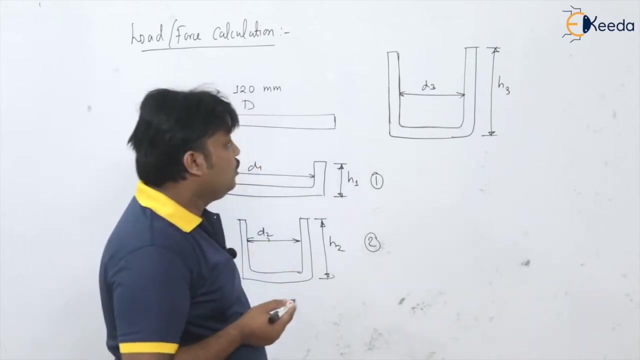 for the cup. so like that, we are going to have the number of passes, so the force is also going to be calculated in the number of stages. but let us say how to calculate this force for this deep drawing operation. so it is simple: the cross-sectional area multiplied by the yield. 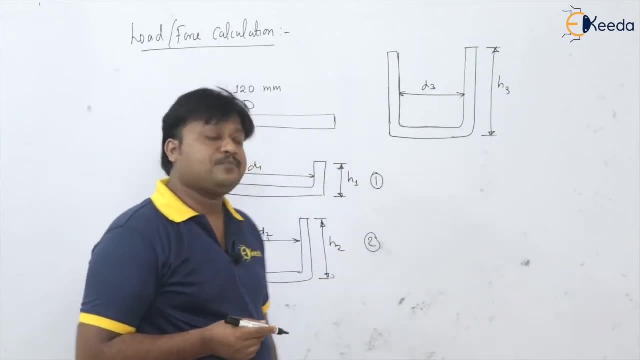 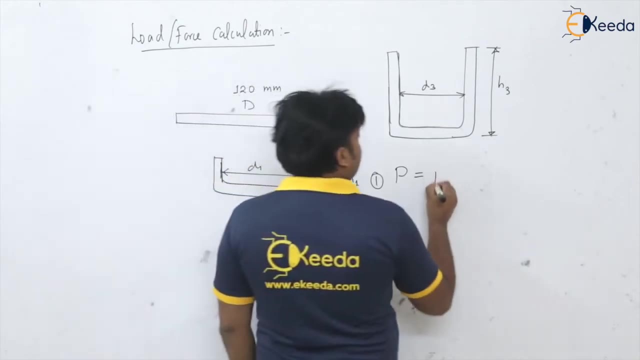 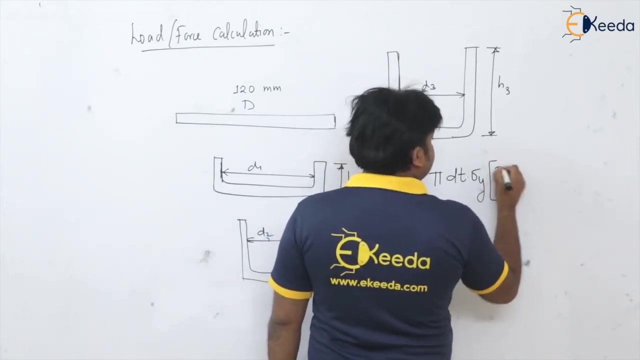 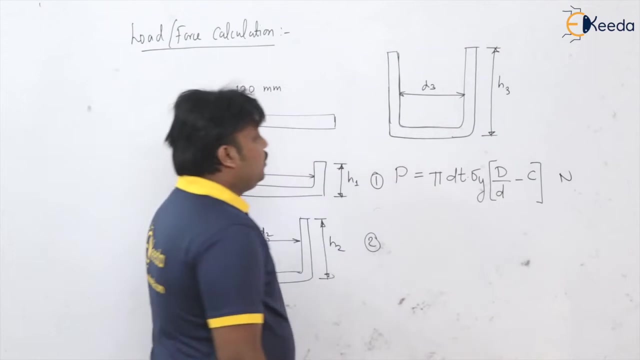 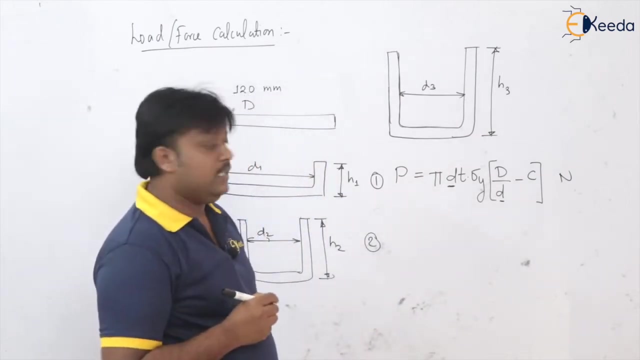 strength of the material we can going to get the force which is indicated by p in the deep drawing operation, as it is, pi d, t, into sigma y, into bracket d, capital d upon small d minus c times newton, okay, okay, okay. so here, this d, small d is diameter that you want for that cup. okay, suppose this is a cup. 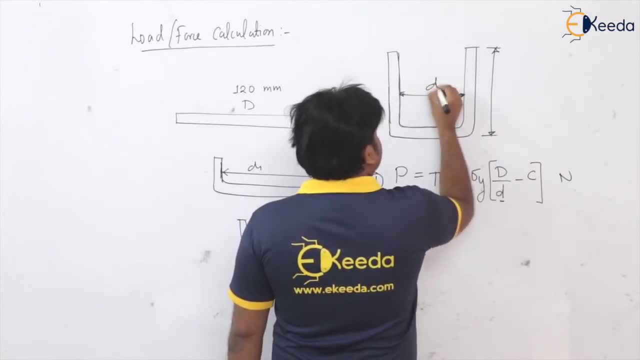 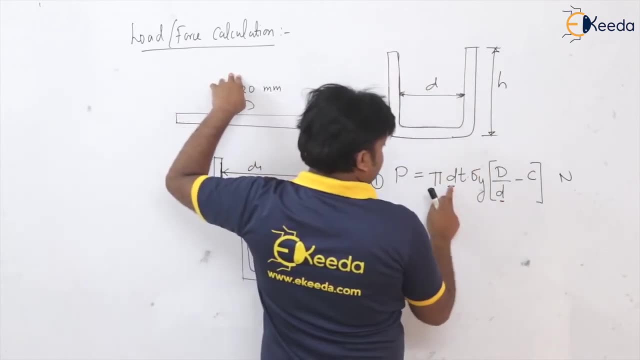 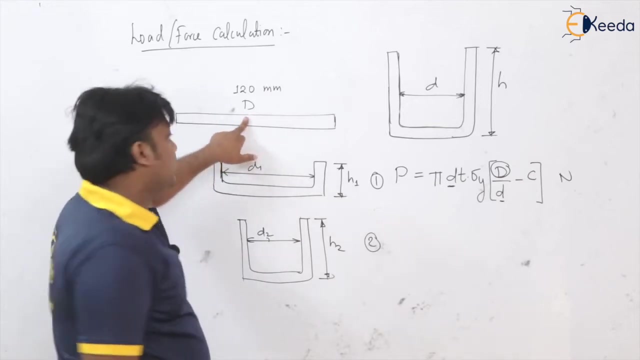 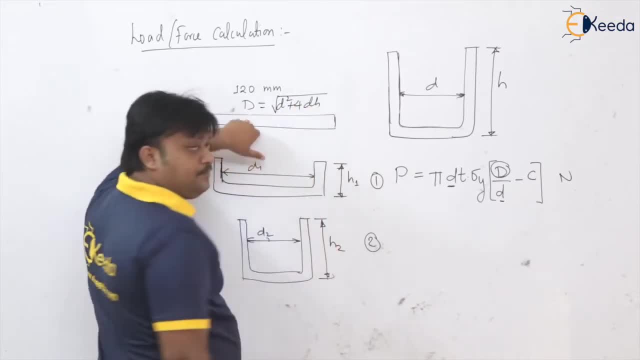 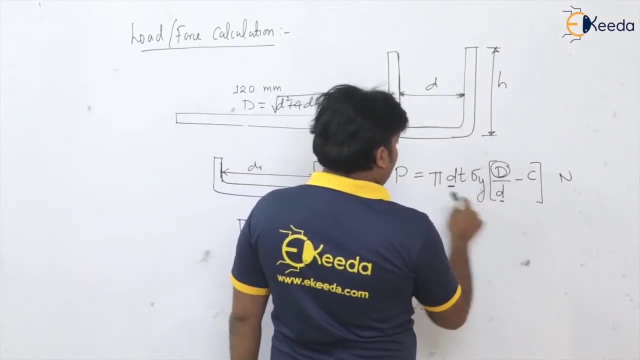 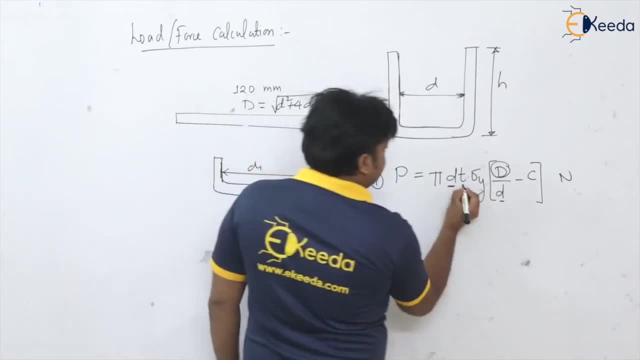 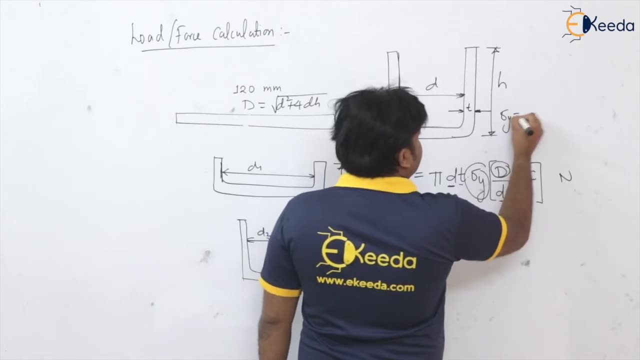 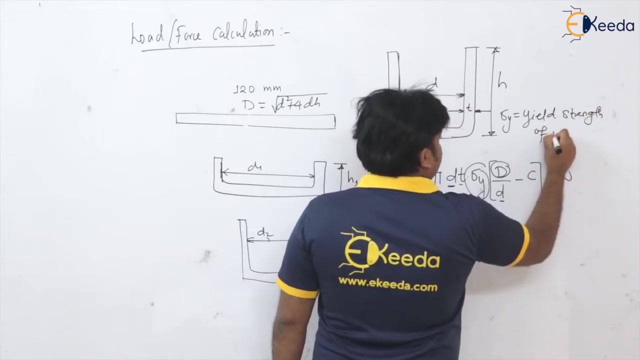 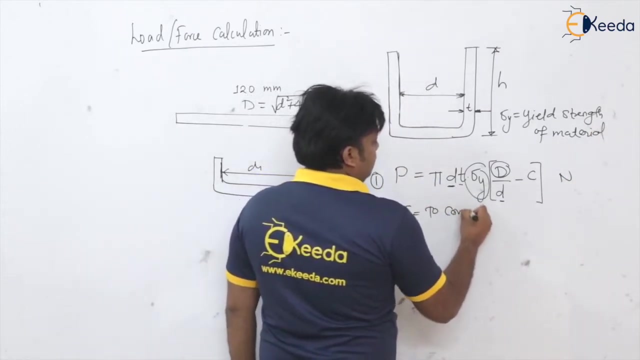 Aye formula for this deep drawing operation, where t is what the thickness of the sheet and Sigma Y is what the yield strength. doctor, remember, this is the yield strength of the material. okay, uestos, alright, okay, well, bye, see you, bye and what you see. this is the constant to cover the friction and bending of the 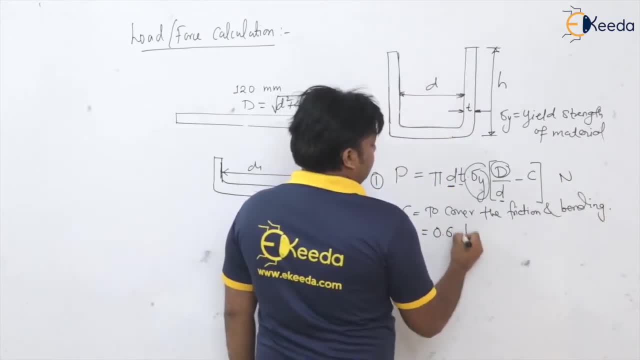 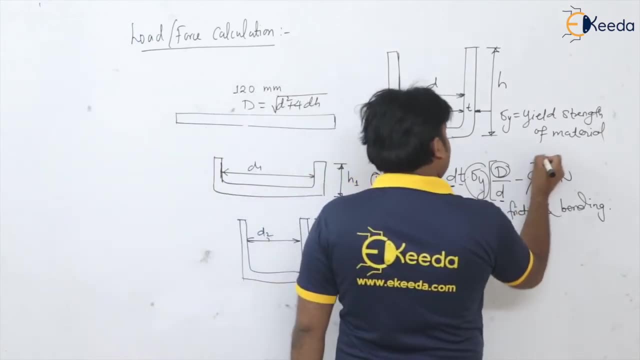 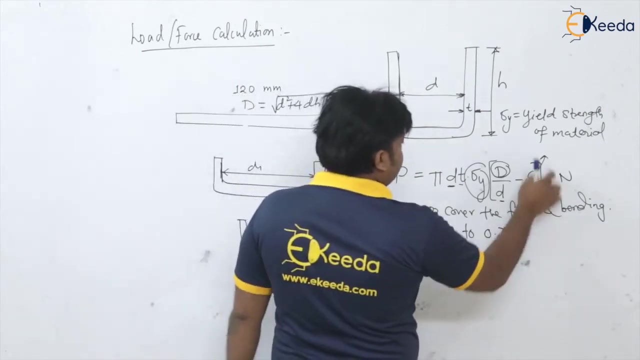 sheet. okay, so generally it is equal to 0.6 to 0.7. okay, suppose it is not given in the question. you directly neglect it, you directly negate it, so what you are remaining with? so if c is neglected, so you can have only here. 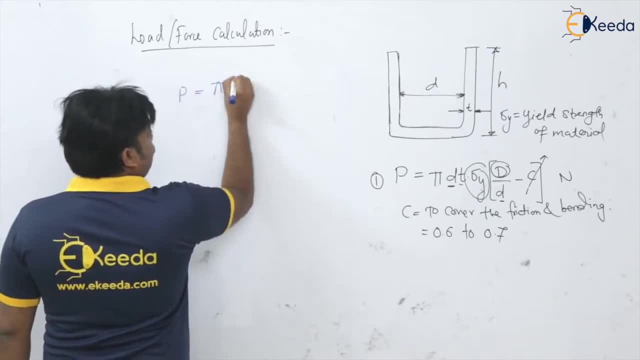 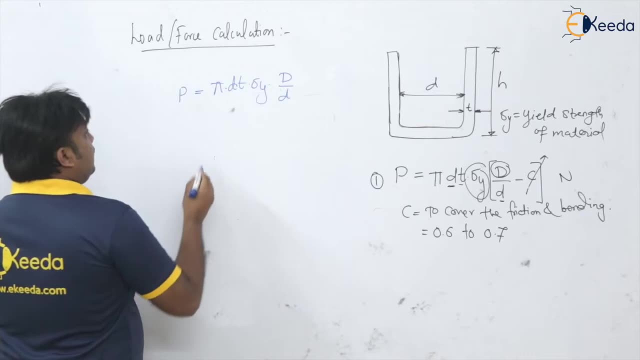 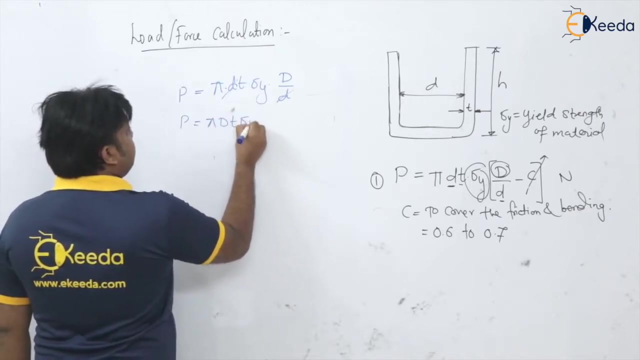 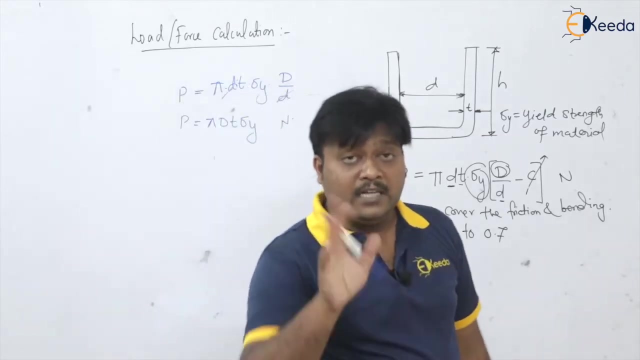 that p is equal to pi into d, into t, into sigma y, into capital d divided by small d. okay, now from this, this d d get cancelled. so p is equal to pi d t sigma y times newton. okay, so this is the force in the deep drawing operation. now what we discussed. we discussed that. 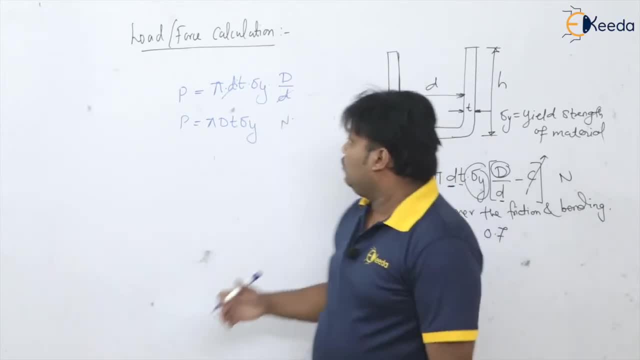 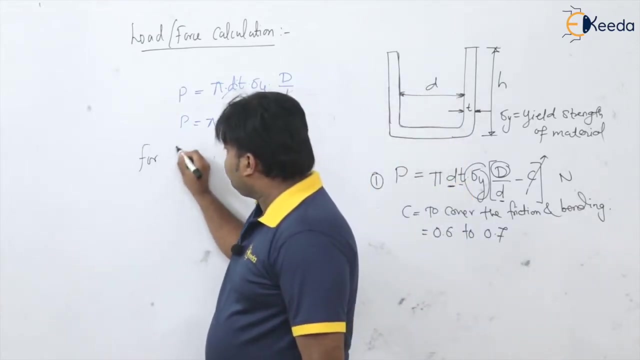 so go for the stage wise operation. so so also the force will be the stage wise, isn't it? so let us say: i want the number of stages, i want to do the operation in the number of strokes. so definitely the for the first stroke, suppose for the first pass or stroke. 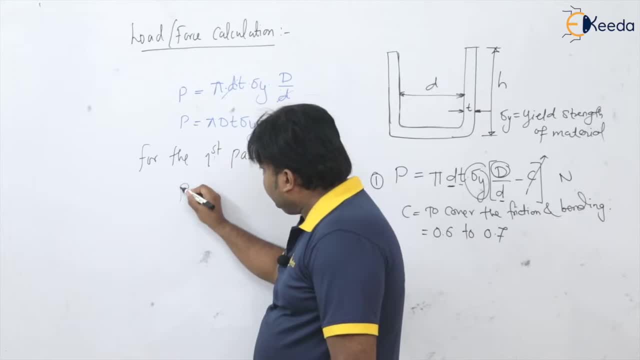 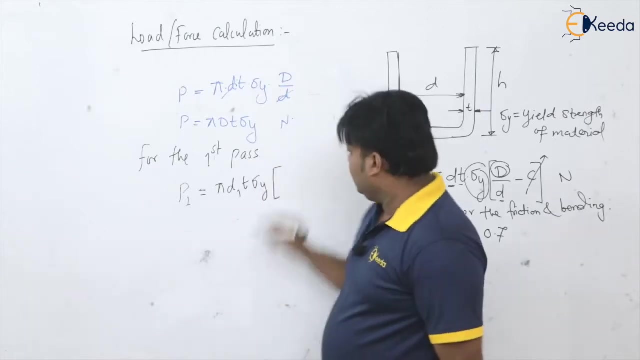 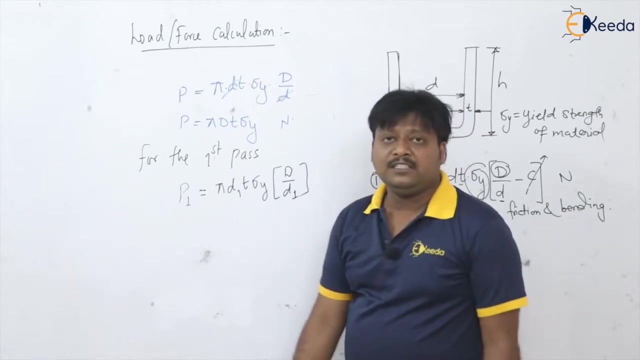 what will be the force? so i can write, say p is replaced by no, p1 is equal to. i will write the full blanket d1. i am not considering c, it is neglected. so the first for. so the force or load in this secondłbymше. 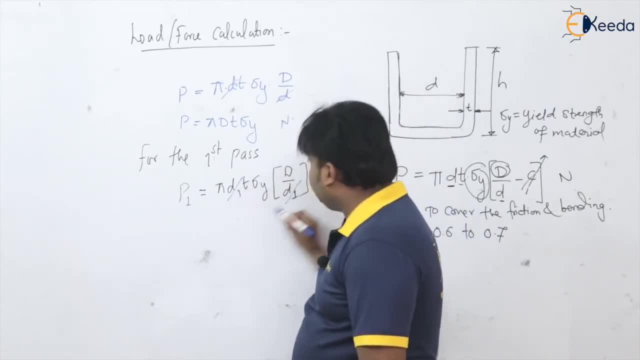 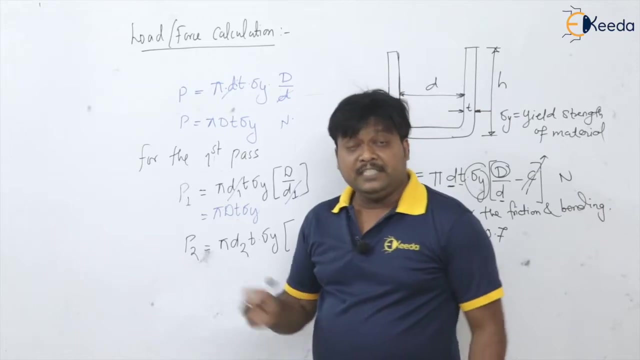 the first stage is how much this d1, d1 gate cancels. you got here pi capital d, t into sigma y, like that. if you want to find out the force or load in the second stage or second pass, how to write this pi second stage d2, t times sigma y. now which, which diameter you are drawing. 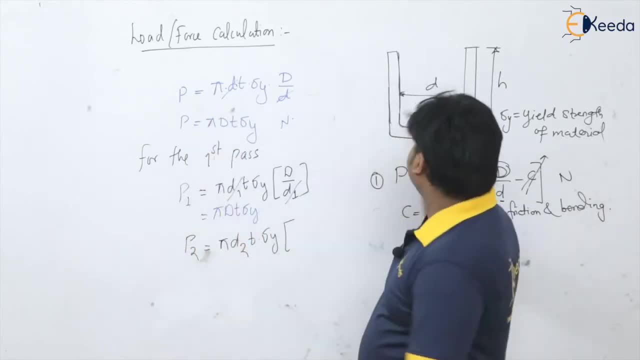 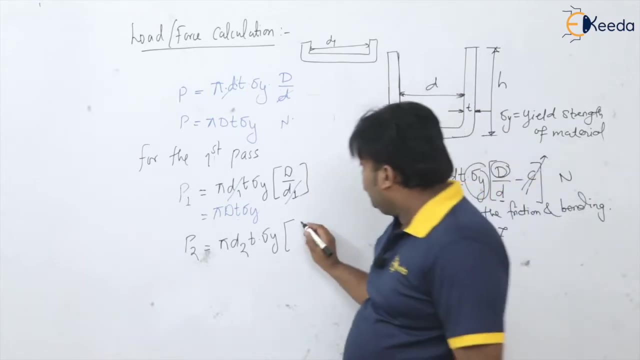 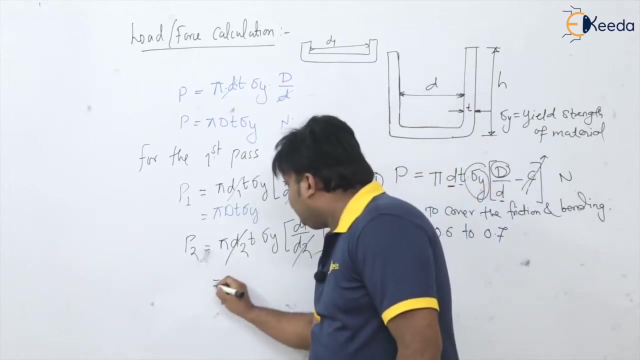 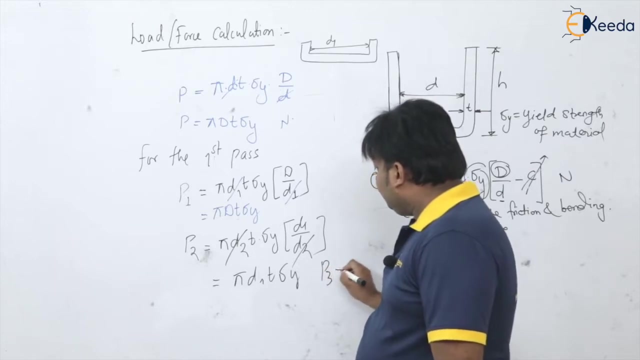 now capital d is no more. you are available with the first stage diameter and you are going to deform this. so this is d1 divided by. go ahead and get second stage d2. so d2, d2, gate cancel. you left with pi, d1, t sigma y, isn't it like that? p3, yes, say pi. so d1 came here. 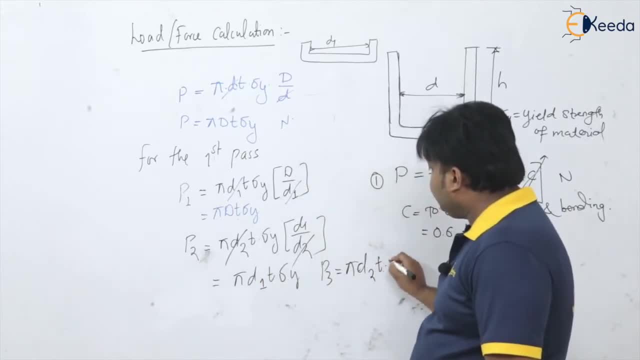 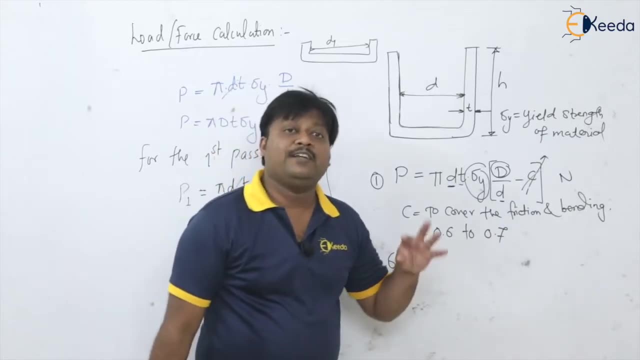 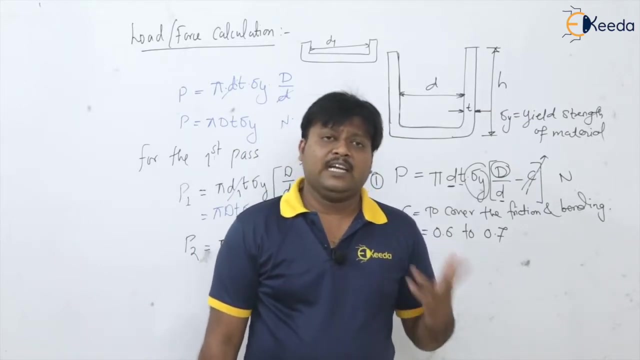 then you got d1 here. now capital d is no more. you are available with the first stage diameter and you are going to here pi, d2, t times sigma. like that you can go on calculating the force for every stroke, every stage in the deep drawing operation. please remember this once you are calculating the force. 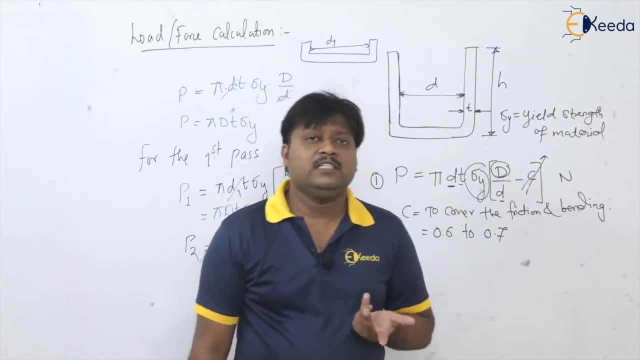 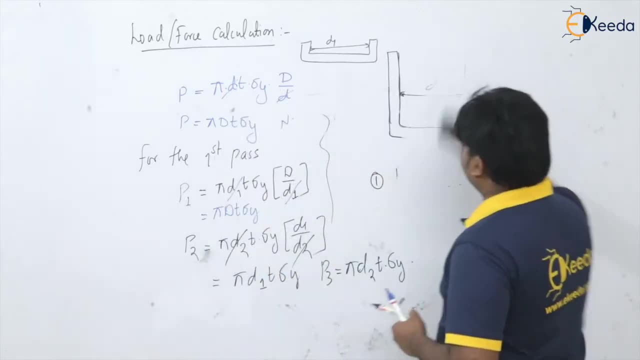 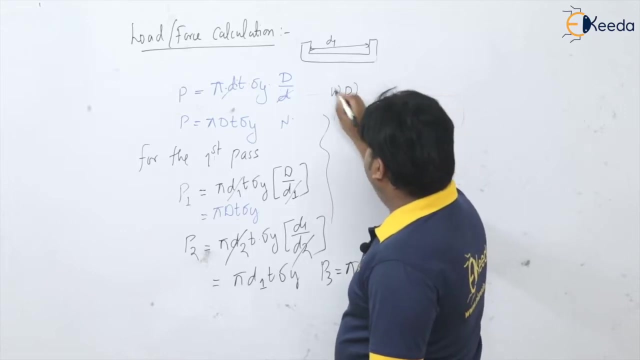 then also then the work done. calculation is much easier. how to calculate the work done? so you know work done is what? the force into distance. so if i ask you to find out the work done at the first stage, or first stroke, first pass, how will you do so? it is force into distance. 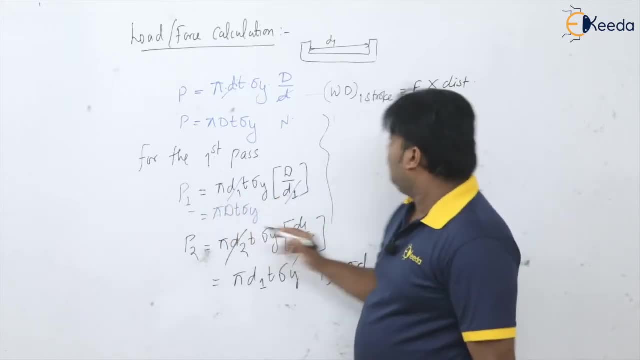 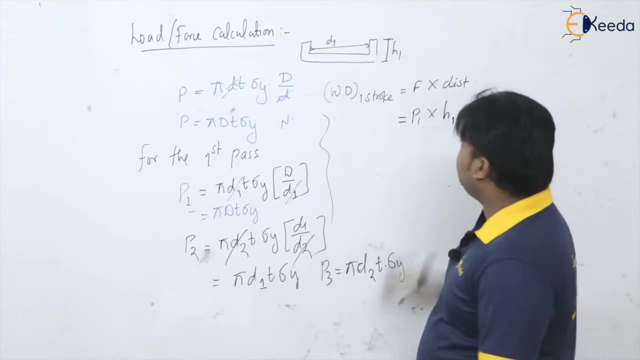 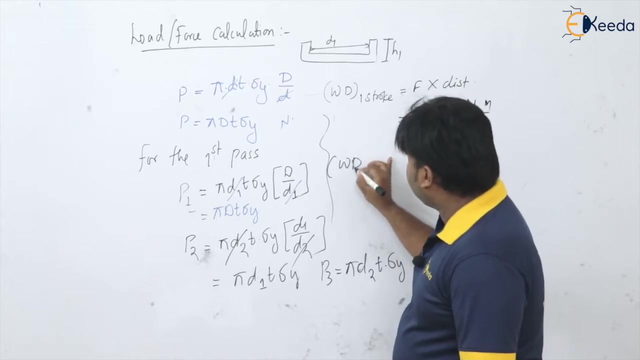 so how much is the force of first draw p1 into how much height of first draw h1? so p1 into h1. you get this work done in the first stage. newton meter. please remember if i ask you to calculate the work done in second stage or second stroke. now second stroke. 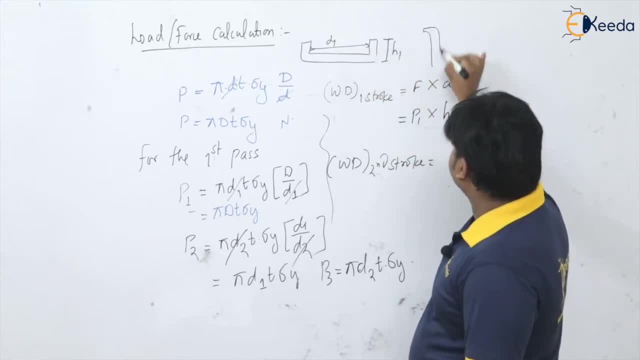 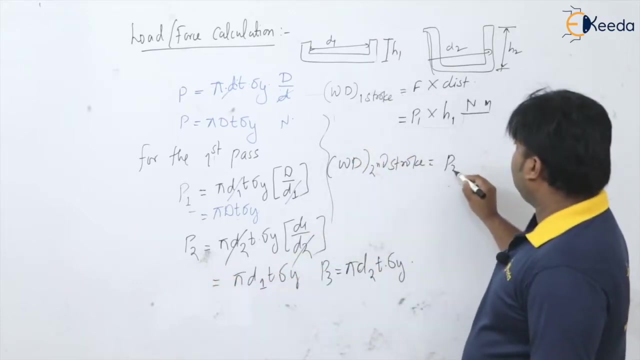 so tell me what is the force? p2 into work done is equal to force into distance. so distance, how much this? h2 minus h1, h2 minus h, like that for the third stage we are having p3 into h3 minus h2, so you can go on calculating the work done also. 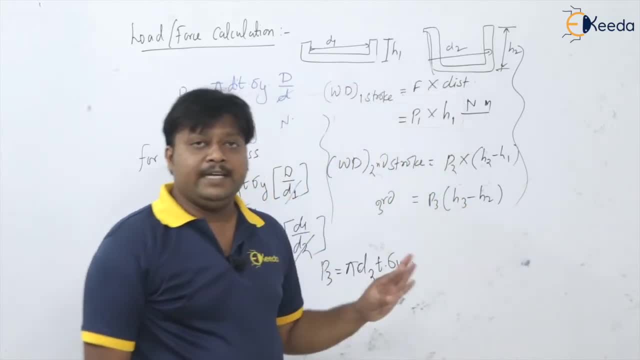 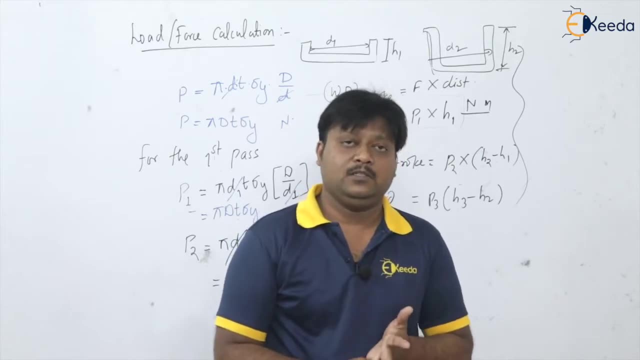 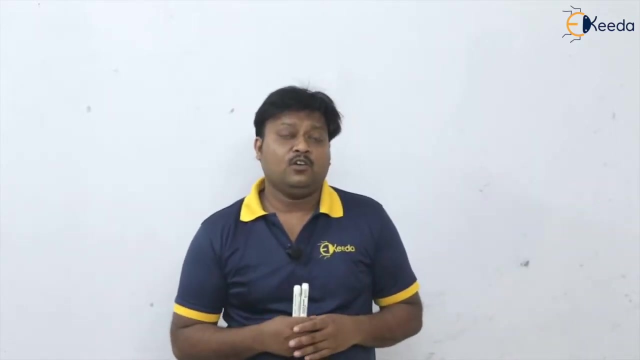 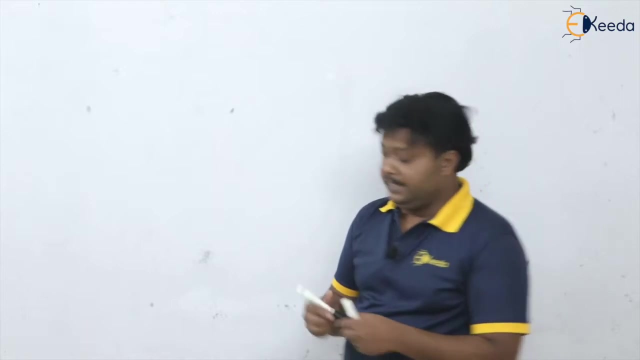 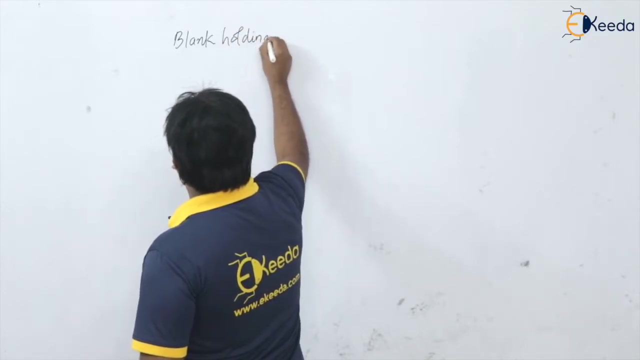 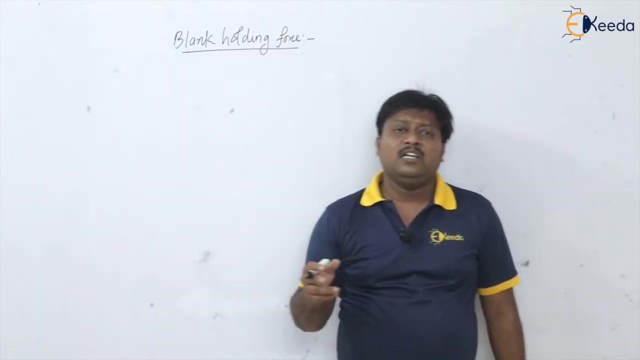 in number of stages. okay, so what we see here in deep drawing operation: force calculation and work done, calculation- okay. so, dear students, after talking about the, the force or load in the deep drawing operation, now let us discuss about the blank holding force. the blank holding force, so basically, this blank holding force is depend upon the tendency of the sheet or plate to get. 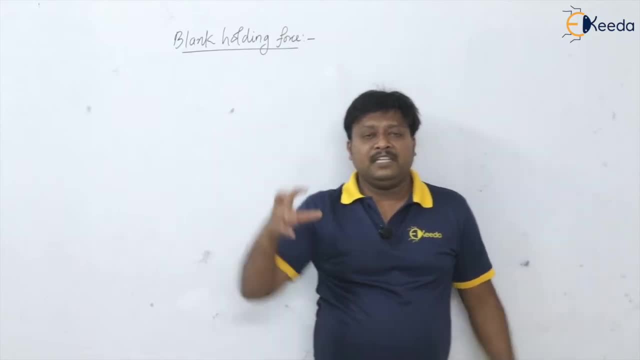 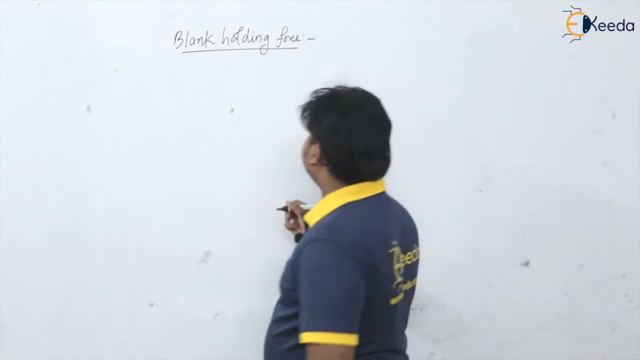 lifted. okay. so when the force is applied by the bunch on the sheet, what happened? the sheet is trying to lift in the upward direction. so this is the sheet, say: and this is our die, When 친근 nhất hasélé force applied by this in upward direction, what is going to happen? this sheet is going to lift it upward. 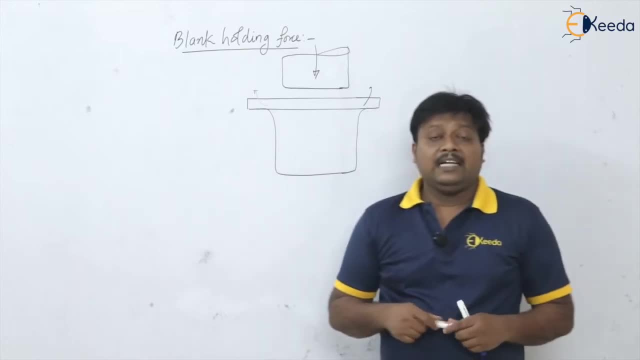 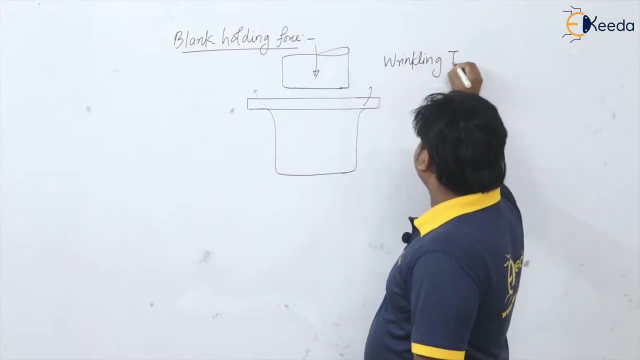 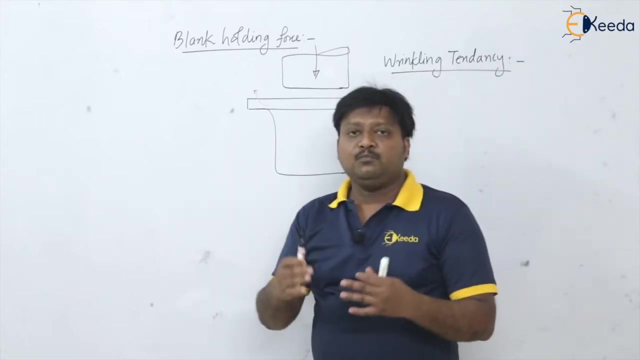 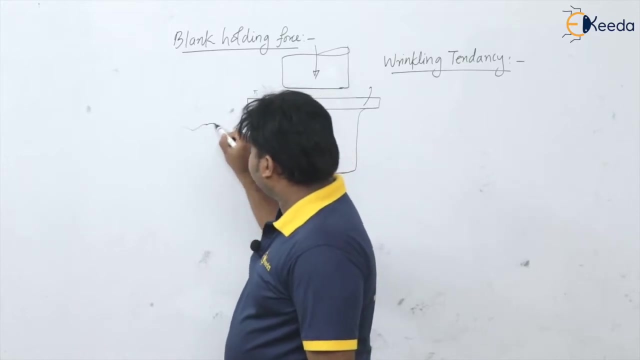 lift in upward direction. okay, and this will leads to the wrinkling tendency. wrinkling tendency: actually, what is wrinkling actually? so wrinkling is nothing but the foldings produced on the flange portion of the cup like this. so your cup will look like this. okay, so this is actually wrinkly. so the 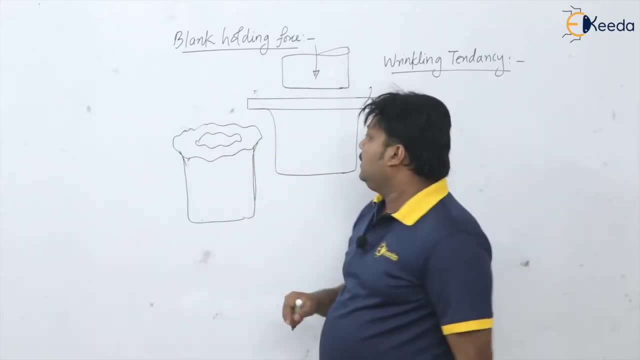 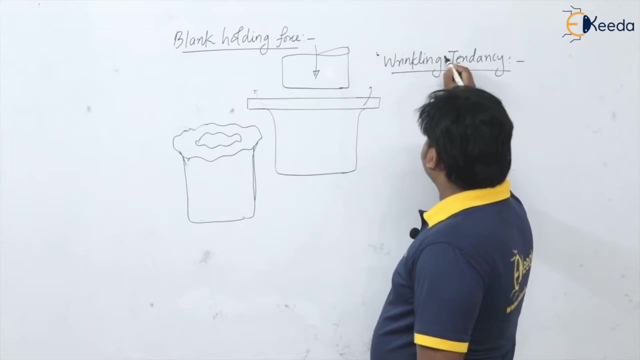 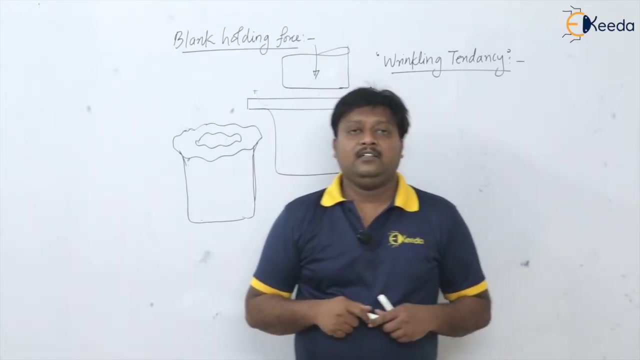 foldings on the flange portion of the cup. this is the actually wrinkling. so this, these are the wrinkles, and this tendency is wrinkling tendency. so because of that, see, the calculation of this blank holding force is very difficult and to get this value the trial and error method is used and empirically we 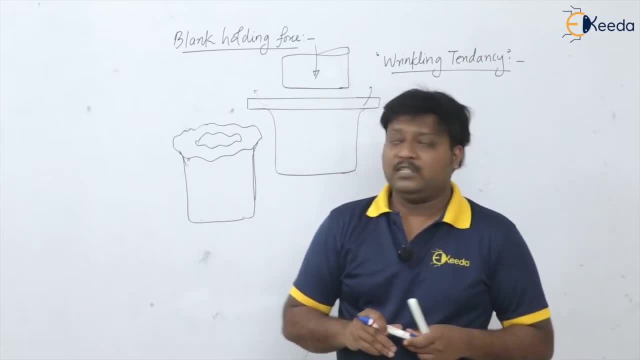 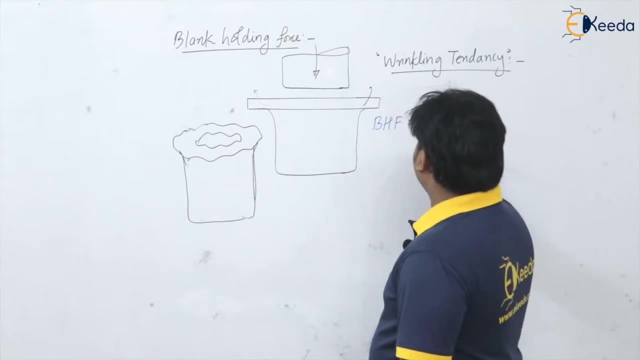 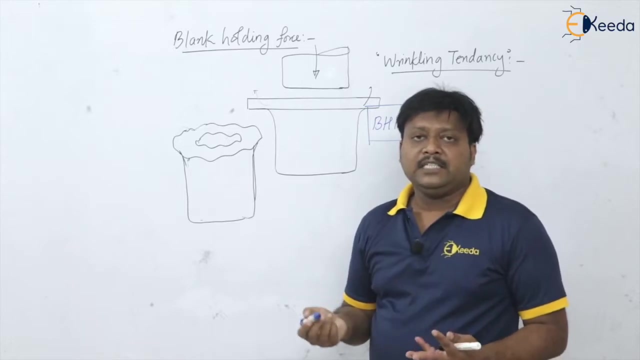 are taking this value of blank holding force as the one-third of BHF that is blank holding force is equal to one-third of the load in the deep drawing operation, please remember. and now, of course, BHF will be the same as that of the load that is in stage two, stage three, stage four, stage five stage. 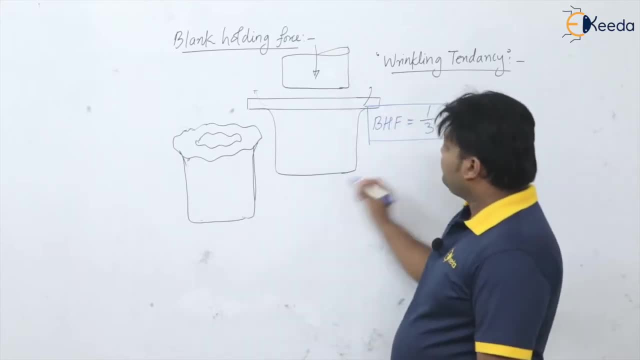 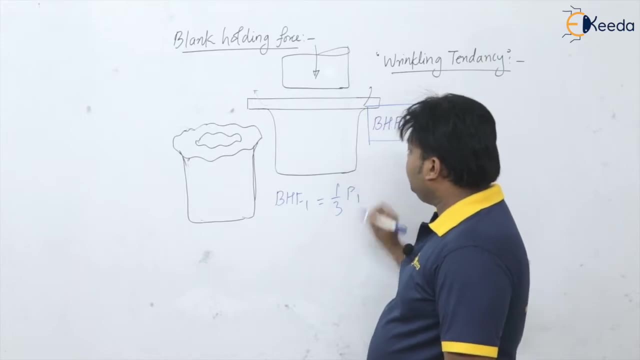 every stage it will be the different. so for the stage 1, BHF 1 will be what? one third of P 1, isn't it? VHF 2? VHF 2 will be one-third of P. to like that, you are having the blank. 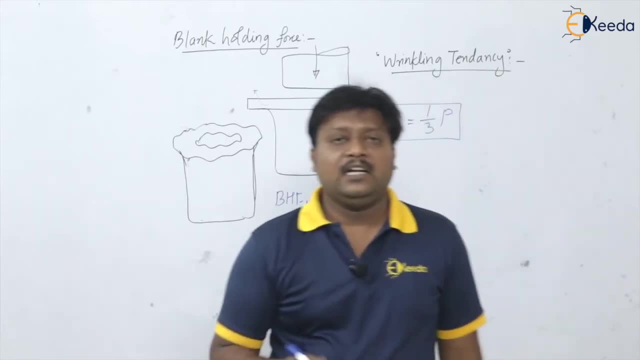 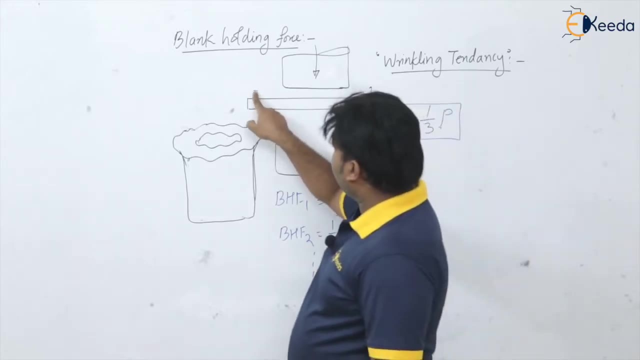 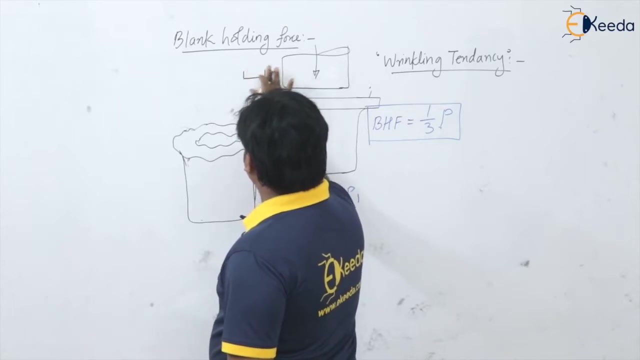 holding force for the every stage, and how much it is. it is generally one-third of this P. the output is: lifting up this, this plate or sheet, what we are using, this blank holding force, that is, these are the spring loaded plates we are going to put here. 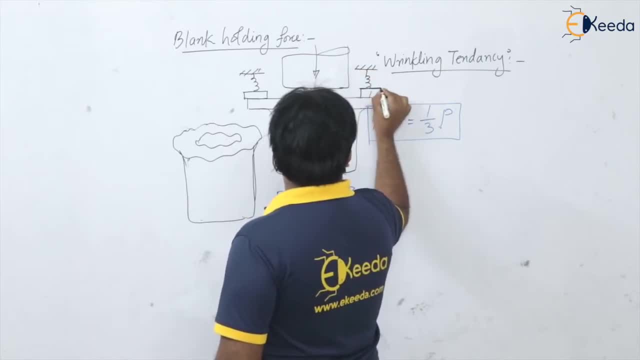 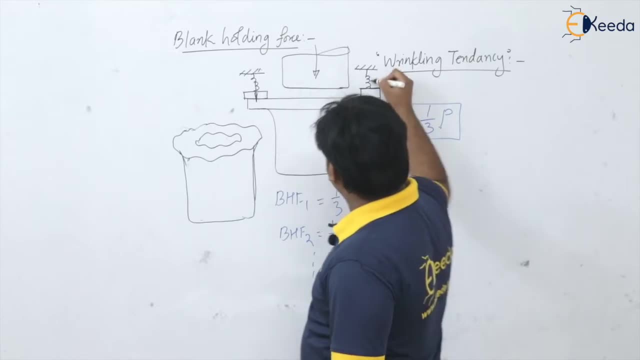 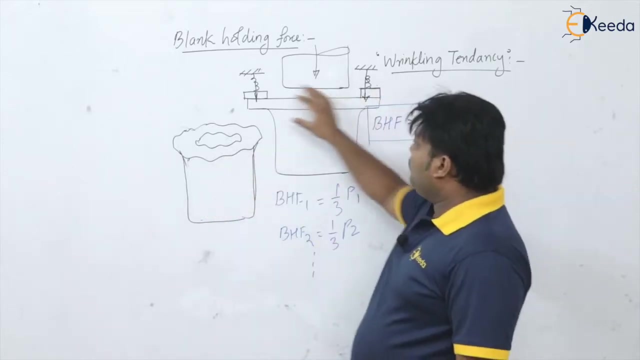 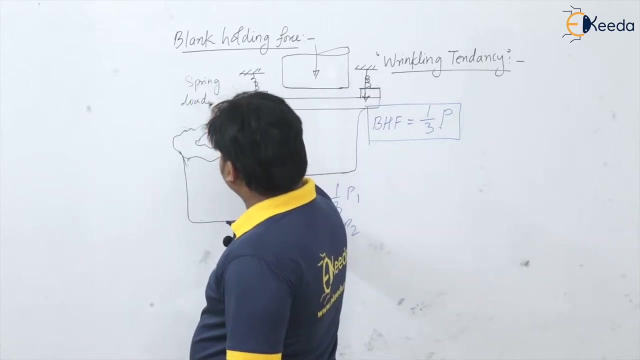 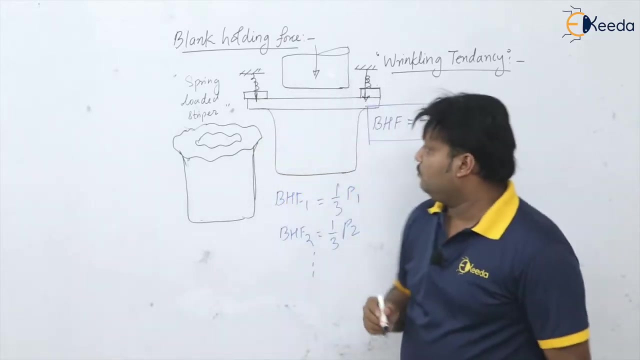 these are the strippers. okay, so these are applying this force onto the plate so that the lifting can be how it. so, by using the spring-loaded stripper. these are what the spring loaded stripper are used. okay, to apply the blank holding force. now see the blank holding force. if you get maximum, what? 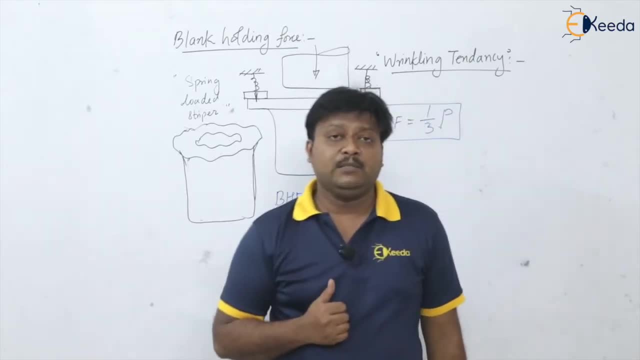 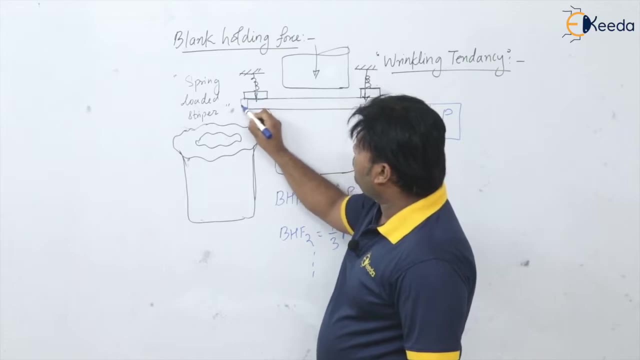 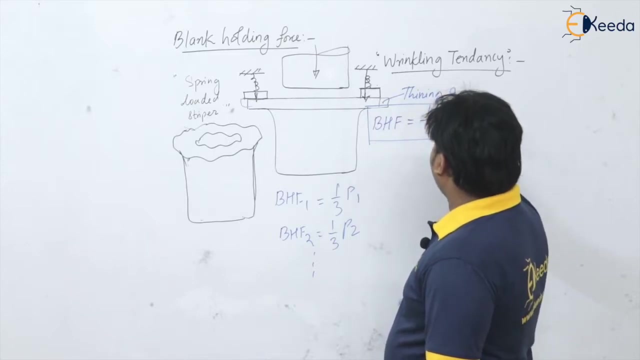 will happen, why it is 1, 3rd of only the load in the deep drawing operation. so definitely, if you apply the maximum blank holding force. so what will happen? the thinning of the sheet may get happen. okay, what happened? the thinning- thinning of sheet or blank, that is going to. 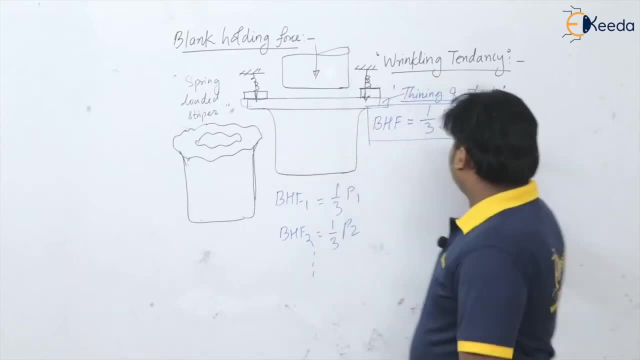 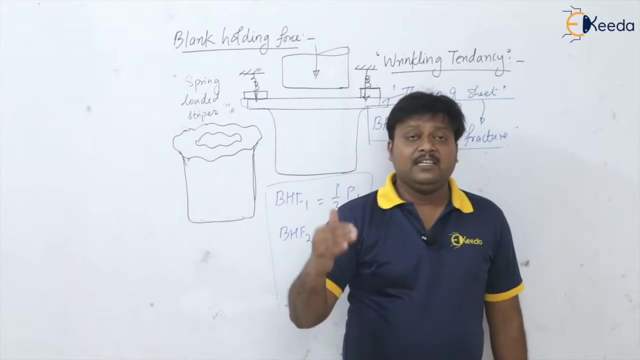 happen, and if it is more so it can lead to the failure or fracture. okay, so that is reason why we are keeping this blank holding force actually in the limit, that is, we are providing only one third of the load in the deep drawing operation, otherwise the thinning will occur and the sheet 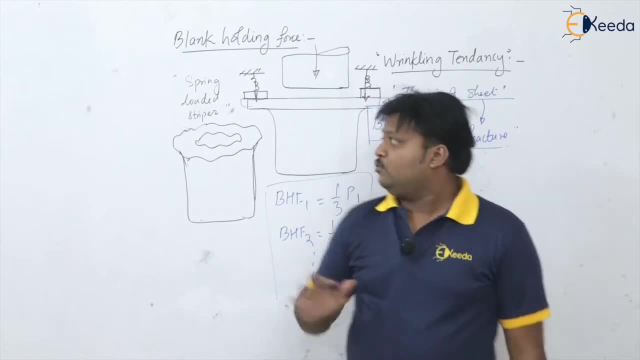 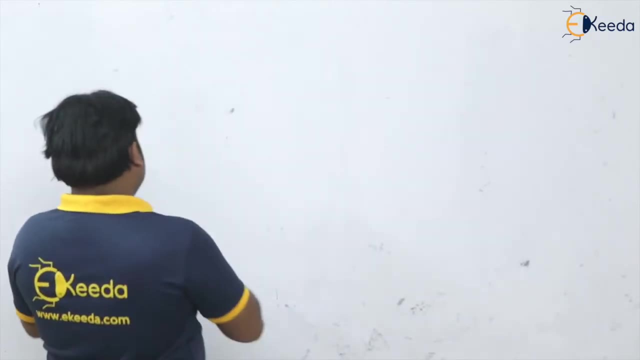 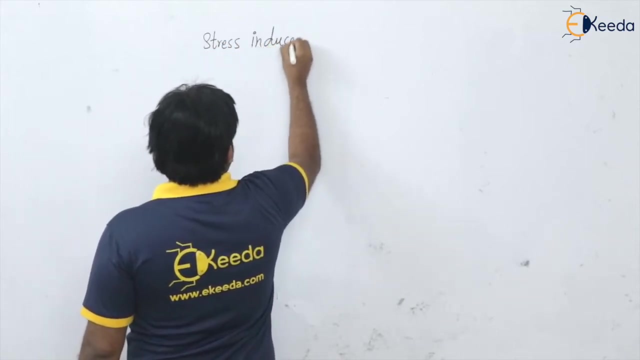 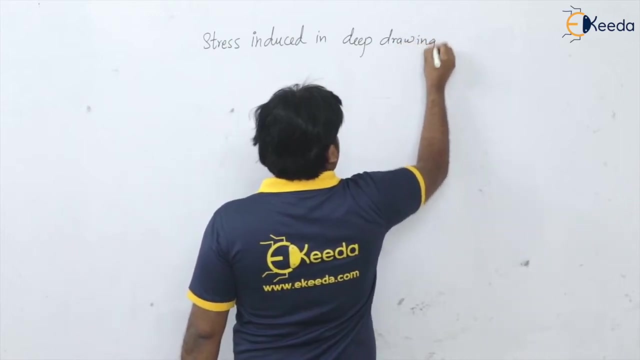 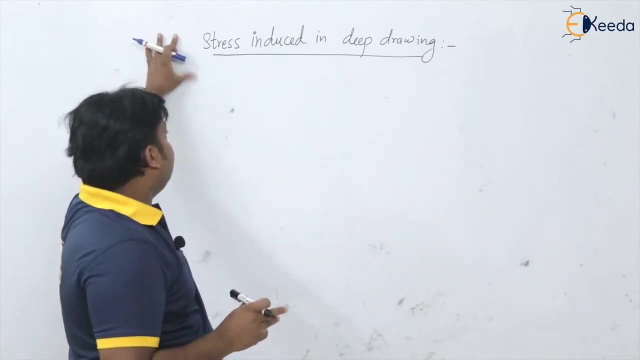 is going to fail. okay, so this is the blank holding force. now let us consider the stress in the deep drawing operation, the stress or stress induced, the stress induced in deep drawing, deep drawing operation. so now we have calculated the force. okay, now how to calculate the stress and, of course, the 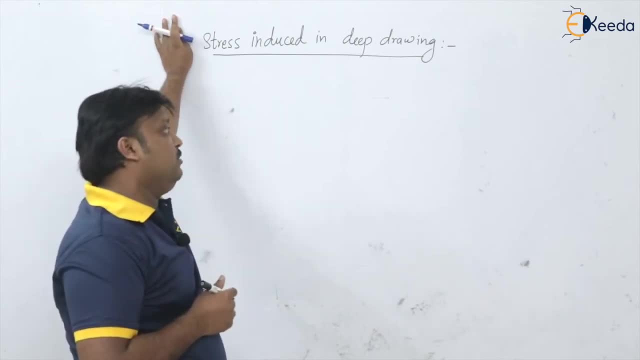 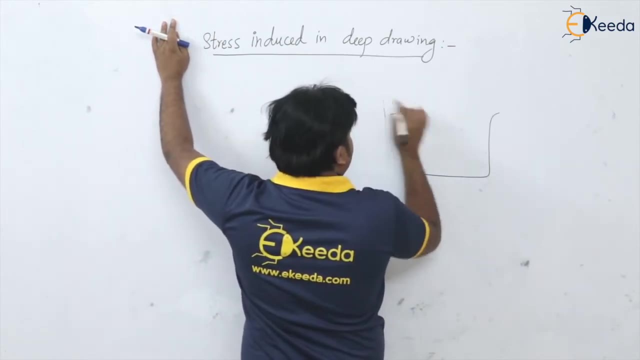 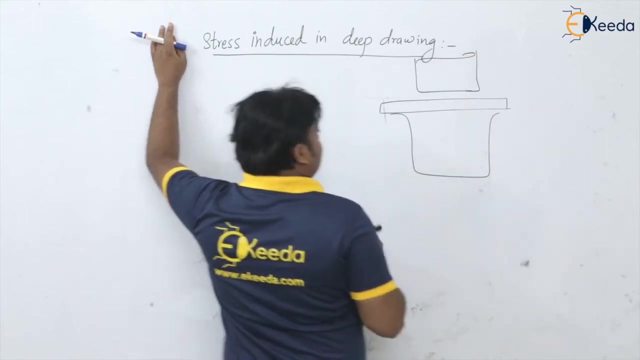 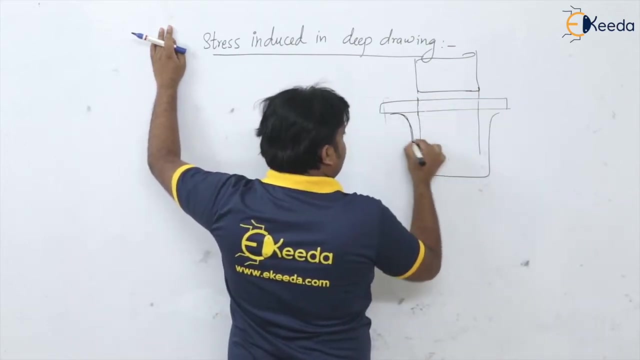 stress is also in every stroke we can able to calculate. okay, so let us say we are having our cup is forming here by the force from this punch, and you know that in the deep drawing operation how much the clearance between the punch and die, it is equal to what? the thickness? okay, it is equal to thickness of 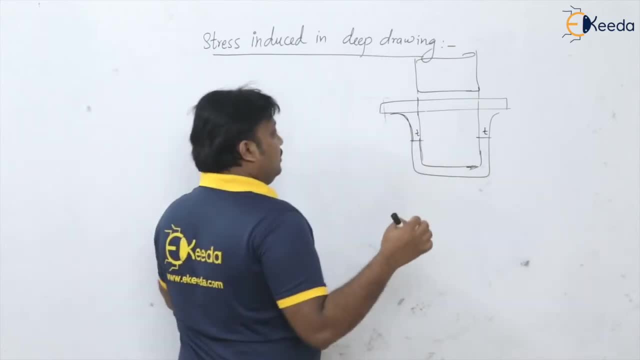 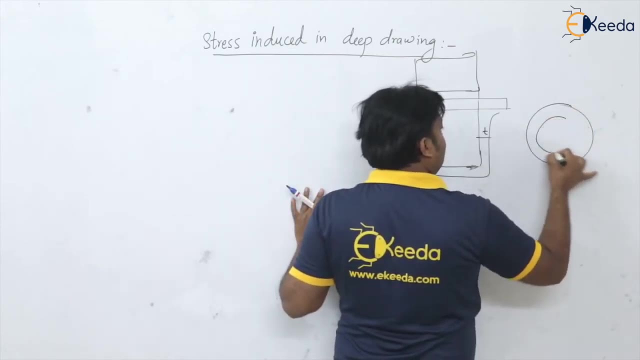 the sheet. this is nothing but the clearance. okay, so once you, if you see from the top, if you see from the top here, so how it will look like, if this is the punch diameter, isn't it say: this is outer diameter? that is nothing but including the thickness. so 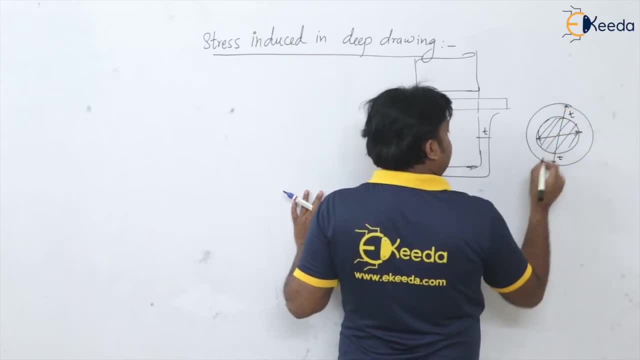 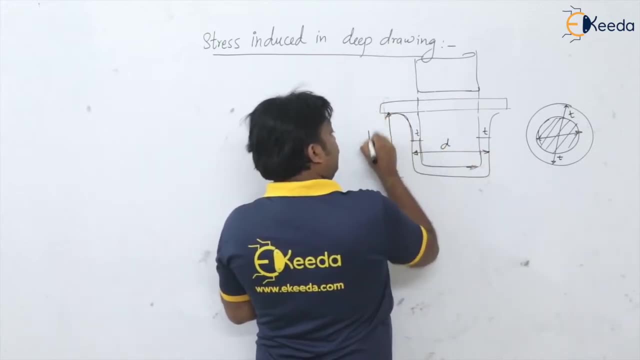 here is thickness T. here is thickness T. okay, if D is, we are taking D like this only so. D is the diameter and this is the height of the curve that is going to produce in this die. so tell me this distance. inner diameter will be this D. 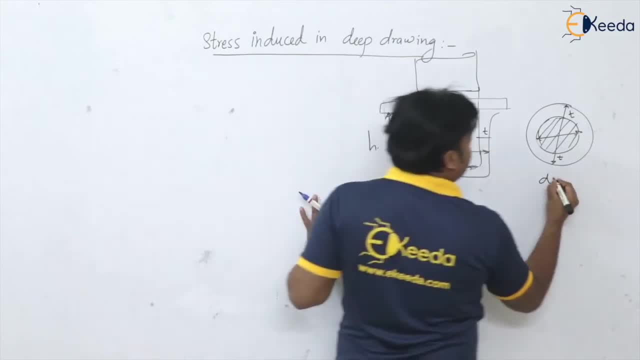 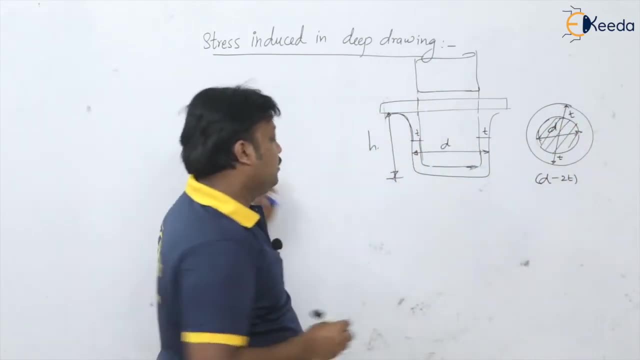 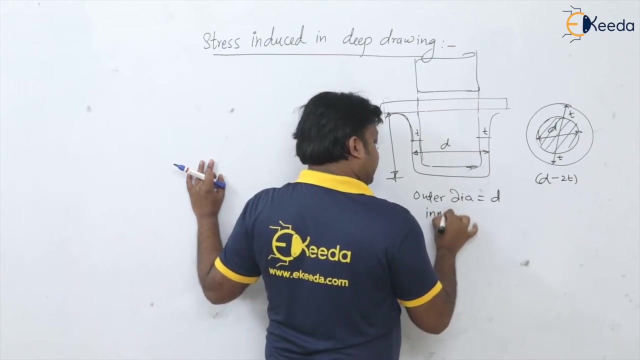 total D may say: yeah, I said T, guy on city God, a minus 2 T, isn't it. and outer diameter is D, you know that? okay, so outer diameter here is equal to capital small d, and inner diameter will be D minus 2 D. okay, now, if you want to. 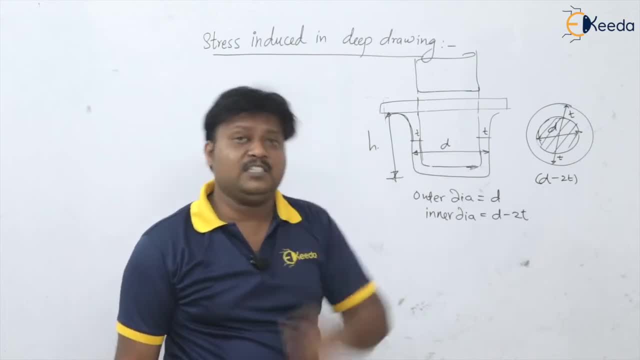 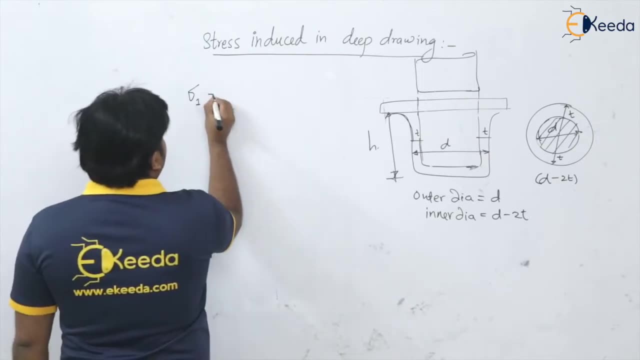 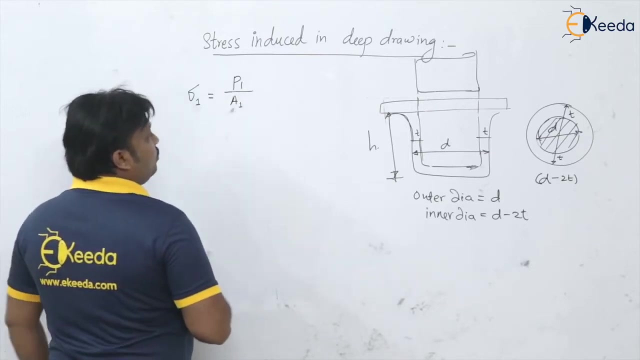 produce. if you want to find out this trace induces in the first pass or first stage. so say, singlet 1 is the stress induced in the first stage. so Sigma is equal to what P 1 divided by the area in the first stage, isn't it? so P 1? we know how to calculate. 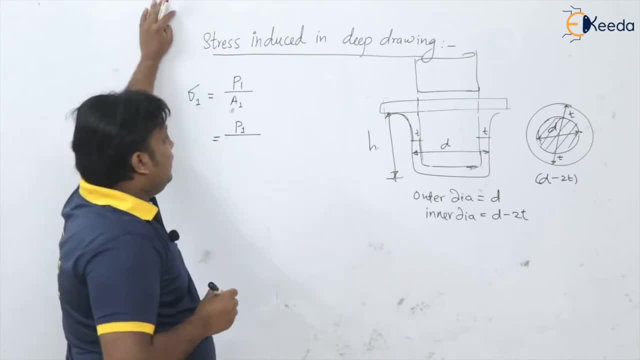 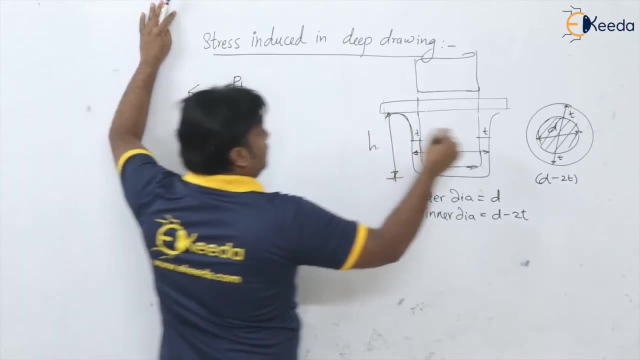 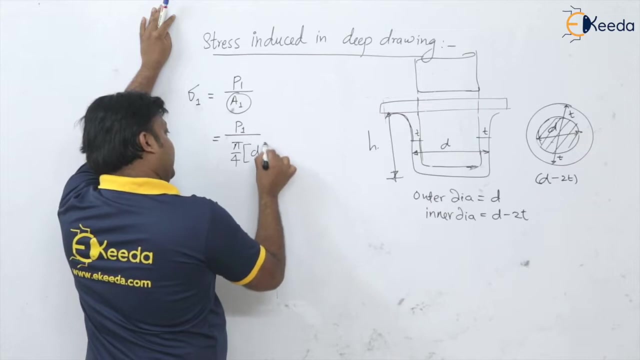 pi D P into Sigma Y, isn't it? that is, Sigma 1 is equal to P 1 divided by what is the area, which area you are getting here? that is, pi by 4 D 1 square, because we are talking about the first stage minus inside area, this D 1 minus 2 T. 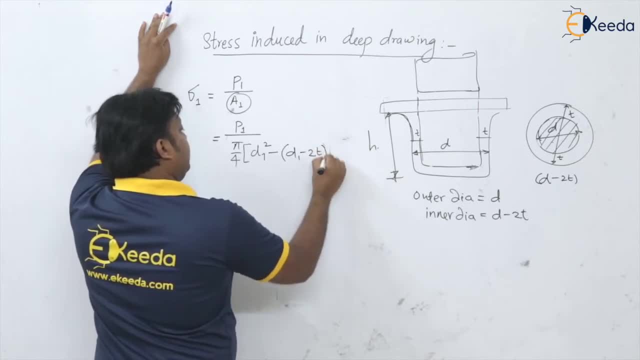 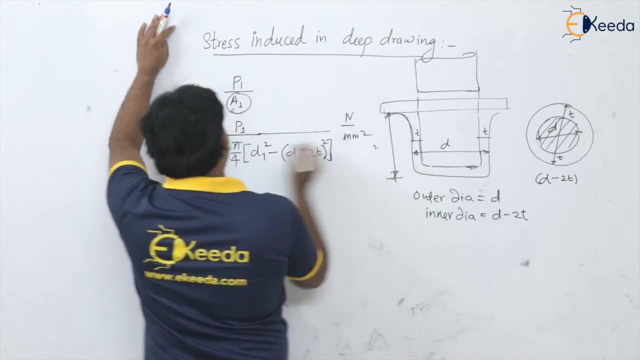 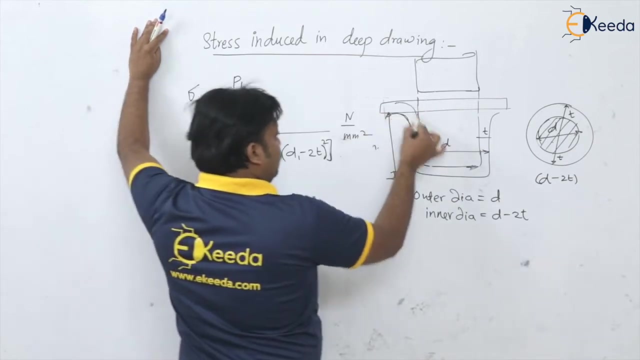 whole square. sorry, D 1 minus 2 T whole square. so you get this stress in Newton per mm square for the first case, isn't it? and one very important thing is that when the deformation is going to happen, when this Sigma one is greater than the yield strength of the material and of 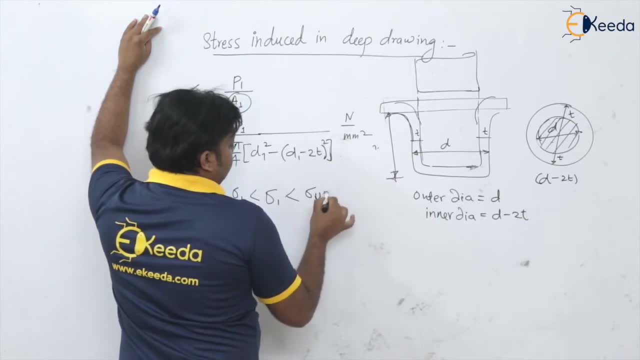 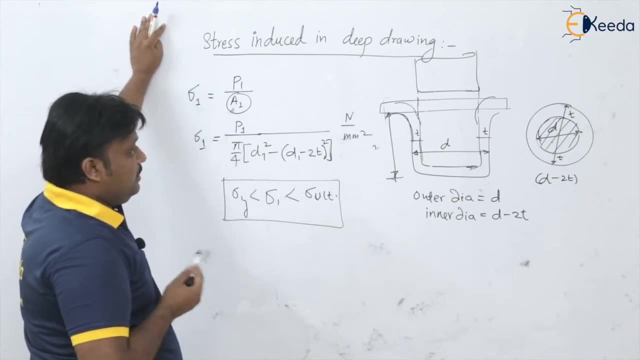 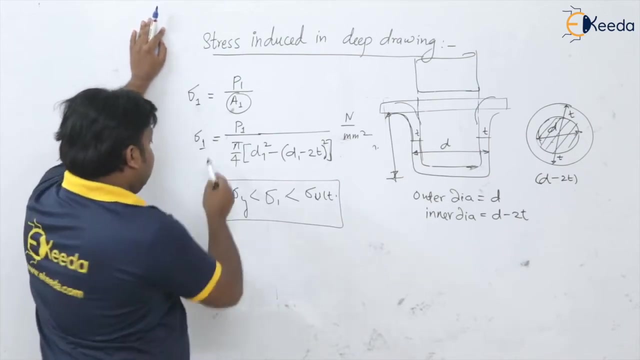 course less than the ultimate strength of the material. please remember, you know this because deep drawing is the deformation process. there, a default. because of deformation the size and shape is going to object, isn't it so? like that you can have the Sigma one plus P 1 divided by d Y and P 1 divided by sigma one plus sigma one. 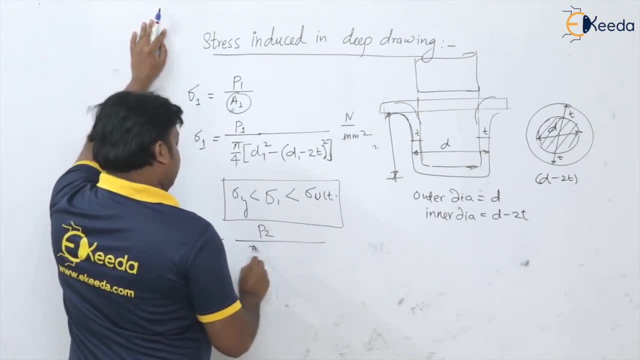 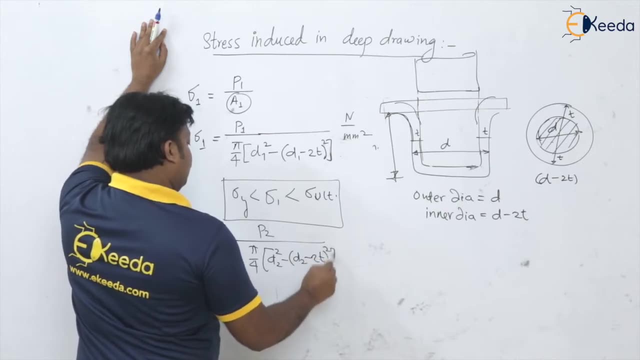 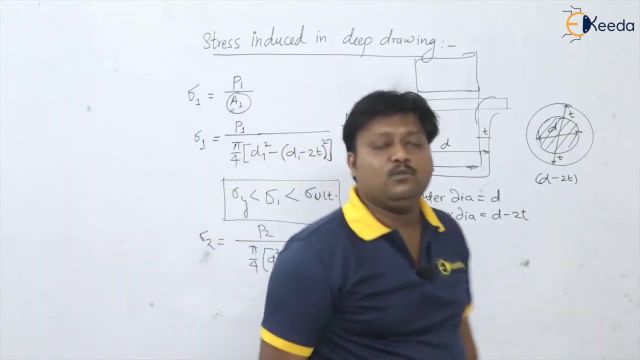 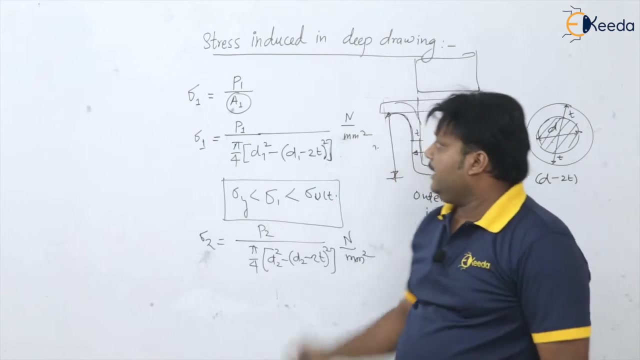 2. now this is p2 divided by pi, by 4, into d2 square minus d2 minus 2t, whole square. like that you will get again the stress in the second stage. like that you can go on calculating the stress in the respective stage or stroke very easily. okay, so this is the stress calculation, or induced. 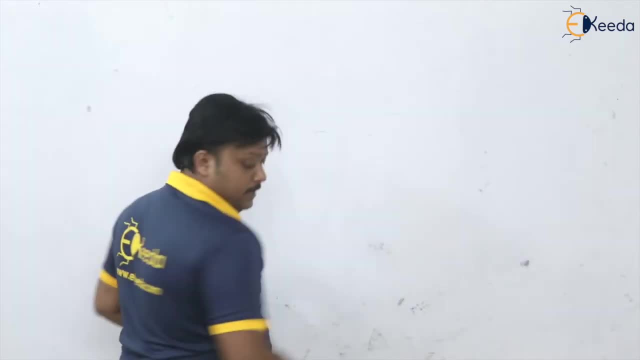 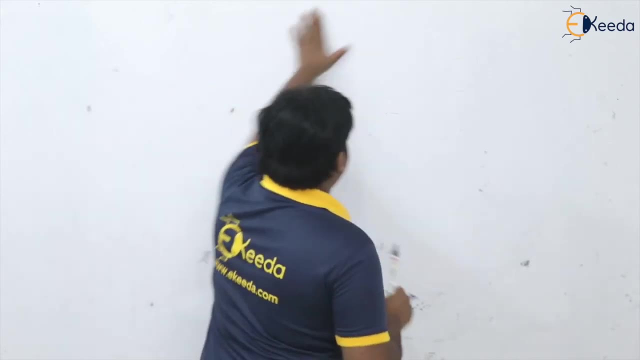 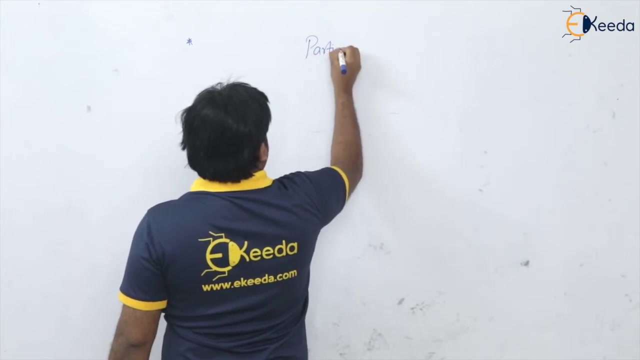 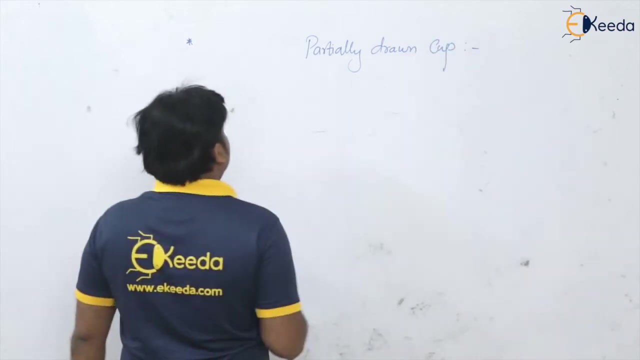 stress calculation in the deep drawing operation. okay, now in this stress analysis. okay, what i'm going to have here, suppose we have the partially drawn cup. okay, we have the partially drawn cup. partially drawn, partially drawn means process, okay, and i want to have, or i want the stresses. 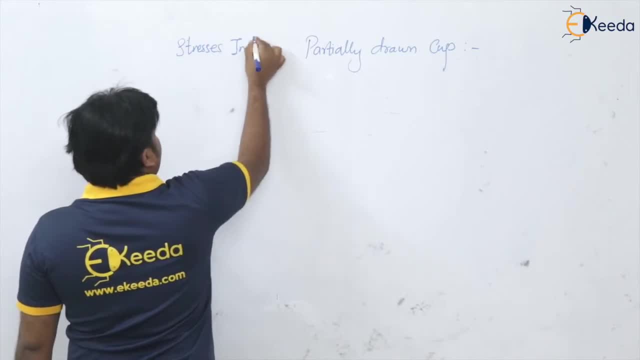 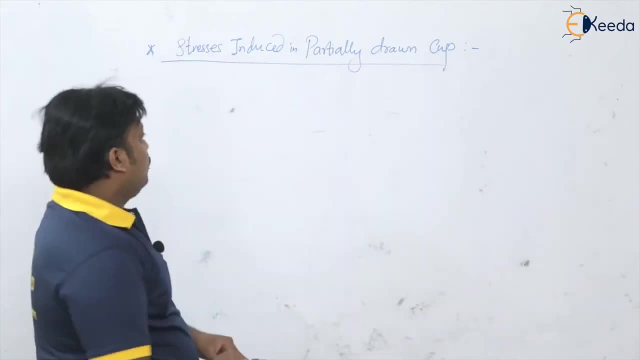 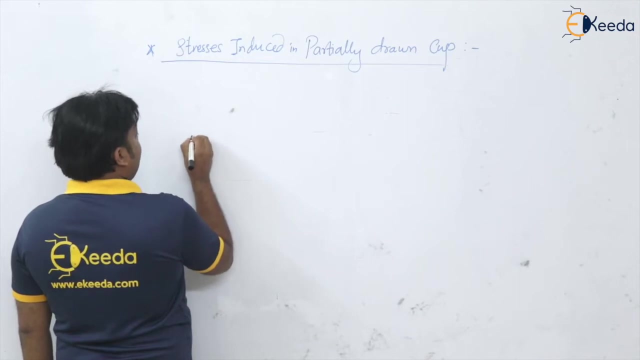 stresses induced in a partially drawn cup. okay, so let us see this. for that, what i have to draw here, the partially drawn cup, okay, we will draw it say: this is the die and this is the flange portion on which our blank is rested. now, and it is partially. that's why i will show. 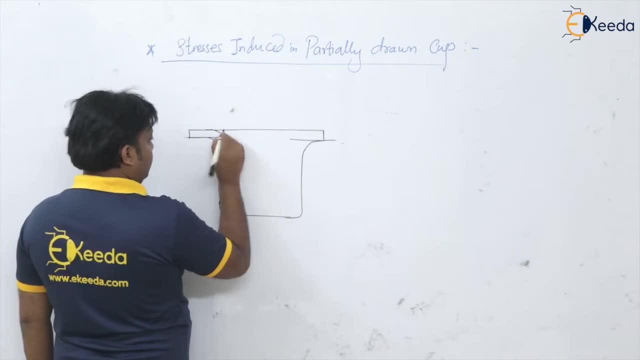 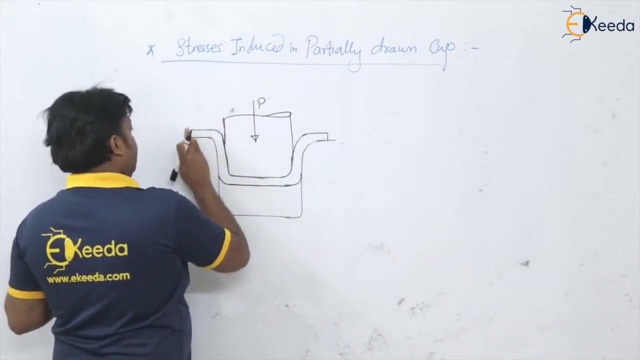 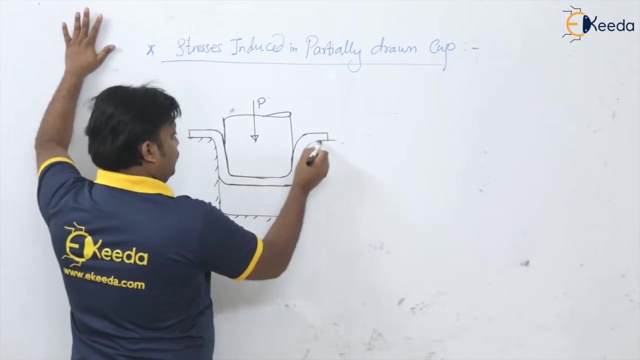 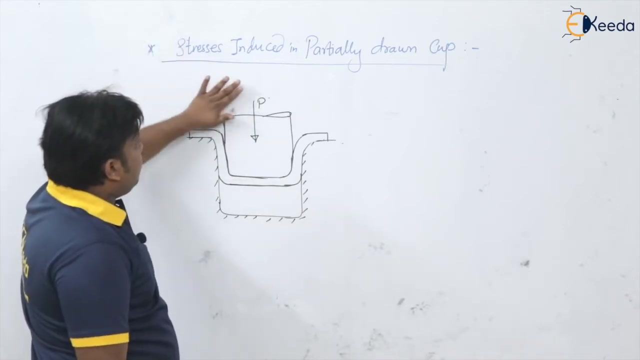 like this: that operation is in process and it is applying force p. okay, so i hope it is clear now. this is the die. okay, in that die, the process is progressing. now let me show you. let me show you what someone has already done. found that one guys for making a cup from a given blank. okay, so this is a partially drawn 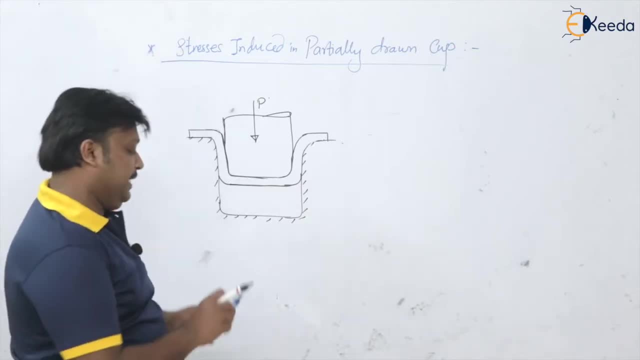 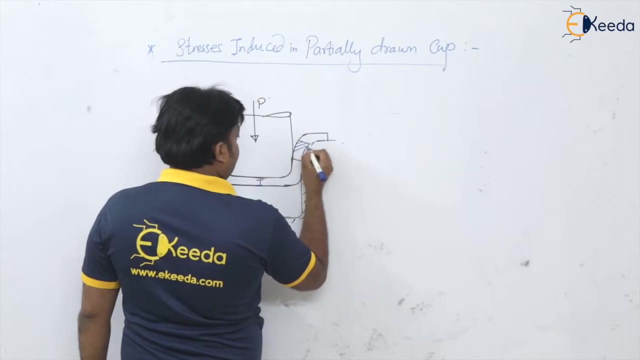 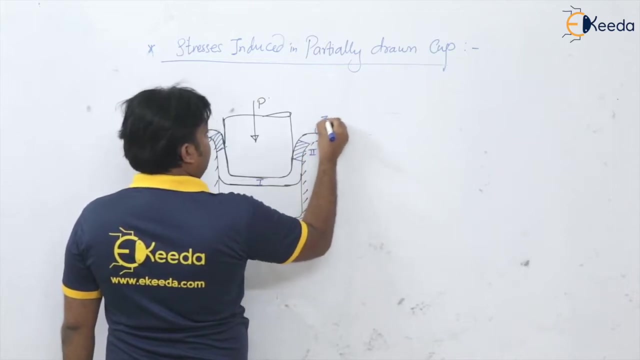 cup, isn't it? so here we are having the three zones. okay, so this is zone number oneki for deformation. actually say this is zone number two and the flow flange portion is as say, this is second zone 2: provocation here there is a second zone for this. check out my chart. check out my chart here. look at it. the incoming zone will be long, so it will be difficulty and small. 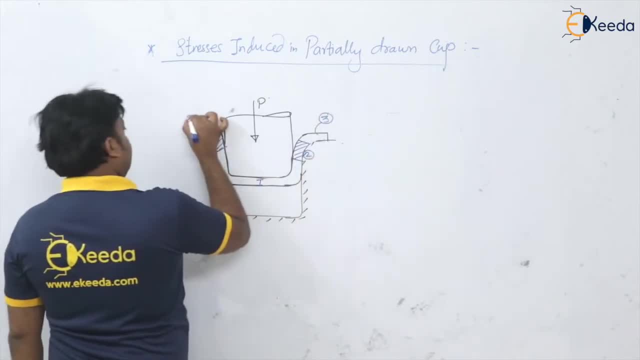 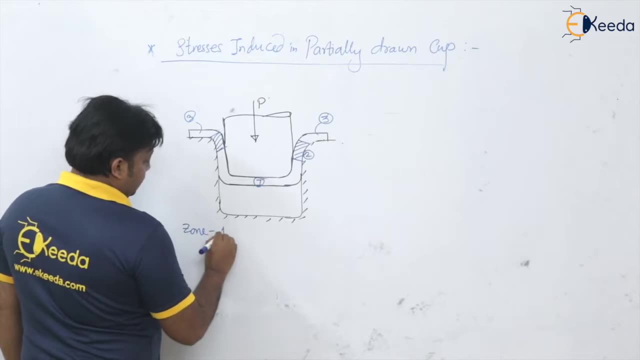 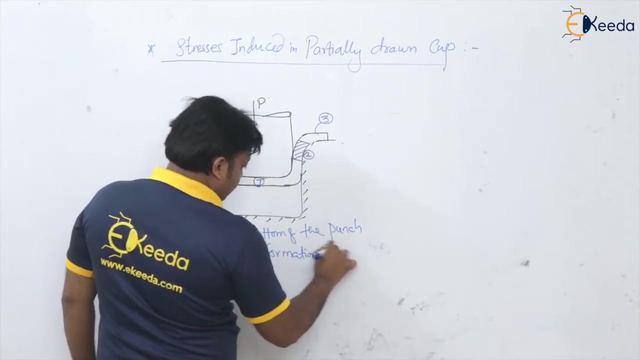 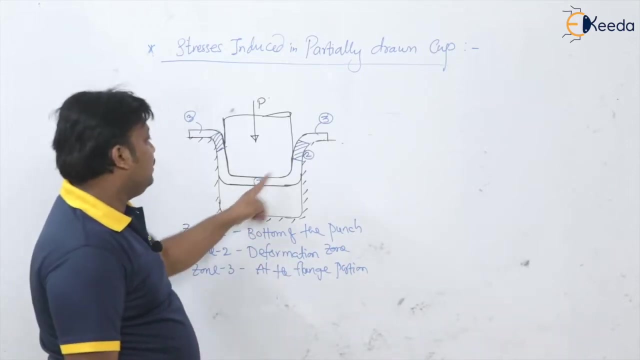 Say this is second zone and this is the third zone. Okay, So first zone, I will write: zone number one, That is bottom of the punch, Bottom of the punch. Zone. number two, That is the deformation zone, Deformation zone. and zone three, at the flange portion, The flange portion. So what we are going to see is that the stresses induced in these three zones in the partially drawn curve, Okay, 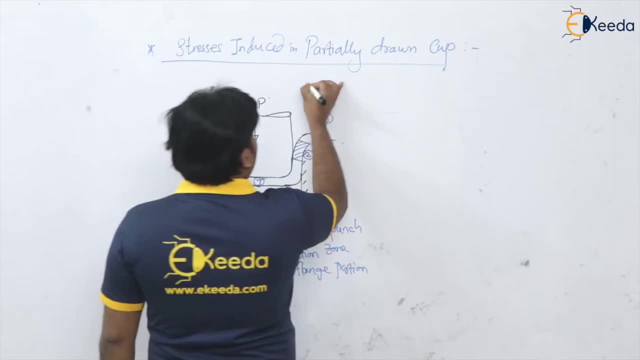 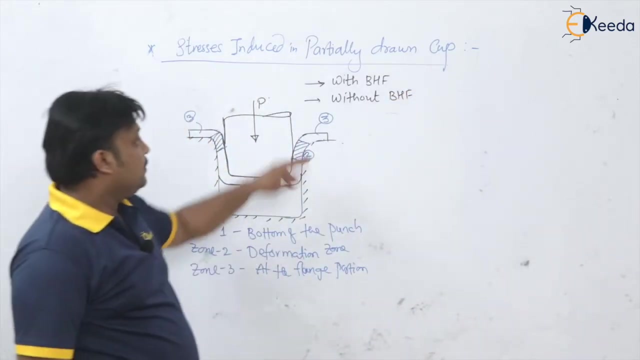 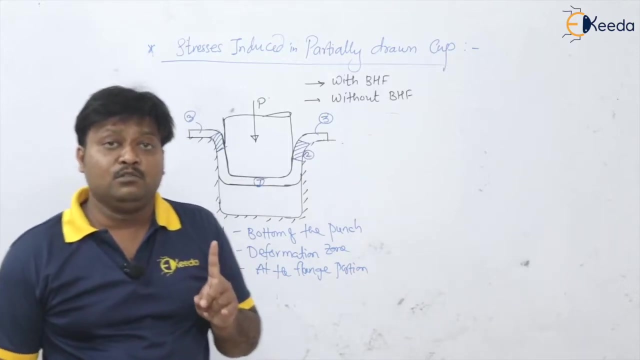 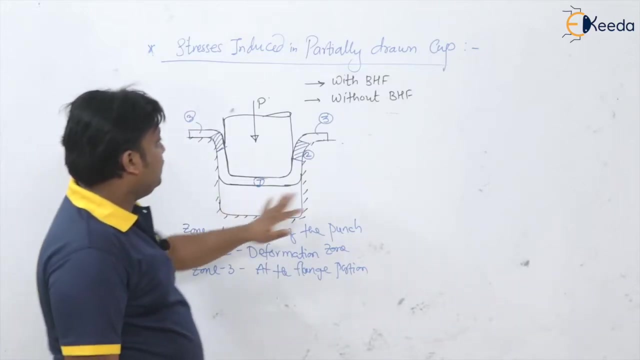 And, very importantly, by considering this, By considering the two conditions or cases. One is with BHF and without BHF. Second is without BHF. So this is the condition. Okay, So for these two conditions, we are going to see in each zone what kind of stresses are going to induce in the partially drawn curve. Okay, Very important. Many times this question are framed on this topic. 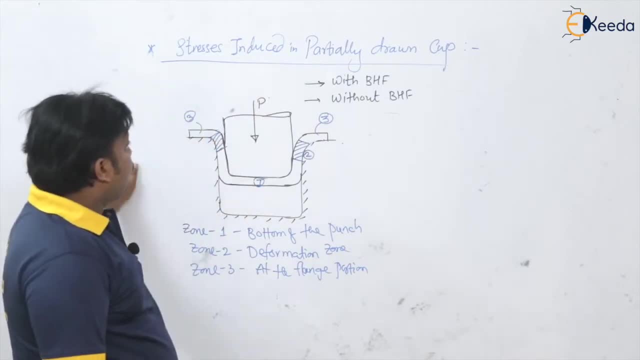 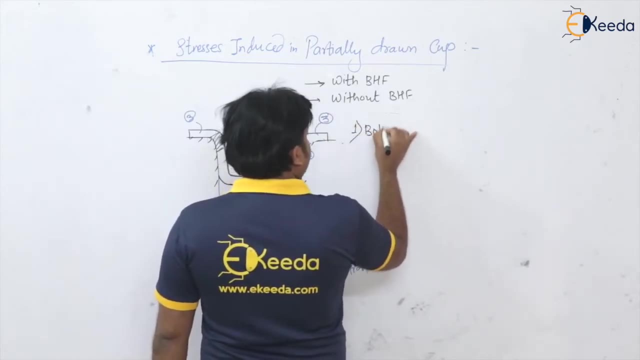 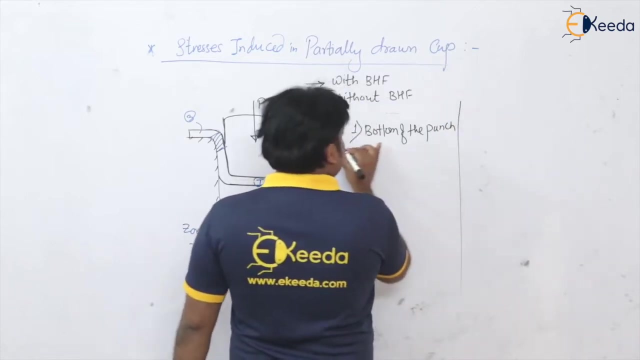 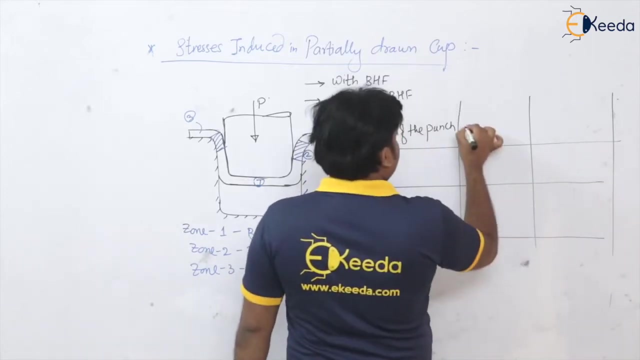 Subtopic: stresses induced in partially drawn curve. So see here, Let us see, we have the first zone, Bottom of the punch, Bottom of the punch. So tell me which kind of stresses are going to induce. Say here, with BHF and without BHF. 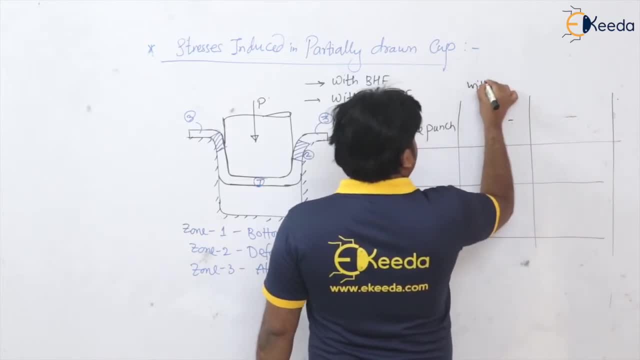 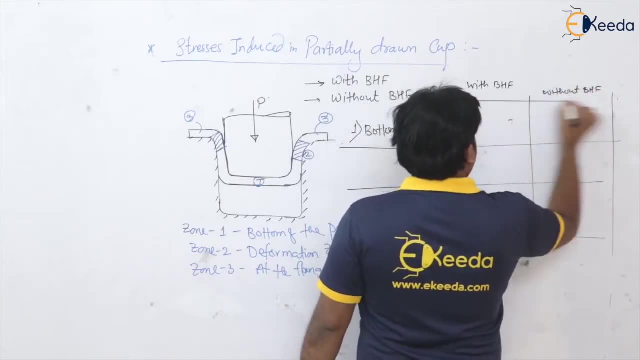 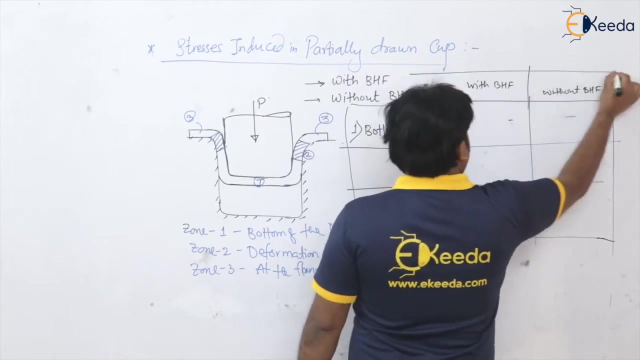 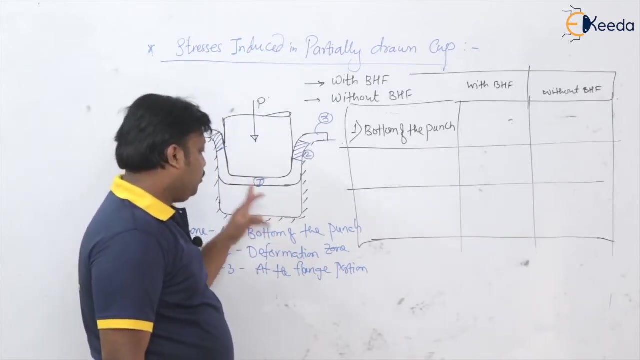 With the BHF and without BHF. Okay, So that we are going to see. Okay, Now see at the bottom of the punch. Okay, At the bottom of the punch Say: if you are not applying any BHF, We are not applying any blank holding force. 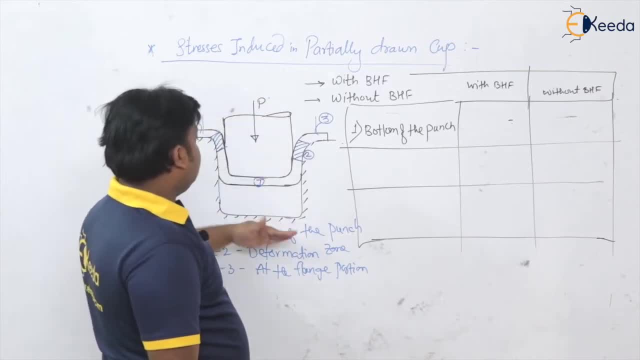 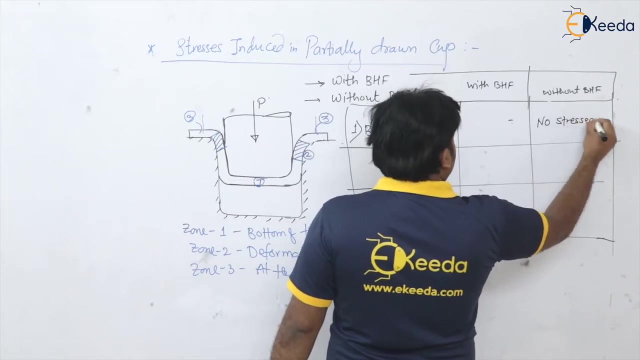 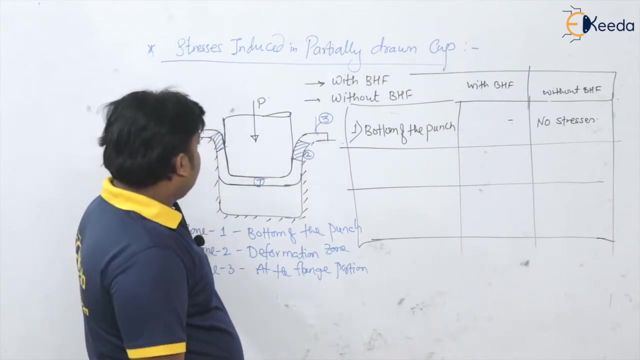 So simply the punch is taking down this sheet into the die. So actually there are no any stresses. So without BHF at the bottom of the punch, No stresses. Okay, Even if you apply the blank holding force on the flange. So even application of this BHF also there will be yes stresses. 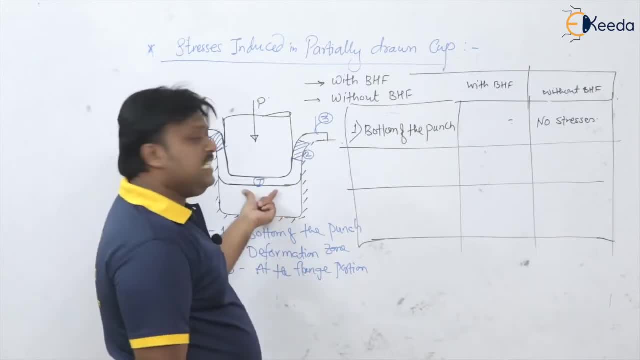 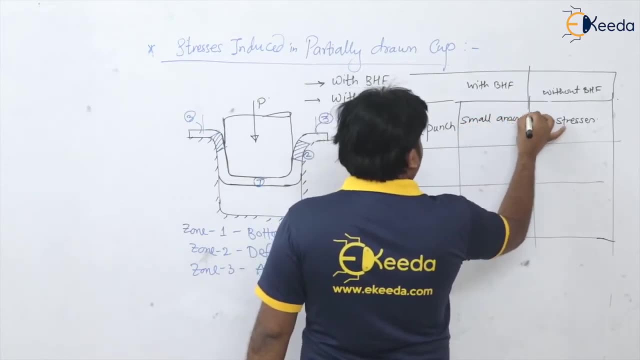 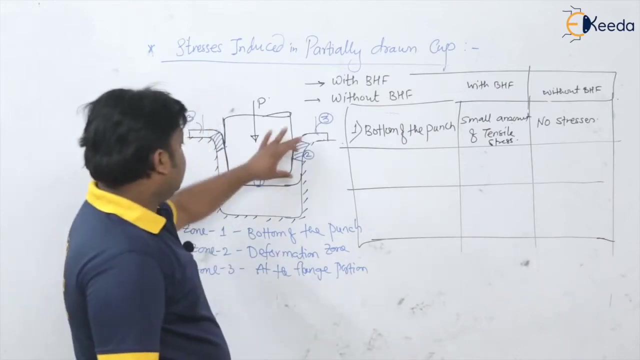 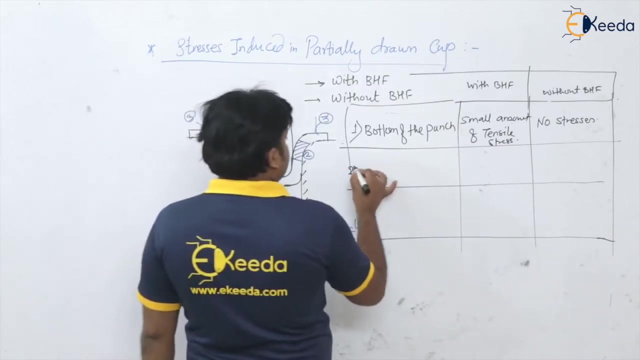 But very little amount of which stress, tensile, or very small amount of this very small amount of tensile stress, only tensile stress. Okay, With the BHF, the little amount of tensile will be at bottom of the punch. So now come to the second zone, that is, the deformation zone. Deformation zone. So here, please remember, 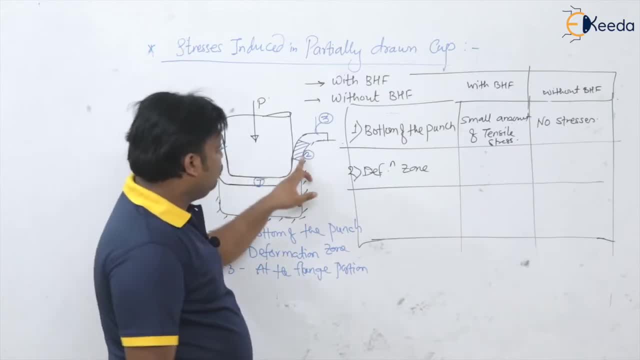 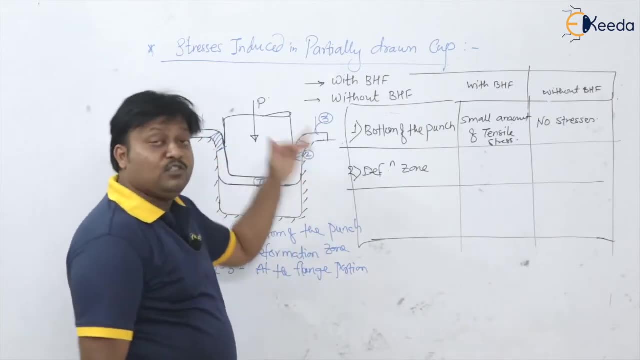 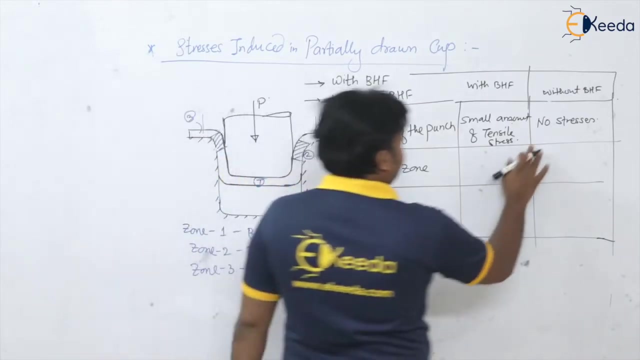 The force induced or the stress induced in this zone is responsible for getting the change in its shape, Isn't it? And it is responsible to have deformation. So definitely So. in this deformation zone, the shape is going to change. That's why, with or without BHF, no issue, What will happen here, Which kind of stress will be there, With or without BHF? 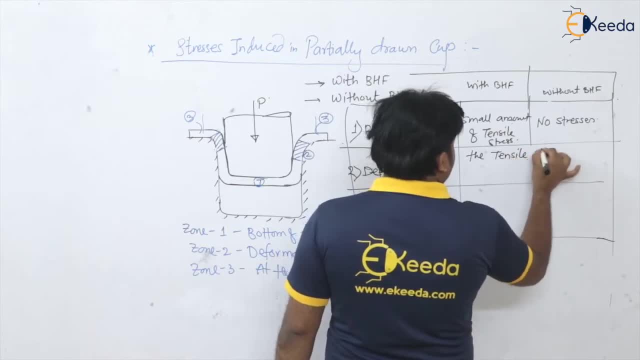 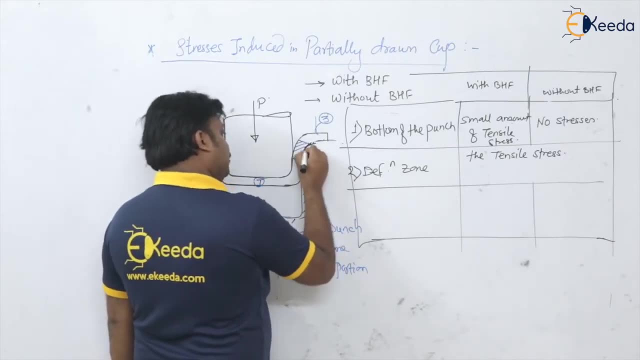 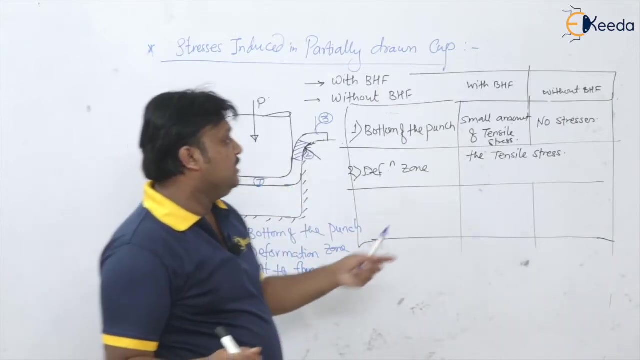 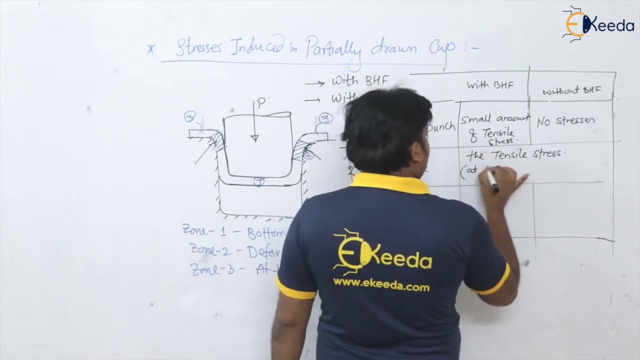 Tensile, The pure tensile, The pure tensile stress only. However, if you look at the corners, if there are these corners, there is a compressive stress, but it is very, very less in amount compared to this pure tensile. That is why we are neglecting. So, at corners, compressive stress is there. 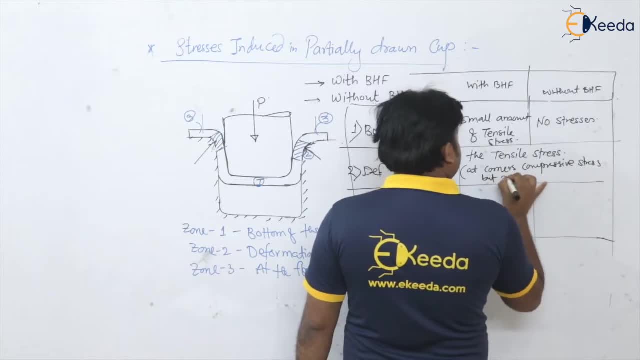 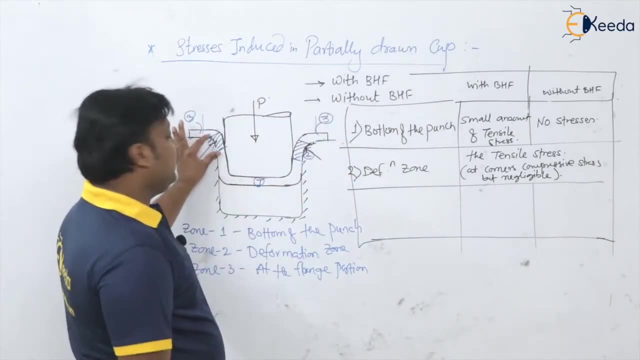 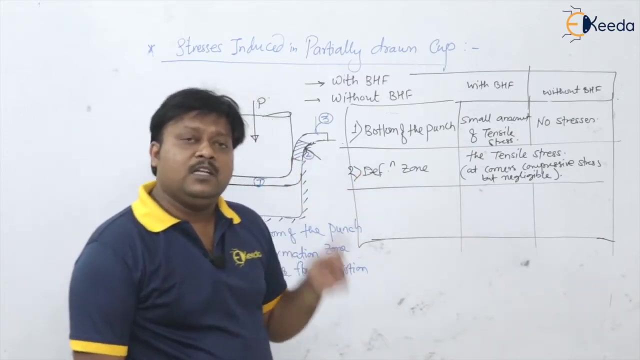 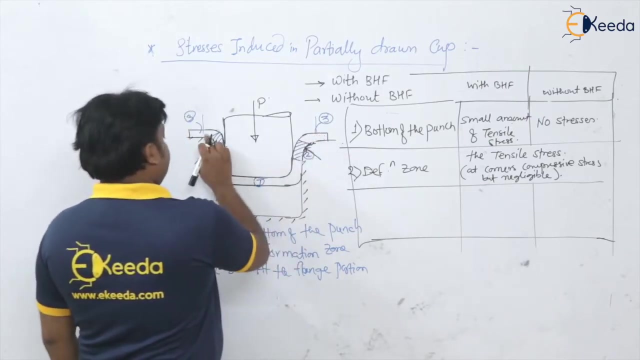 But negligible, Negligible, So that's why I'm neglecting. So pure tensile actually in the deformation zone, Please remember Very important. So second zone, may BHF apply, There will be always. pure tensile is going to produce pure tensile stress. Now come to the flange portion. When you are not having at flange portion, at flange portion, 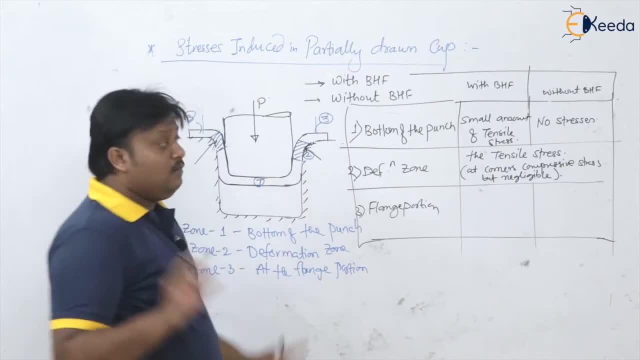 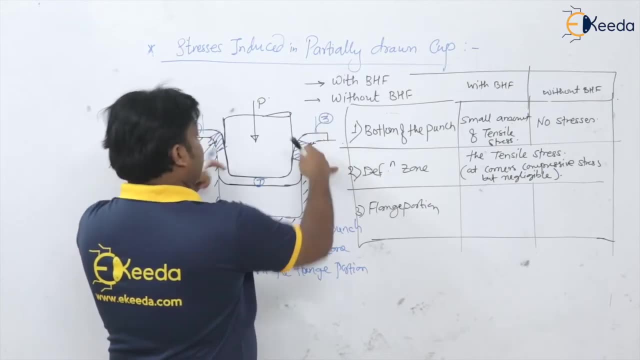 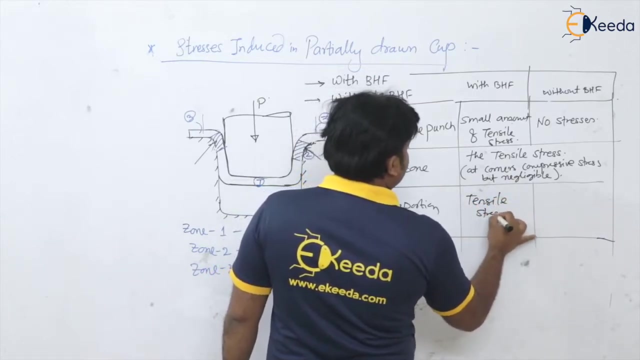 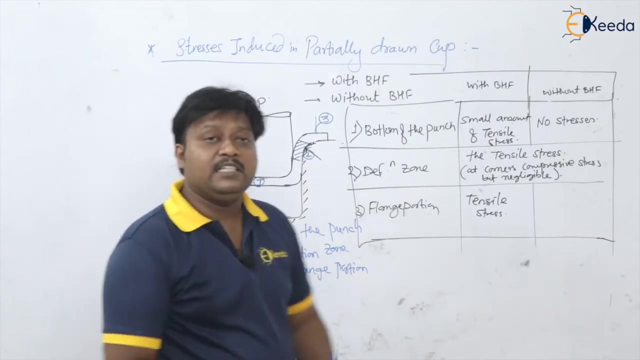 When you are having the BHF, when you are having the BHF, what the material is going to have? deformation, Okay, Because of the tensile stress, Isn't it? So? only tensile with the BHF, tensile stress only, But without BHF. without BHF, what will going to happen? There is a flow of material radially. Okay, There is a flow of material radially. 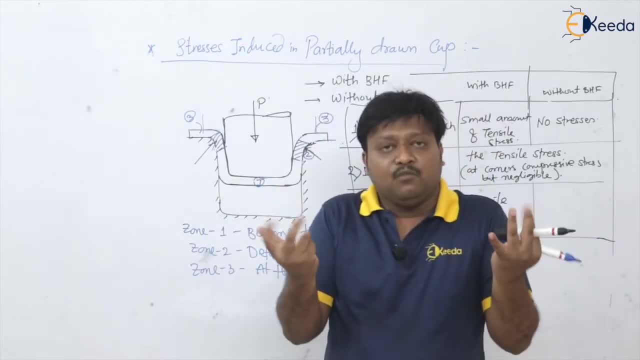 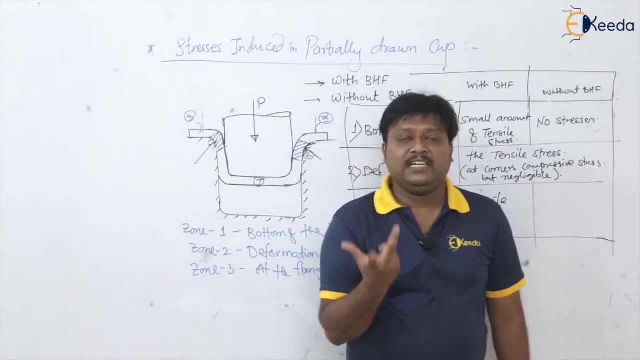 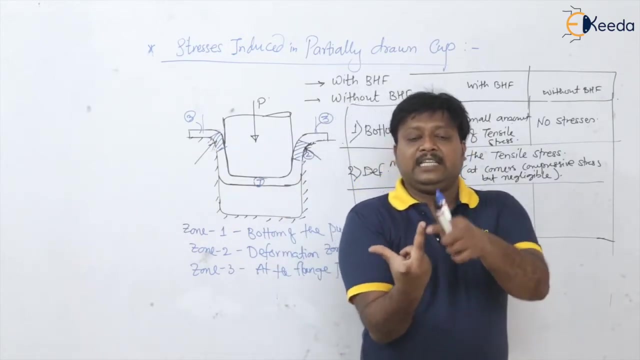 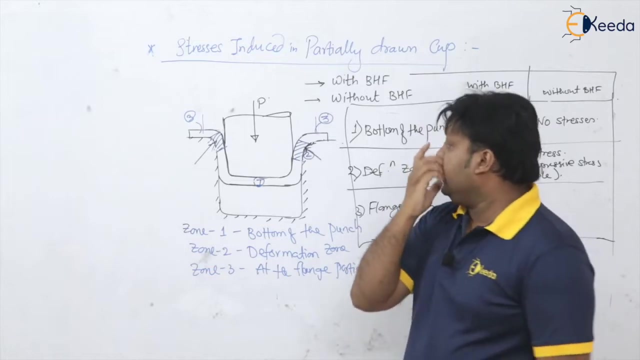 And there are going to produce the foldings, They are going to produce the wrinkles, Isn't it So, if you look there, the kind of stresses that are going to induce at this third zone that is, the flange portion. So these are two directional tensile. These are two directional tensile and compressive in and compressive in third direction. Please remember, So with BHF only. 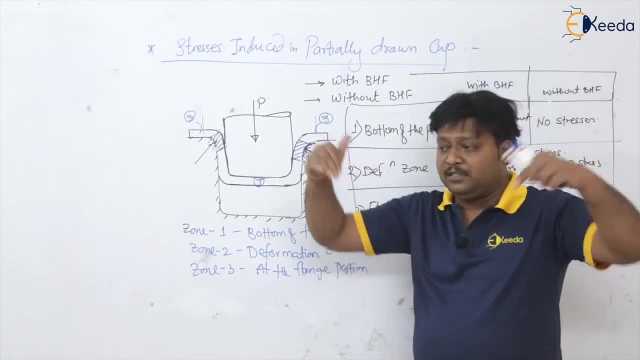 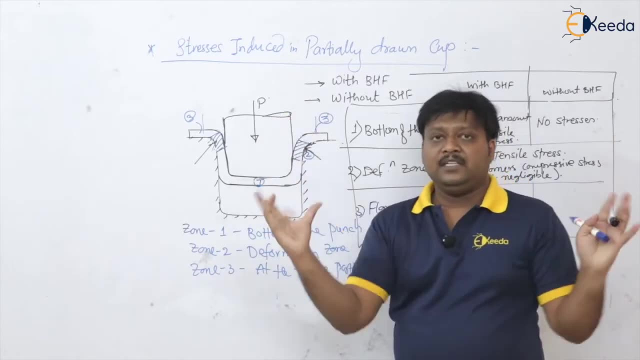 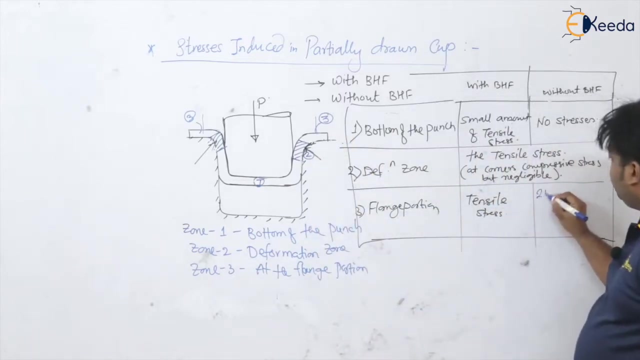 The tensile stresses are going to generate in the flange portion, at what is flowing inside the die. But if you are not using any BHF it will be simply lifted. It will be simply lifted at was two directional tensile and compressive. in third directional, two directional, two directional tensile stress and compressive. 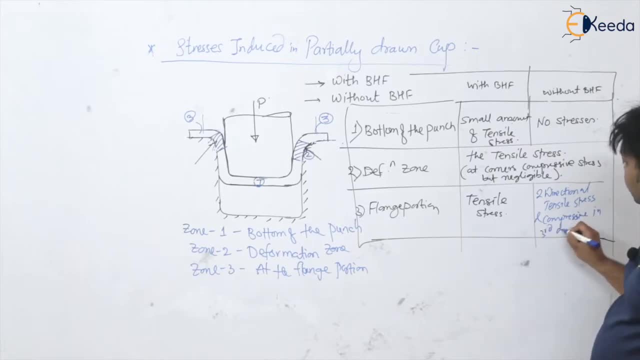 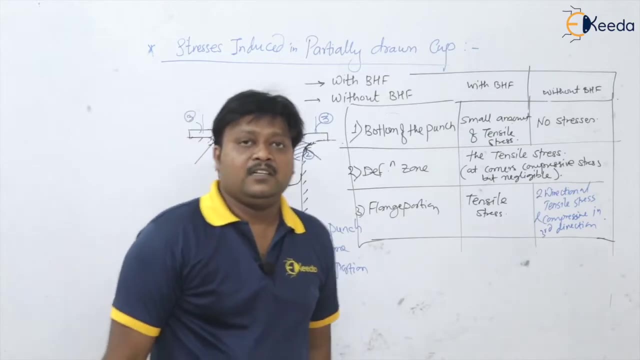 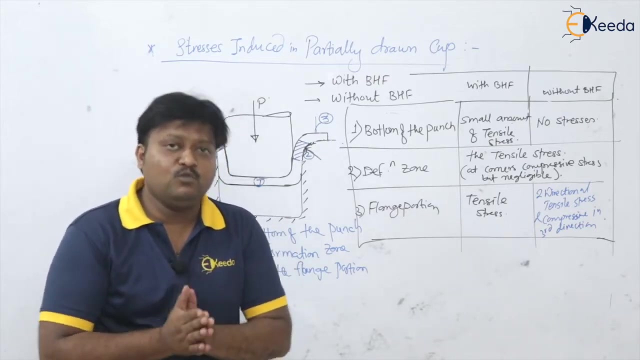 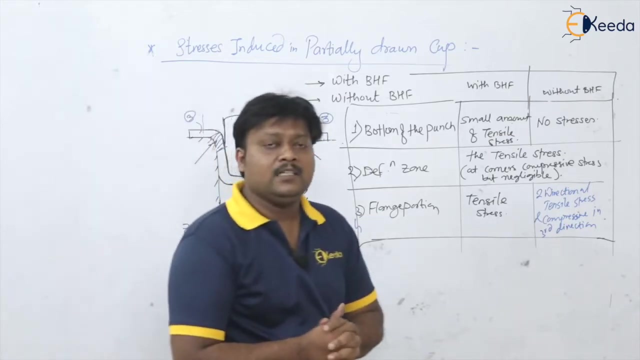 Compressive in third direction. third direction, So these are the stresses, kinds of stresses which are going to produce in the partially deep drummed cup, in various zones, For example, bottom of the point, in the deformation zone and in the flange portion. Okay, So this is about the stresses. Now, in this video we are going to see, 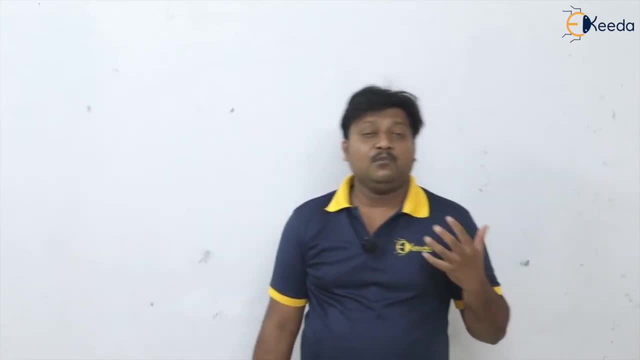 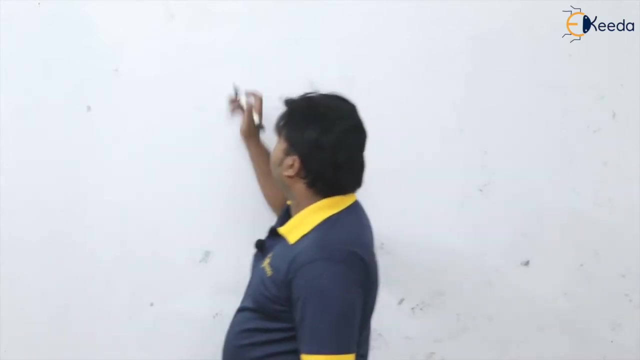 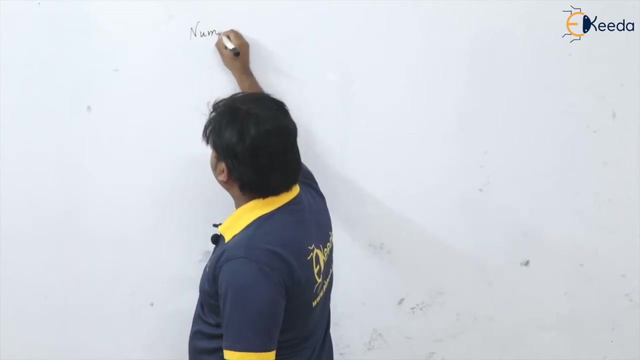 The number of draws, Okay, The number of passes, The calculation for this. So many times I use this word: the pass draw, blow stroke. Okay, The reader draws. Okay, So how to calculate this, actually? So let us see the number of draws. Number of draws. 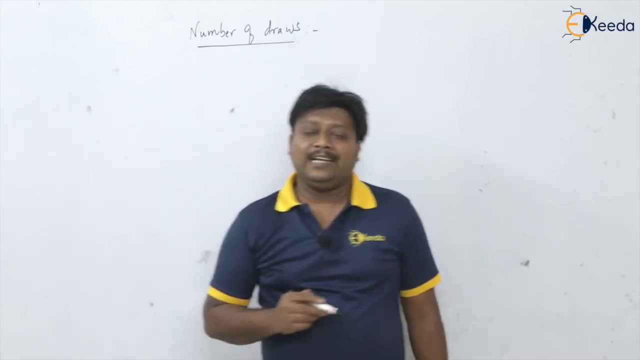 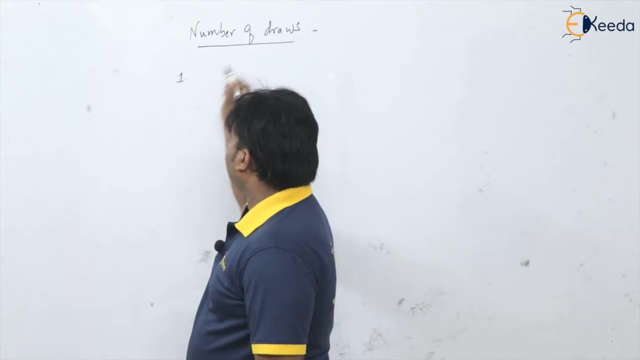 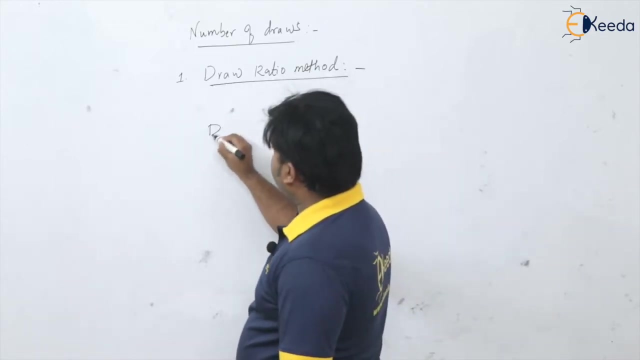 In deep drawing operation. So for calculating this number of draws, there are two techniques. So technique number one or method number one we can have, That is draw ratio method. Draw ratio method, Very easy. What is draw ratio method? So this draw ratio? This draw ratio is equal to the diameter. 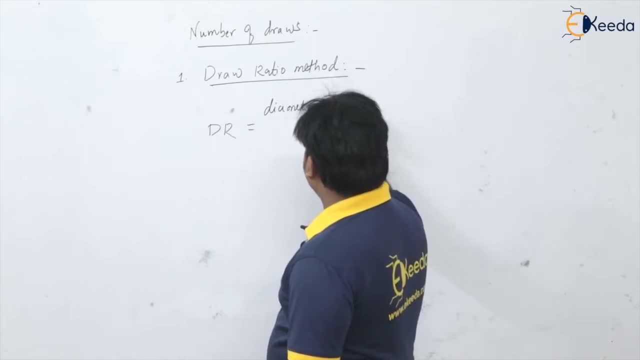 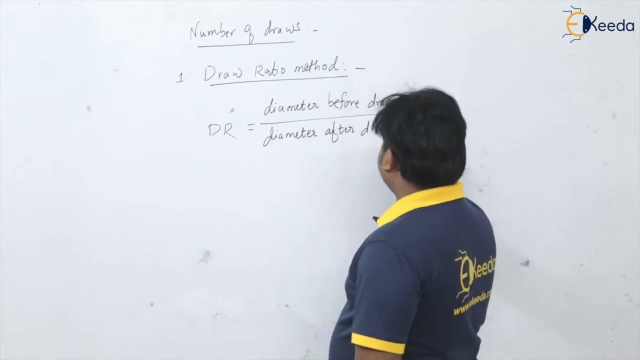 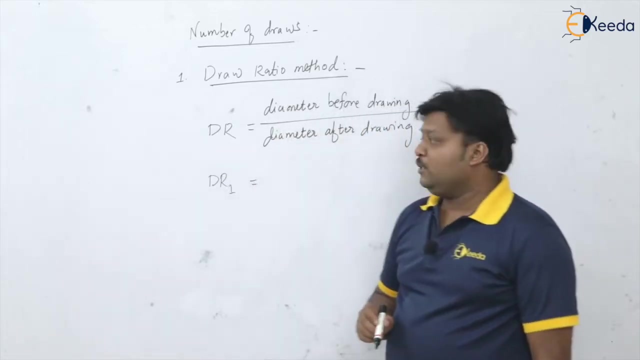 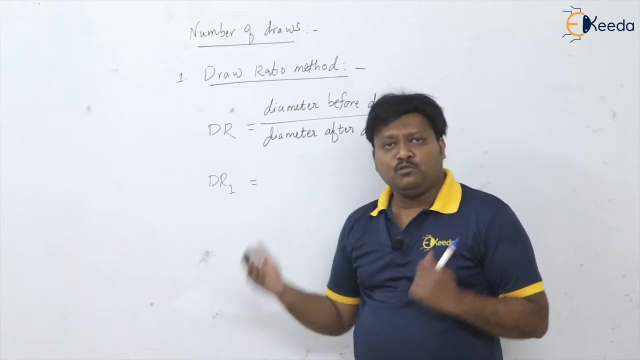 Before drawing: before drawing divided by diameter after drawing. diameter after drawing: Okay, So let us say, if I want the draw ratio one. So for that, when we are today, We are starting the operation App declare, consider my blank. using that blank, we are going to produce the cup. okay, so we are having before operation or before 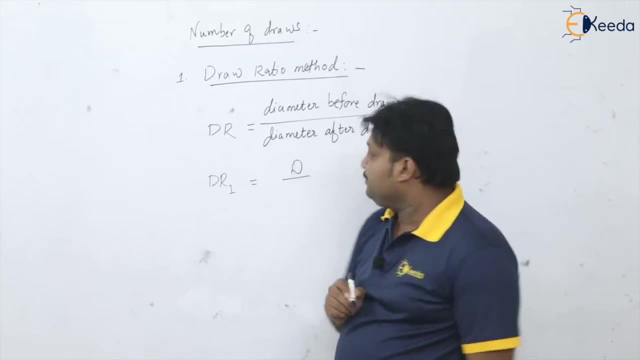 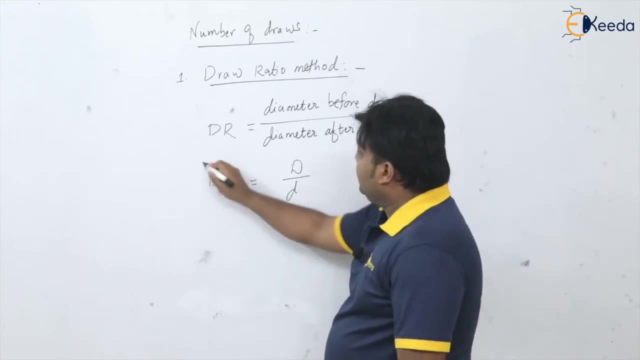 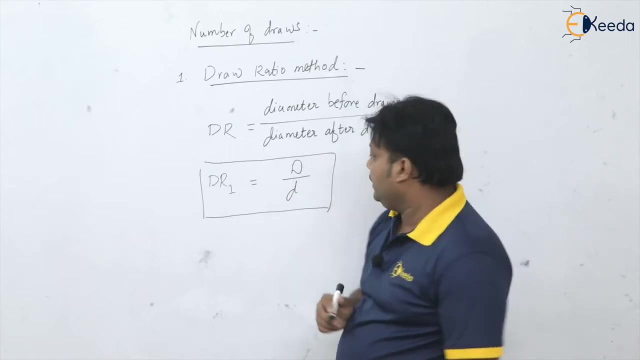 drawing: capnipass capital. d is the blank diameter divided by after drawing camel name i like cup diameter, isn't it so simply the ratio of diameter before drawing divided by diameter after drawing. so definitely, here d will be replaced by d1 because this is the first draw. okay now. 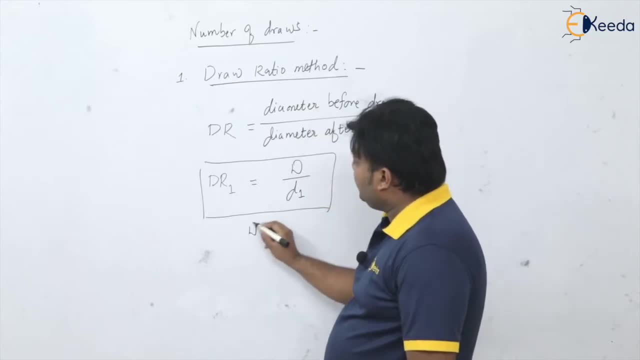 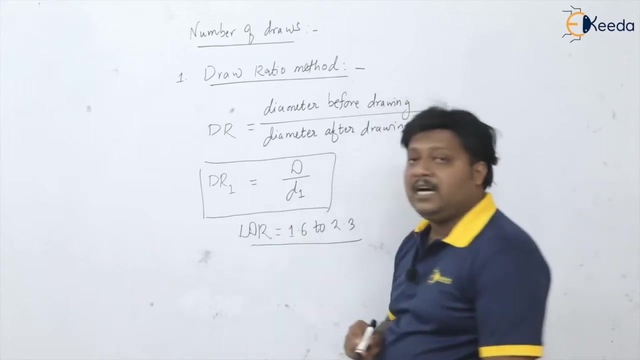 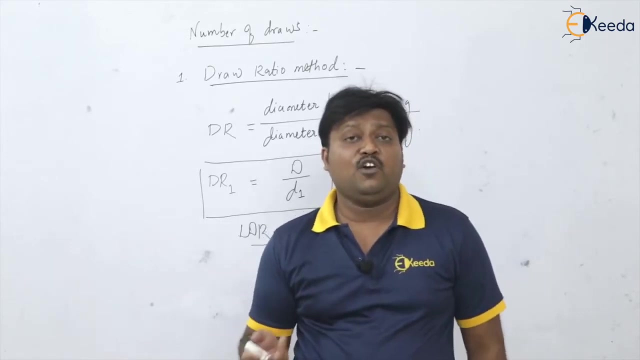 this draw ratio actually ranging from 1.6 to 2.3, please remember. okay, so these are the limiting draw ratios. these are what ldr, that is, limiting draw ratio 1.6 to 2.3. okay, if in the question they are asking for the calculation of number of draws and they have not mentioned anything about. 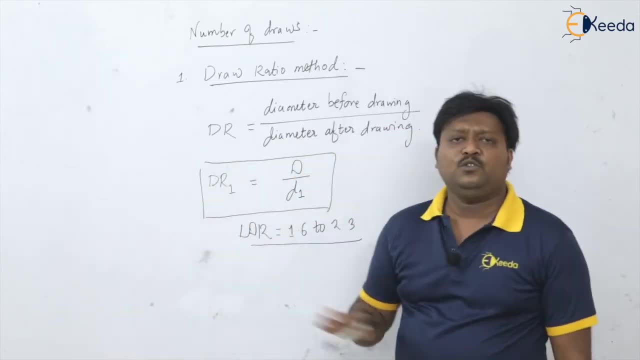 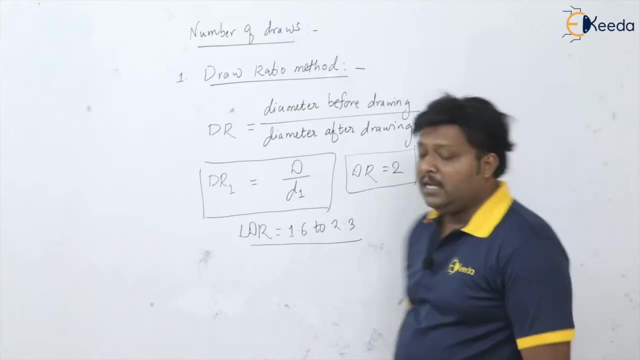 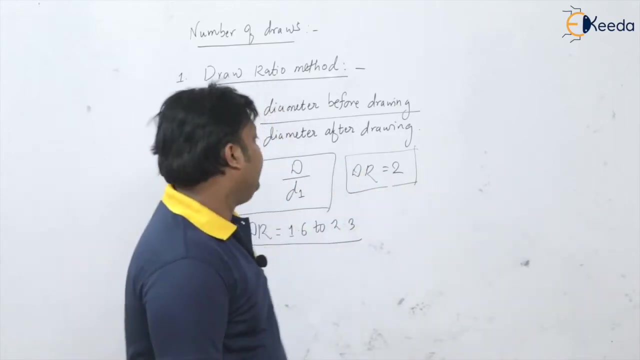 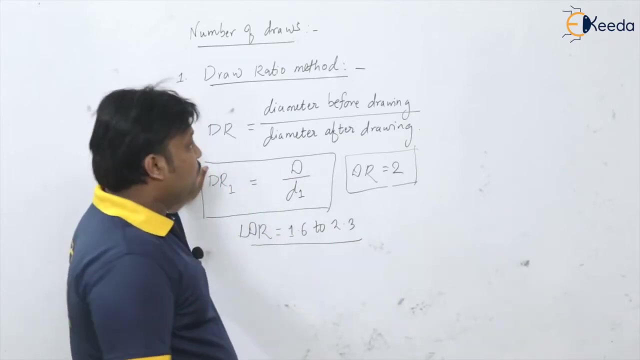 the this draw ratio or limiting draw ratio. you just simply consider that draw ratio is equal to 2. please remember this very important: whenever no, any data given for this draw ratio, you can take it as 2. okay, so, like that, you are go on calculating the number of draws to get the required size of cup. okay, say the diameter. 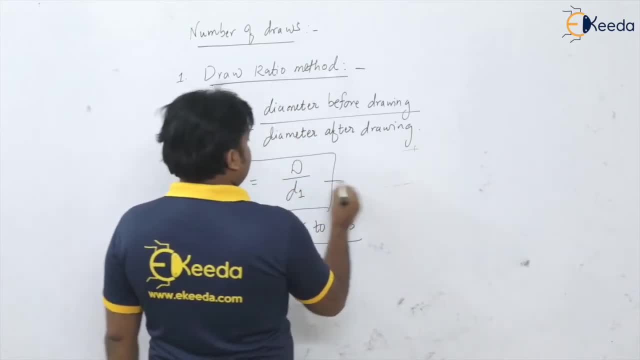 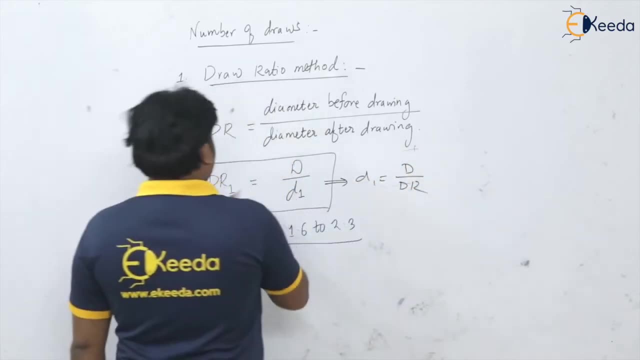 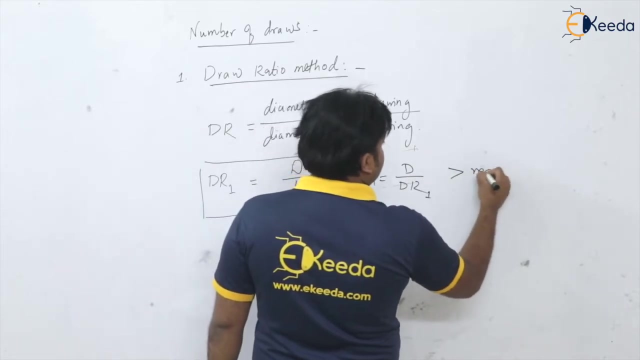 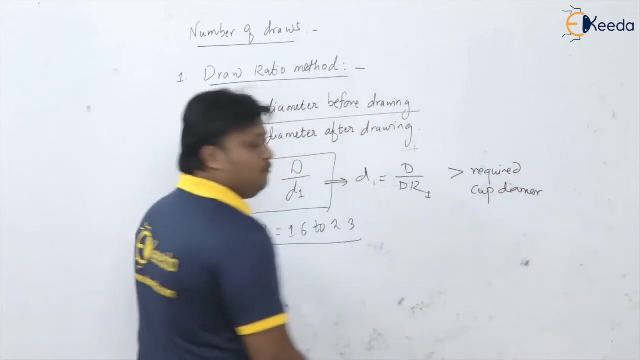 you get from this first draw, that is, d1 is equal to d by draw ratio, isn't it okay? so, draw ratio 1, but still it is greater than the required diameter, required cup diameter, isn't it required cup diameter? so, again, what you will do, you will go for the next draw, you will go for subsequent draw then. 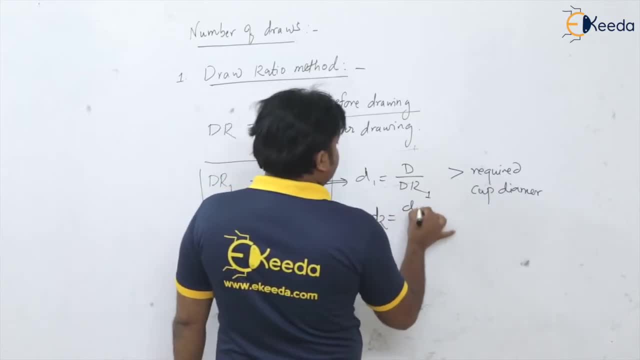 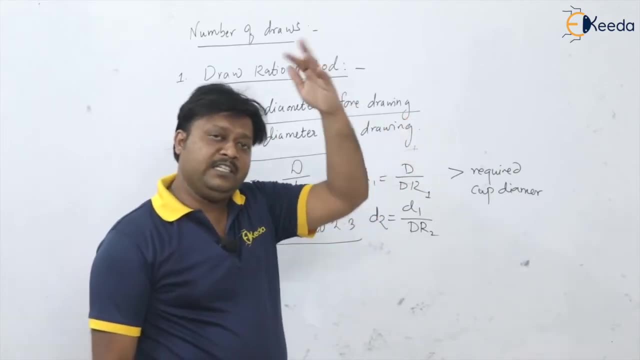 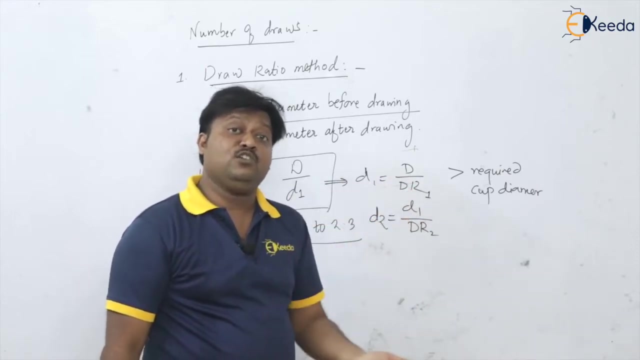 you will get this. d2 is equal to say d1 divided by the draw ratio. if same draw ratio we are going to use in the every stage, then this dr will be same for every, everywhere. if again you are changing the draw ratios also in particular stages. 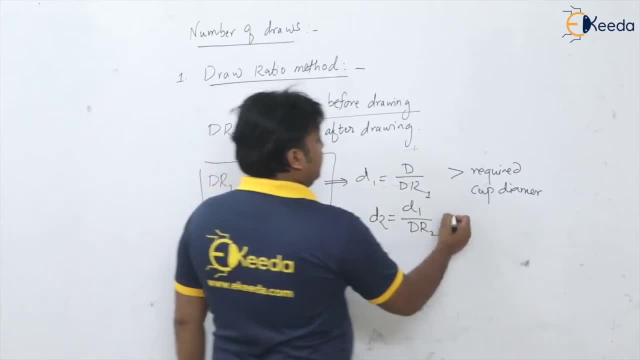 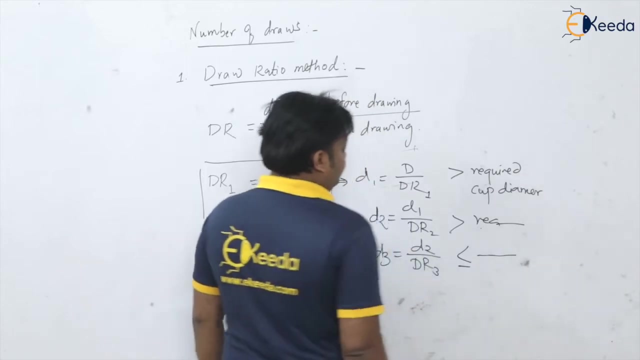 then you can have this dr2 here again. if this is greater than the required diameter, you again go for the third draw. okay, that is d2 divided by draw ratio at the third stage, and once it is less than equal to the required, you will going to stop there and there will be. 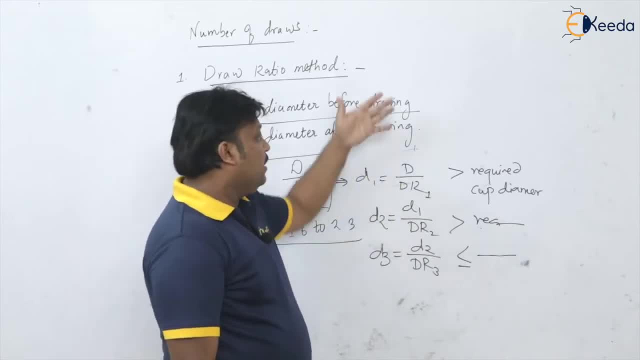 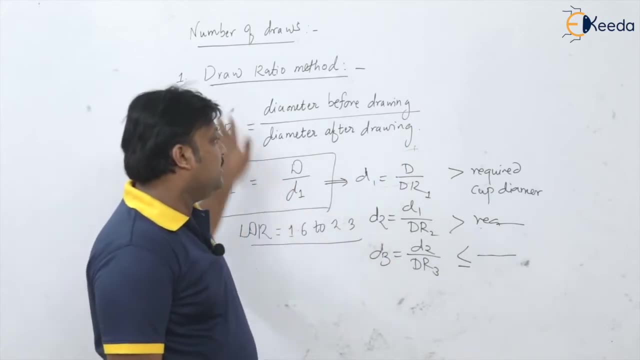 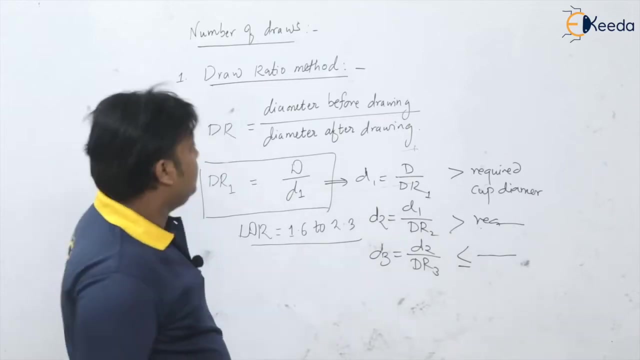 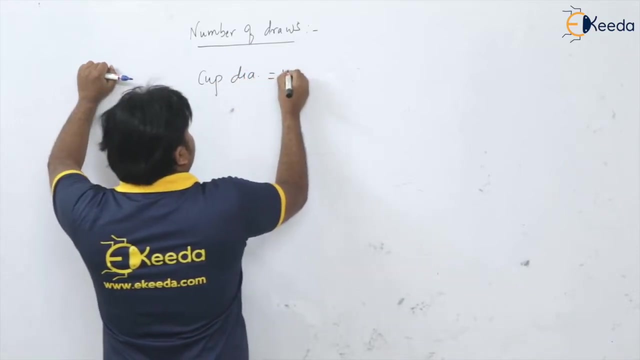 how many stages- one, two, three- so the operation, deep drawing operation- can be done in these three stages. okay, like that we can able to find out the number of draws. let us- i will take one example- say: suppose a cup of diameter 15 mm is required and height of the cup we required at 60 millimeter. 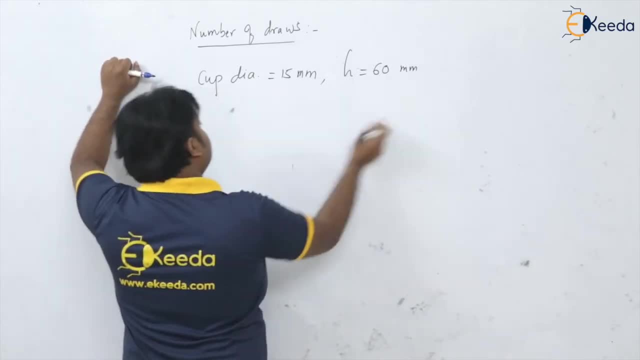 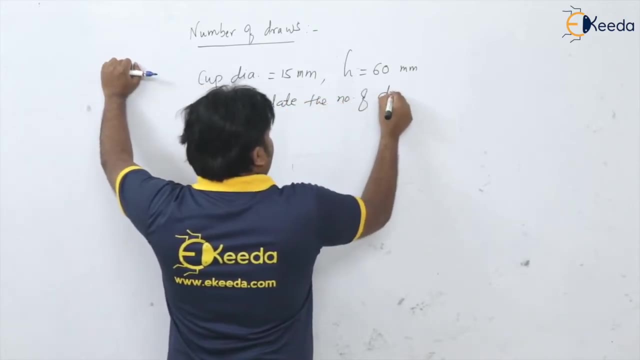 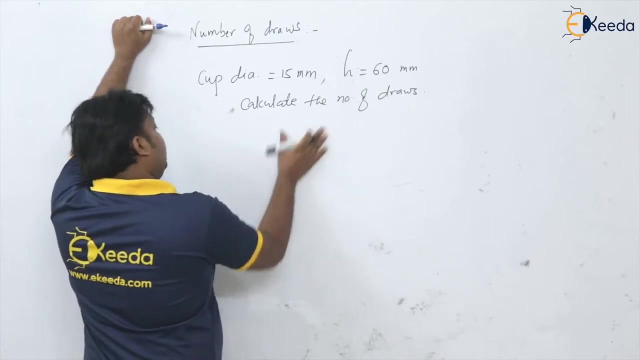 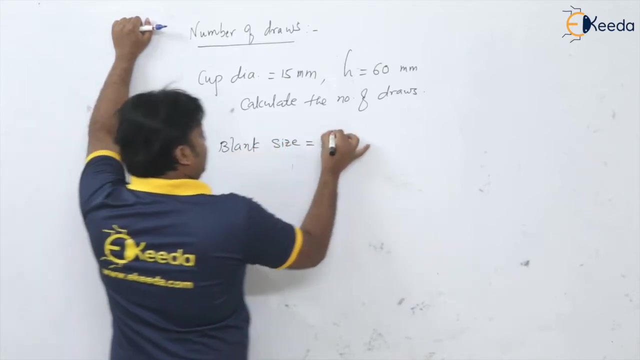 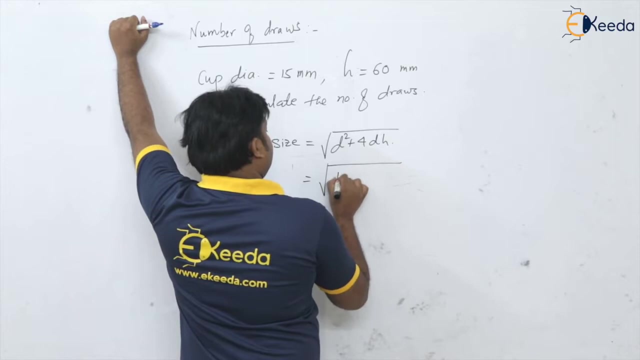 okay, and the question is: calculate the number of draws required to do this drawing operation? so here, first of all, we required what? the blank blank size. very important blank size is very simple under root: d square plus 4 dh, isn't it so? diameter: 15 square plus. 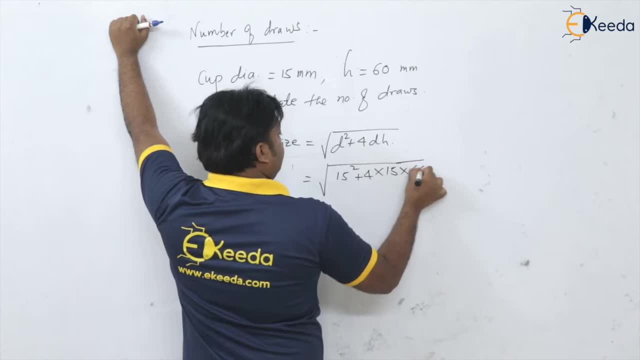 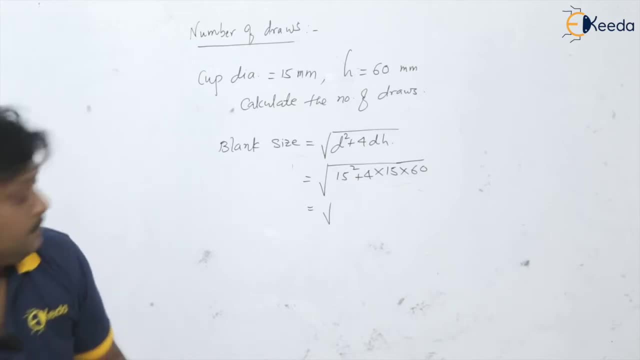 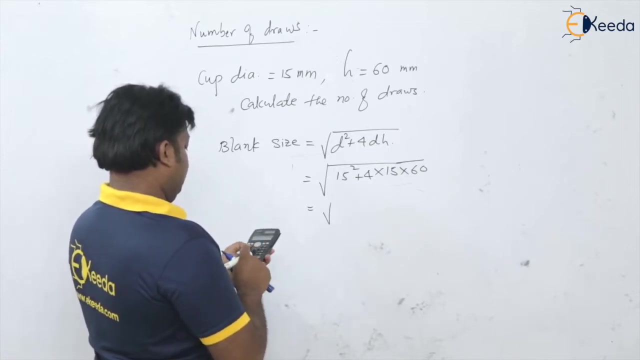 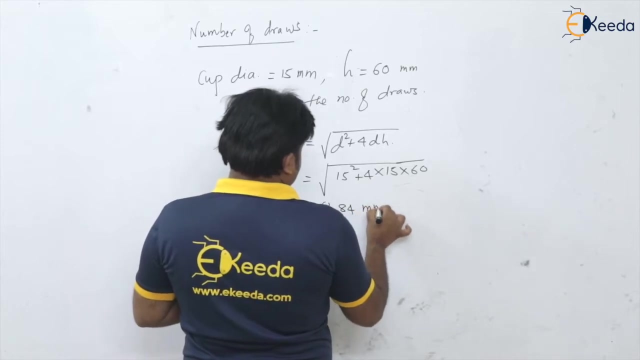 4 times 15 times 60. so how much it is if we solve it, 60 square plus 2 to 5 under root answer. so it is around 61.84, 61.84 millimeter. okay, so this is the available blank size with you and. 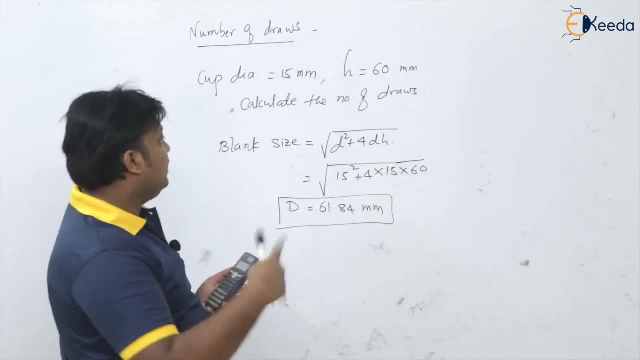 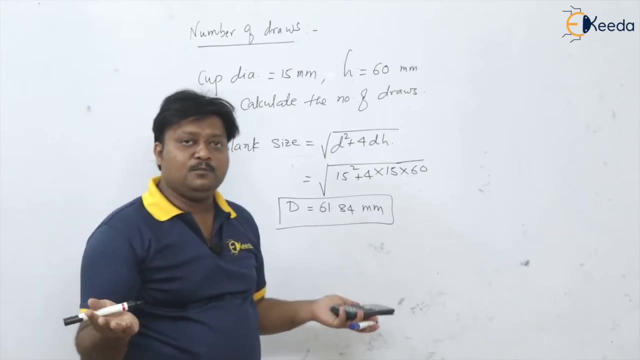 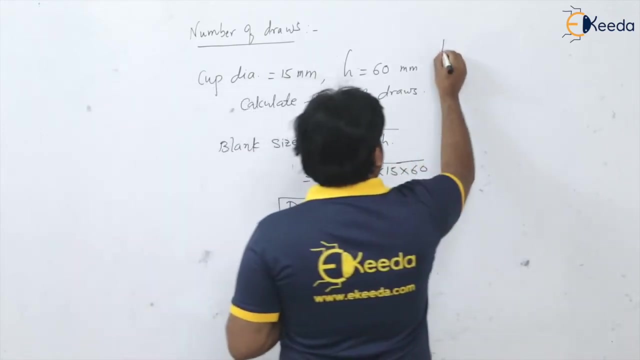 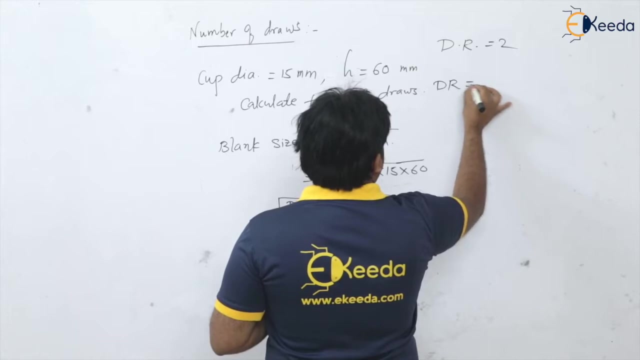 this blank size you are going to draw into the required cup diameter and height. okay, so here nothing is mentioned about draw ratio, isn't it? nothing is mentioned about draw ratio, so simply, we can get take it as draw ratio. how much you are going to take? it is 2, isn't it? so let us write: the draw ratio is equal to what the 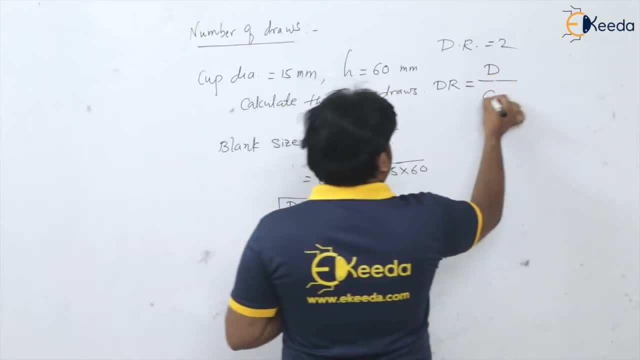 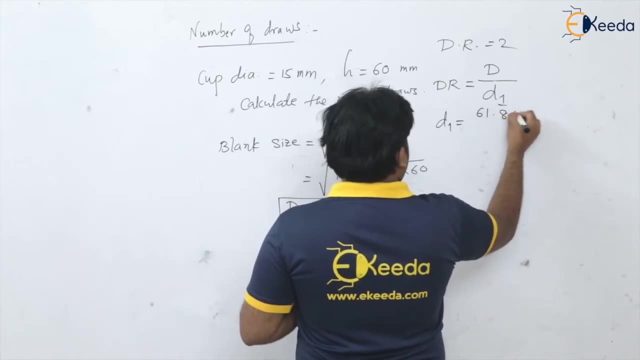 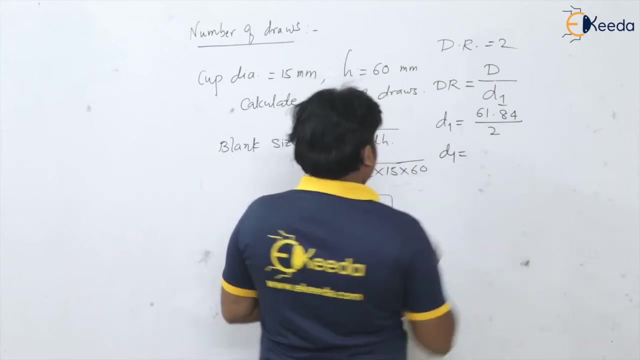 diameter. before drawing it was D divided by D 1, we are going to see. so D 1 will be what, 61.84 divided by what is draw ratio, 2, isn't it? so D 1 will be what divided by 2, 61.84 divided by 2, that is 30.92. 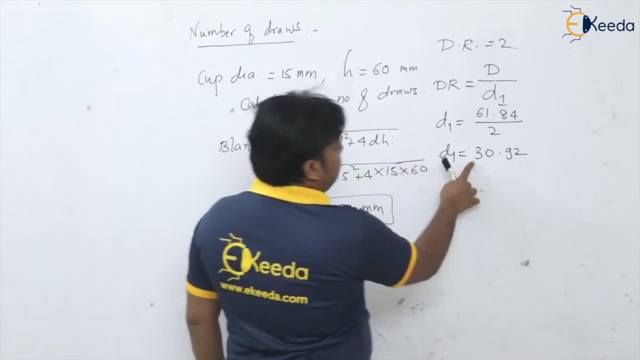 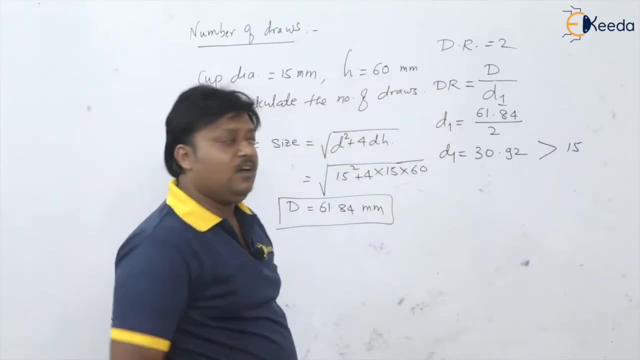 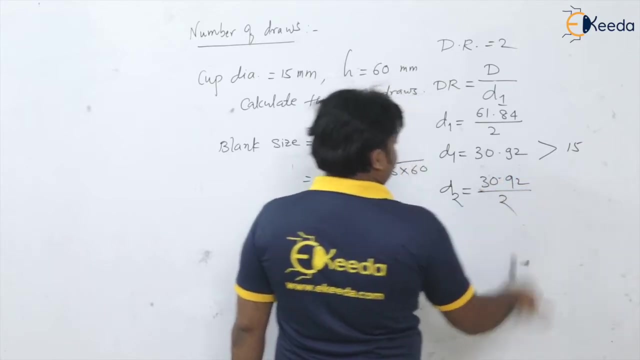 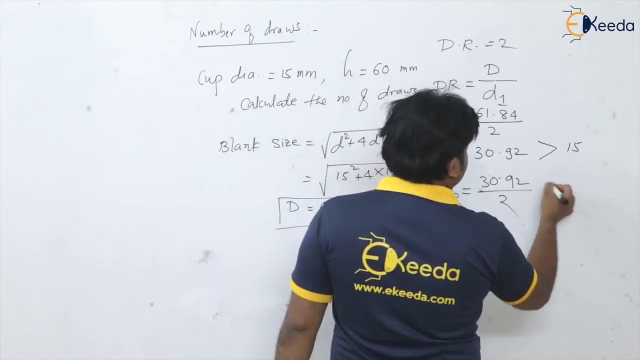 okay, you would just tell the following: similar thing. this is a D value, its equal to equate to 15. you was doing your work, that is 15.完成. its 15.二 divided by two. then how many you could get each 30.92 divided by 2? divided between the 2 things, the first H s, every step is different, which considers gumWhy don't proceed. this marks 30.94 divided by 2. first whole expression, forgetting s1, and then total value, then dr9, which is 15, dd15. so I really have to go for. now. how can we пять it minus 40 and then you move it shown. a control system changed the code again. now how can we find time given, which is 15 points? so we will now go off this first pass, so will go for the secondyou can make this 30.92 divided by 2, okay, but it as much as 30.92 divded by two. so if we keep her in the second pass, just like that, so we can. 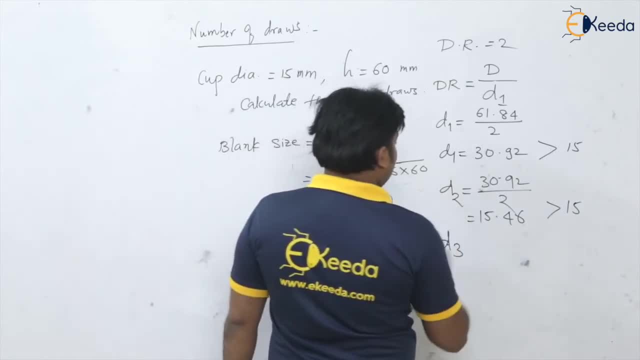 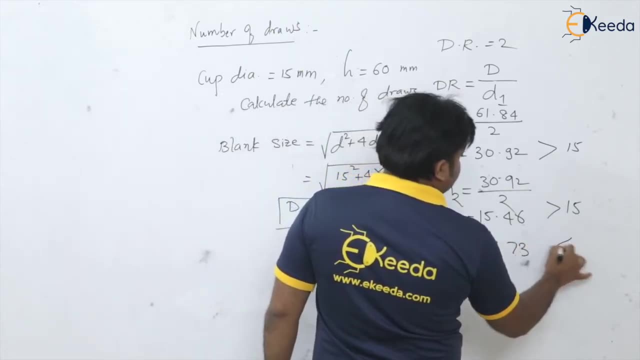 So definitely in the third stage, how much you will get? You will get 15.46 divided by 2, that is 7.73, which is less than equal to 15.. Okay, that is the capability. of the third draw is to. 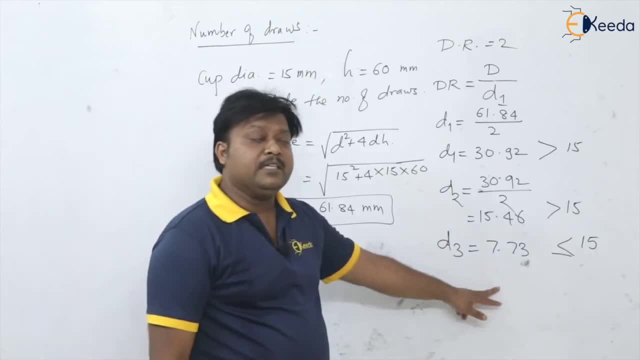 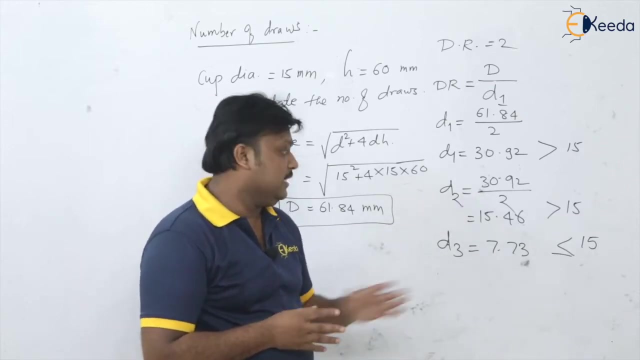 take the diameter to the 7.73 millimeter, So, but of course in the second draw it is greater than 15.. So definitely we have to go for the third draw. it is not like that direct 7.73, it is not like that we can control. we can control the diameter once you get this 15. 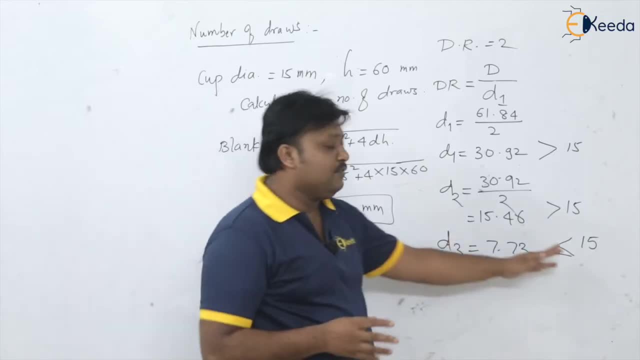 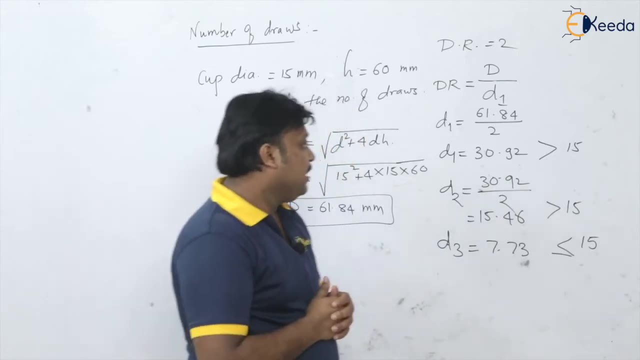 you can stop the operation there. Okay, and required 15 mm only. you can get. it is not like that. the cup will directly go to 7.73 millimeter. it is not like that, please remember. So, of course, at the third stage, the diameter now lesser than equal to 15.. So, how many stages you? 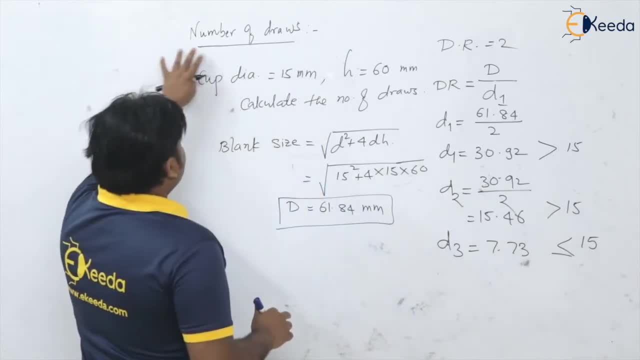 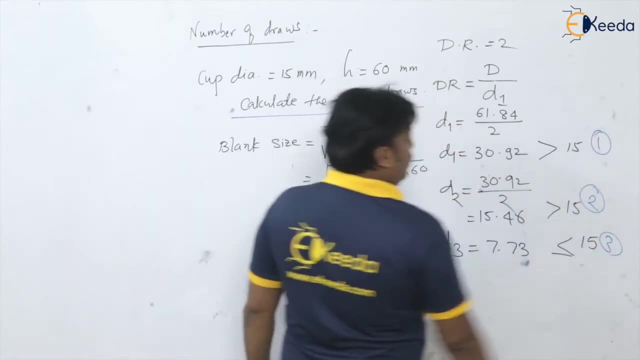 require. So you have to go for the third draw. it is not like that you have to go for required or how many draws. required question was same, only the calculate the number of draws. say, draw number 1, this is second and in the third draw the operation gets complete. you. 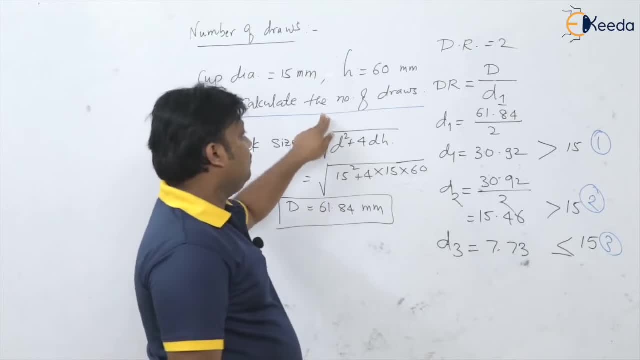 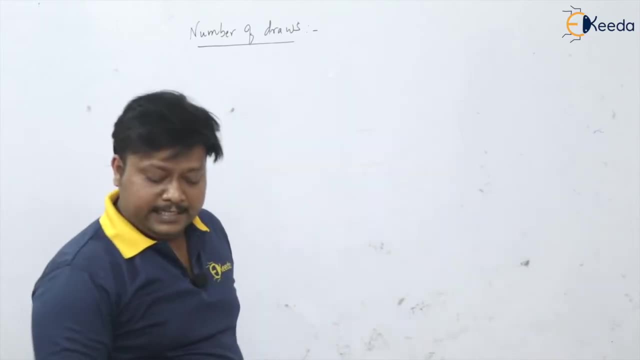 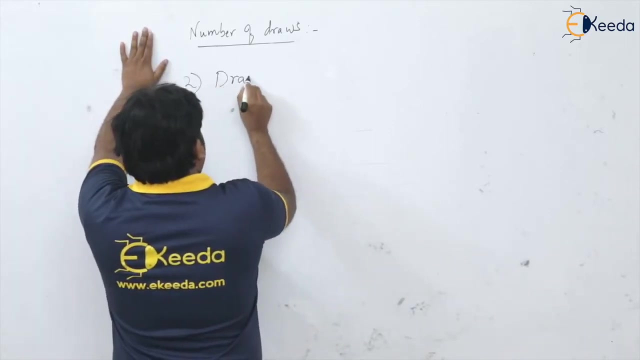 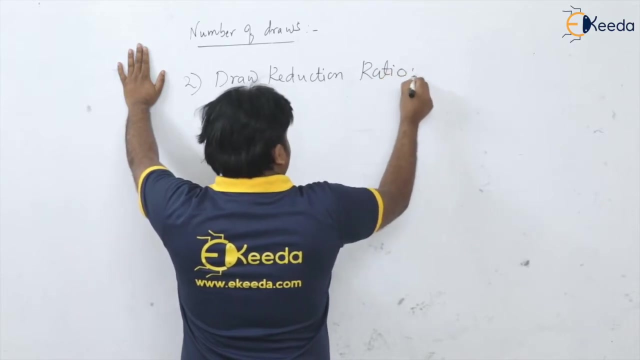 reached with a 15 mm diameter. so the answer is: 3 draws. how many draws are there? 3 drawsLike that? you have to solve the questions now. the another technique to calculate the number of draw is the draw reduction ratio technique. draw reduction ratio technique or method that is known as a DRR. 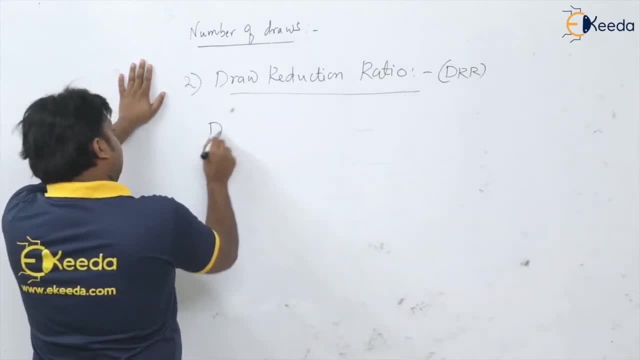 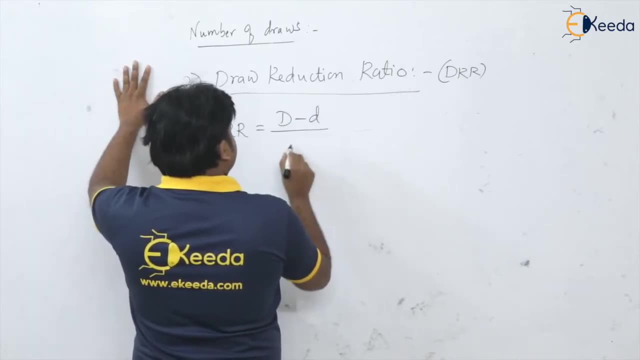 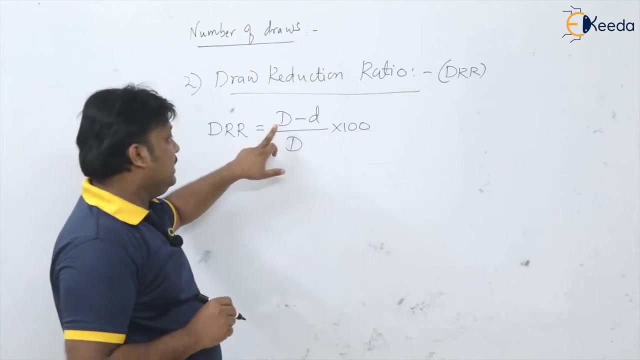 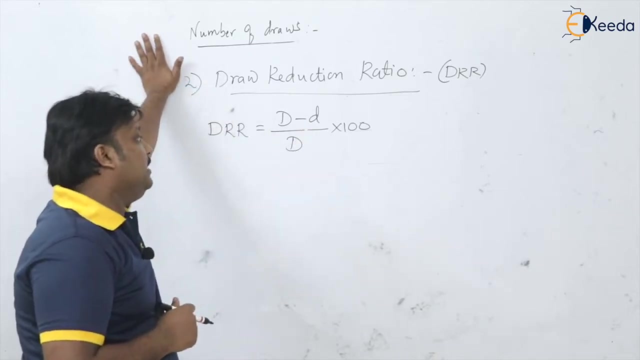 DRR. so how to calculate DRR? so DRR is equal to: so D minus D, divided by capital, D into 100. okay, so the initial diameter minus the diameter in the respective stage, divided by initial or original diameter, you will get the draw ratio. very simple, this is percentage reduction, like. 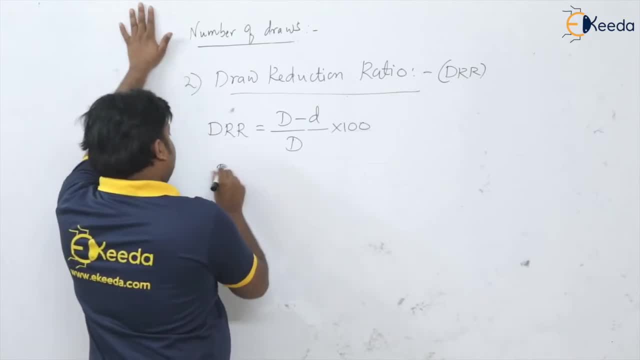 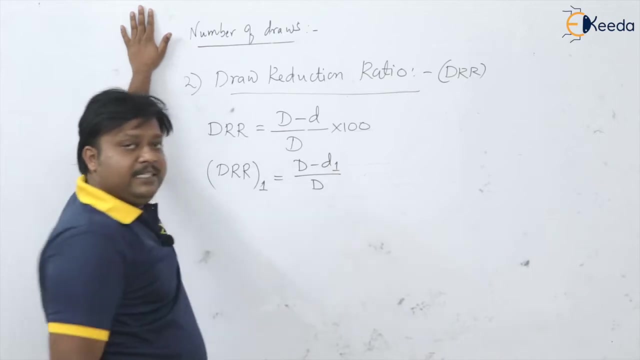 thing, okay. so if I want to write for DRR 1, okay, DRR say first for draw reduction ratio, then it will be D minus D 1 divided by D. that is D is the blank size and even is a diameter in the first stage that I'm going to get okay into 100. 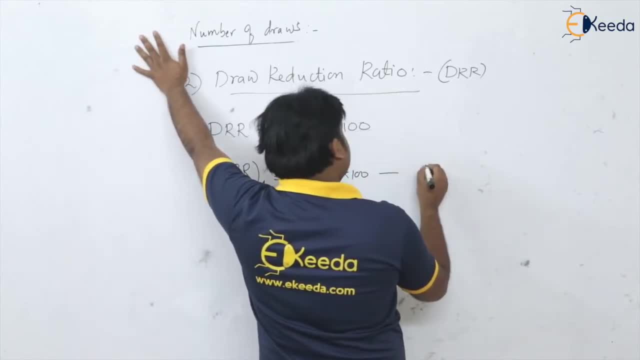 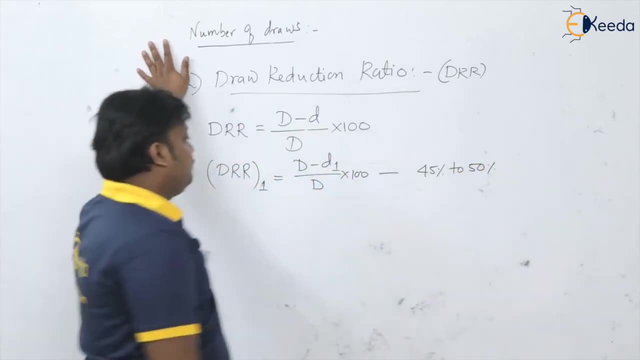 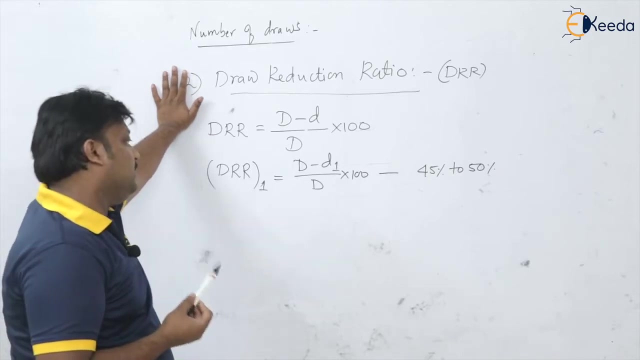 so it is in percentage. so draw ratio, draw reduction ratio in the first stage is about 45 to 50 percent. please remember this. okay, so definitely draw ratio in first stage, how much you can get 45 to 50 percent, that is draw reduction ratio we are getting here. so 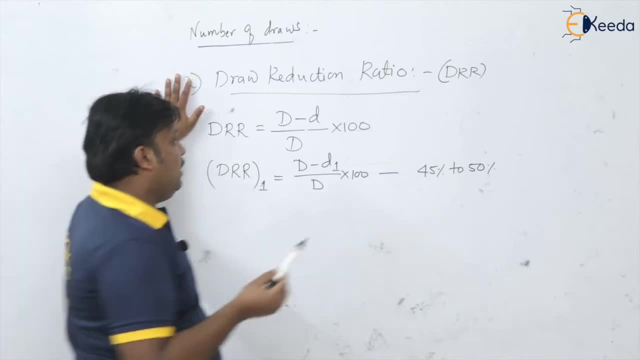 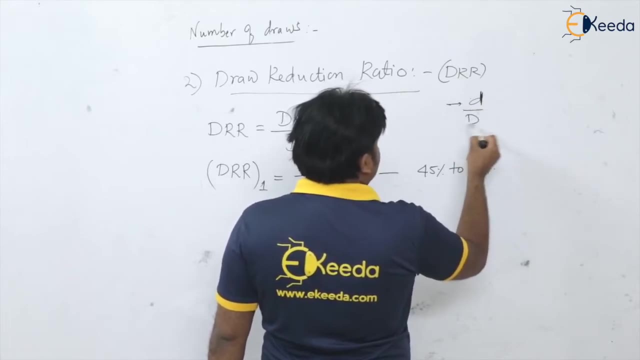 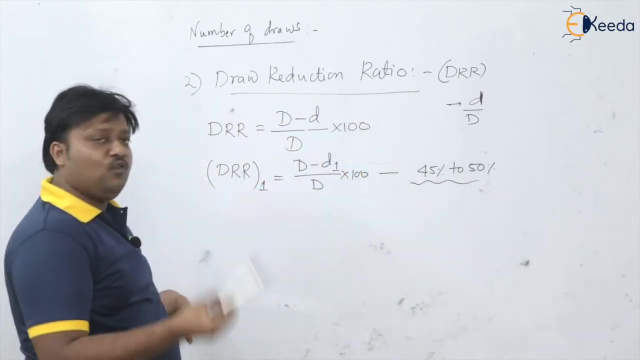 suppose directly from the given data. suppose you have got the value as capital small D, that is required diameter divided by blank diameter. if this ratio is more than, say, 50 percent, so definitely you have to go for this reduction technique in the number of stages. okay, so for 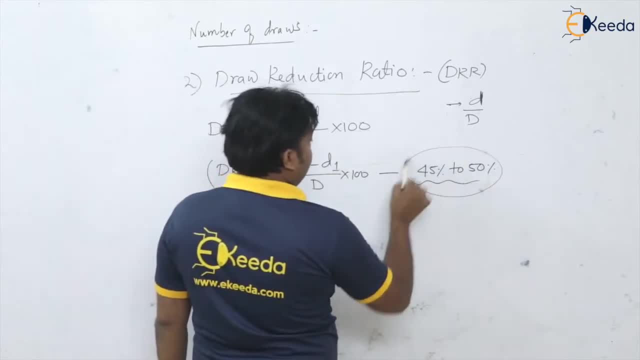 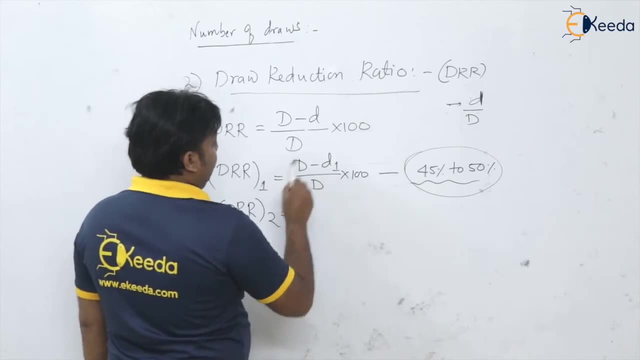 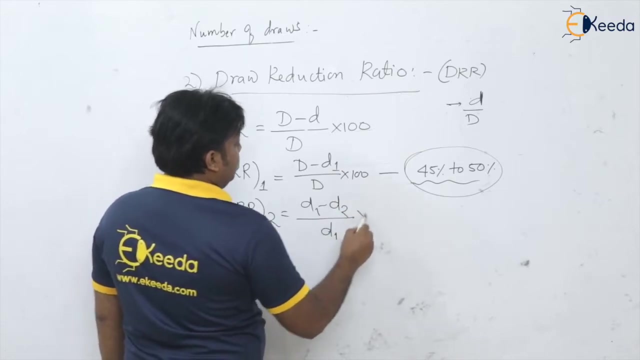 first reduction you got is about 45 to 50 percent, like that you are having in the DRR reduction ratio in the second draw, as now available diameter D 1 minus, going to get the diameter D 2 divided by P 1 in 200. ok, like here, 30 to 35 percent of reduction you are. 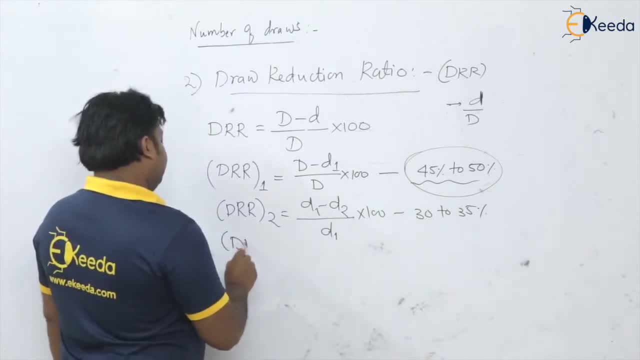 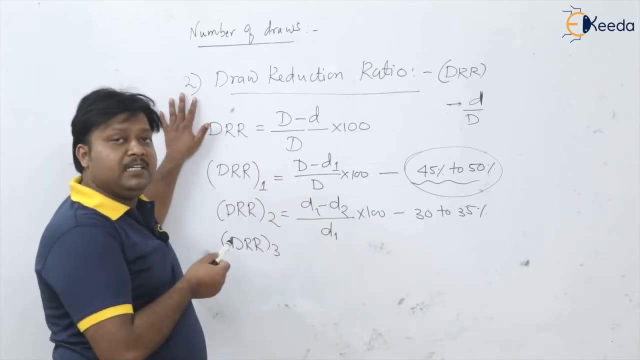 going to get in second row and now see when you are third or fourth draw. it is very important to have you remove the material and go for the enhancement of the ductility by the annealing operation okay, so that you can get the further deformation, further reduction into the deep drawing operation. please remember. 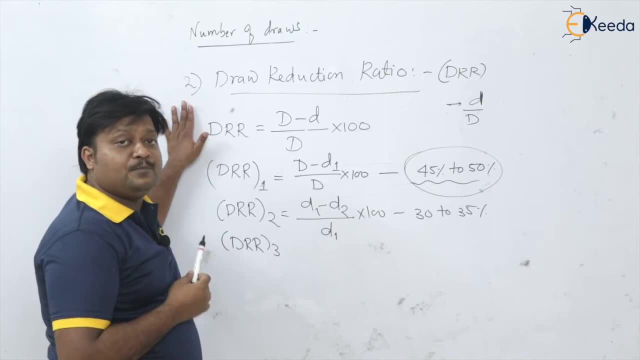 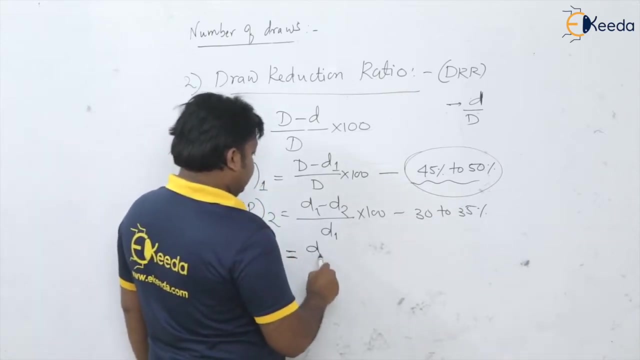 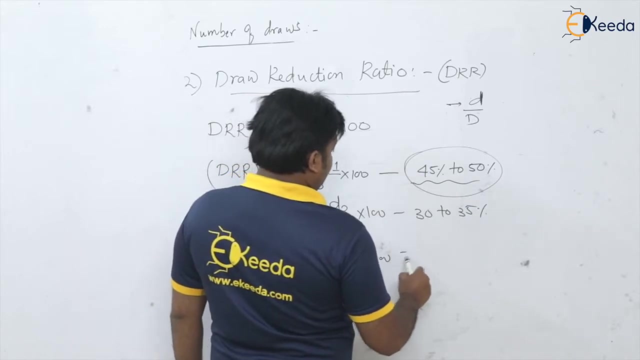 you have to have at the enhancements enhancement into the ductility so that it can be easily drawn by the annealing process. so that is not so much important, but for your information i am telling this. so, third draw: it is d2 minus d3 divided by d2 into 100, around 20 to 25 percent of reduction. 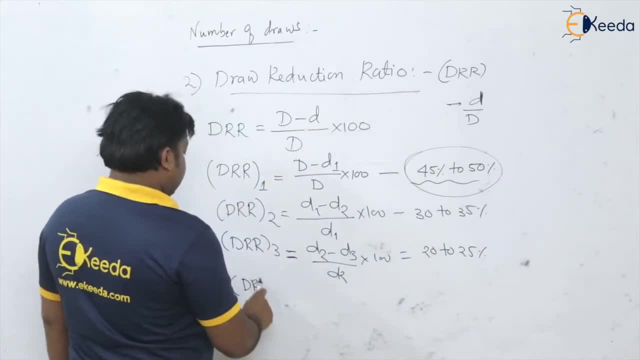 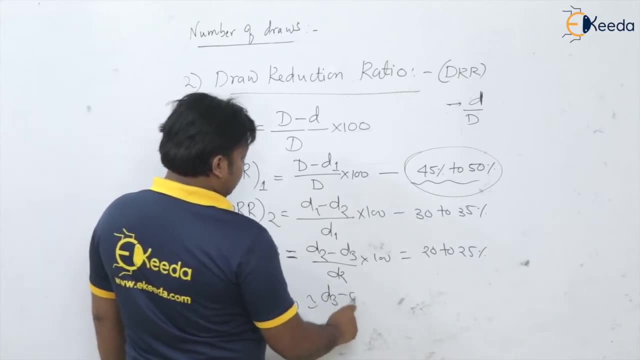 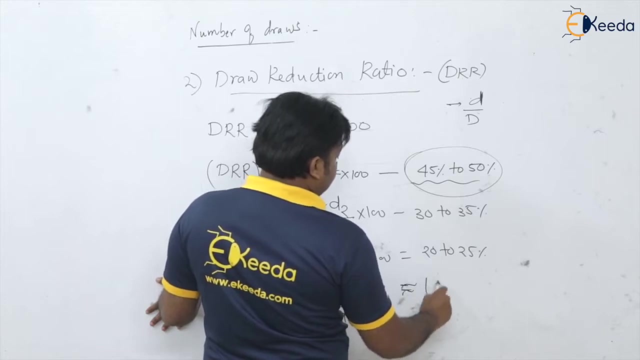 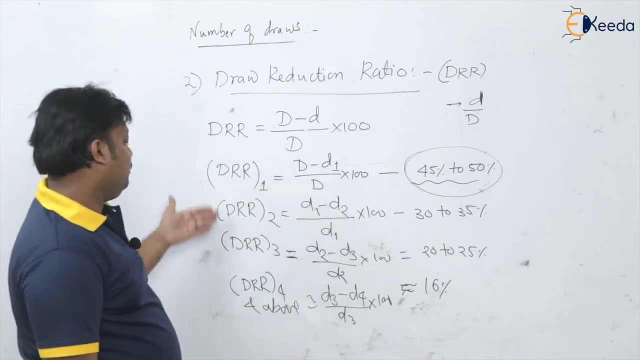 you are going to get here and last drr 4 and above. so maximum reduction: you can get d3 minus d4 divided by d3 into 100, isn't it? that will be nearly about 16.. percent, 16 percent. so easily again we can have the number of draws you can. 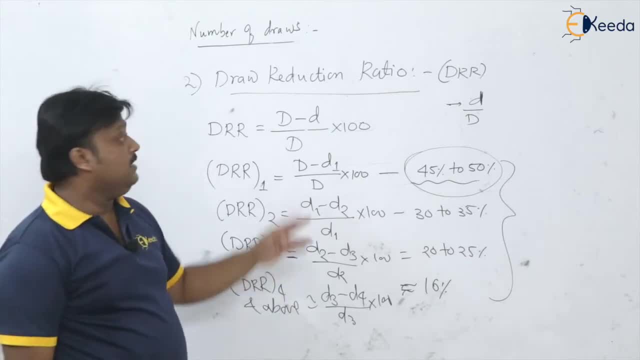 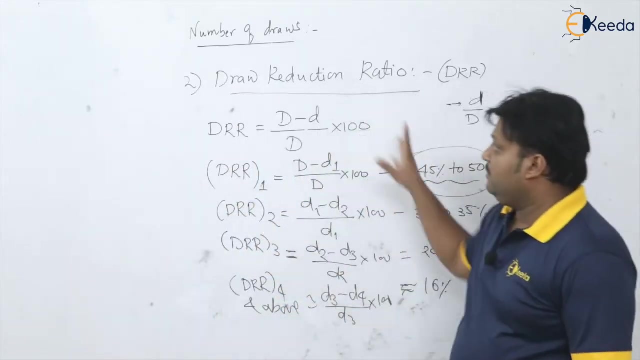 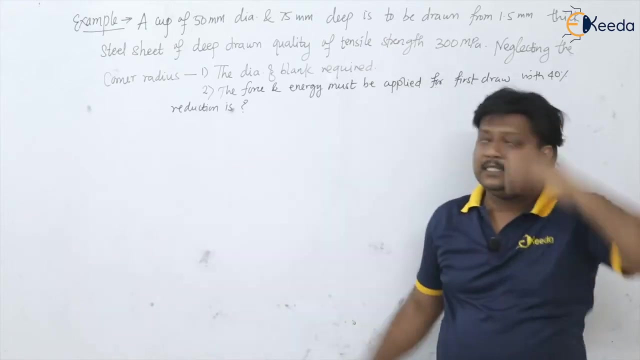 able to calculate kidney draw if you are having the draw reduction ratio technique, so in this fashion, you can calculate the number of draws. okay, so, let us discuss one example where we are going to consider this draw reduction ratio technique. okay so, students, let us discuss this example. the question is a. 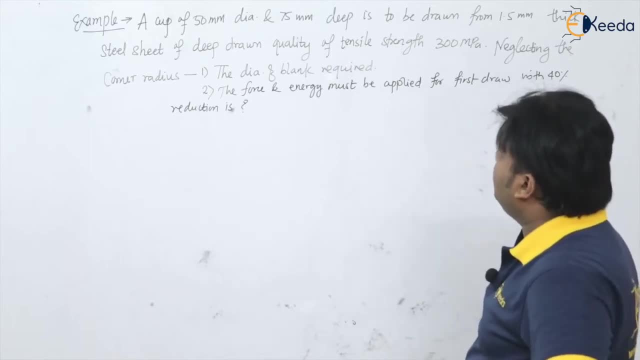 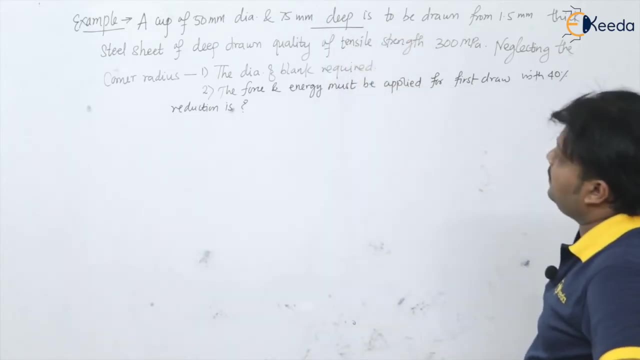 cup of 50 mm diameter and 75 millimeter height. this is the deep. okay, and that is height- is to be drawn from 1.5 m thick steel sheet of deep drawn quality. of the tensile strength: 300 mega Pascal, neglecting the corner radius, calculate number one, the blank size and the force. 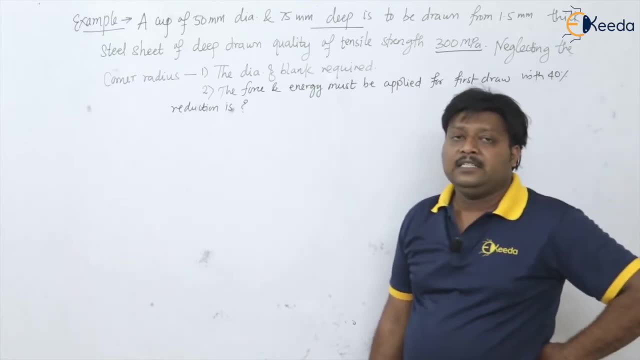 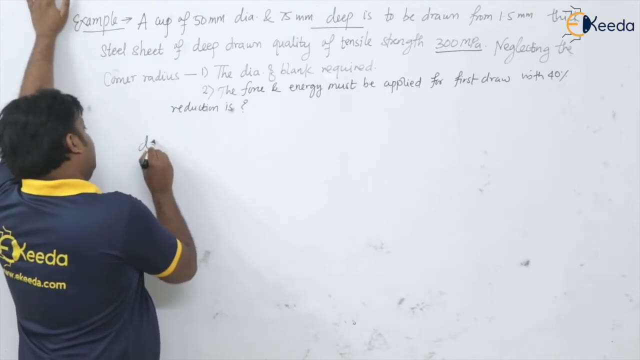 and energy required for the first draw. in the reduction in first draw, how much? 40 percent is given. okay, so see diameter of curve. how much 50 millimeter height of the cup is 75 millimeter, say Sigma tensile strength is given, isn't it we? 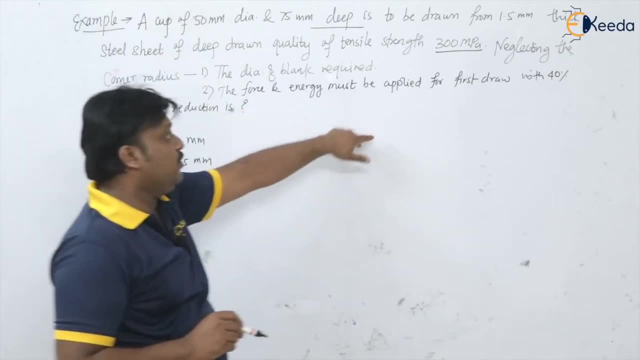 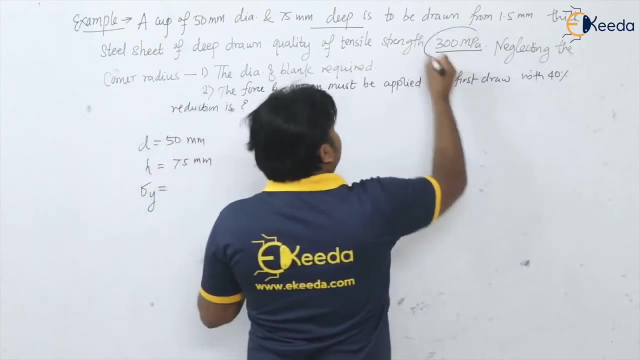 want here Sigma Y. so please remember many times in week drawing questions they are giving us the ultimate strength of the sheet or they are giving the tensile strength of the sheet, but we want here Sigma Y is strength of the sheet. that is generally we are taking as half of this. 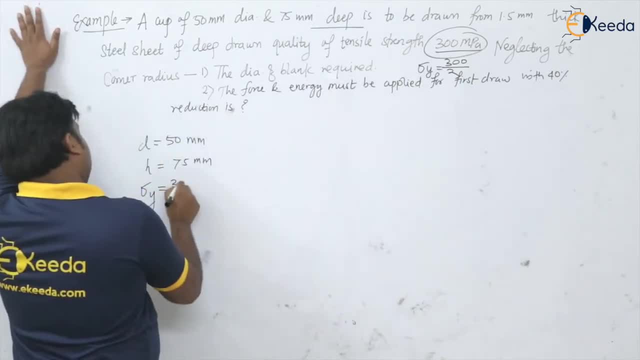 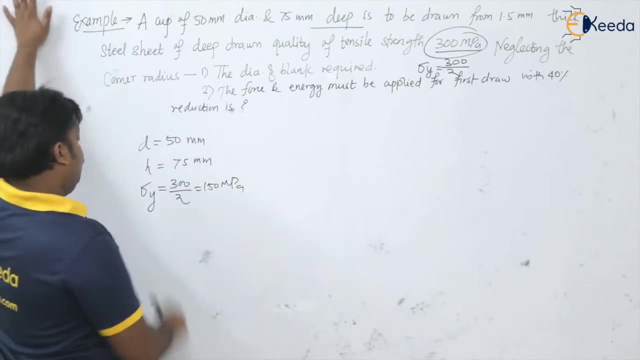 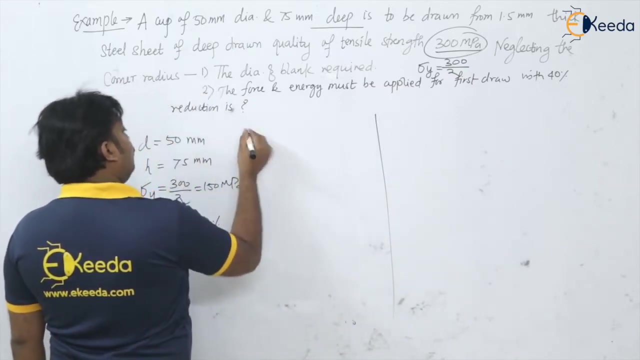 tensile strength. okay, so here Sigma Y will be 300 divided by 2 it is 150 mega Pascal. and then you can go for the calculation. draw reduction ratio. in the first stage, how much? 40 percent is given. okay. now what is the blank size? very, very easy thing. corner radius is not given so directly. 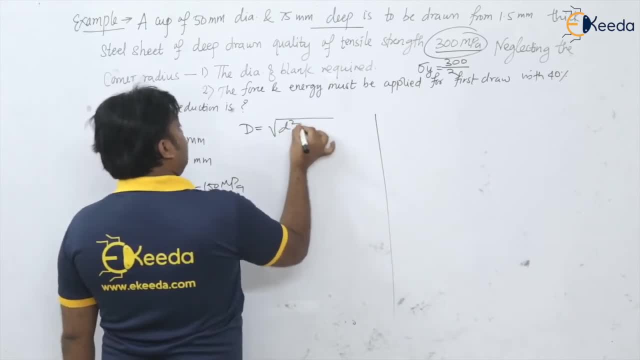 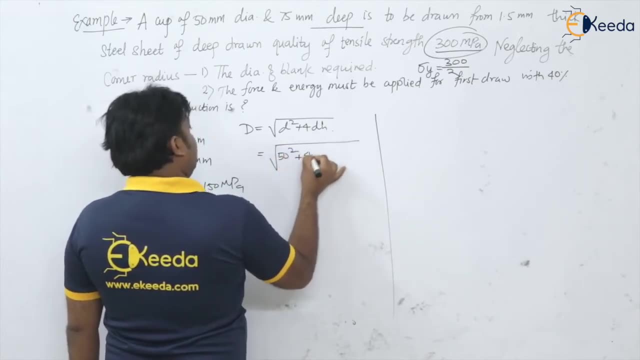 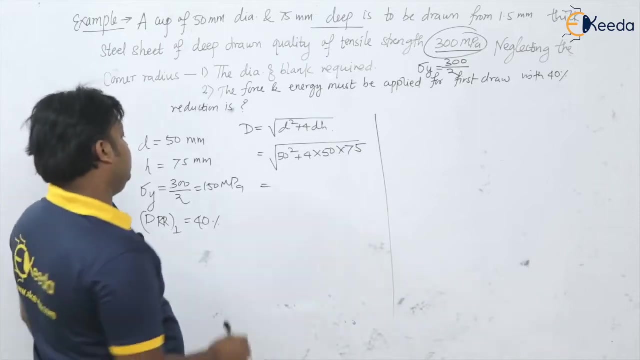 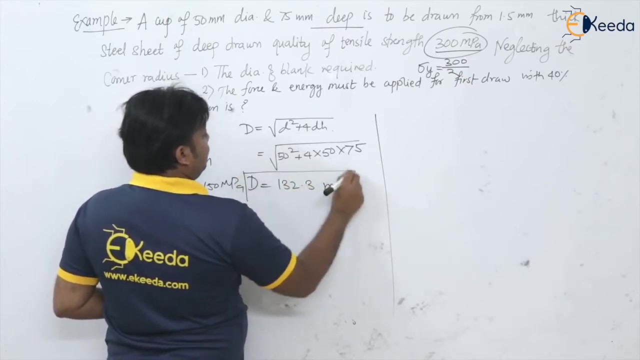 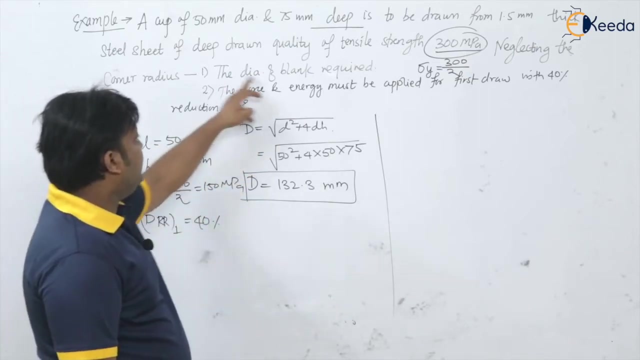 blank size is equal to, under root of d square plus 4 dh. so what is diameter? 50 square plus 4 times 50 times 75? what is the answer? see, you will get this answer for this d as 132.3 millimeter. so first bit of the question is clear. very simple calculation of the blank size. okay, so diameter of 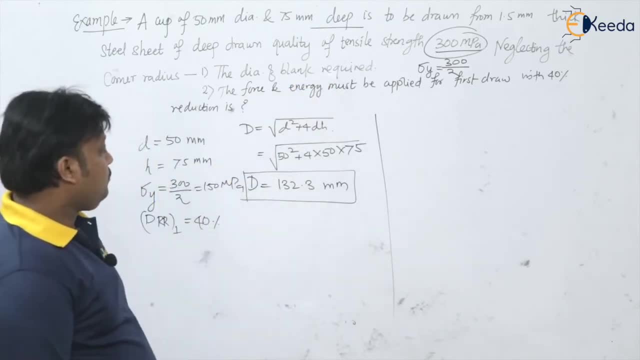 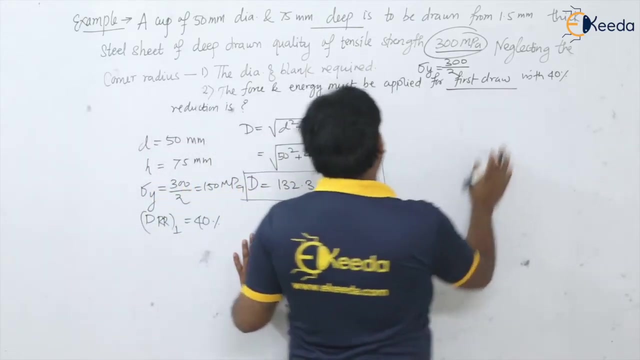 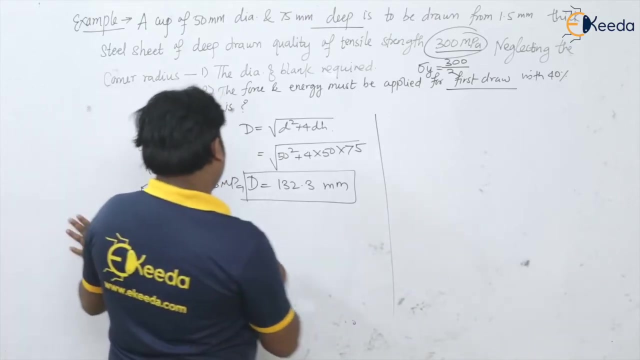 blank. we get it here now what they are saying: that the first draw, the reduction, is 40 percent. so let us go for the calculation of the force and energy for the first drop. they have asked force and energy they have asked, so let us say the force for. 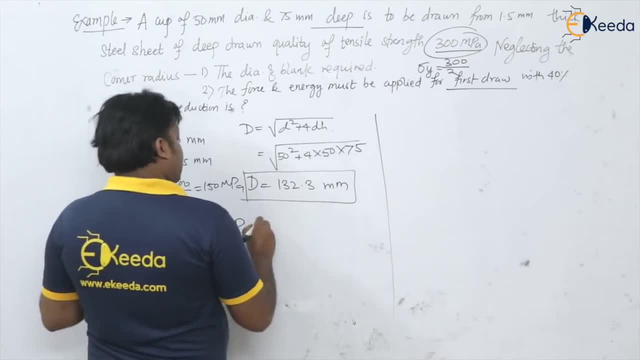 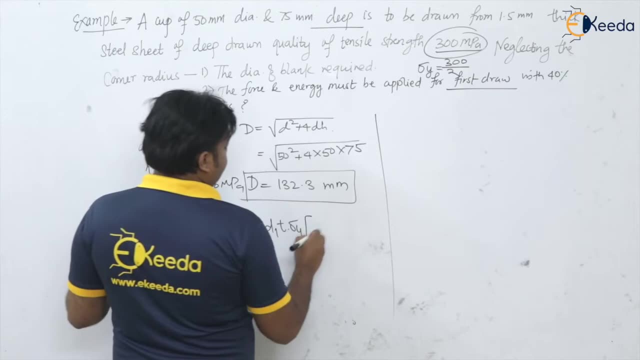 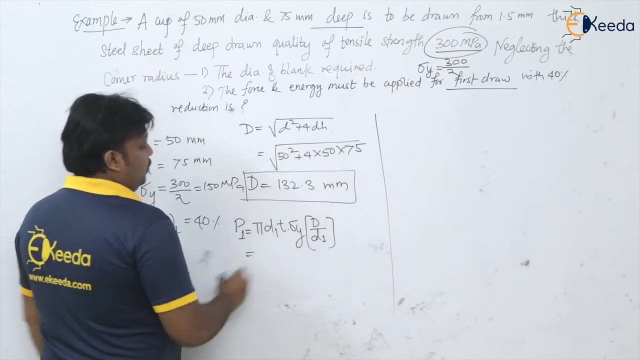 first test, we know it is, p1 is equal to what pi d1 d into sigma y, into bracket capital d by d1 minus c is not given, then it is not there. so get zero. so d 1 d 1, get cancelled. so pi times capital d times. 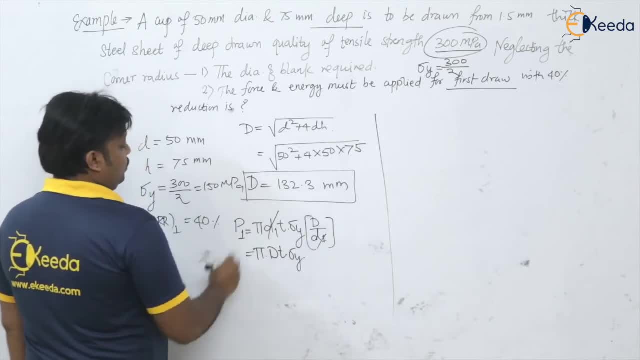 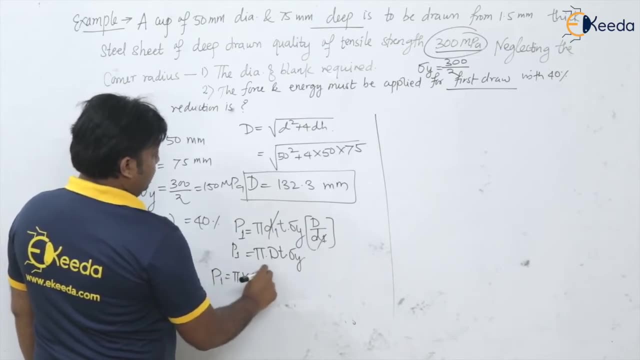 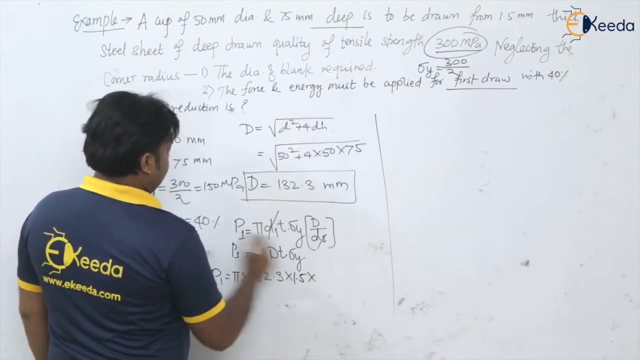 t into sigma y will be the force in the first stage. so put the values: p 1 will be equal to pi. into 132.3. into thickness, is how much 1.5 millimeter? into yield strength, 150 mega possible? so if you calculate you get it here 93.5, this kilo newton. okay, so this is the p 1. 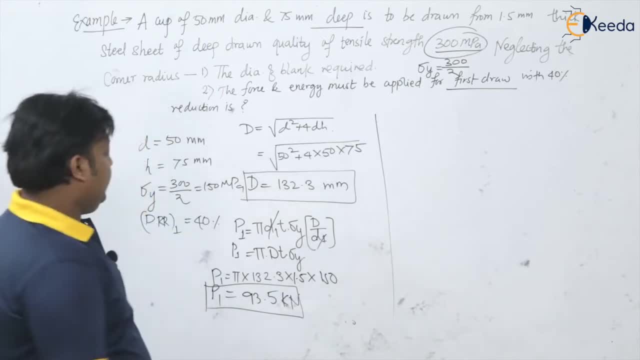 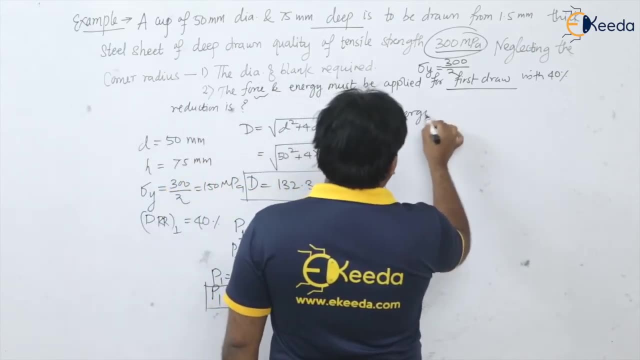 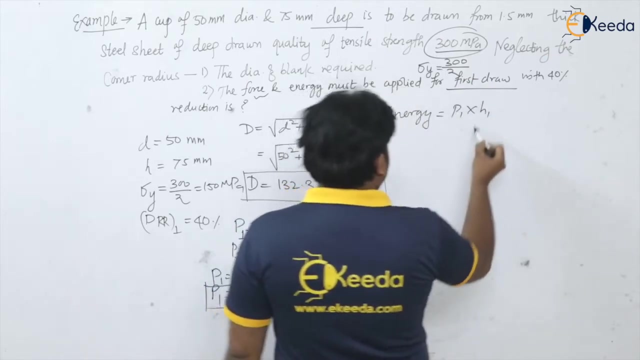 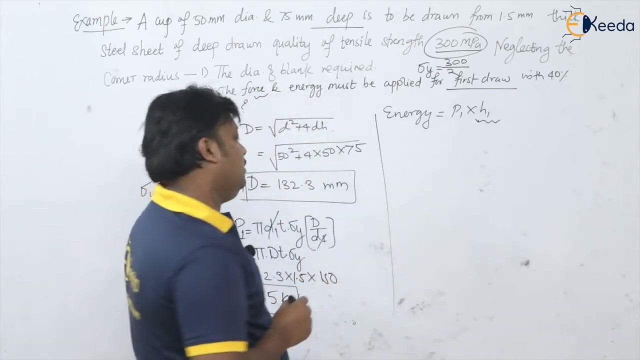 okay, now the force also get calculated. now energy in the first draw. energy is how much, that is p 1 into h 1. okay, now h 1 is here important. so what is the height in the first draw? to calculate this height in the first draw, we 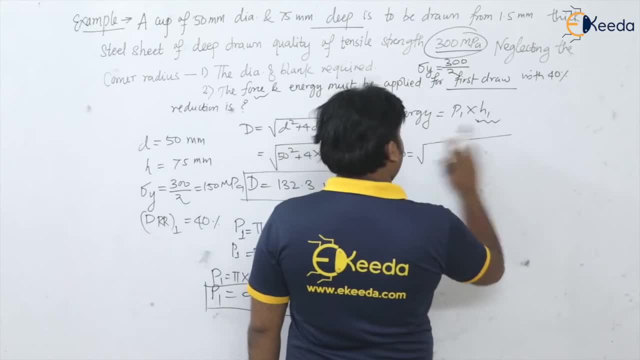 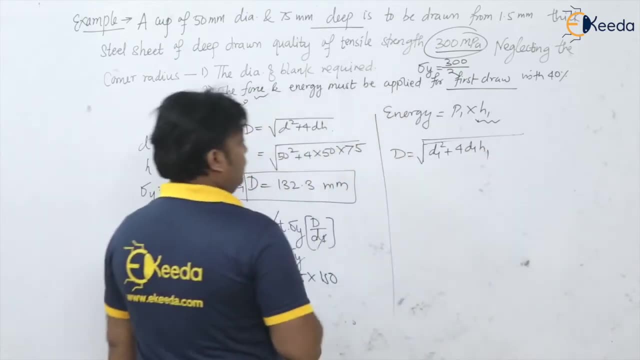 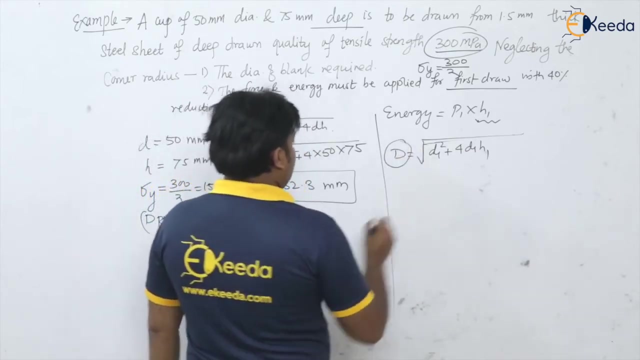 know that this d is equal to under root of, and i write for: write for the first draw: d 1 square plus 4, d 1, h, 1, isn't it? now what is the blank size for the first draw? 132.3 is equal to. 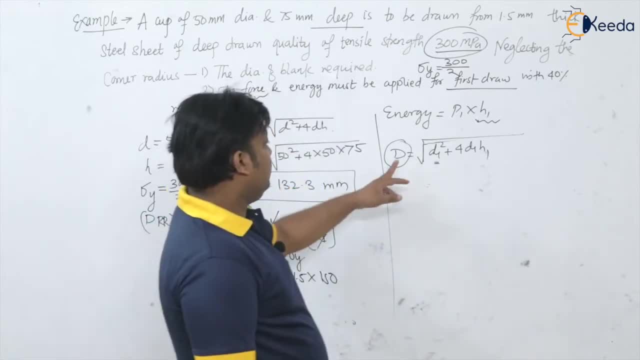 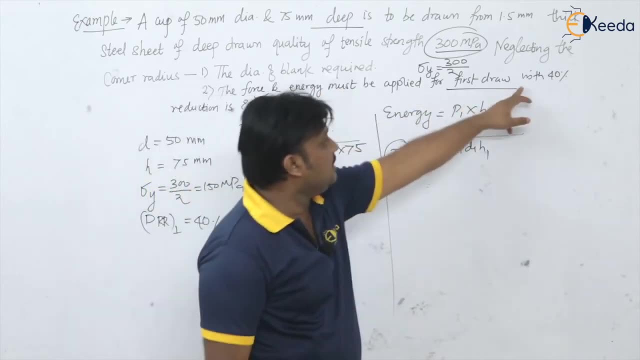 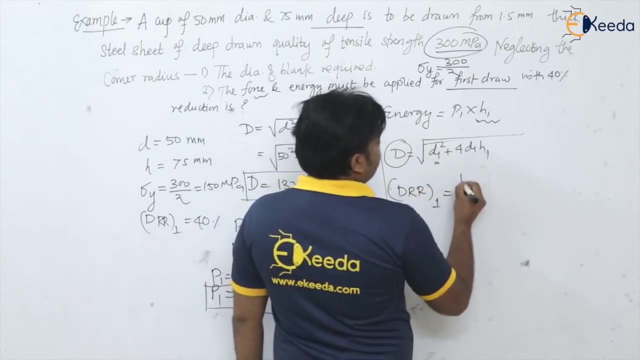 we need this diameter. okay, to calculate the h1, we need this d1 also, isn't it so how much first draw reduction di. so first draw draw reduction ratio for the first draw is: how much is d minus d1 divided by t into 100? so it is given as how much? 40 percent, that is 0.40. 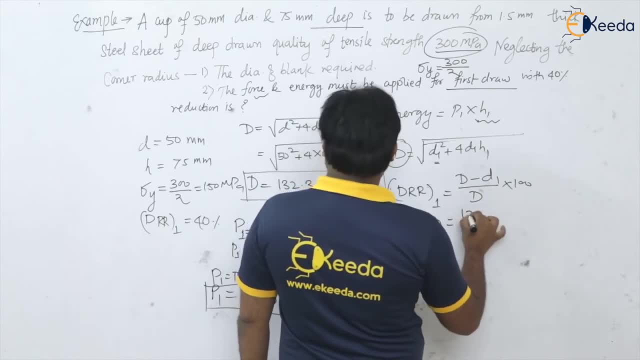 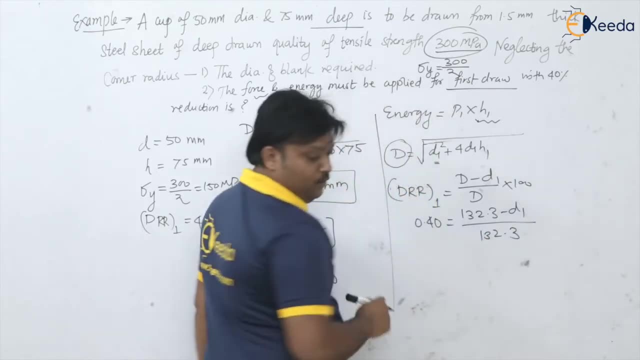 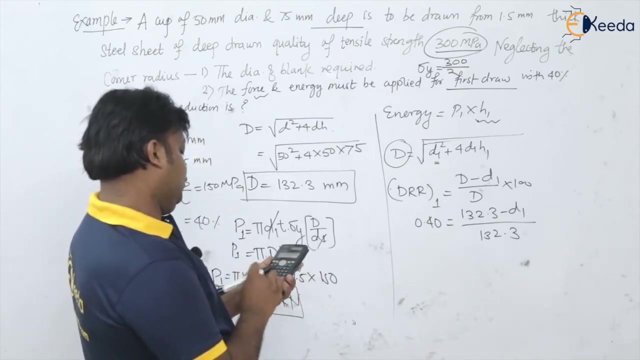 is equal to capital: d 132.3 minus d1 divided by 132.3. so calculate for d1. it will be how much 132.3 into 0.40 and 132.3 minus this answer, you get 79.38. so d1 will be 79.38. 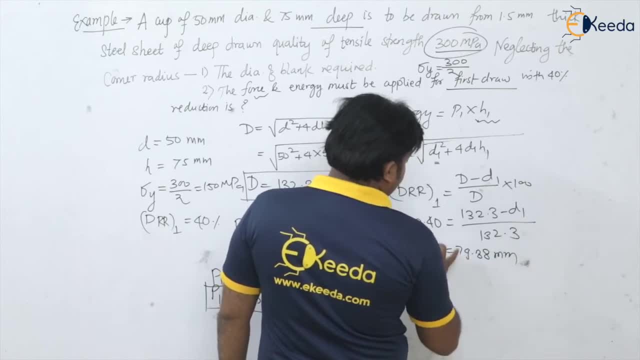 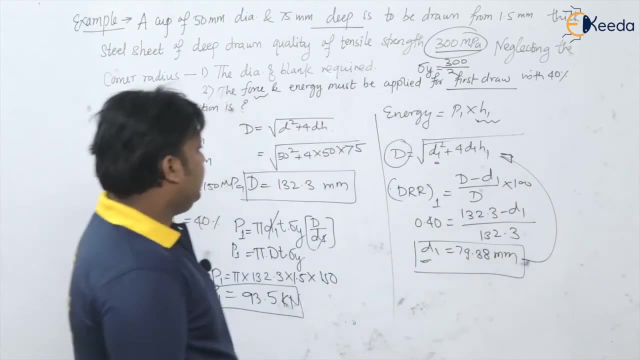 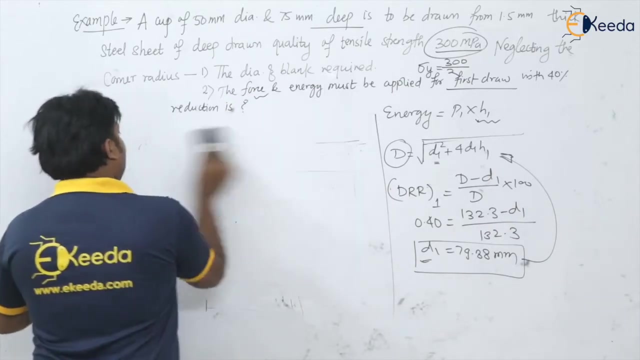 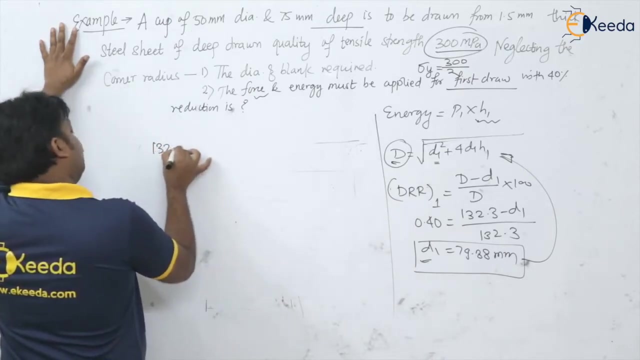 millimeter. okay, now put use this d1 value in this equation, you can able to get the value for h1, that is the height of the cup in first draw. okay, because you want to find out the energy in the first draw, that is p1 into h1. so what is value of d? 132.3 is equal to under. 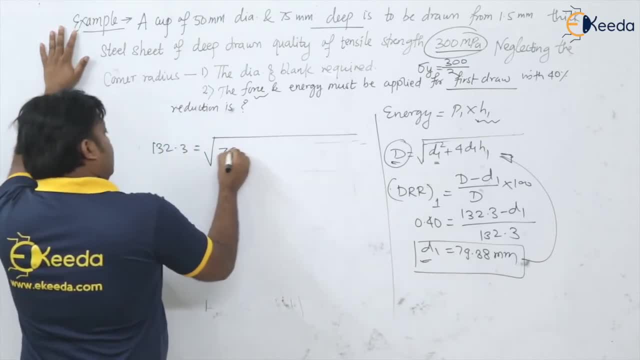 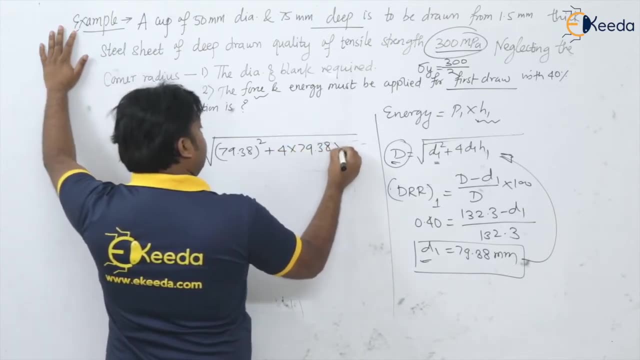 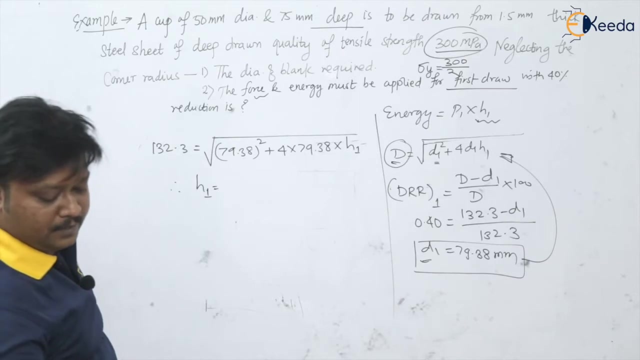 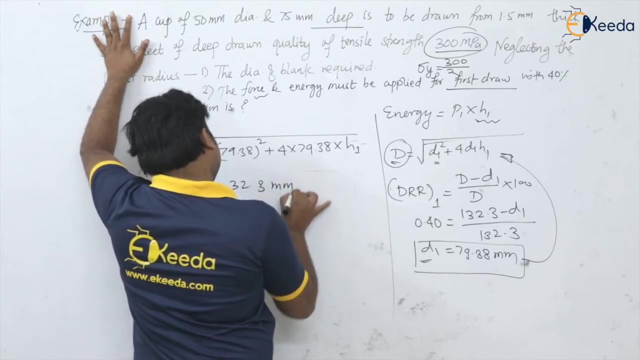 root of d1, 172.3, 79.38 whole square plus 4, into 79.38, into h1. dear students, please calculate for h1. i will write directly here. i am having this value as 32 point 32.3 millimeter. okay, so this is h1. 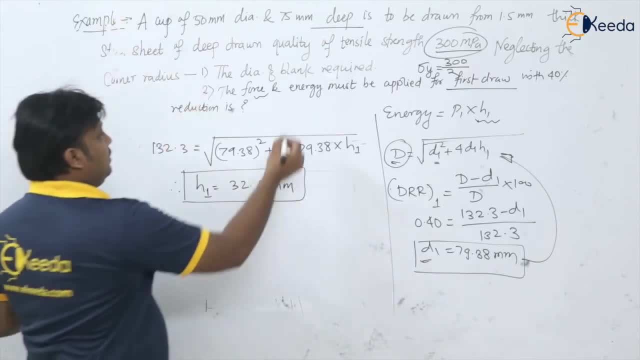 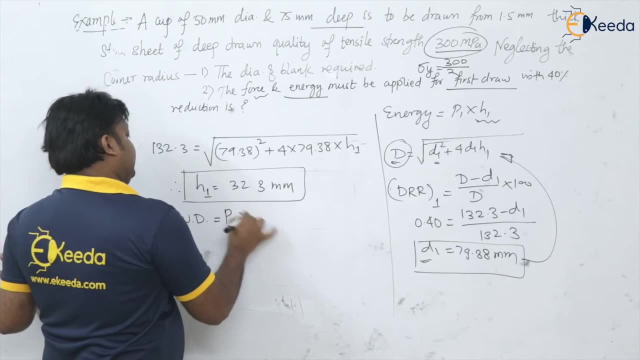 32.3 millimeter. now, very nicely, you can calculate the energy in the first draw, that is say, work done or energy same, which is equal to p1 into h1, so p1 having 93.5 kilo newton, so into 10 to the power. 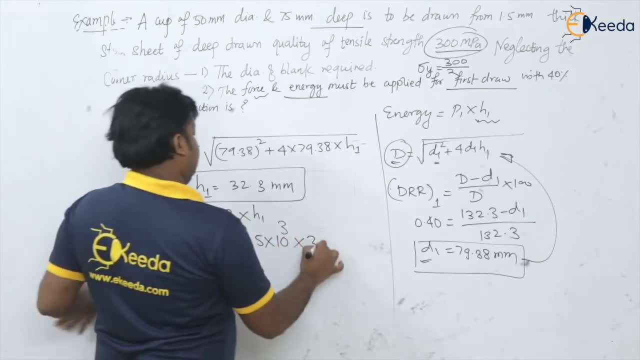 3 newton into h1, 32.3 millimeter. we have to convert it into meter, that is, into 10 to the power 3 newton. so this is h1, 32.3 millimeter. we have to convert it into meter, that is, into 10 to the power 3 newton. 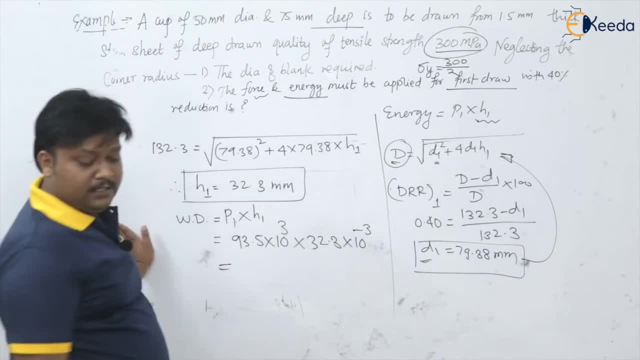 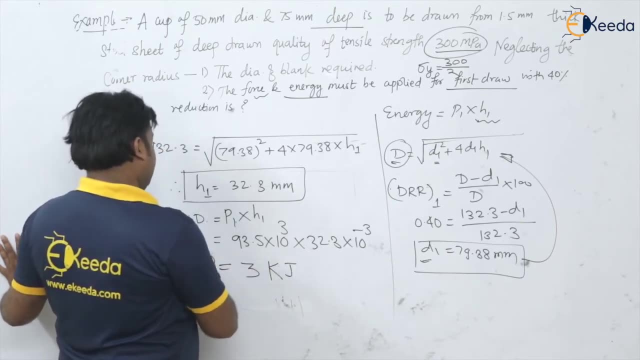 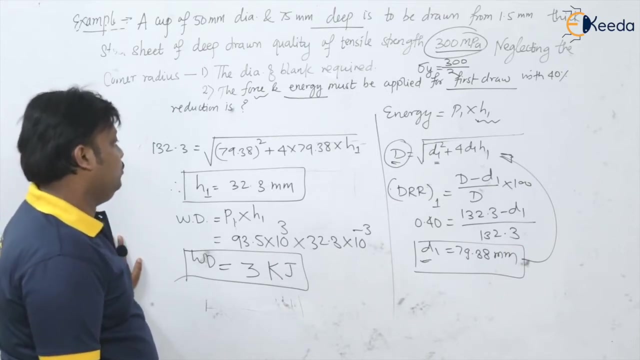 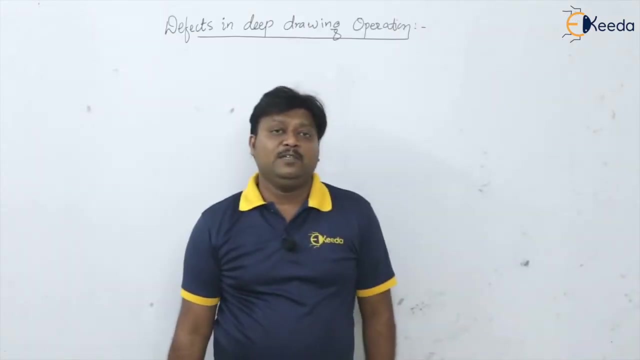 into the power minus 3 and if you calculate you will get the answer nearly equal to 3 kilo joules. please check and tell me. so work done or energy in the first draw. so this is the answer understood how to solve this. please check, dear students, in this video. 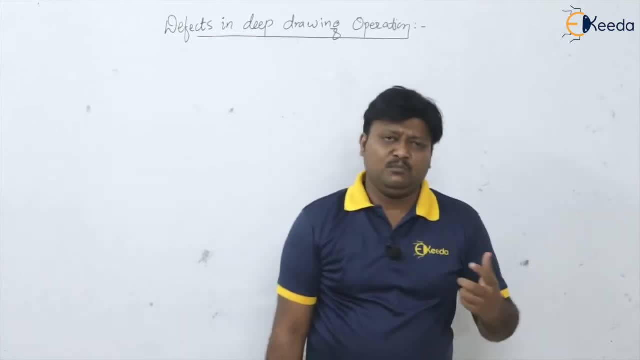 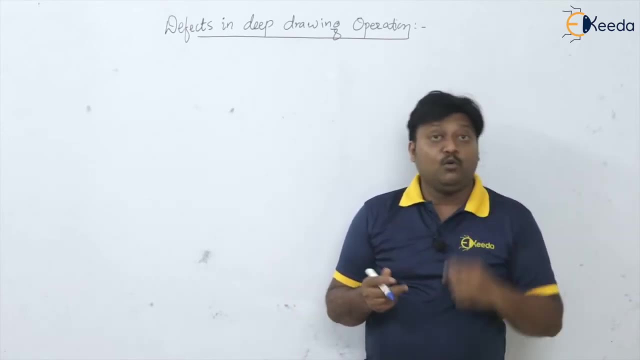 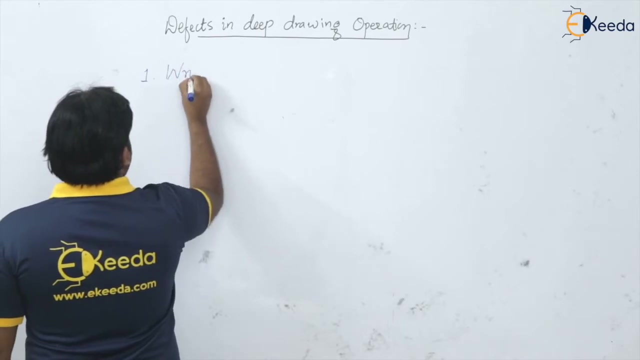 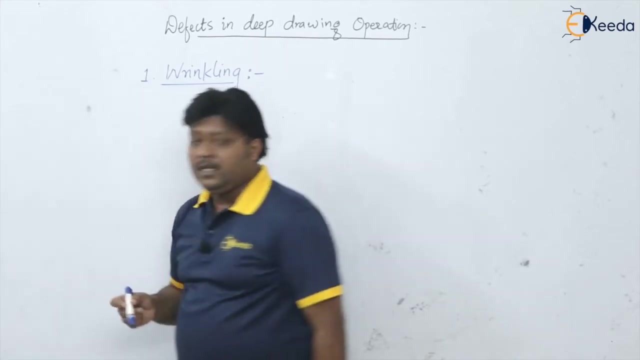 we are going to discuss the various or the most common defects in the deep drawing operation. so in the deep drawing operation, the one of the most common defect that we know already, that is the wrinkling, the wrinkling. so this is the most common defect that we are observing into the wide, into the deep drawing. 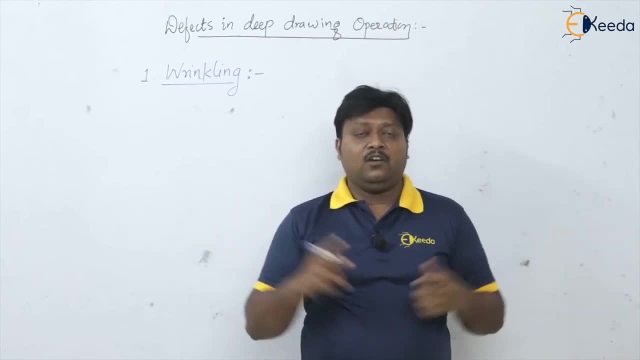 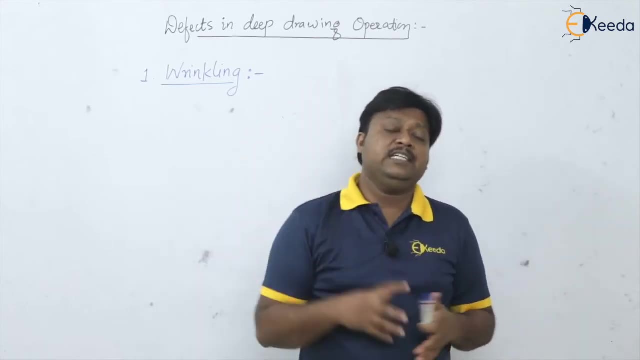 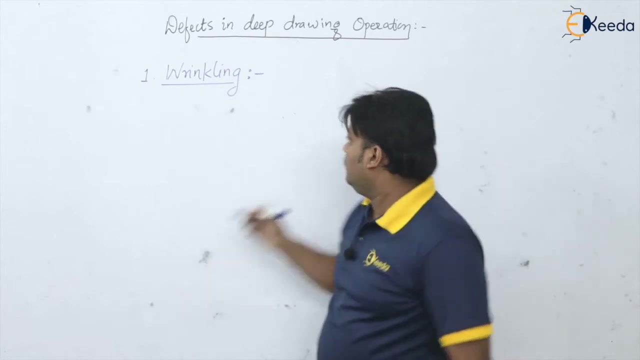 operation where there are the foldings or the lifting of the the sheet in upward direction, when this force is applied by the punch on the sheet. so what happened? because of this lifting, the foldings are produced on this, a flange portion. okay, so we are getting this. foldings at the flange portion of the curve is nothing but the wrinkles. 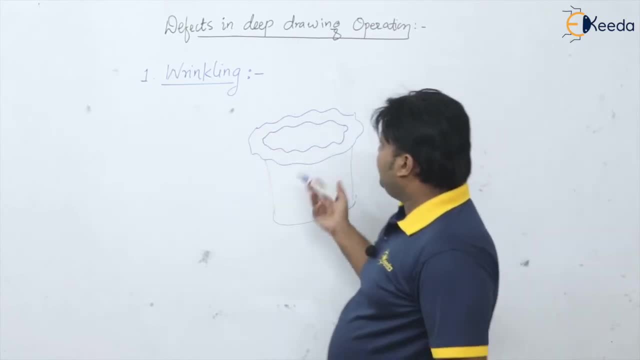 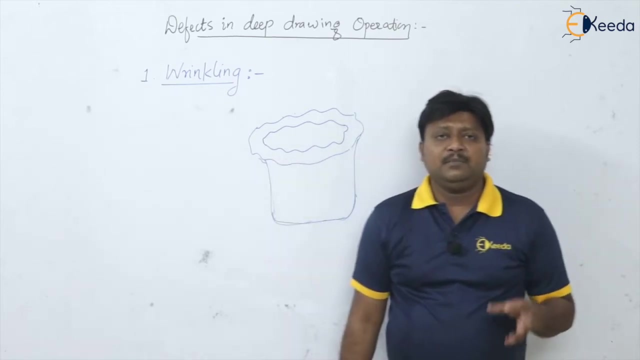 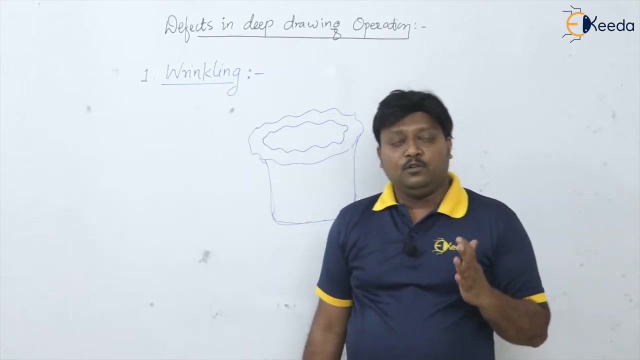 okay, so this is most common. so again, this is what material is flowing the radially, so we are getting this foldings, okay. so the main reason behind production of these wrinkles is basically the insufficient blank holding force. okay, so we have to provide the necessary blank holding force to avoid. 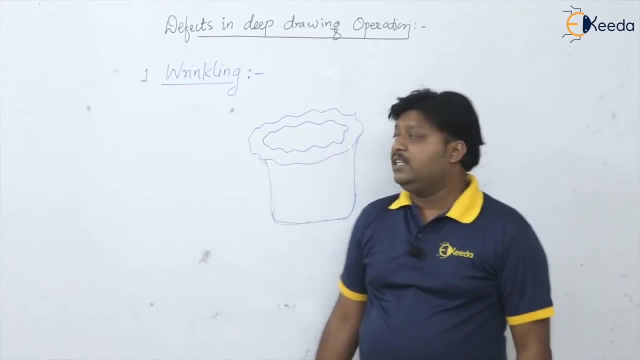 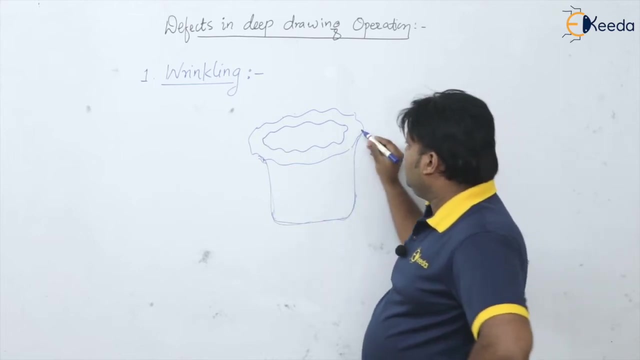 the lifting of the edges so that the folding will not produce, you can able to eliminate the defect called it as wrinkling, so actually the wrinkles which are present on this flange, these are the flange wrinkles. sometimes, what happens, the wrinkles can be extended up to the 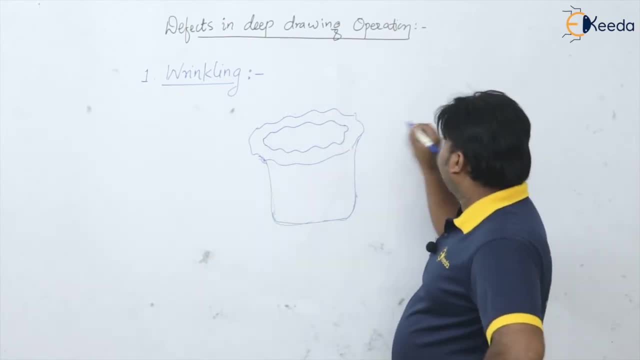 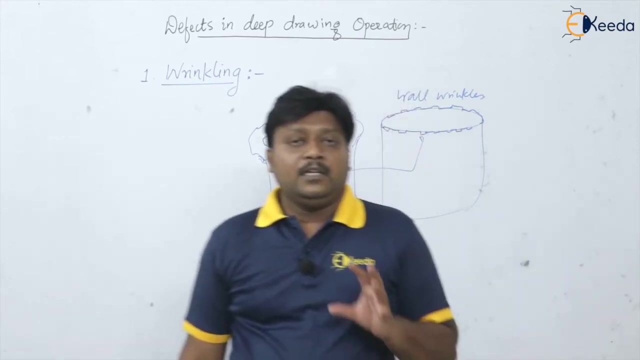 wall of the cup and say this is wall of the cup and it is now producing the wrinkles on the cup. wall of the cup like this: so this is our cup. okay, so these are known as the wall wrinkles. these are nothing, but these are the flange wrinkles, flange wrinkles and these are the wall wrinkles. okay, so these are wrinkling. so 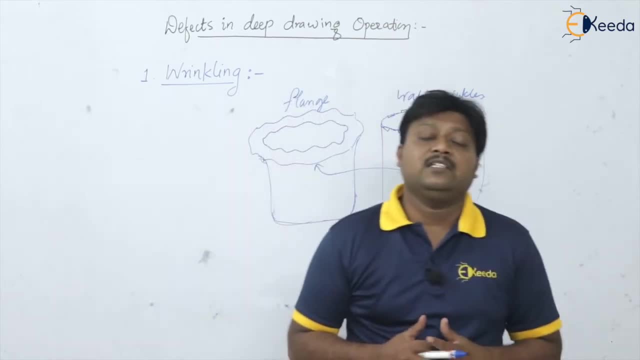 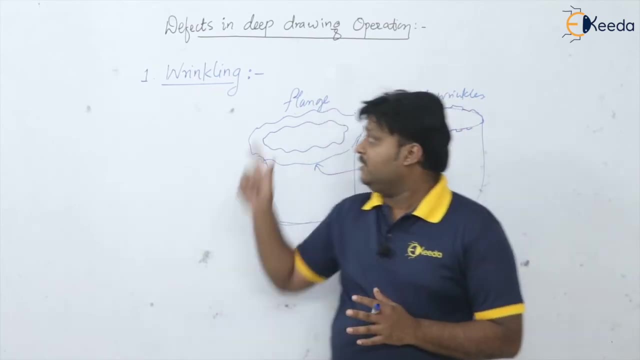 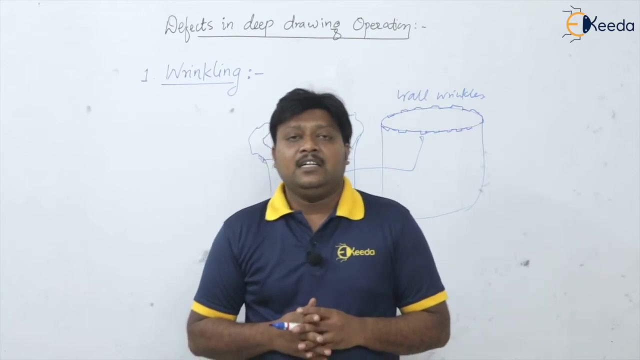 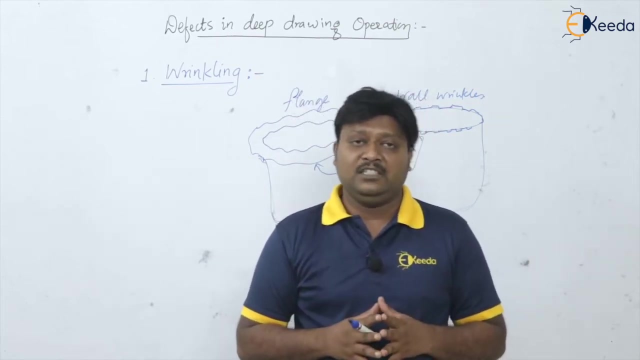 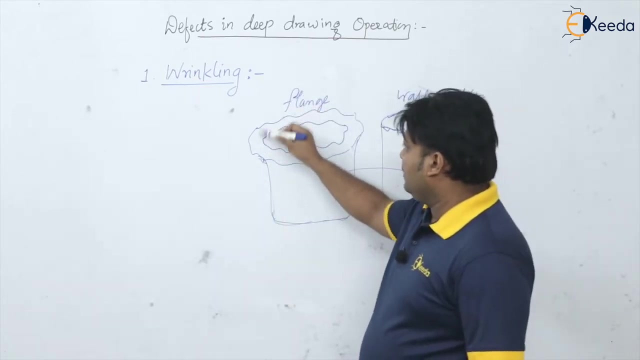 the main remedy for this is what we know. the main remedy for this is what we know: that we have to provide the sufficient amount of blank holding force so that the lifting get avoided and these wrinkles can be eliminated. now, the another remedy for to eliminate the wrinkles is that we know that in deep drawing operation, the clearance we have provided is generally equal to the thickness of the sheet. that is clear now, but in the deep drawing operation, this, this, nothing but this- wrinkles are. 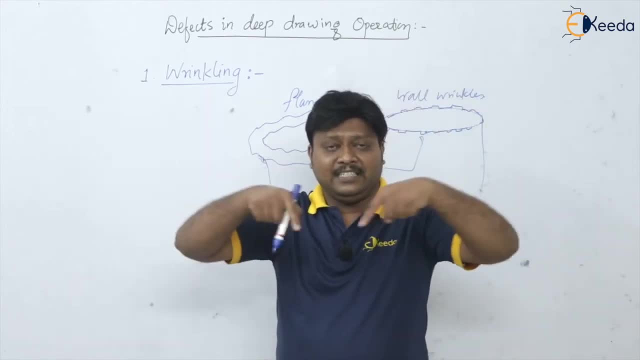 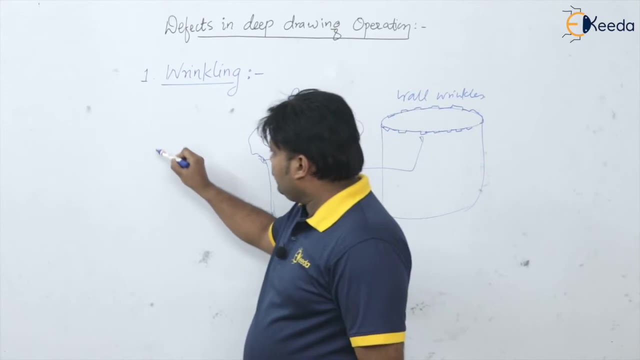 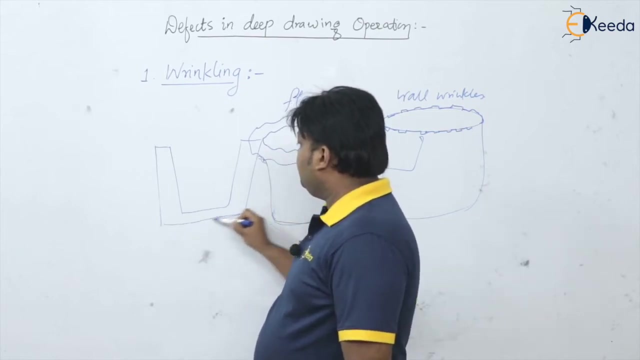 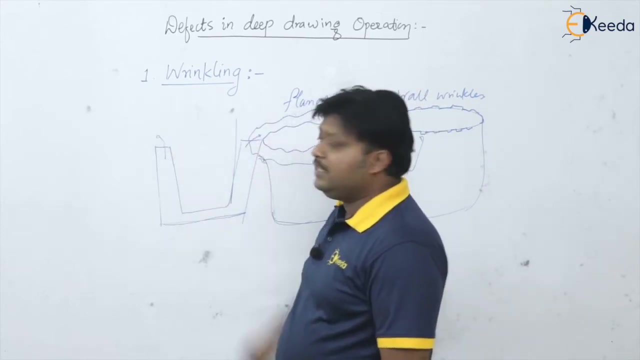 caused due to the flow of the material radial direction, in the radial direction. that's why these are folding, are getting produced. so actually, in deep drawn cup, you see the cross section, the side walls are becoming thicker than the bottom of the sheet. okay, so we can do, and this material is going to flow here in terms of the wrinkle it is going to generate. so what happened? 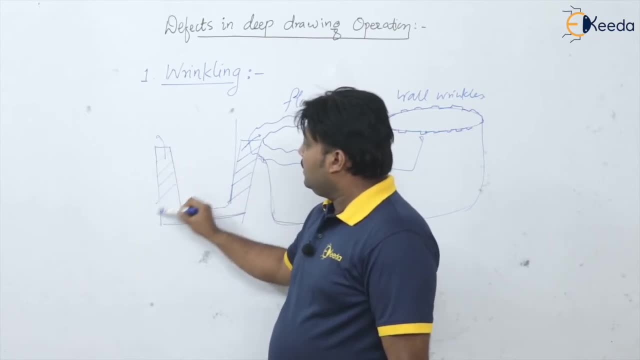 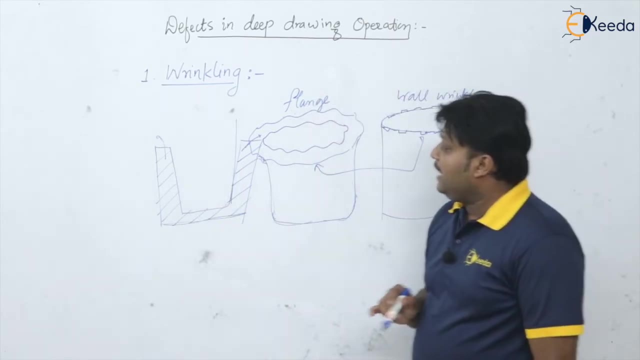 to help. and all this is going to be applied to the middle and third plate, so it's much easier so obtain to get this thinning easily by Kurtz. alright, this thickening of the sheet inside. what's of the curve? what we're building is that we are. 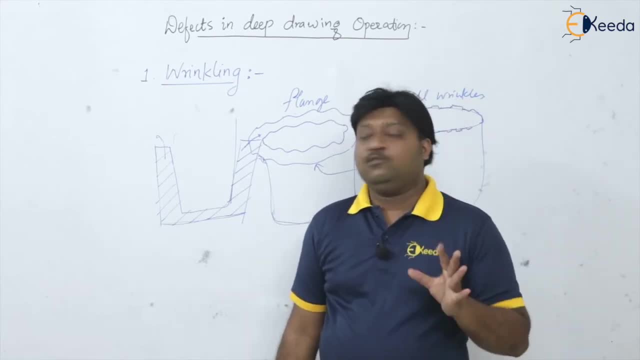 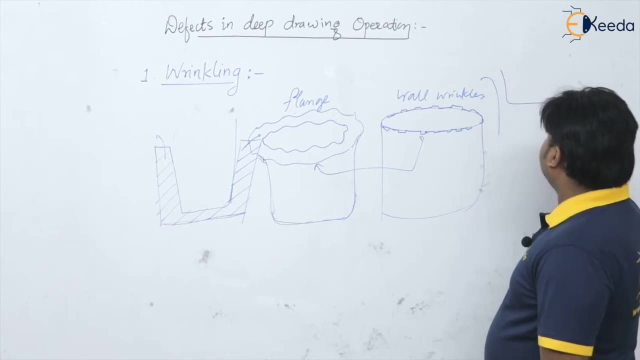 Providing this clearance in the deeper I have a patient is slightly less than the thickness of the sheet. okay, that's what we'll do. what will be happening did, if you aren't keeping the clearance in the seat- deer driver pressure- then definitely what is going to happen? this material getting squeezed, isn't it? and it will. 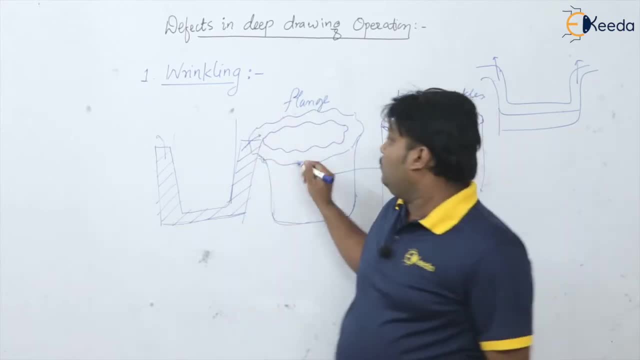 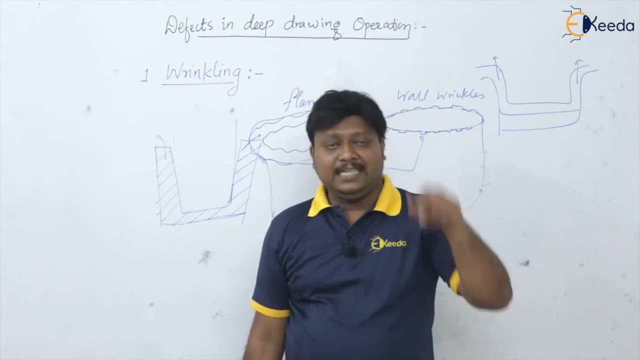 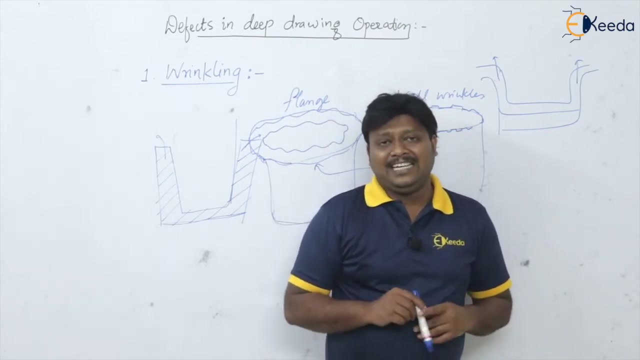 flow uniformly with the pressure so that it can go and equally distribute on the flange portion. so what happened actually? and that action or that effect is known as the ironing effect. so what is the ironing effect actually? that we want to squeeze that material from. 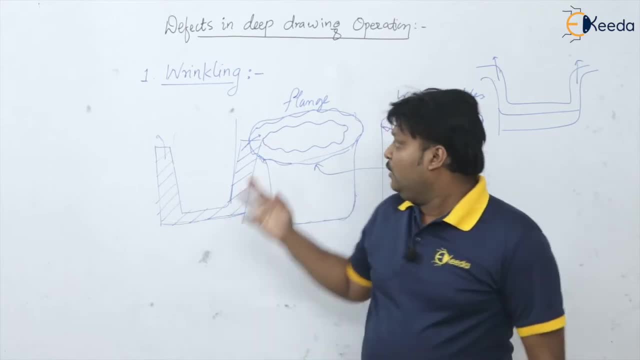 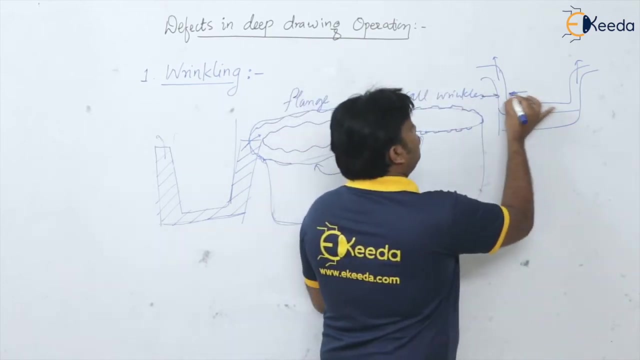 between the punch and die, so that we can able to eliminate this radial flow which is non-uniform, producing the foldings which are nothing but the wrinkles. so this effect, that is, provision of this clearance, this is clearance, you know and we know. deep drawing, it is thickness, but we are providing. 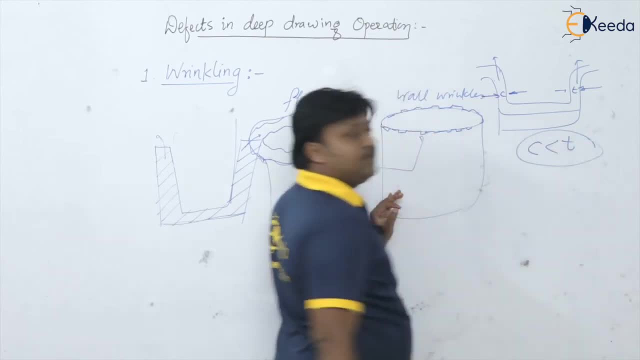 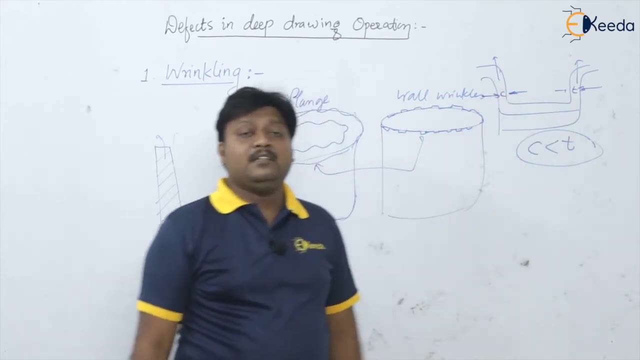 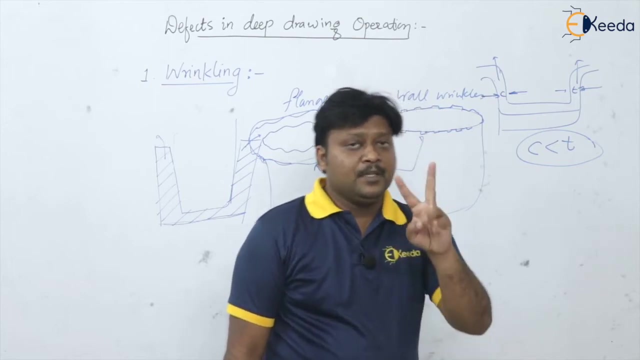 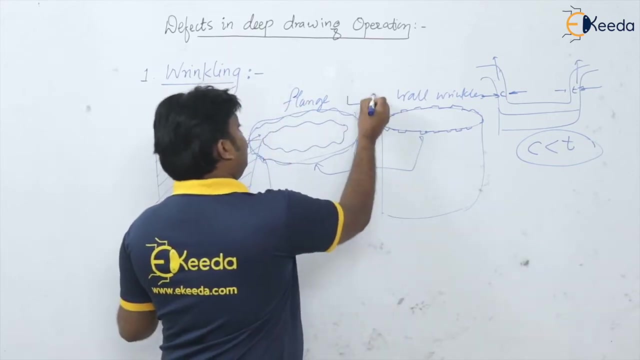 this clearance slightly less than the thickness of the plate. okay, that's why the material gets squeezed in between these. you gap and it can eliminate the wrinkles. okay, so first remedy: to have the sufficient amount of blank holding force. so on the edges you can have the blank holding force by using the spring loaded. 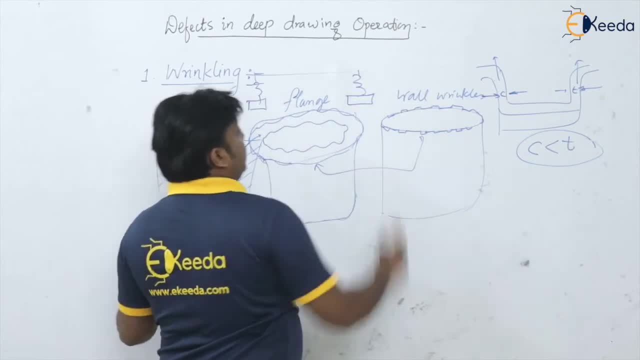 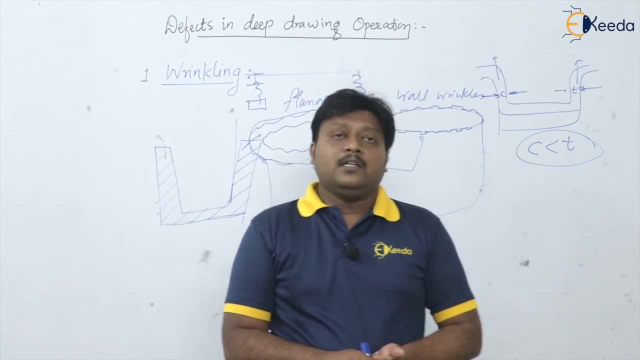 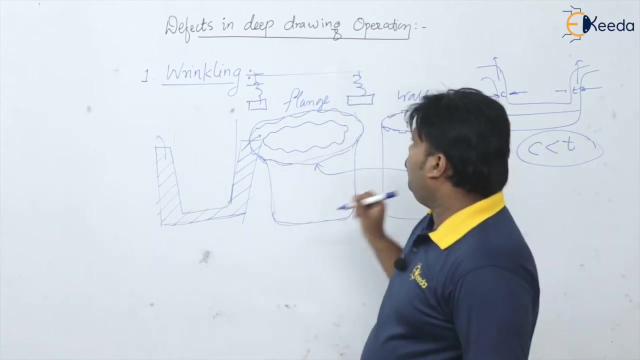 strippers. okay, and the second remedy that you have, that is the ironing effect. okay, now the third, and if you have blank to you, the angle of the iron it can also飛 over wasn't directly seen in the photo, or fossell, and so basicallyende the railing will admit a. 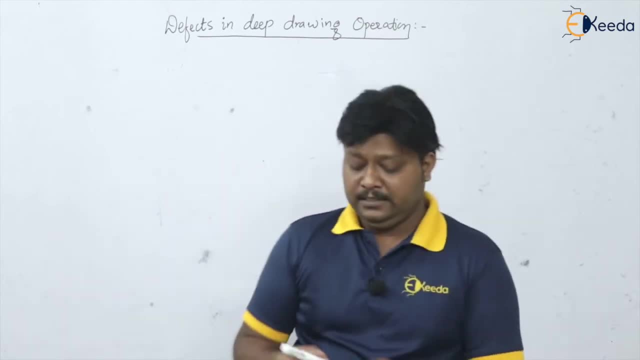 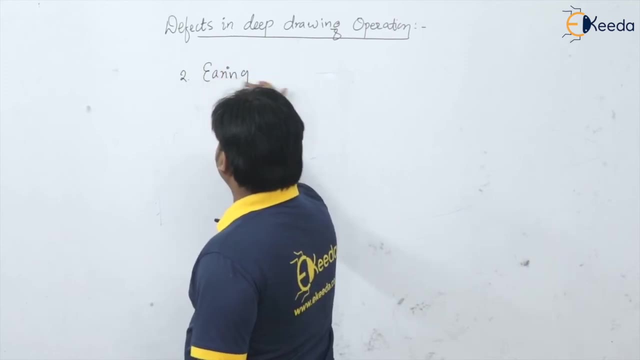 much higher direction, at the luxurious inner侧 direction also. and the next defect in the deep drawing operation is that the ear or lobs, the ear, very important, please remember. first defect is the wrinkles or wrinkling and the second defect that we are going to discuss is the earring. the earing or these are simplyeto avoid the ears or lobes where the outside layered experience. 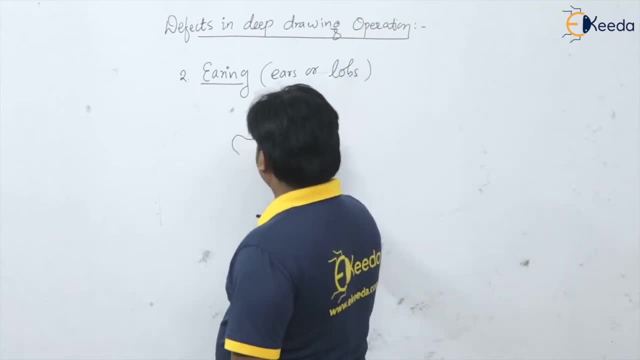 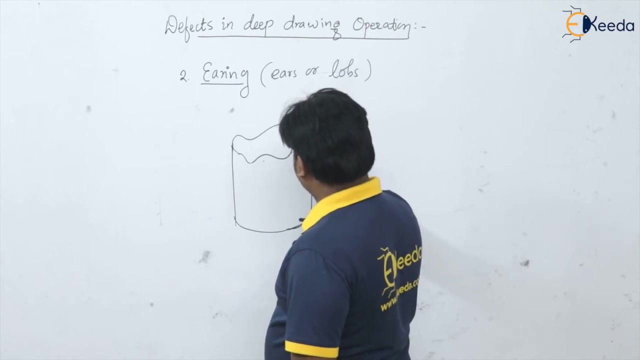 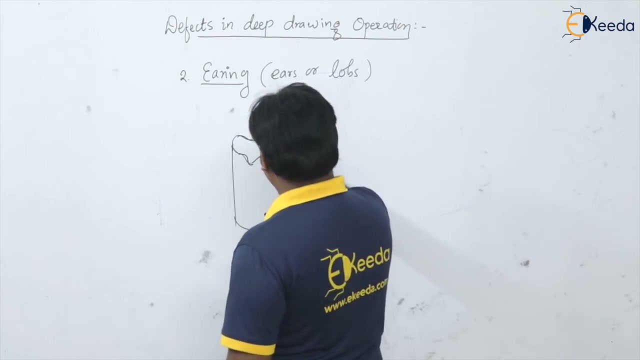 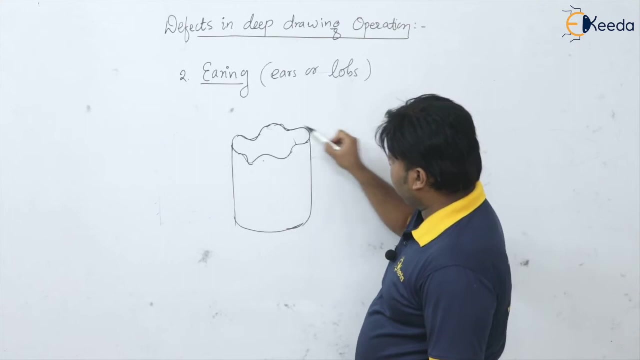 lobes where these are going to get produce. these are producing. on the vertical wall of the cup, on the wall of the cups, say: these are going to produce, so these are nothing but the lobes or ears. the lobes or ears, okay, so on the vertical wall. this is wall. you can have these ears now see. 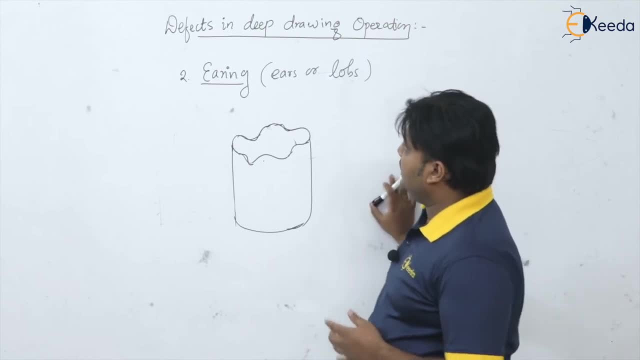 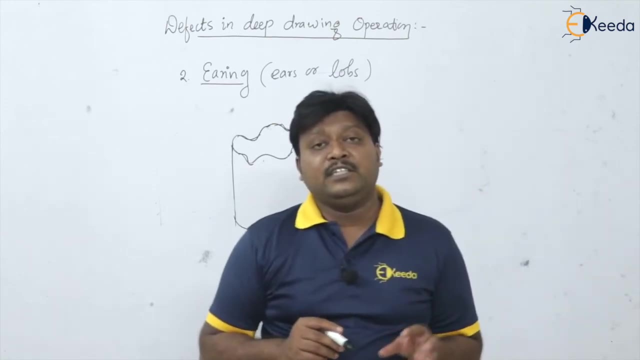 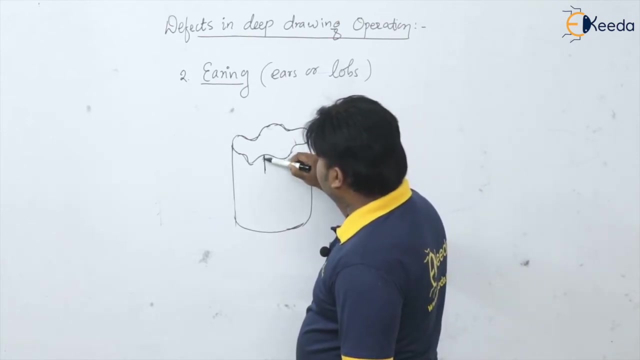 in the ears. you can also call it as the wrinkles which are present on the vertical wall of the cup are known as the ears, and the main reason for producing this earing effect is here you can have. the ear which is compressing, here is subjected to the compression, whereas the outer layer, which is coming out, it is. 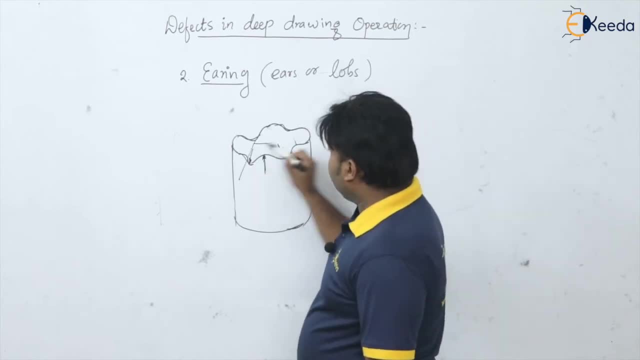 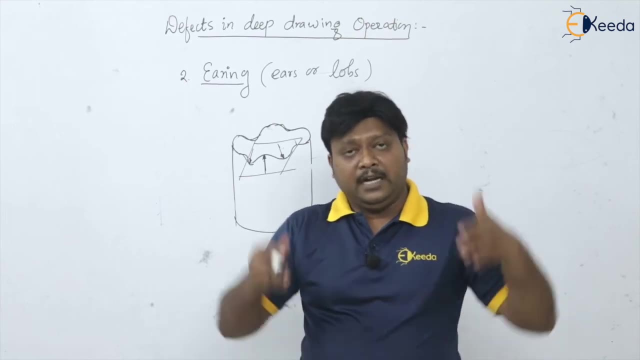 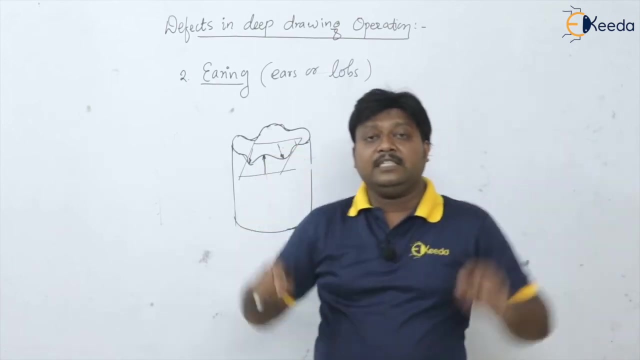 subjected to the tension. it is no so in a single plane. if you talk about this, so in a single plane, we are having different properties at: at inner surface of this ear, it is compression. at the outer surface of the ear, it is tension. so, in a single plane, if you are observing such a kind of 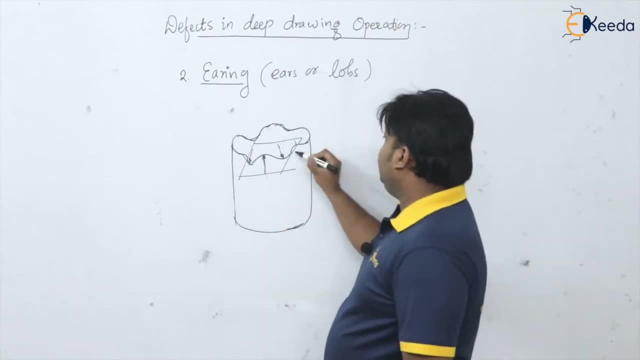 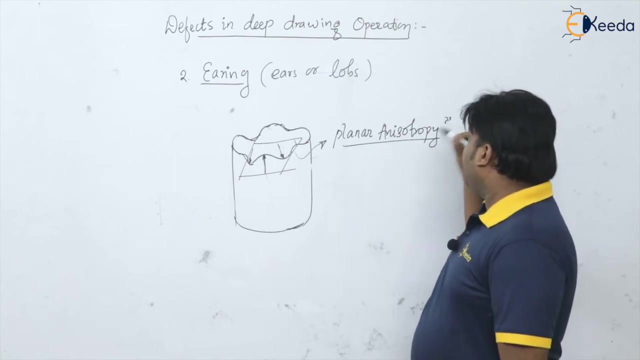 different properties. so definitely, this property is actually nothing but what? this is nothing but the planar anisotropy of the material: anisotropy at a point, in a directions, properties are changing. that is the planar anisotropy, and this is the reason for this production of this. 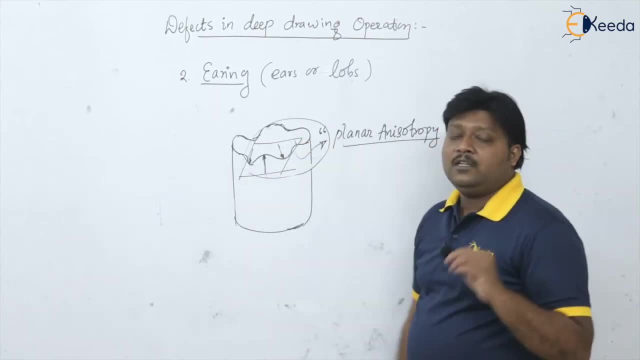 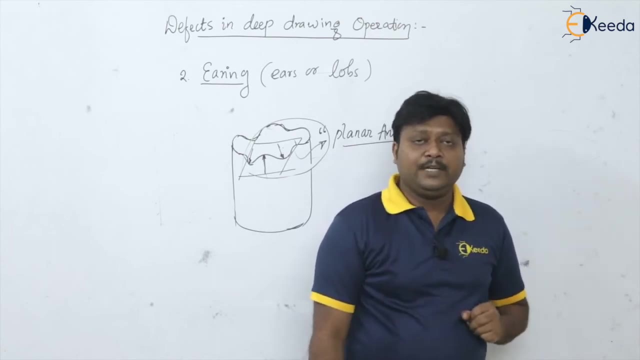 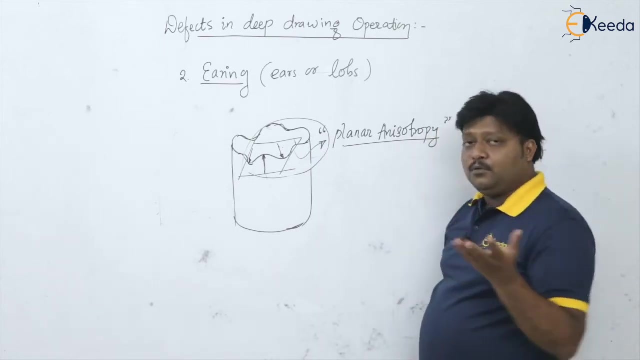 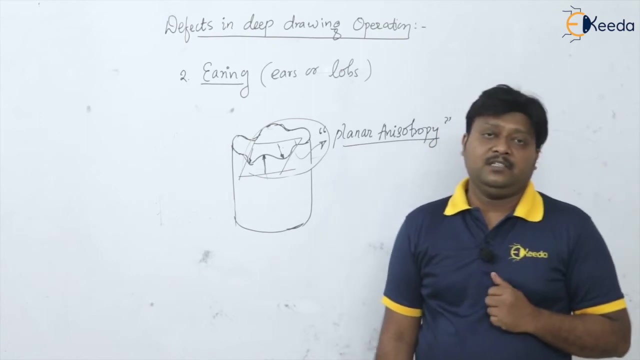 tension ears. okay, so the ears, or the lobes are going to produce because of the planar anisotropy, called it as the earring defect. okay, now how to minimize this earring defect? okay, so of course, the production of bhf is one thing. you can have the use of the drawbeads, the use of drawbeads, so. so this is the 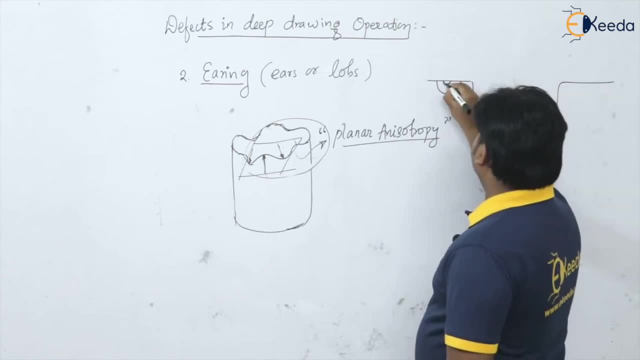 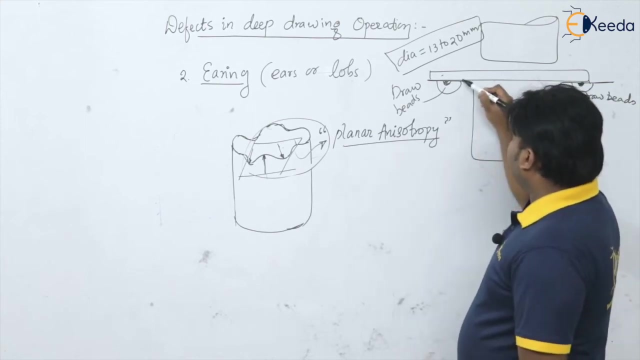 so the red 입ðr- Finnish of the draw bead. sorry, the diameter of the draw bead is actually from 30ちゃesses until 32 трساılar to 20 millimeter. please remember. diameter of the draw bit: 13 to 20 millimeter. but again, see. 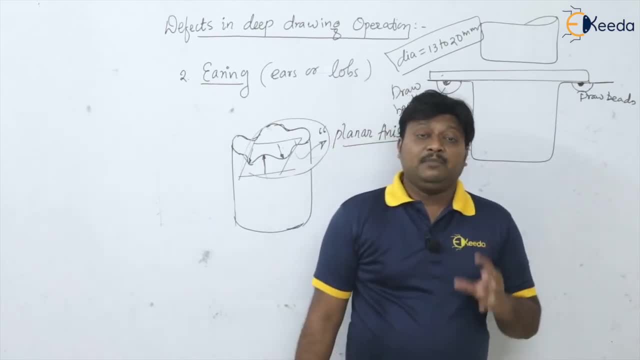 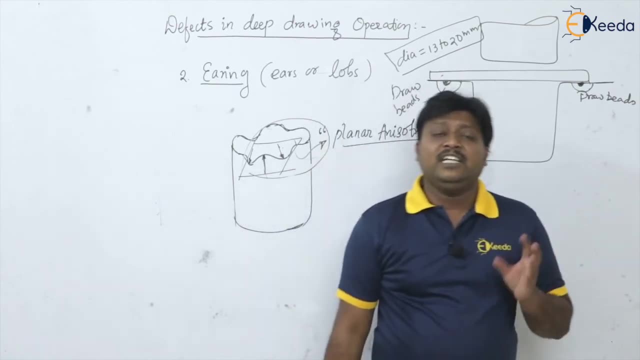 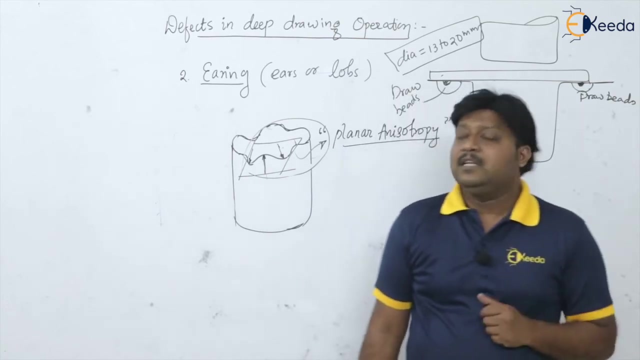 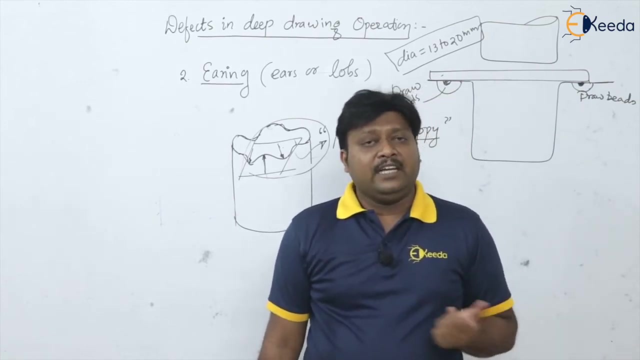 the earring defect is cannot get eliminated completely, even though the use of the dry use of the draw bits, using of the bhf, it is still present onto the, it is still present onto the cup. so that's why we have to use the trimming allowance, so it is not in our hand. so, ultimately, 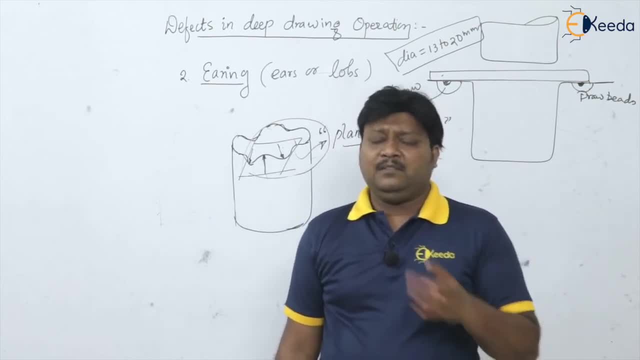 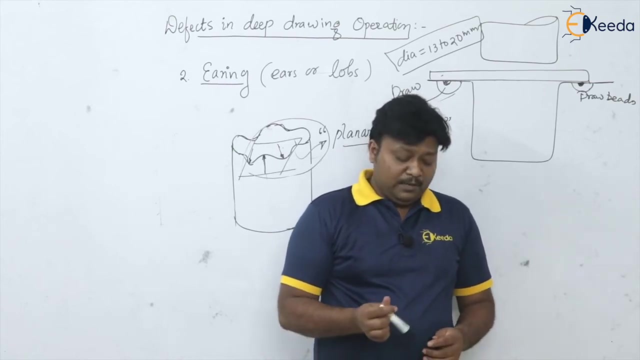 whatever the years are going to left, by doing this, by provision of the bhf, by doing this provision of the draw bits, whatever the years now left, they simply are going to cut it and you are going to get the required dimension. but what happen, as we are going to? 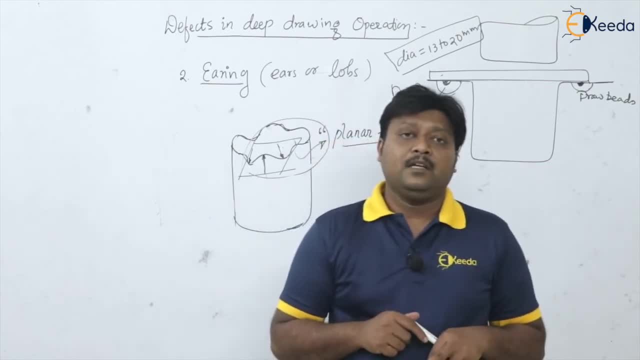 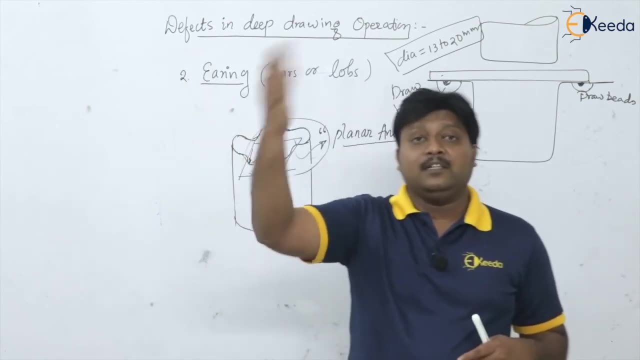 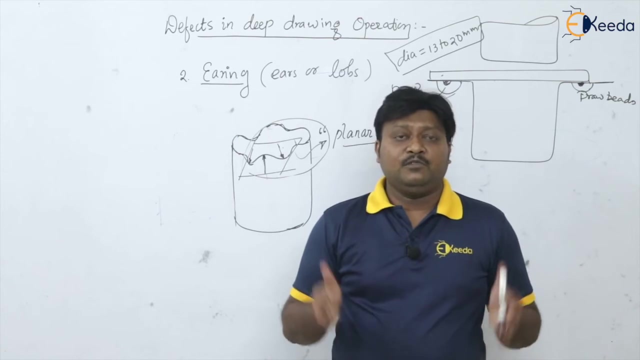 use this trimming allowance so you have to put the excess size okay so that it get. it can be get cut to after the process and it will give to the trimming allowance. so for that in advance, we have to provide this trimming allowance that these years are not going to leave. we. 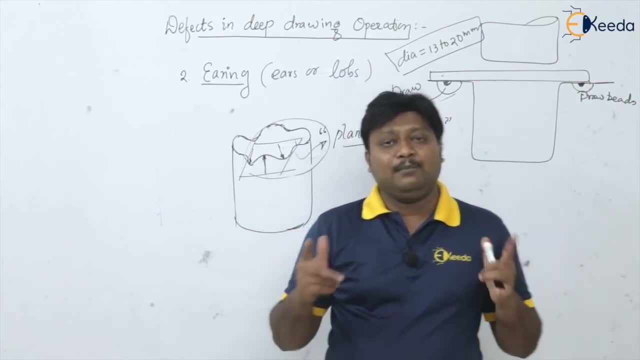 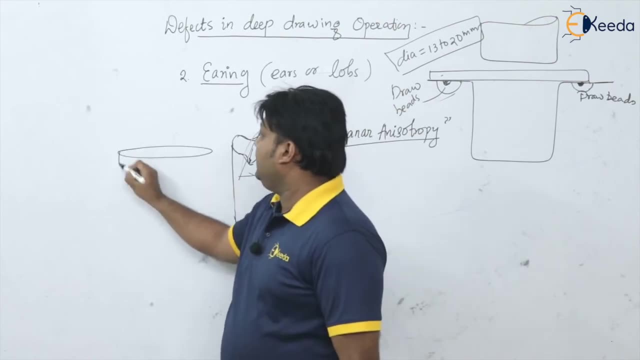 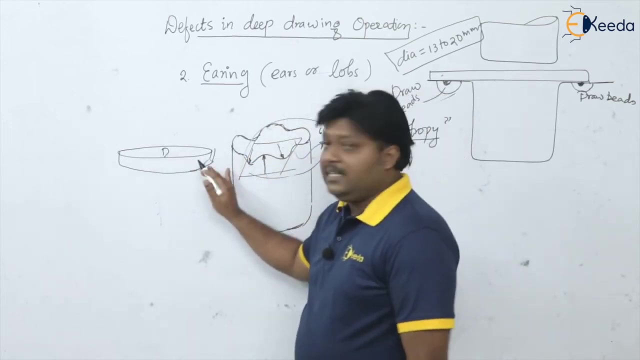 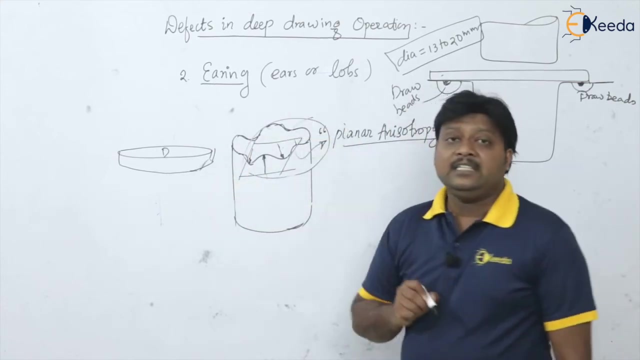 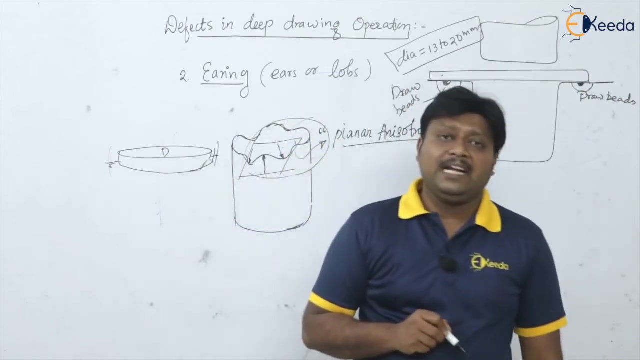 have to cut it finally and remove it. so we have to give some excess dimension on which the diameter- okay is- of the vinegar can say vinegar, it will make one made by this blank of diameter D okay, and we are finally going to spring this producer parameter to account for the years. so definitely I have to add some extra diameter on to the blank. 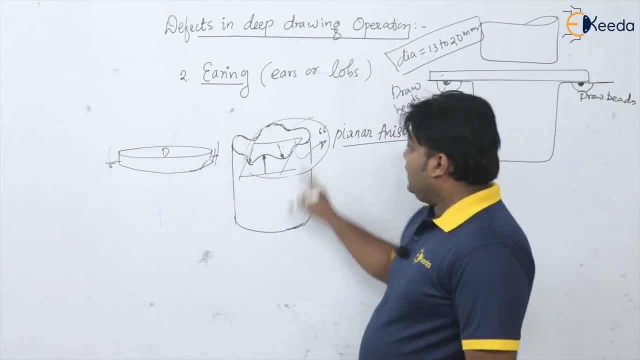 is, and it so at that time you can from 0 and 0. is some extra limits really? nhh a very important value of all right good, let us go into video. let us see how perthast canım opportunity of know what is going on. I do not have tovaisanúsica when this was known to be the men from her. 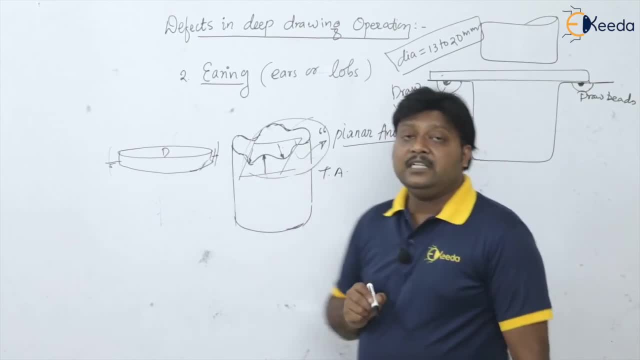 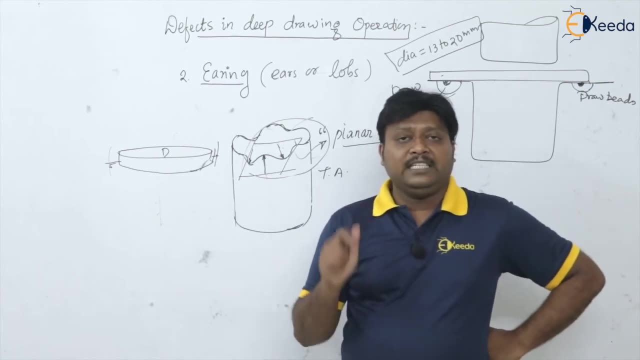 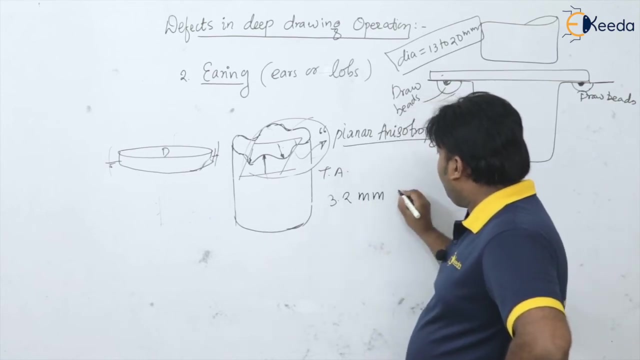 meditation П Dutch only toップ. so if you are a woman with Hernan being also given to by the allowance, if we are given with the trimming allowance, so by thumb rule- see, this is by thumb rule- it is given as 3.2 millimeter on 25 millimeter of the cup. 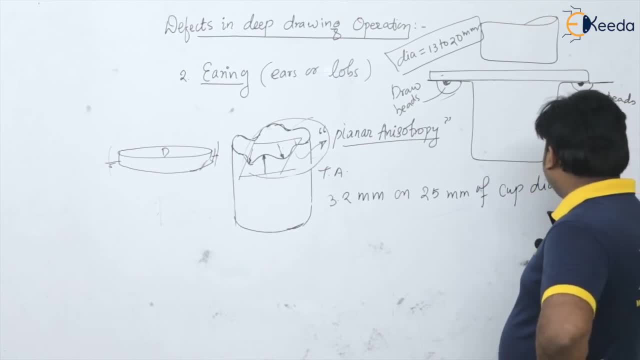 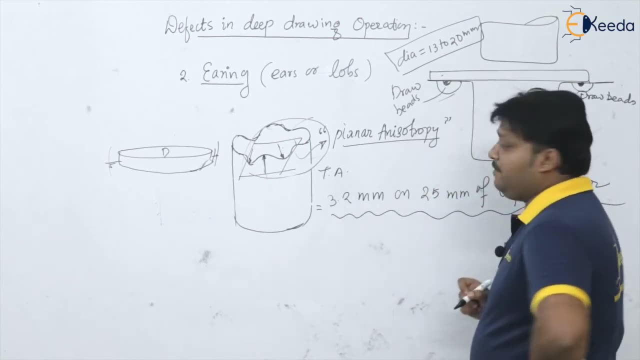 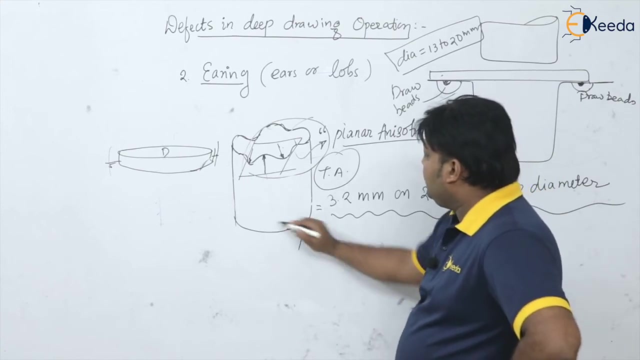 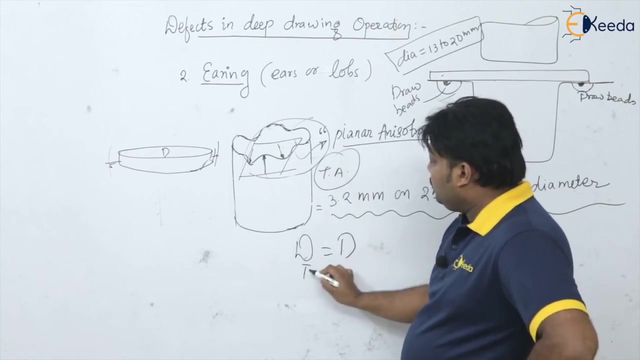 diameter, the cup diameter. please remember it how it is given as 3.2 mm on 25 millimeter of cup diameter, or if it is given radially directly, then it can be asked if you find out the diameter of the blank by provision of the trimming allowance. that is so D total- here I will write D total- is equal. 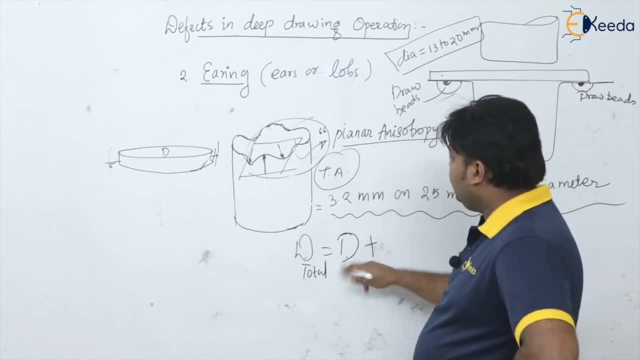 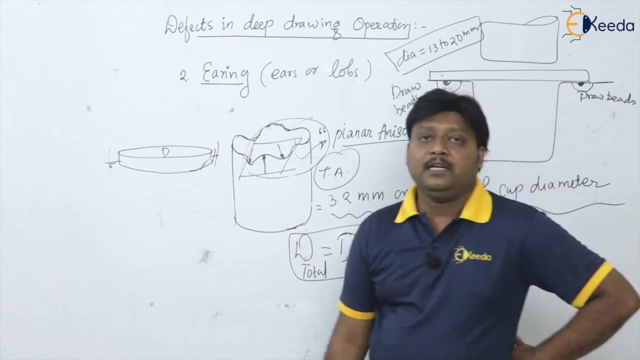 to D, that is our blank- says that you calculate the diameter of the cup diameter, and the diameter of the cup is calculated in that you have to add two times trimming allowance. like that you can add the trimming allowance. but thumb rule, kya kehta hai, you have to add 3 millimeter, or 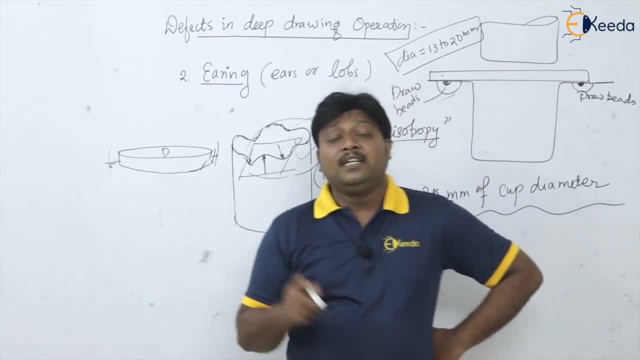 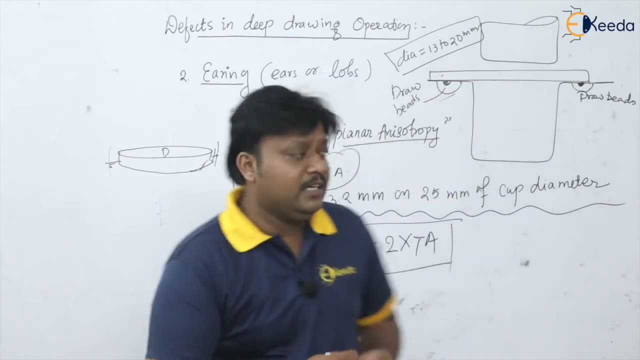 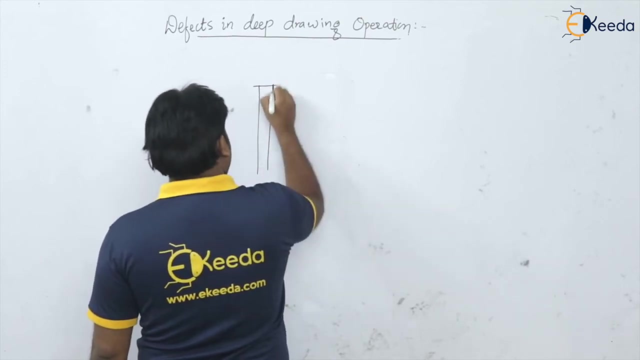 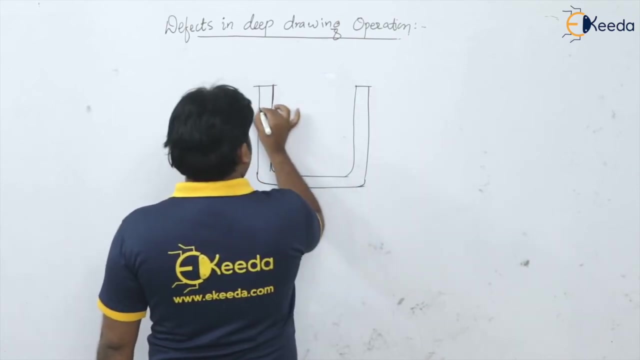 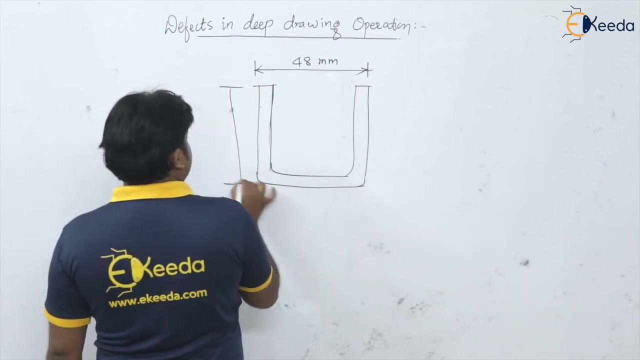 3.2 millimeter for every 25 millimeter of cup diameter and that you have to add into the capital D. let us take example that, so that you can able to understand. so say this is our cup, say 48 millimeter diameter and 48 millimeter height. okay, you are going to. 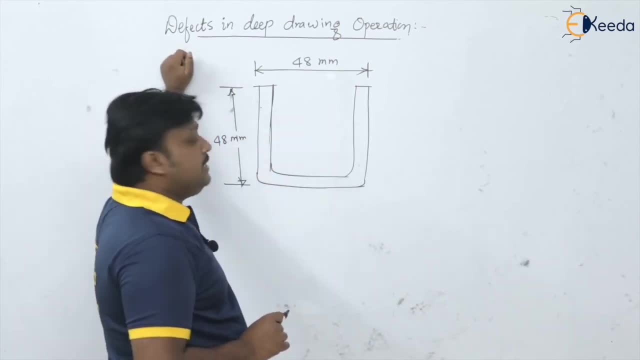 have the cup of 48 millimeter diameter and 48 millimeter. height of thickness: say 1, 8 millimeter diameter, 4 millimeter and 48 x 7 millimeter diameter: se agree, if you are, could calculate the diameter of the cup? say 28 Akbar comic ad and we are going to add 2 x 3 millimeter diameter. diameter of the cup of thickness: say 1 mm. cream of thickness: say 6 kal. Jesus, if you are, people are not upgrade because you can pay a вык Sépt. 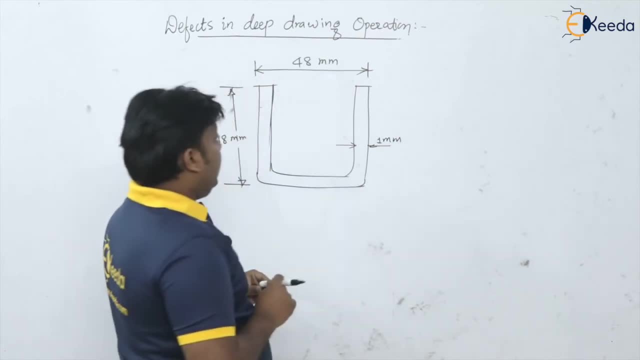 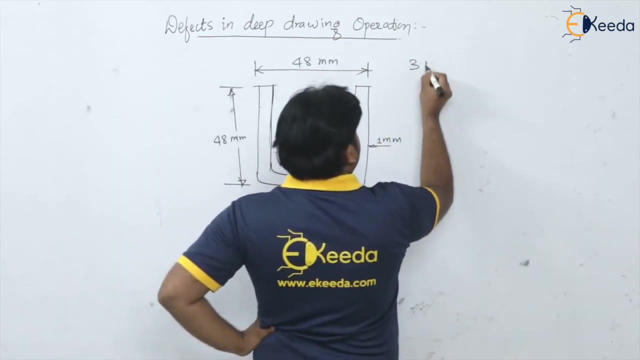 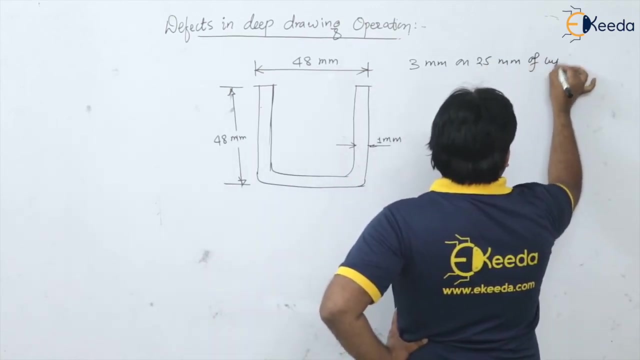 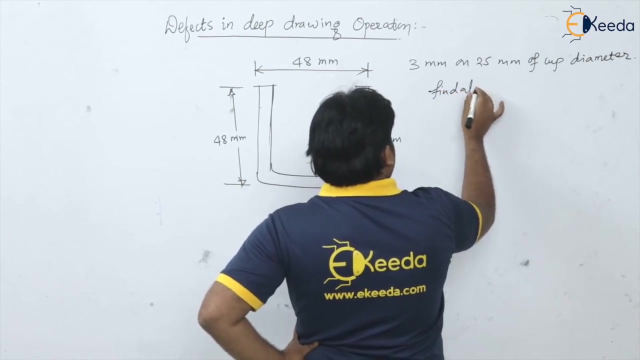 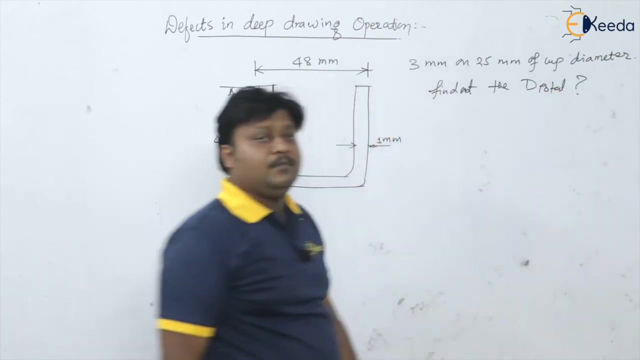 millimeter, okay, and in the numerical suppose I am saying that the trimming allowance is how much? say 3 millimeter on 25 millimeter of cup diameter. so find out, find out the D total. okay, so this is the actual blank side that we have to. 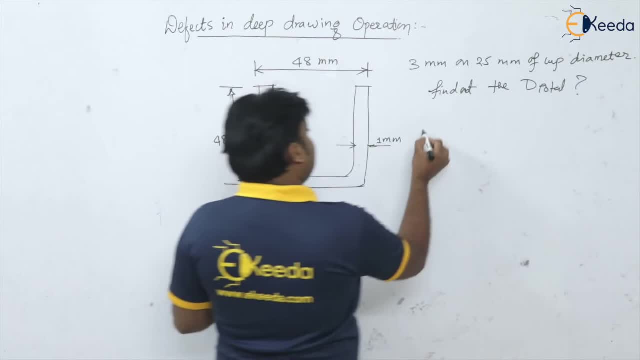 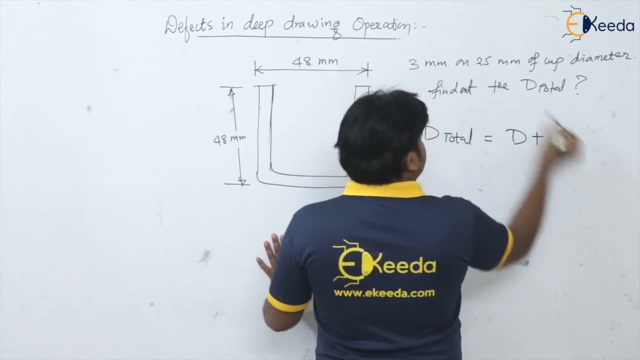 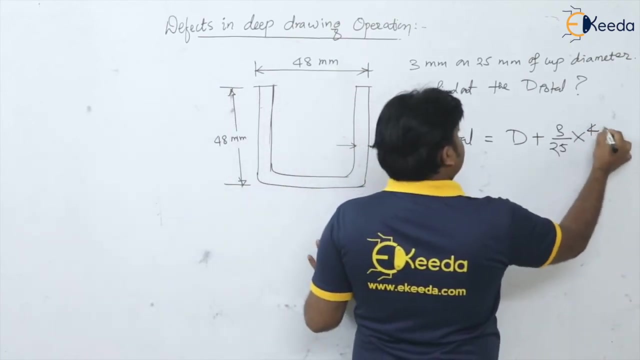 take in account of the trimming allowance, isn't it? so what is D total? D total- how to provide this? so D total will be D plus. this is 3 millimeter, or 25 mm for the cup diameter. cup diameter is 40 mm. so for that, first of all calculate these blank sides. D is equal to what under: 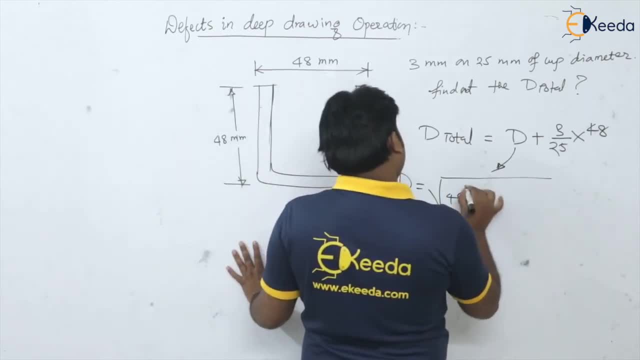 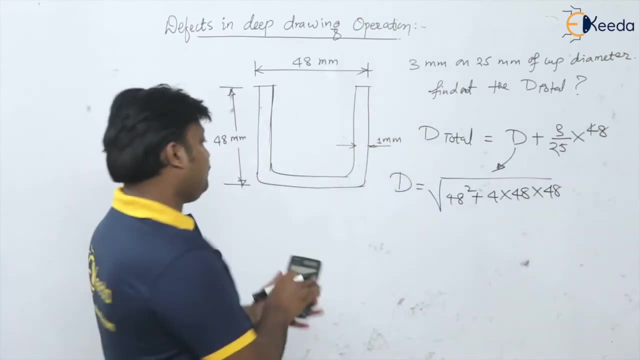 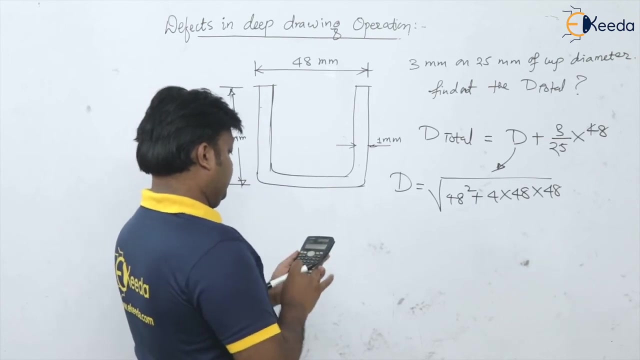 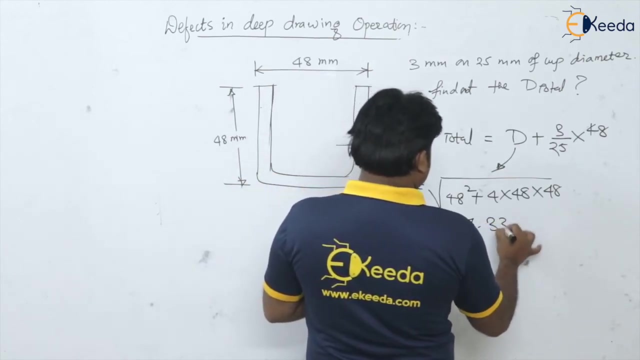 root of D square plus 4 DH. so diameter 48 square plus 4 times 48 diameter and height also 48. so if I calculate so 48 square into 4 plus 48, square root of answer it is around one, not seven, point three, three. 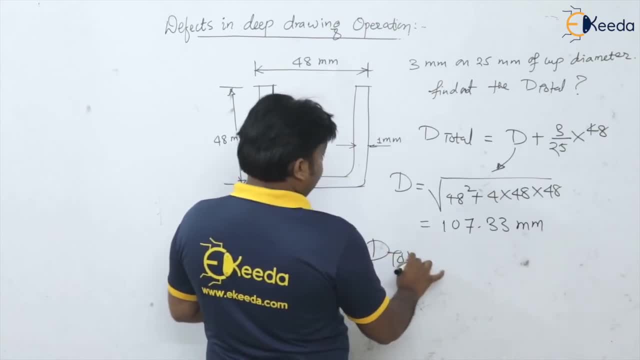 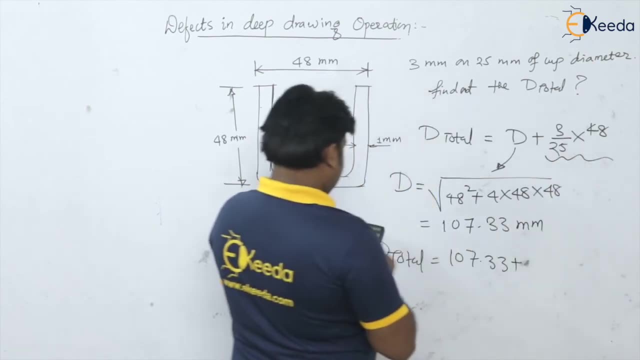 eight millimeter. so for that, first of all calculate these blank sides. D is equal to three millimeter. so what is the value of D total? so D total will be one, not seven point three, three plus this is this value. how much for tea at into 3 divided. 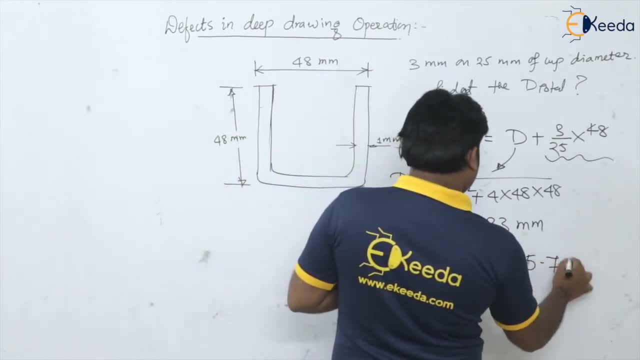 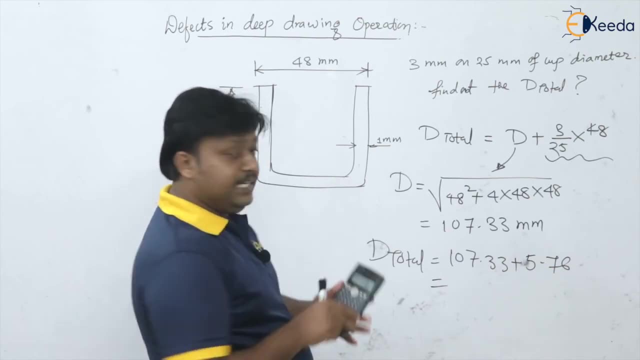 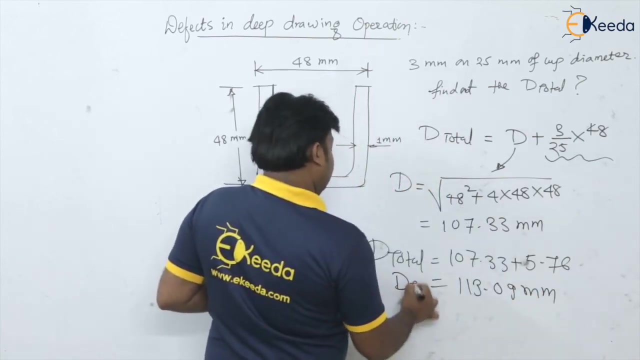 by 24, so it is five point seven six. so it is your D total, plus one zero seven point three, three. so one one three point zero nine. one one three point zero nine millimeter is your d total, that is. this is the theoretical blank size, but when you are 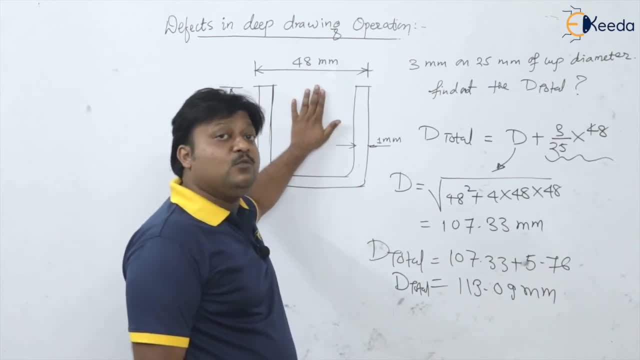 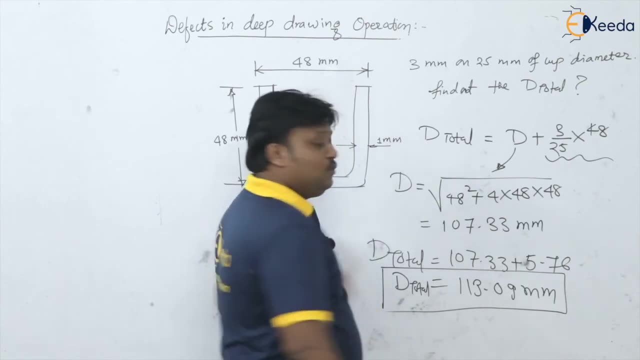 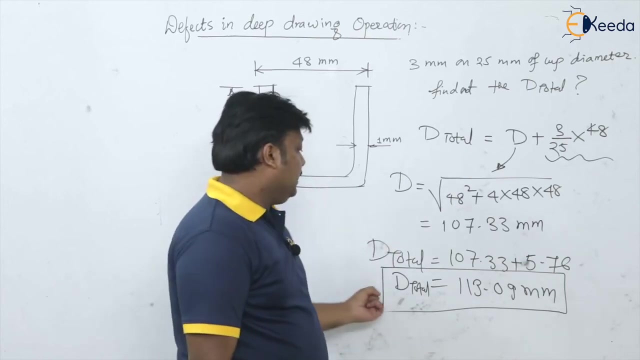 accounting the years also here that they are going to cut by provision of the trimming allowance. this will be the actual diameter that you have to put for the blank size. okay, so this is how we can able to calculate the uh actual blank size by provision of the. 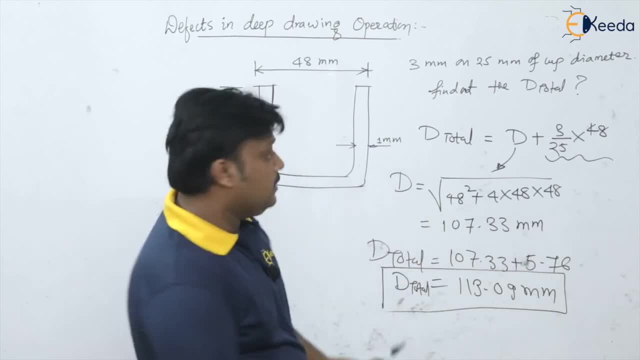 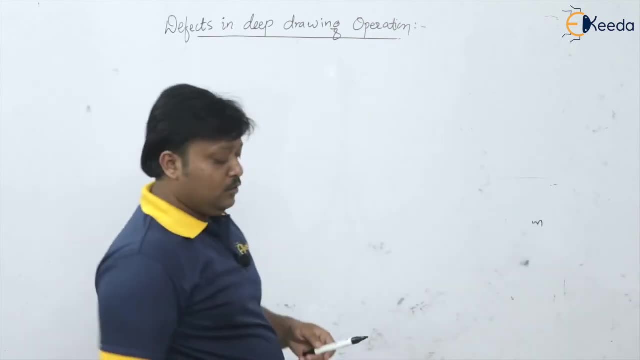 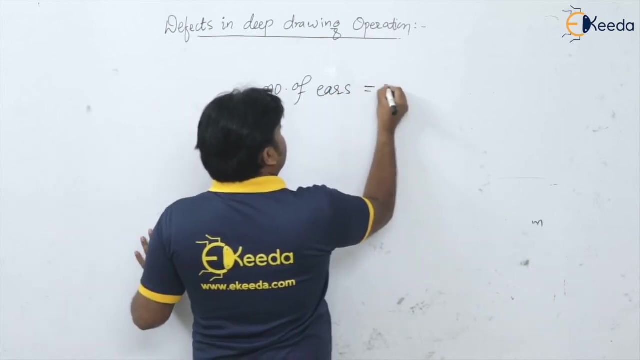 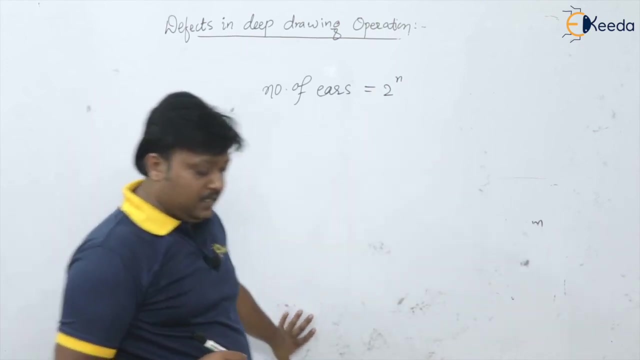 remaining allowance. okay, now see these number of years that are produced in the deep drawing operation. so see this in the earring defect: the number of years can be given as two to the power n. okay, how to get the number of years it is given as two to the power n. where n is the integer? 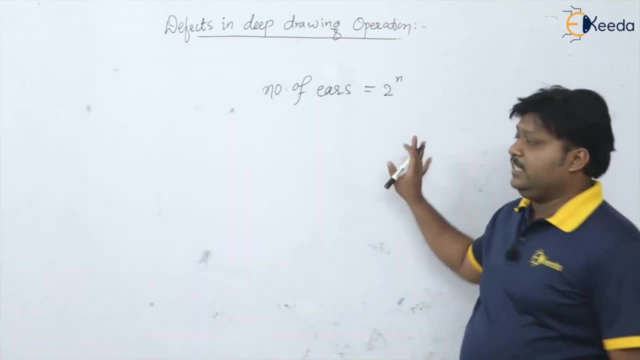 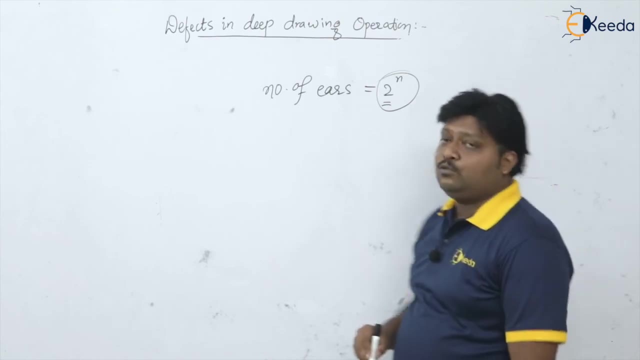 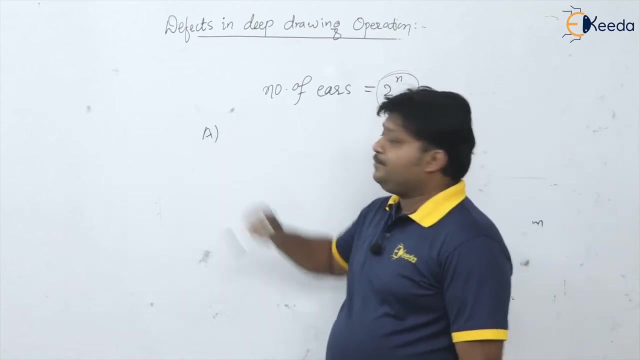 which values depend upon the properties of material friction. bending all these conditions, so generally, please remember that so number of years are given as 2 to the power n. so suppose in the examination they ask you to calculate and the options are okay. say it is 14, option b is 25, option c is: 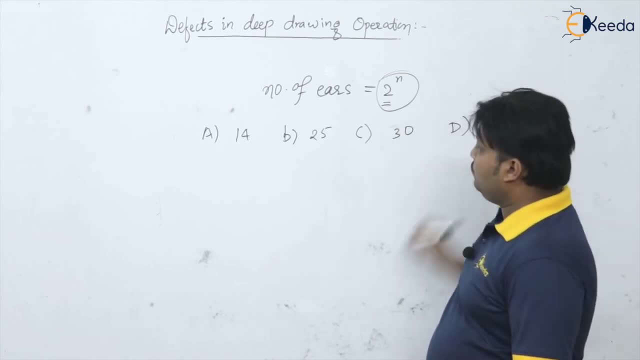 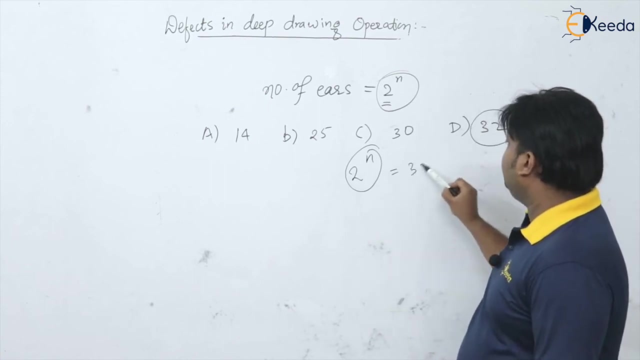 say 30 and option d is 32. okay, so what will be the answer to calculate the number of years if they ask? so it should be 2 to the power in terms of this. so the answer is only what? 32, isn't it? 32 should be the answer, that is 2 to the power. if i say: 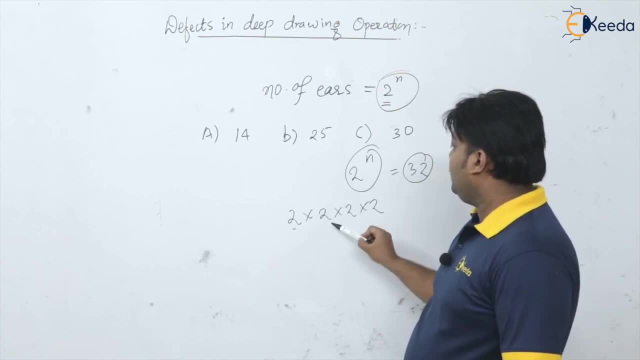 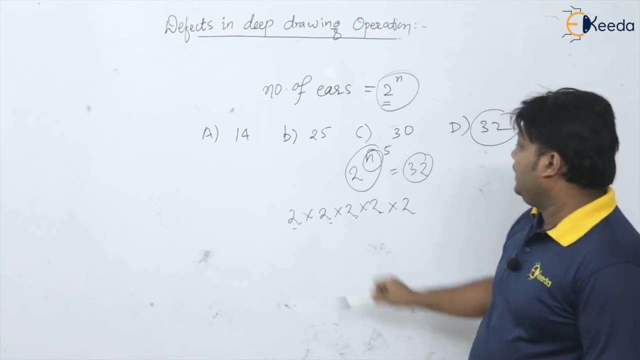 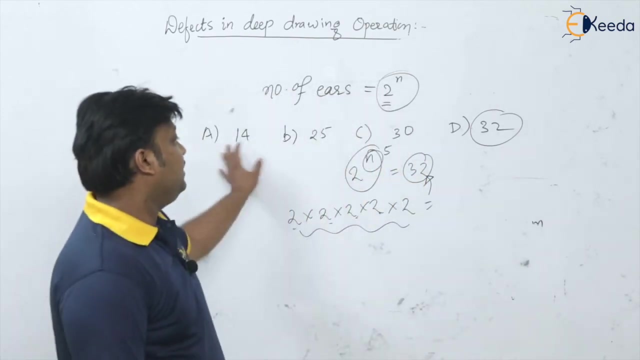 2 by 2. by 2 by 2, 2 twos are 4, twos are 8, 8, twos are 16, twos are 30. that is n. here is 5. okay, then, and only we are get this 32. so number of years produced are how much the 32? 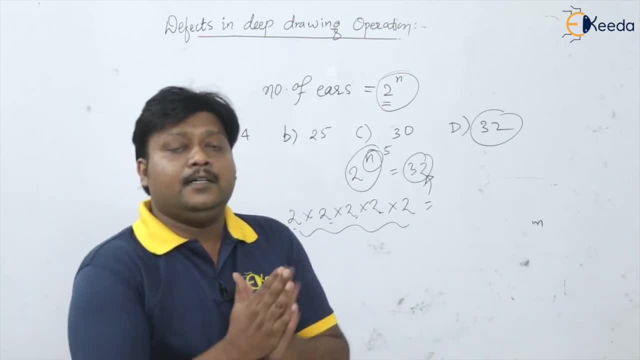 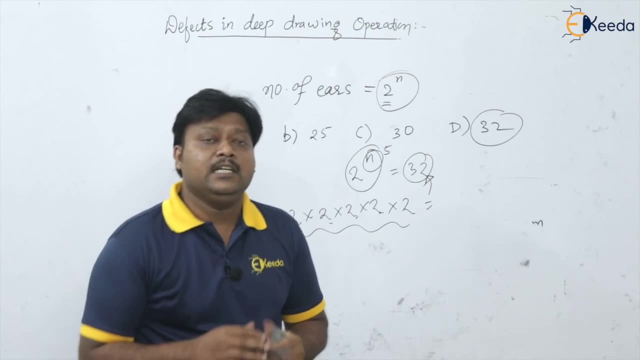 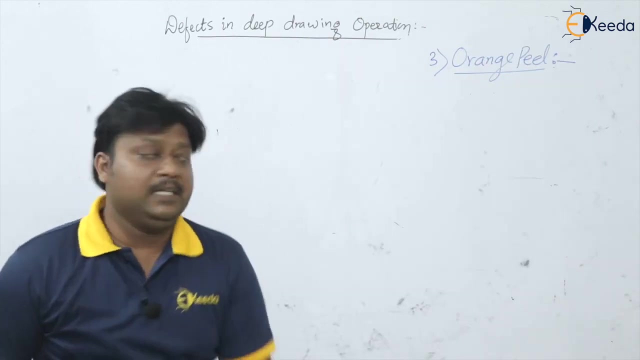 so this is the second uh defect and the remedy for that we have seen. now the third important effect in the deep drawing operation is the orange spill. the third defect is what orange? so this orange pill? this is kind of metallurgical defect which is what we are going to use in the TRPT to 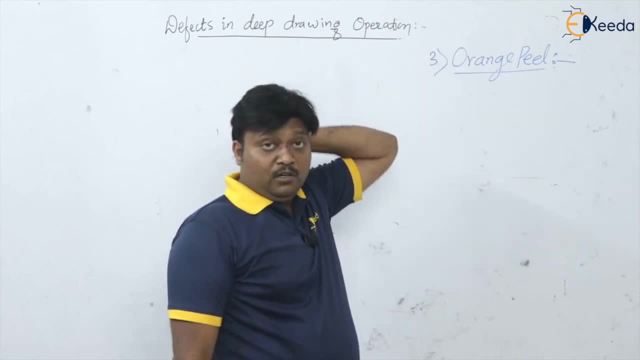 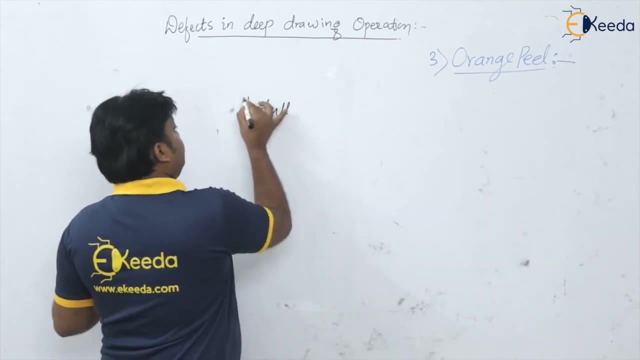 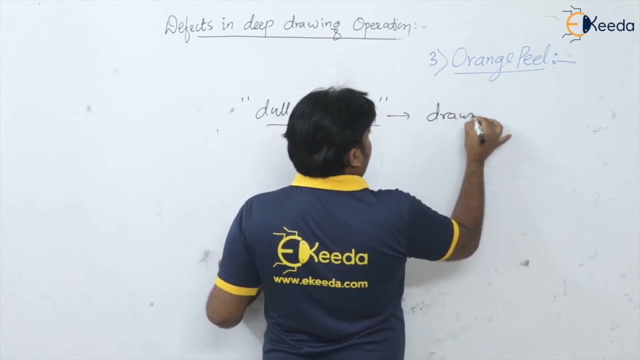 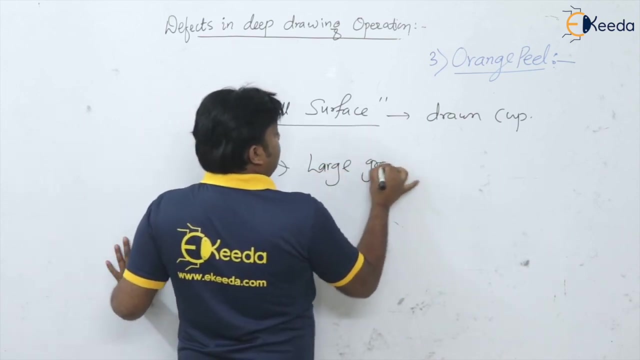 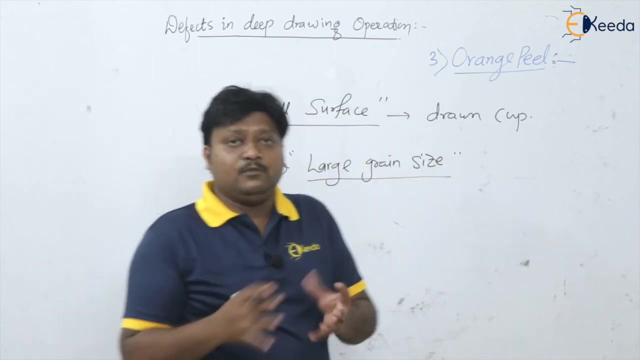 defect that is going to produce in the deep drawn component where we are get the dull surface. how you can see dull surface. you are getting on the drawn cup, on to the drawn. it is because of what: the large grain size. this is because of large grain size, you are getting the surface which is you can see on the 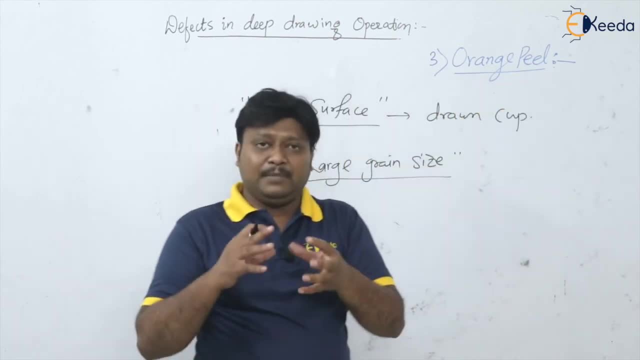 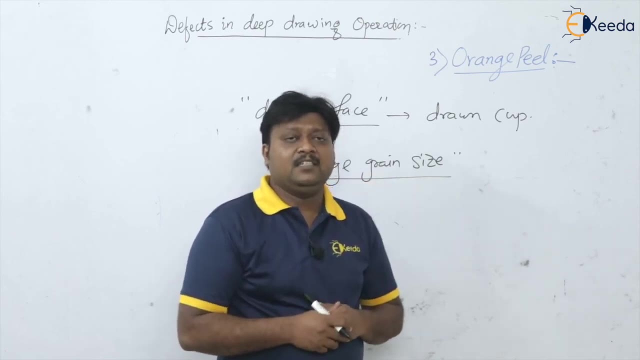 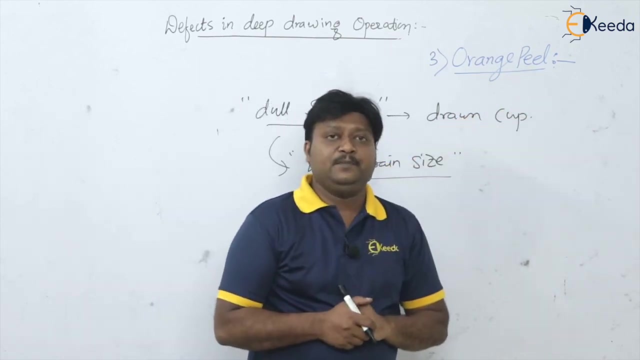 orange, orange, that kind of surface. this is a metallurgical defect. you can get on to the drawn cup. okay, the dust surface, which is because of the large grain sides. their defect is known as the orange. okay, these are the Okay thersere are the main froze of crates. okay, well, the right side source of Abdul gum Una Bar, worshлишwood, çevin przed James 컬 위� Djâild이.